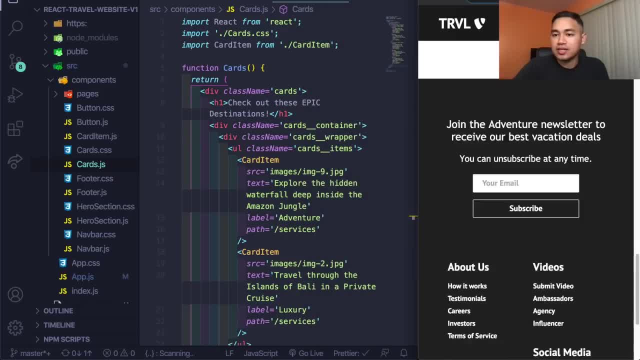 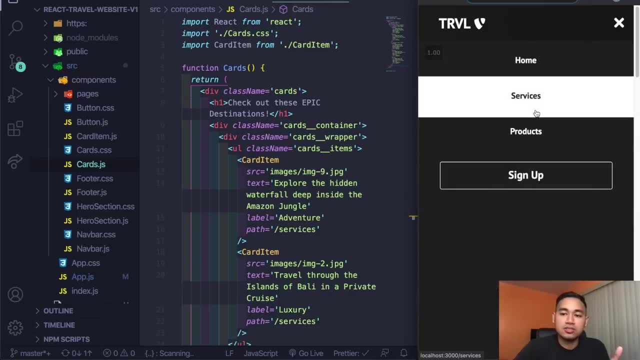 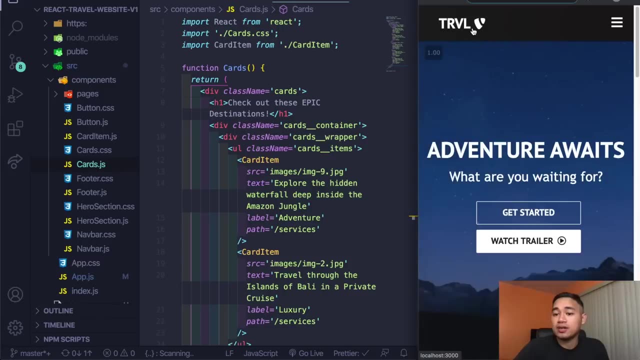 like this, and then we shrink it down like that. and then, last but not least, is the mobile hamburger menu. obviously we got that going on here and also, when we click on any of these, they switch the page and they close out the menu. and then like, for instance, even if i click on the home icon, it does. 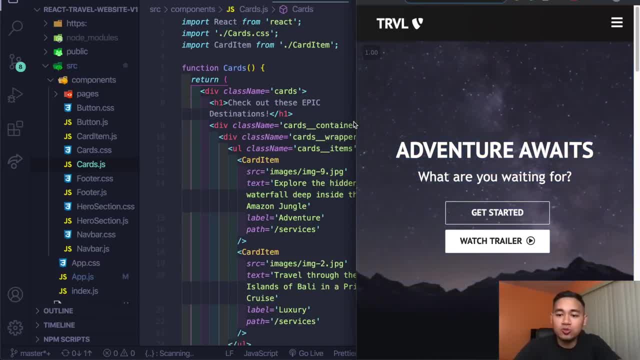 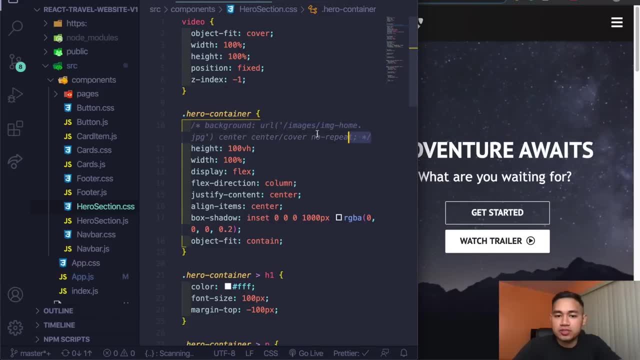 like this. and one thing i want to show you that's pretty cool too is we don't have to use a video, so let me just go over to. let's just show this. watch this. so if i go here, actually let me show you another video first. that's a little cooler than this one, i think at least, so let's change it up. 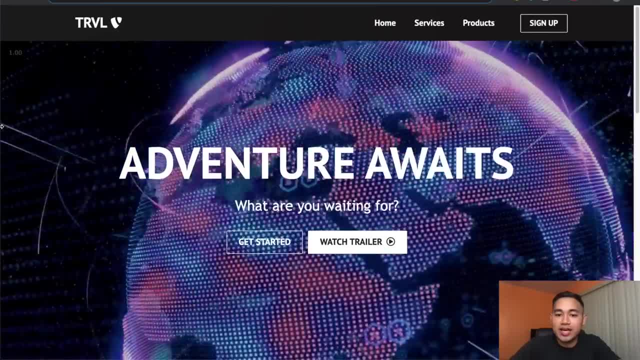 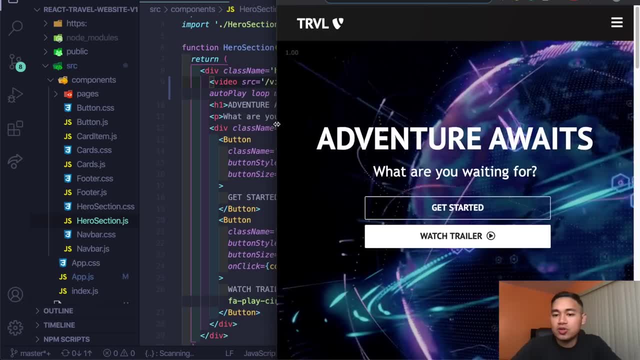 here, and then i go over here and refresh it and we can see that we can add this video too, and i'll also uh, link all these files to you so you can use these or you can use your own. and then, if you're like, yo, i don't want to use a video, i want to put a picture. we can just go here and basically let me. 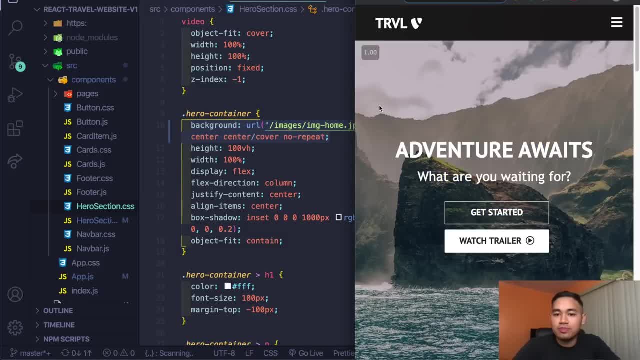 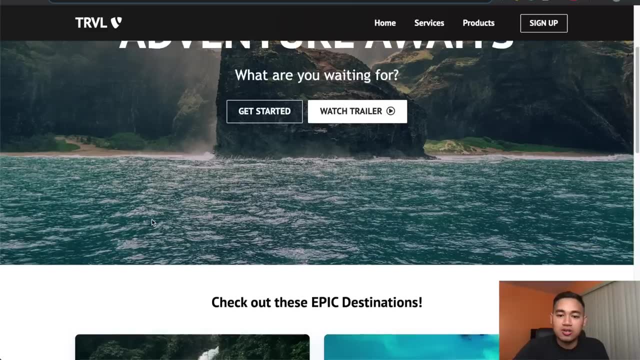 uncomment this line out, save it. boom, we're going to go ahead and save this and then we're going to scroll out and now we have it here. so this is my original design i had beforehand, but i want to get a little fancier with the videos. but you can see this fits sort of the um, the travel theme here, and 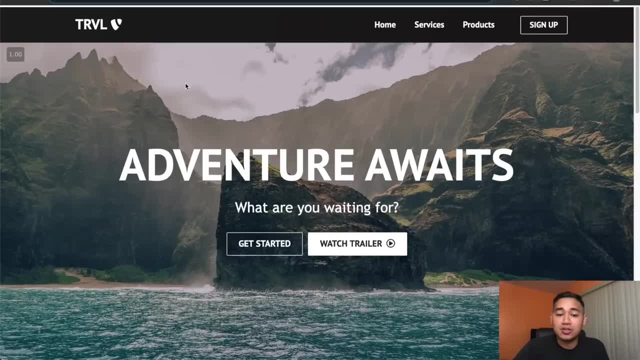 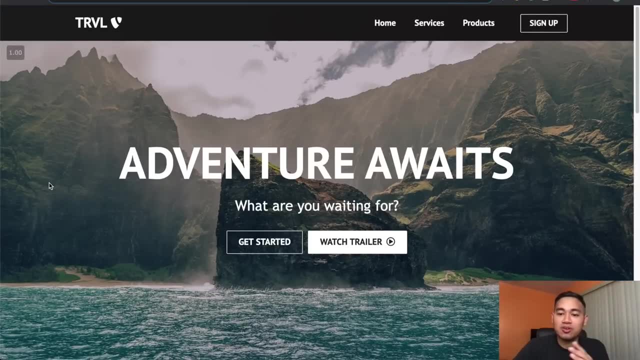 right now the video. technically it's like in the background because i still have it in my code, but ideally this is what it looks like and it's lagging just because i'm recording at the same time. so on your actual um browser this probably would not happen. but yeah, this is what we're. 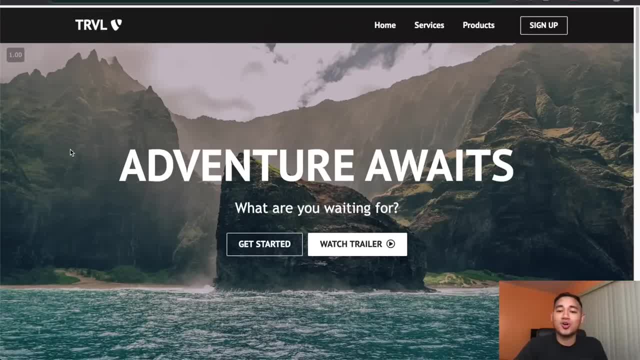 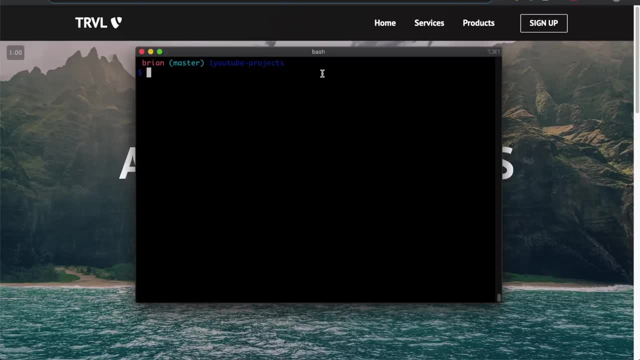 going to create today. so, without further ado, let's hop into our code editor and let's get started. all right, so here i am, on my terminal. so the very first thing is we're going to create a react app. so i'm going to go ahead and make sure in the place where you want your files to be. 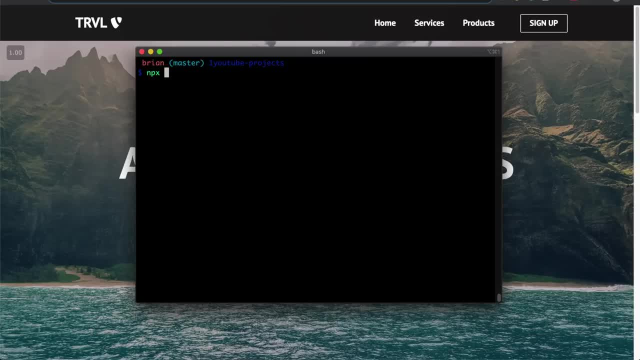 created. so here i am on mine and i'm going to go npx, create dash, react dash app, and then i'm going to name this react website yt for youtube and put one, and then i press enter and then, as this loads up, once it is done, then we can go ahead and get started. and also, depending on your computer, it 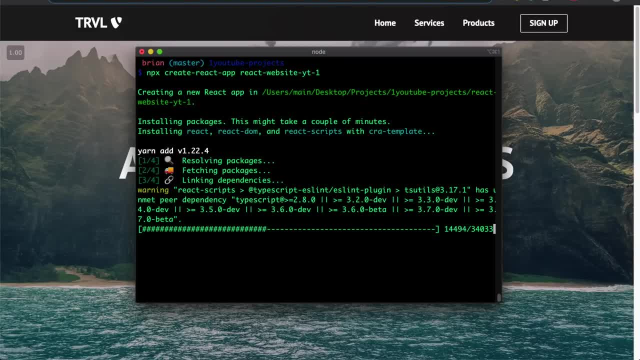 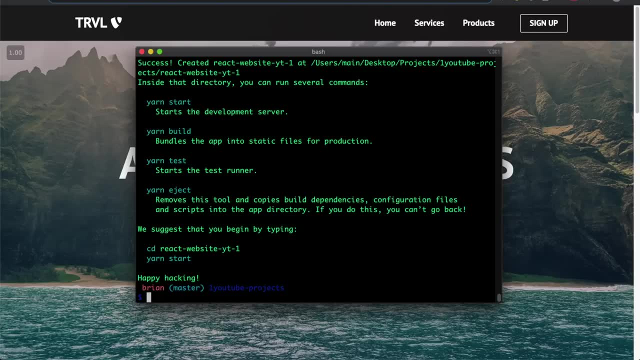 might be super quick or it might be super slow, so just pause the video and then, once it is completed, i'll see you on the other side. all right, so now i have it all downloaded. so now i'm just going to go and cd into the file we just created. so, whatever you named it, type in cd and then the file name. 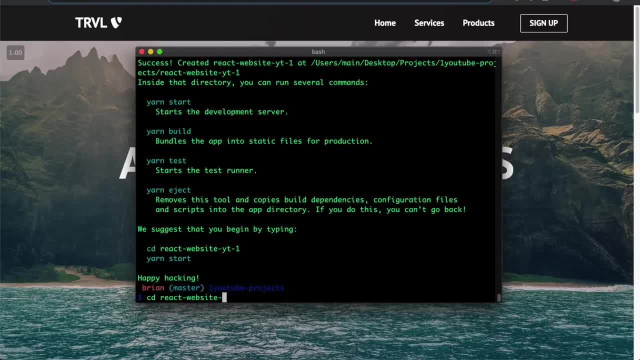 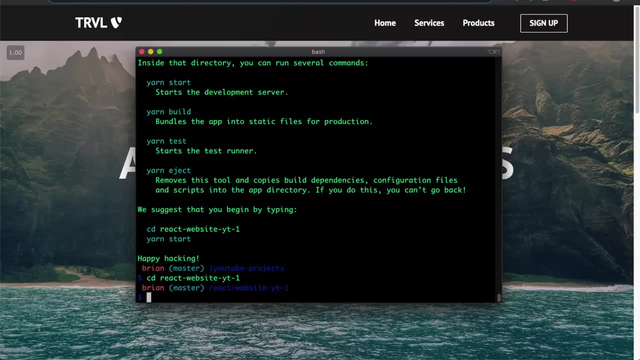 so mine is react: dash website, dash yt, dash one, and if you don't have yarn then you're going to type in npm start. so you do like this, which most people starting off would use, but if you have yarn, obviously you would do it. so whatever yours says on the second line, that's what. 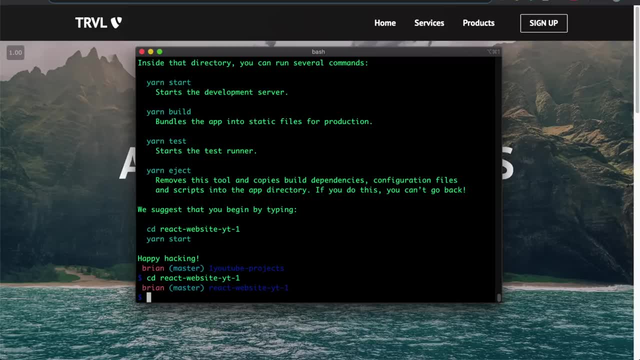 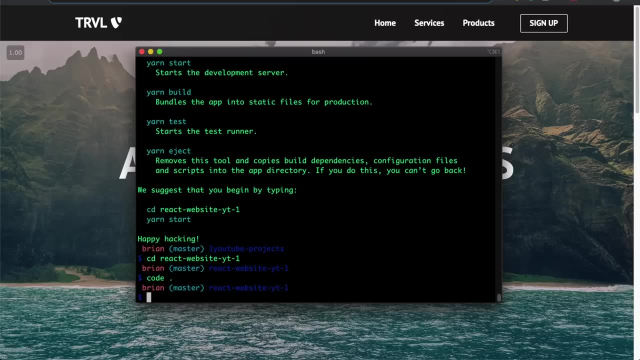 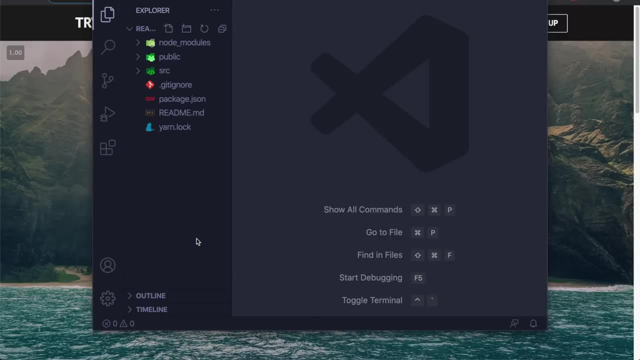 you type in. but before, uh, i do that, i want to actually go into my code editor. so i'm just gonna go ahead and type in code dot and then press enter and they'll automatically open up vs code. if you have that set up, then you should have the same thing here. but if not, simply just google how to, 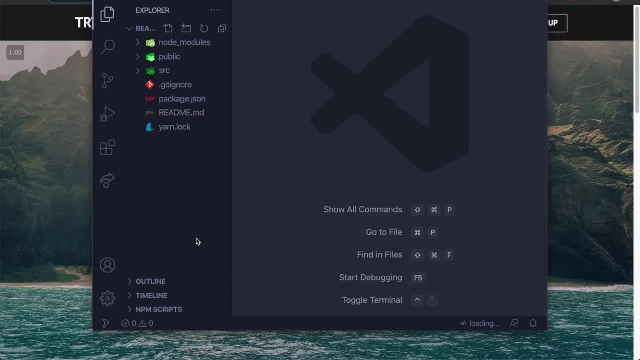 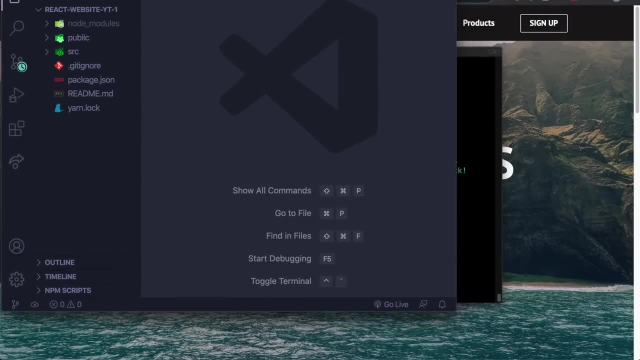 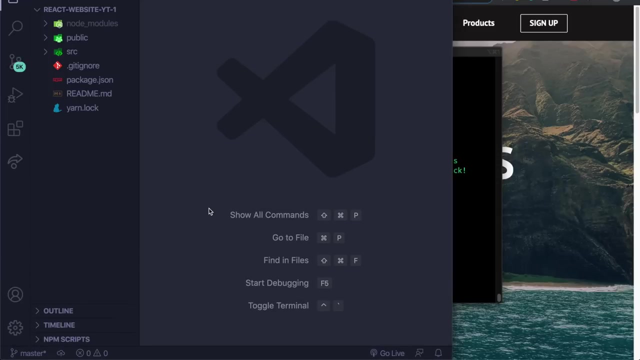 set up code dot to open up your code editor, and there'll be a bunch of uh websites or uh people, i think, on stack overflow you can find and basically tell you exactly how to do it. and now we're here on the actual vs code. so right now i'm going to go ahead and command j or just open up your terminal. 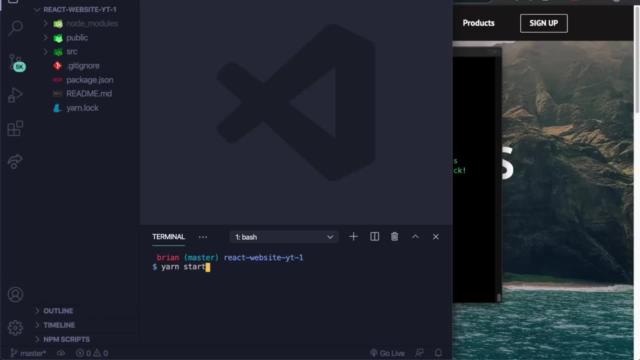 and then here i'm actually going to type in yarn start. so if you have npm, then type in just npm start and then press enter and then what's going to happen? this keeps happening for me. so what i need to do- if you do have this error, just go over to this left side and let's create. 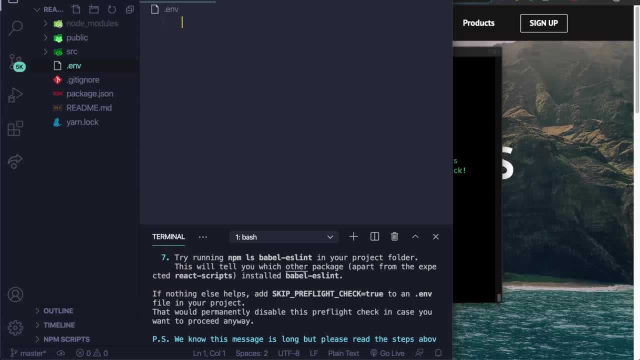 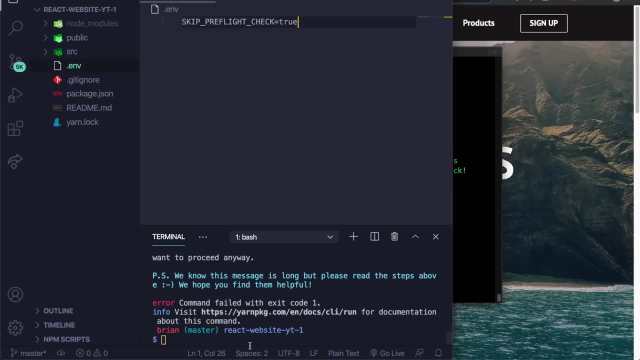 a new file. let's call this en so dot, env. and then let me just copy this code right here and then save. and then let's go back to terminal and just do yarn start again, or npm start, depending on which one you have, and i already have the website loaded in the background. 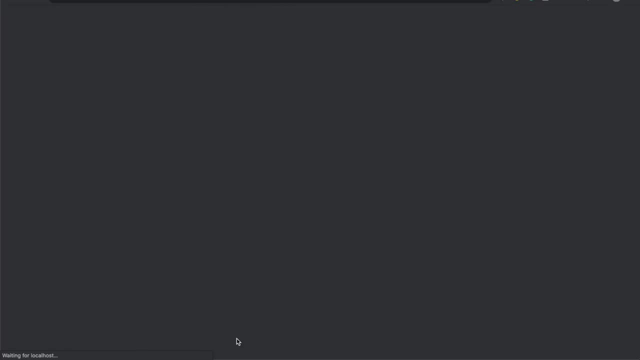 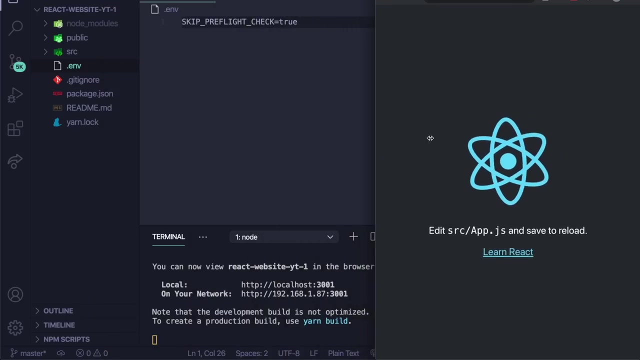 so i'm just going to type: yes, yours would automatically load as long as you don't have another react app open. so boom, now we are here, which if you've already made react apps, then you definitely know this, so it's not too crazy. and now let's go ahead and start deleting some stuff. so let's get rid of. 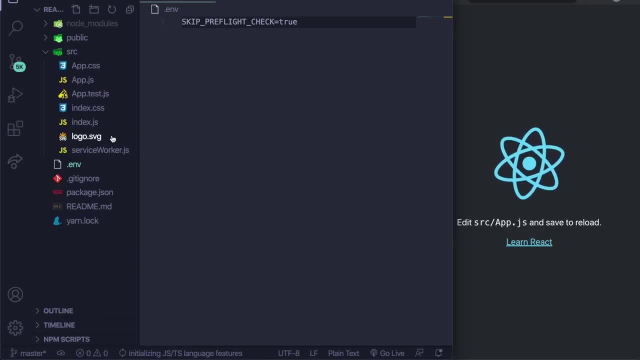 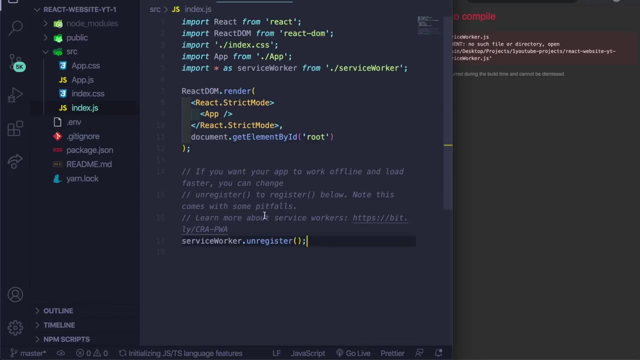 let's get rid of this setup test. don't need this. i don't need the logo or the service worker, so i'm gonna get rid of these. so i just hold shift and click on both of them. apptest dot js. i do not need and let's go to index. let's get rid of these comments. 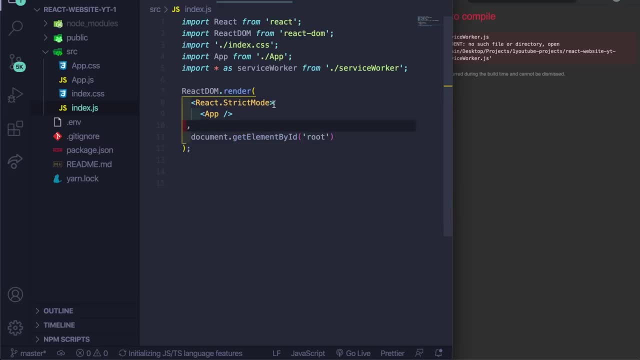 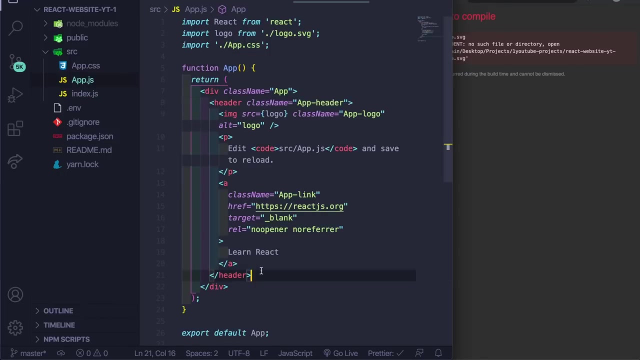 i'm gonna get rid of strict mode for this and i'm gonna save mine here, and then i'm gonna get rid of service worker. let's see, let's get rid of indexcss2. so let's delete this and just leave these three files and go to appjs. go to here, get rid of everything in here and then be like: 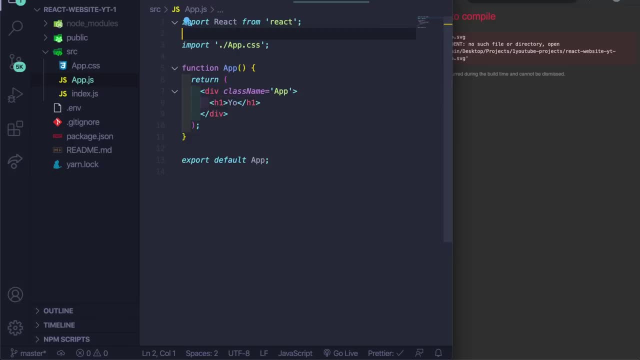 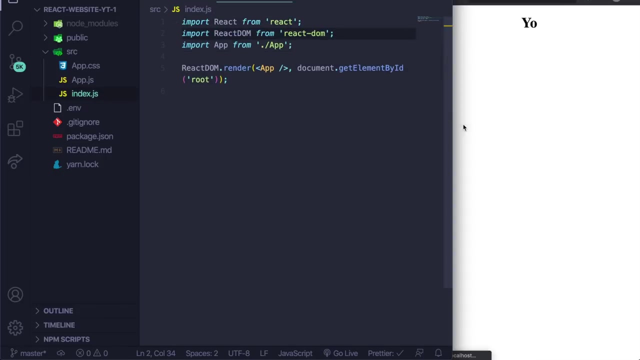 yo save, and then we gotta get rid of this logo. imports. and then let's see: um, what's, what is it saying? right now am i missing? import reacts. let's see indexcss. this one needs to go on the index. and there we go, all right, perfect. and then after css: 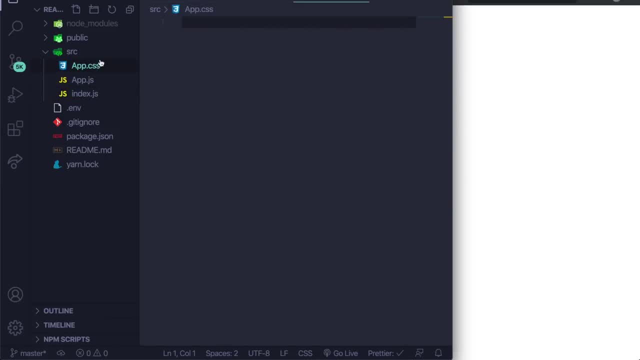 i'm going to command a get rid of everything and save it here and now. we can go ahead and get started. all right, so the first thing we're going to do is create a components folder. so let's go ahead and click on the src- right click- go. 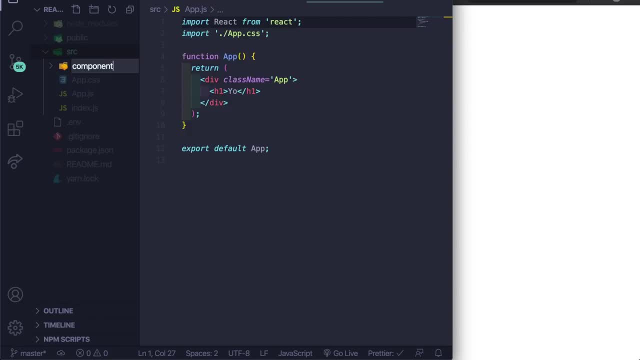 to new folder and let's just say, come components, and then inside of the components, let's start creating the navbar first. so right click components, new file. let's do navbarjs, and then i'm going to create a css file for this too. so right click in the end, new file, and then navbar, dot css. 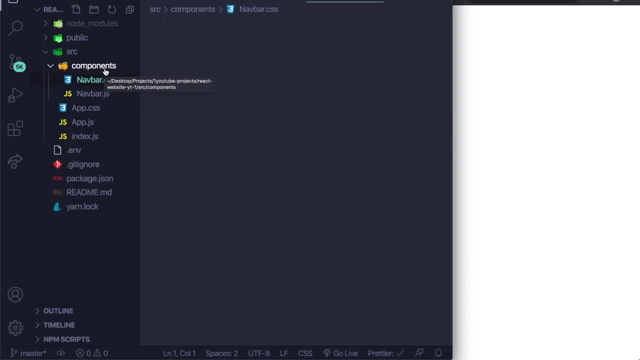 and then let's go ahead and let's just get started with that. first, I have a completely separate tutorial for a custom now, but this one's very almost identical is just there's less stuff to it, and then also in terms of the starter files, so I have images and videos that I 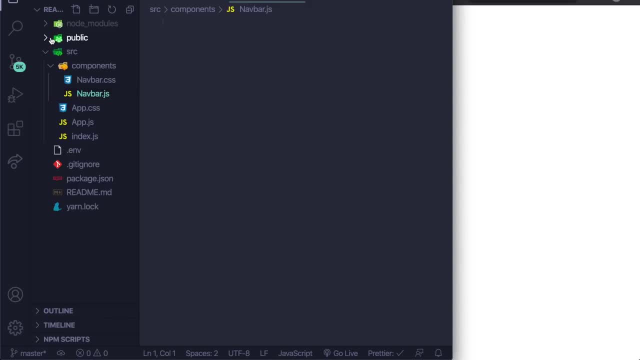 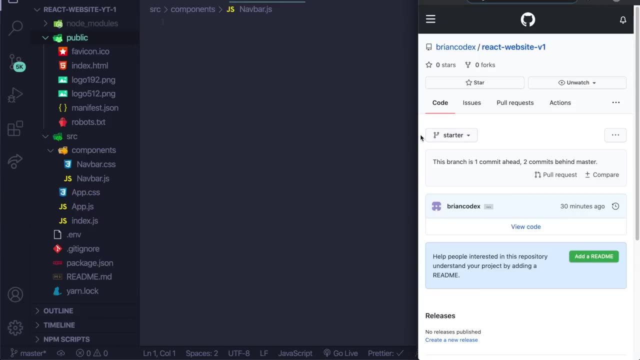 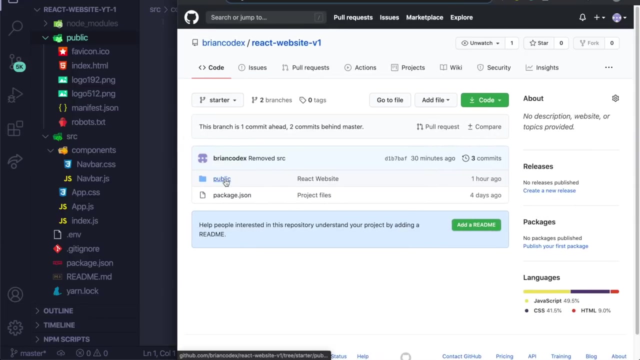 had for this actual site that you saw beginning. so if you want to get those, basically I have the github link, I'll put it in the other github link, I'll put it in the description you should be able to find and basically you'll go here on starter branch and then just click on the public file and then we 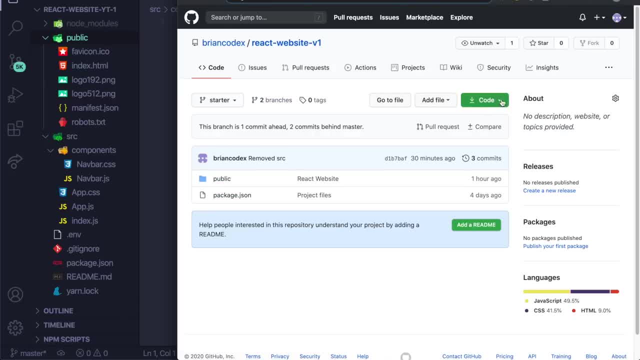 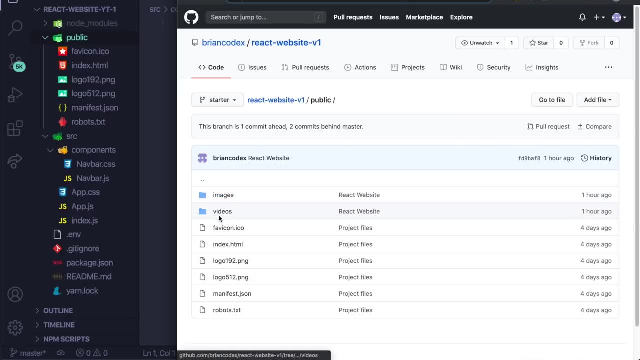 have images and videos. so in case you could just pretty much go here to code and just download the zip, or you could clone it, but basically just go public and then get the images and videos. I have a bunch of images that you can choose from, because I was using it for another thing, but I don't think we use. 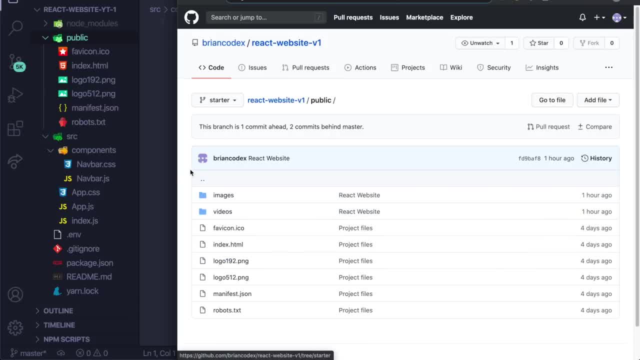 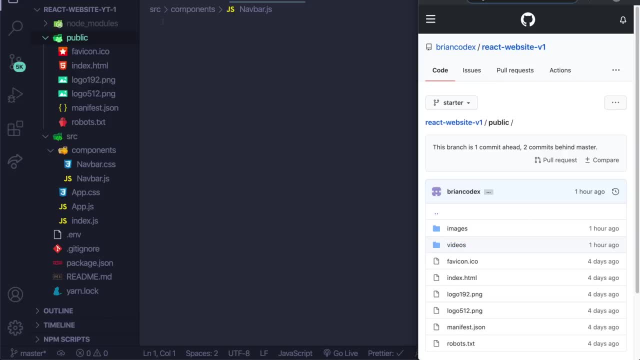 that many in this tutorial. but once you get the images and videos, download it, then drag those into your public folder. so or just download or just replace, I guess, the public folder, since you're copying it. so I have mine set here, so I'm just gonna drag these over and I don't know why it's not showing up. oh, there it is, wait. 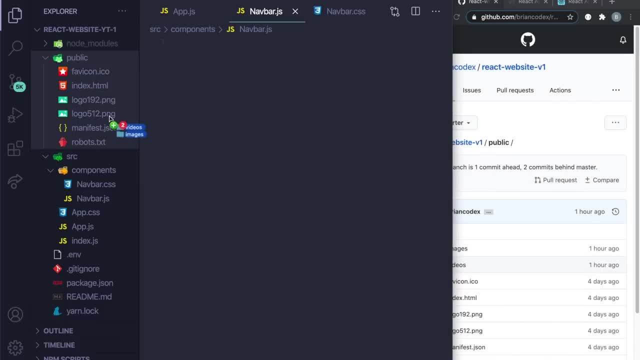 is that it? no, that's not it. hold on, this should work this time. are you doing copies folders? yeah, so let's do just copy the folders. boom, and I, if yours didn't drag properly, I dragged them from my finder on back because I was trying to drive from VS code, but it wasn't working. but 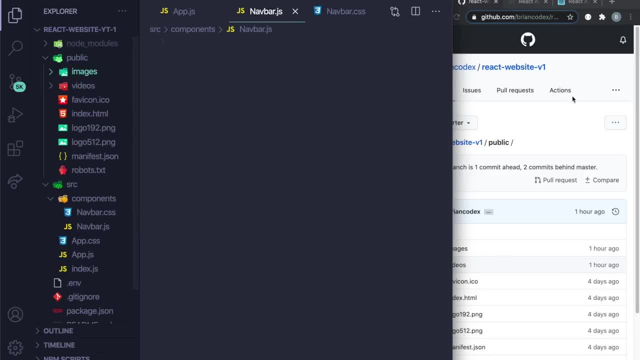 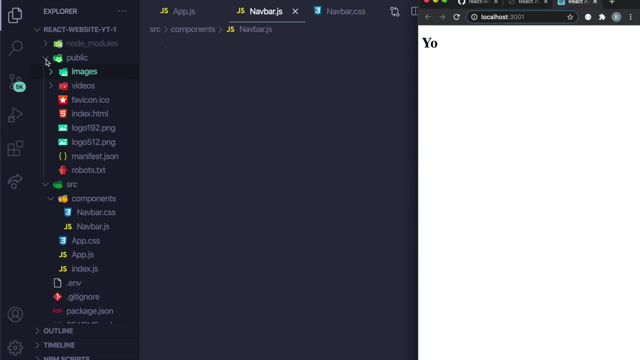 basically, I have these videos here now. you don't have to do this right now, but I mean, since I already showed you might as well, and now we have to go back in the next, like you know, hour, so trying to find these. but basically those are all. 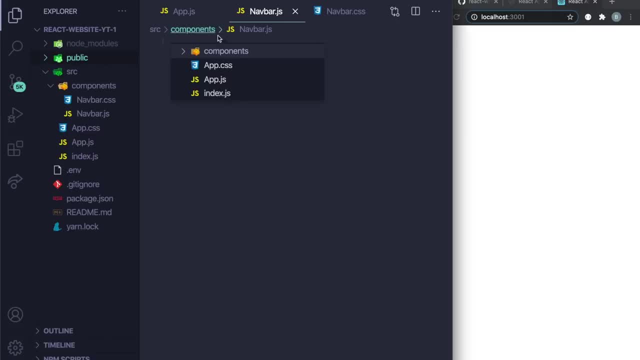 the images. so now let's go ahead and start editing, or nav bar, alright. so what happened? what I just click on? let me get rid of this and let's get rid of this, alright. so first thing again. also, if you don't have this extension, you can go here and type in a. 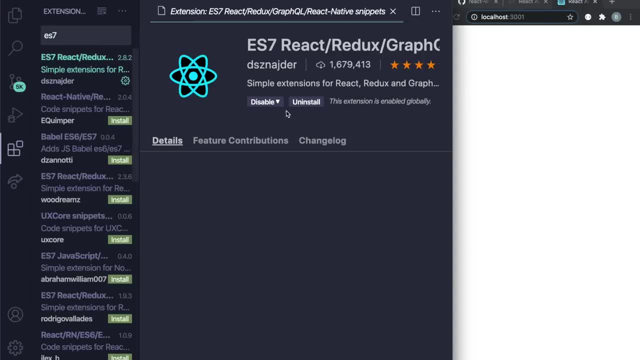 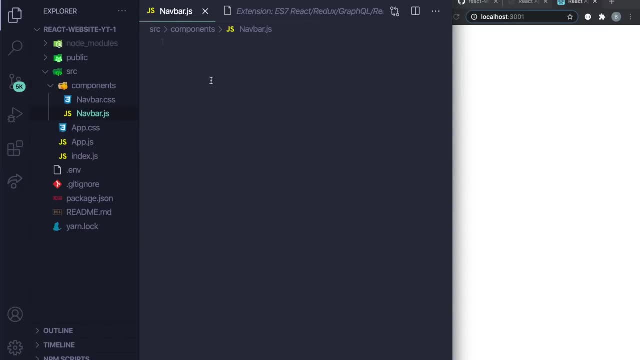 yes, seven or react snippets and then click here and you can install this one and depending- sometimes it doesn't work for me, but some usually. it will see if it does this time. but basically we can go here and just type in our FCE and I can press ENTER and then automatically import react. from react we got a. 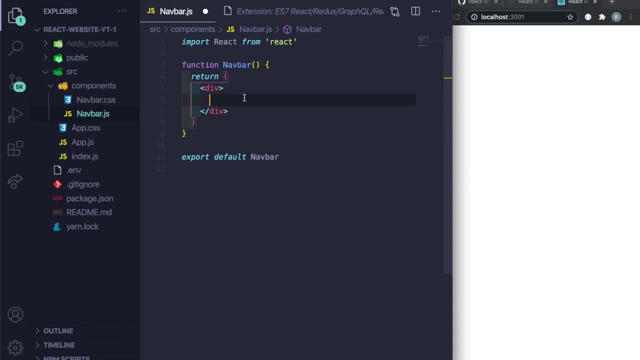 function with the name of the page and we got X export it. so it's pretty clean and essentially what I want to do here is: let's go to the top and I'm gonna be utilizing use state for right now, so let's do use state and then also I'm going to be 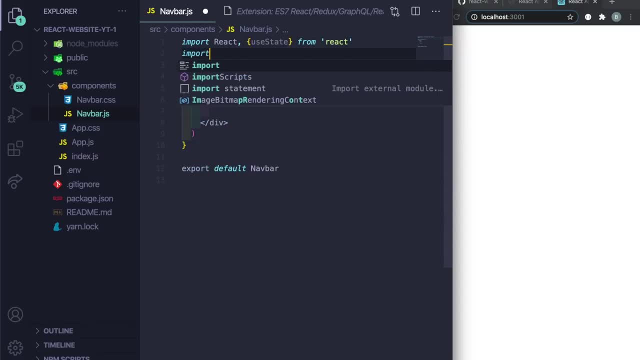 creating a button component eventually so we can do that. imports, you can do a seat. let's wait on that because I want to start the actual JSX first. so let's go here and, pretty much, let's start writing this out. so let's create: get rid of the dizz, let's just make them fragments. I'll just create a nav, so I'm. 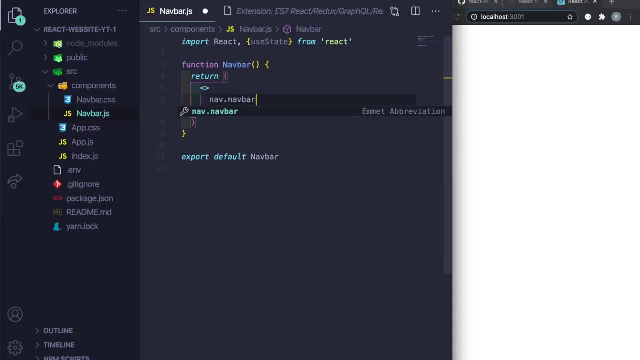 gonna go ahead and say nav, dots, nav bar, and that creates the class name with nav bar enter in here, and I want to create a div and call this nav bar container. let's just go ahead and say dot, nav bar, dash container, now in here. so we're gonna be utilizing react router actually. so since 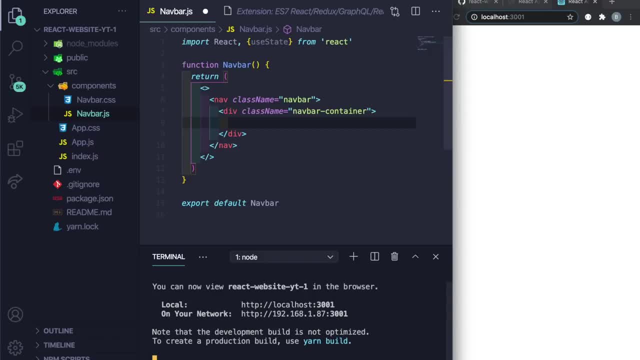 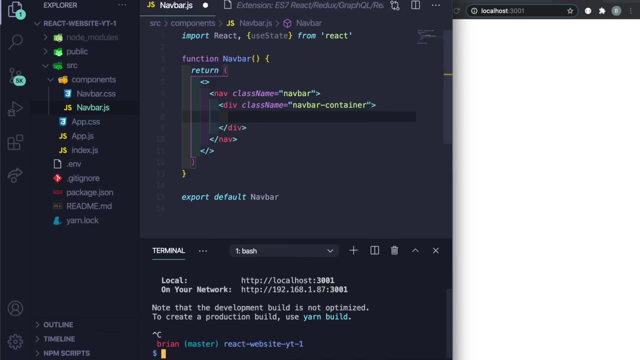 we're here, this might as well command J in the terminal and then do ctrl C so it stops the app, and then pretty much what we're gonna do here is going to do a npm. or for you let's do npm: install react router dom, and then let's just press enter. 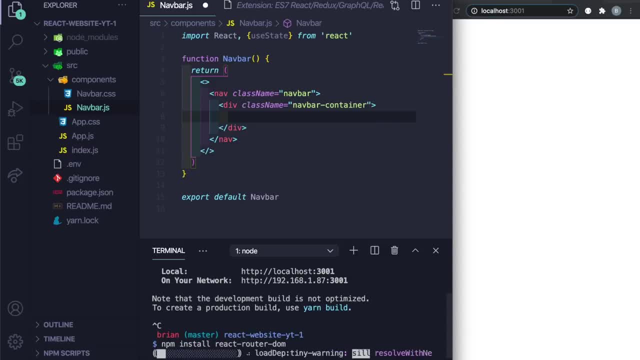 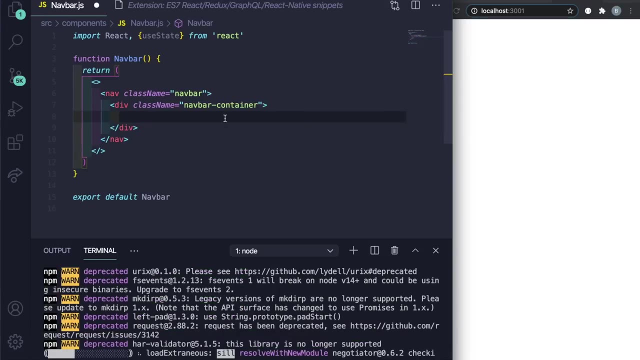 now. this can take quite a while, depending on your computer. so while we're actually waiting for this, let's start adding some more of the jsx. so within here, let me do command b so you guys see what's going on basically. once that is done, we're going to import the link, so let's just go. 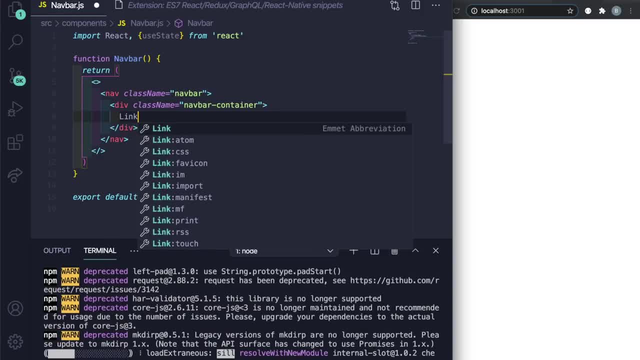 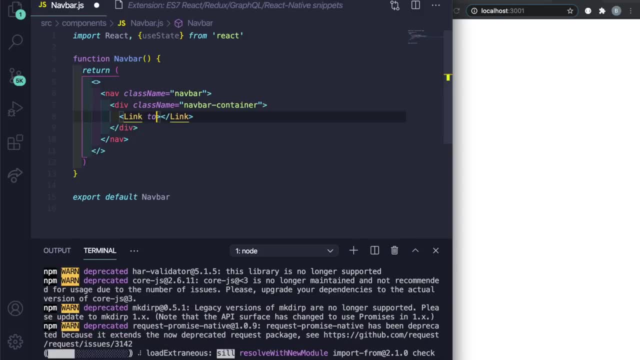 ahead and type it out, since we're loading. so let's just type in l-i-n-k and then press tab and then inside of the link i want to say the path equal to just slash, and then let's do class, name and link. essentially it replaces the a tag. so if you never use react router, then that's. 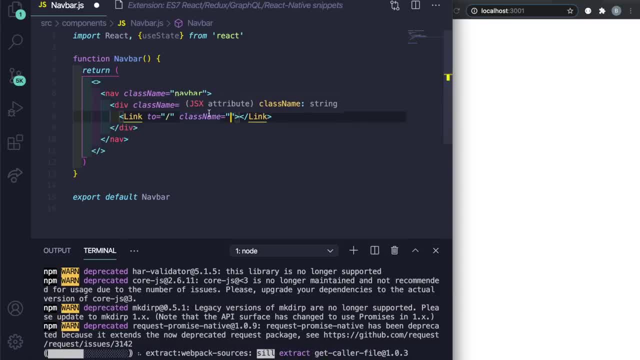 essentially would be an. this would be an, a tag instead of link, normally, and then let's do nav bar dash logo for this. and then i want to create a function, but we'll do that later, once we have everything done. but this is essentially the logo. obviously, you use an image instead of a link normally, but i 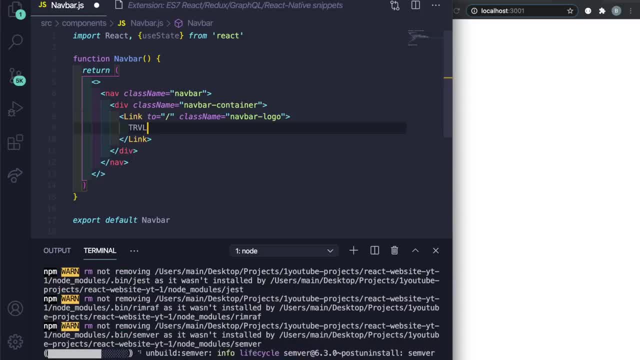 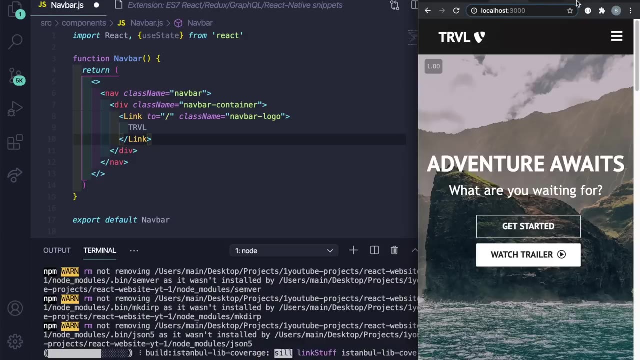 don't have an image, so i'm just typing it out. and also, if you did actually um, let's see one more thing too. let me show you really quick. so here i am, on font awesome. so that's the way i utilize this little icon right here. it's not necessary, but if you want to copy, 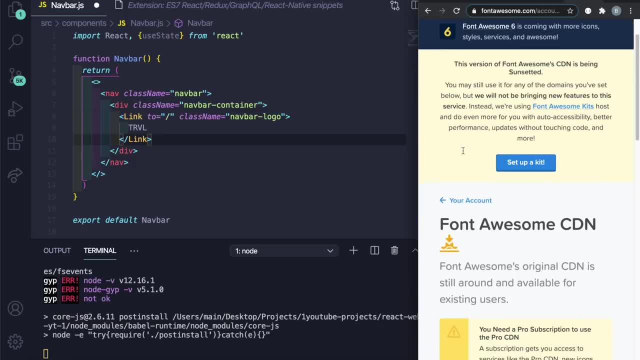 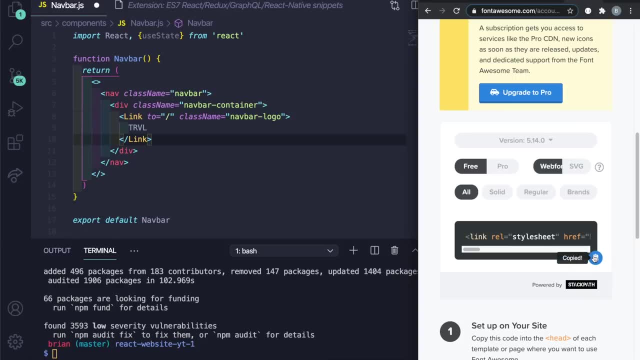 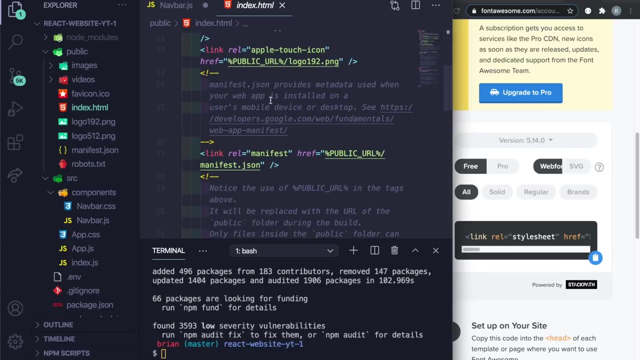 it. i have just make an account at fontawesomecom, sign up, and then go to your profile, click on font awesome cdn and then scroll down here and then basically copy this link and then you would just go to the public folder in indexhtml, scroll under just right here within the head tag anywhere. 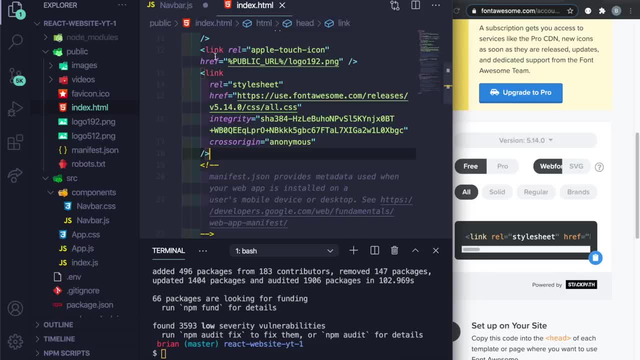 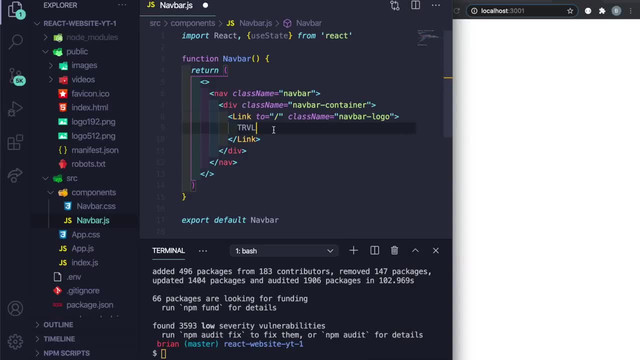 copy it and then save it. so now we have that font awesome cdn here. and then, if i were to- actually let's go back to the app next to the travel- i just did ifabfa-typo, so typo three and then press tab. this creates the. 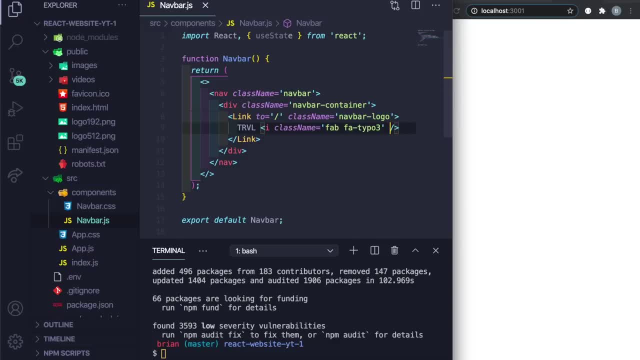 icon right here for us, and when i save this right now, we're going to get an error. actually we're not, because we, we paused the app, so let's go back and do. um, let me just do yarn start or npm start for you, and then, once this loads up, 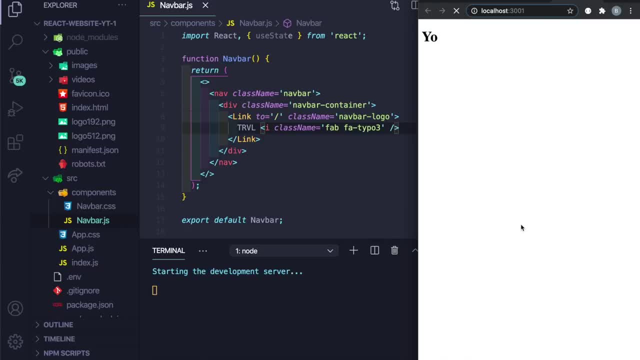 so i have two apps right now. so it's going to say yes, but um, basically it's going to reload and then you're going to see nothing because the link has not been imported. so it's most likely going to show: let's see, yeah, nothing's happening right now. so let's actually go up here to the top. 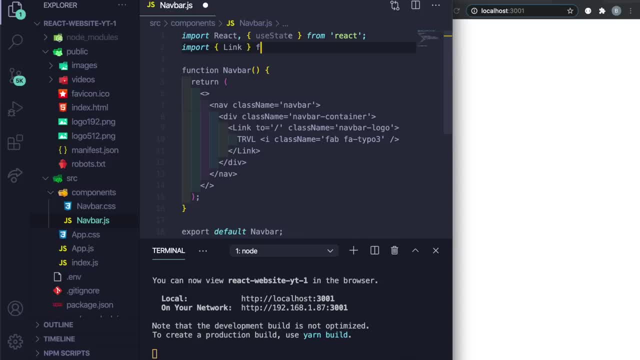 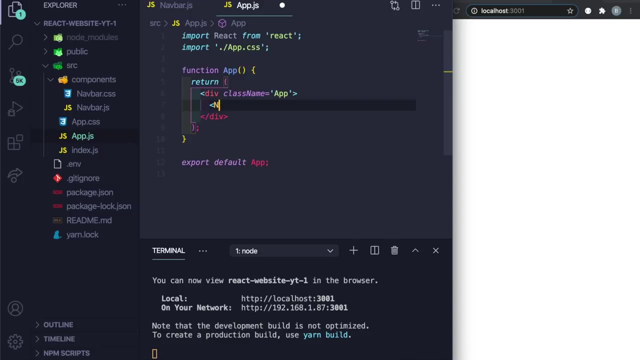 and imports, link from, and then quotes say: react dash router, dash dom. let's save this. and right now you can't see anything because we have not actually added this to our app. so let's go to appjs and then over here within the h1, let's just do, let's add the navbar components and what i like to do is, at the end of it, i like: 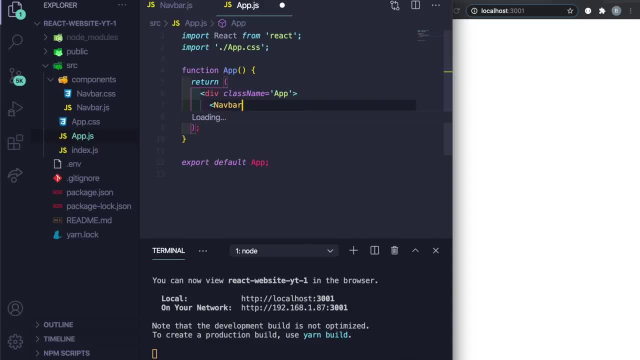 to press enter and sometimes it works. so let me see. yeah, right now my vs code is going super slow for some reason. maybe it's because i'm recording. but let me just add the component there and then just import it manually for now. so imports navbar from dot slash. it looks like we added two. let me do dot, dot slash. yeah, navbar, save this. 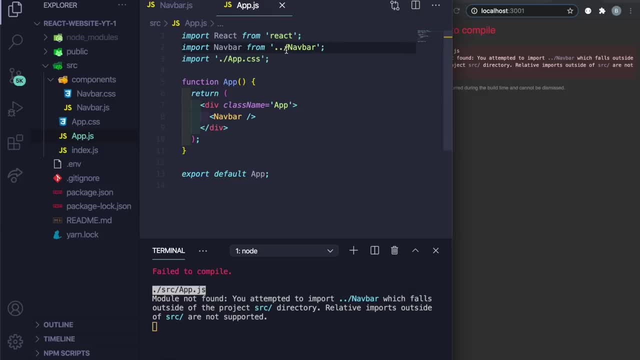 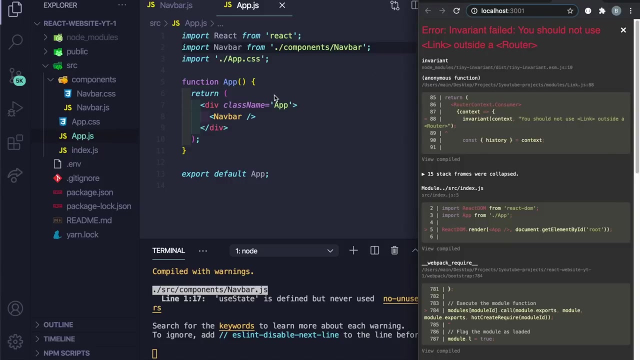 and what happened. oh yeah, i forgot. forgot to add the components folder completely. looked over that. so components, slash navbar and this one should be- yeah, it should be like that. save this. and now it's saying you should not use link outside of a router. so right now, since we do have react router, we're gonna have to. 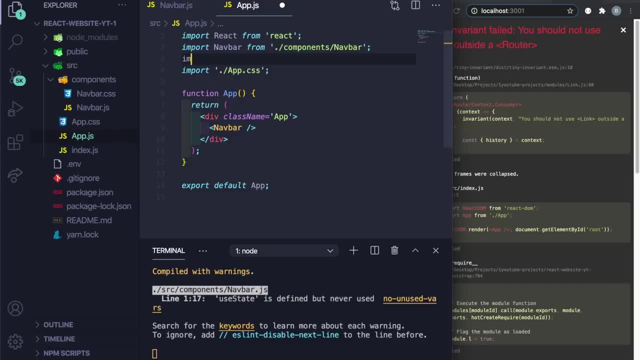 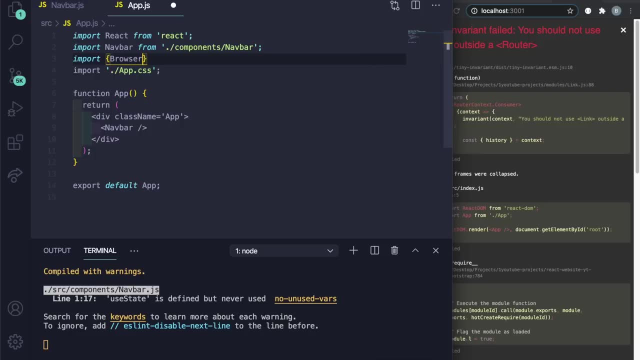 import a bunch of stuff to get this working. and then once we have all this import, it's gonna be easy sailing. so let's import here. i'm gonna go ahead and say browser router as router, and then i'm gonna have switch, and then i'm gonna have routes i'm gonna say from: 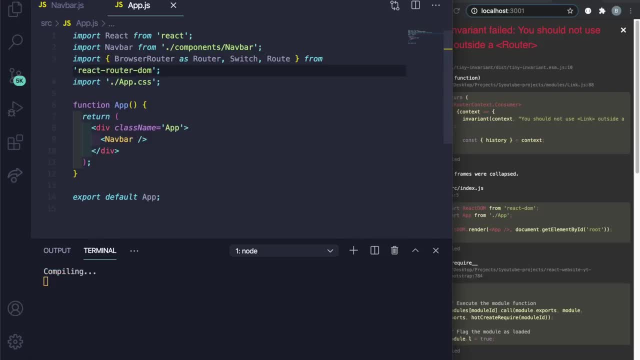 react: router, dom. so let's save that and then around the actual uh, let's see, let's get rid of these divs first, and then let's put a fragment here and then also below this, and then i'm gonna say: save that right now and then under that i need to put router. so this, essentially, is going. 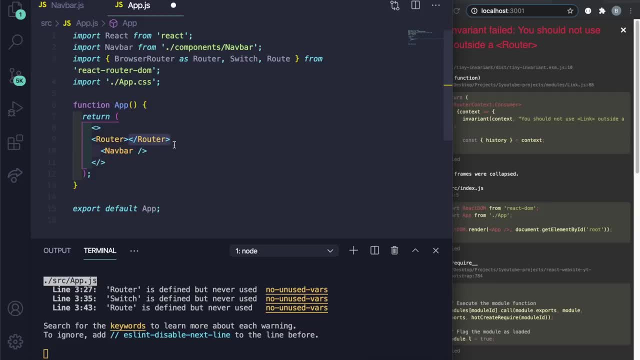 to contain all of our routes or our pages or paths, basically, and then within that, under the navbar, i'm gonna have the switch statements here and then within the switch is where we have actual routes. so i'm gonna say routes and then let's do path equals slash and then say exact, because i want. 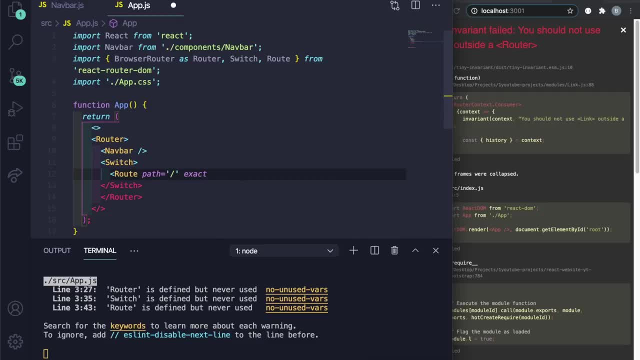 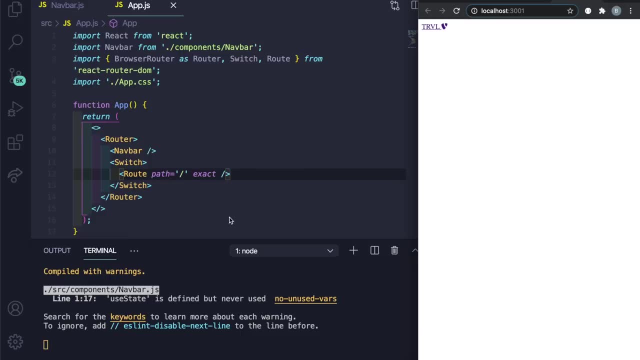 this. this is going to be essentially the home, and then we're going to pretty much, let's just put: um, let's see if it should show the error. yet, all right, now it's not showing the area. now this would be the home component, but we don't have that created yet. but pretty much now you can see everything works and we click on this. 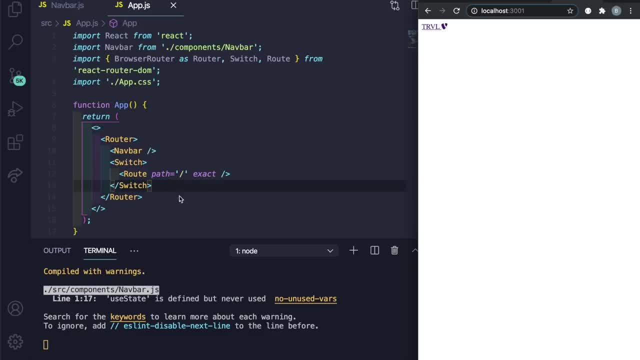 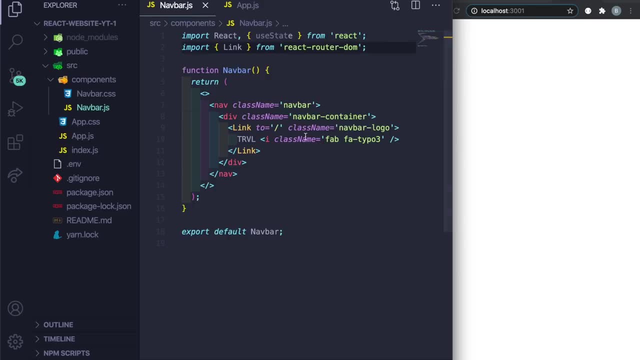 nothing happens because we are going to slash. so that's basically everything set up and also you can see the icons there. so let's go back and let's go back to the navbarjs and let's continue with this navbar creation. so now underneath this link tag, so the icon. 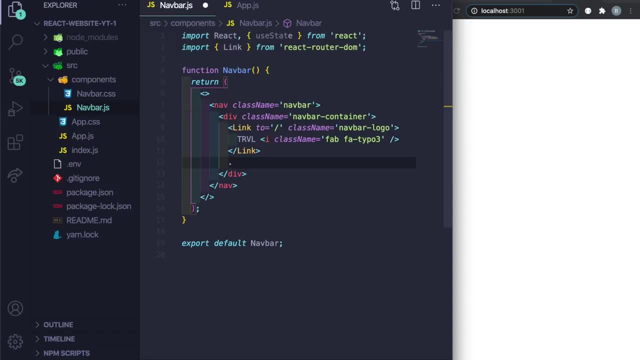 or the logo, i guess you can call it. i'm gonna say dot, menu dash icon, and i don't know why. sometimes it works, sometimes it doesn't, and let's do, let's just create the div, since my uh vs code does not want to auto click this for me. so let's do dot, so class names equal to menu dash icon. 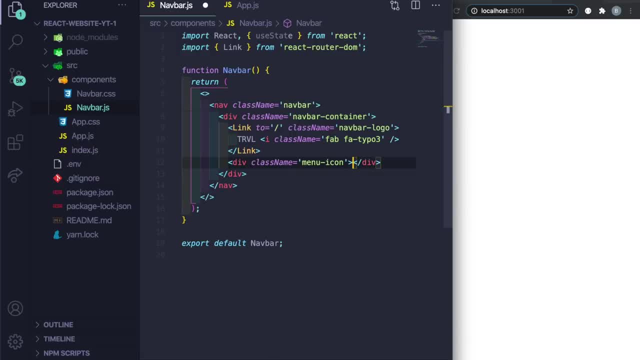 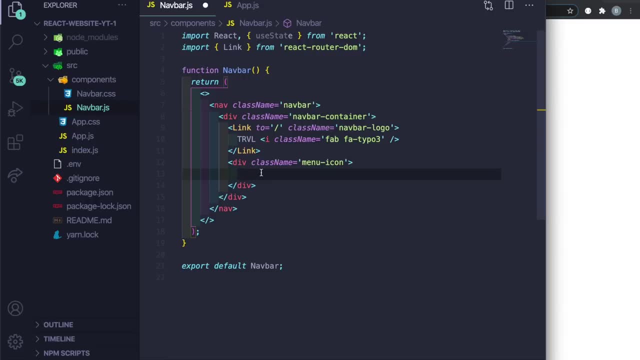 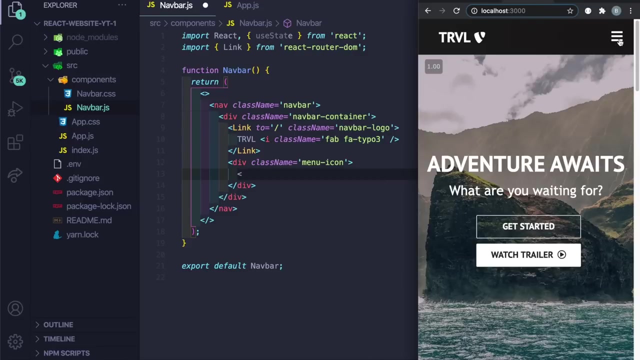 and then here let's close this out, and then let me make this a little bigger so it's just easier to see, and then within the menu, that icon, this, we're going to set the hamburger menu, so essentially, where you saw this, uh, this thing right here, and we're basically going to create a 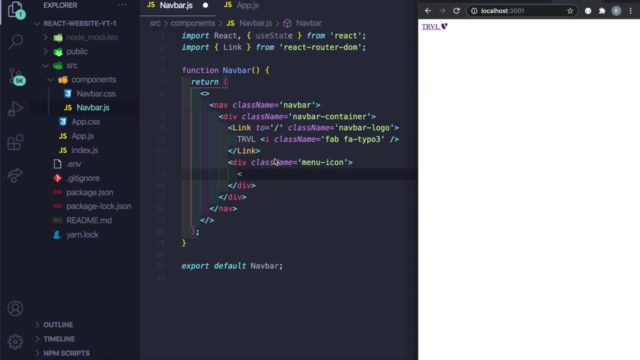 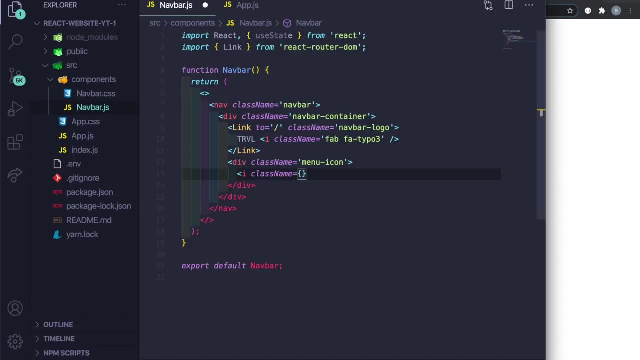 we'll set where you state basically to change it from my x to a hamburger menu. so in here, if you have font awesome imported, i'm going to say i class names equal to curly braces and we're going to create state with click. we're going to call it click and essentially, if click, 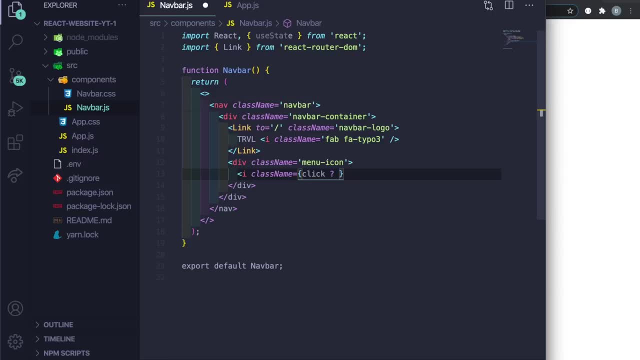 the value. basically, if you click on the icon, then i want to change the class to fas, space, fa, dash times, and if you click again on it i want it to be changed back to essentially the bars and then it'll be a pretty much toggle. so it's going to go from right now if it's not clicked. 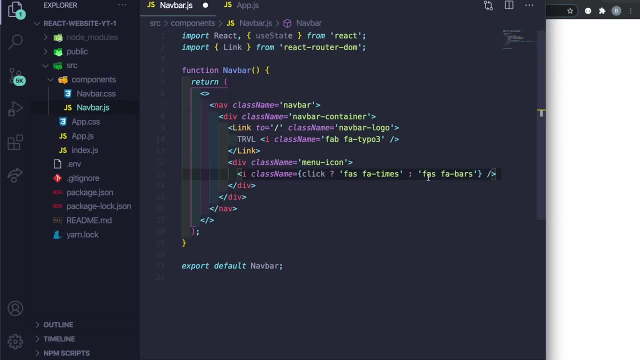 it's going to be the hamburger menu and then i'm going to go from right now, if it's not clicked, it's going to be the hamburger menu and then, once you click it, it's going to be the bar. so right now, if you see it's going to say click is not defined, so we're gonna have to go here to the bottom, right here. 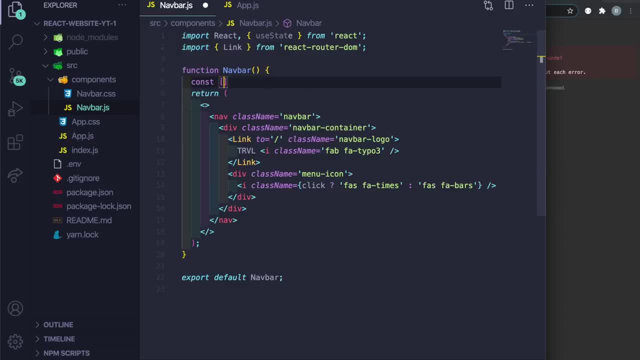 under function and we have to say cons. i'm going to set state now, so this has the use state that we imported up here. i'm going to say click and then essentially we say set, whatever you named it. so set, click, and this is basically what's going to update the state and essentially change it from. 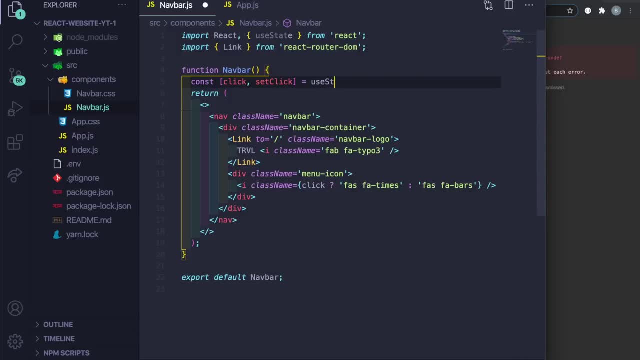 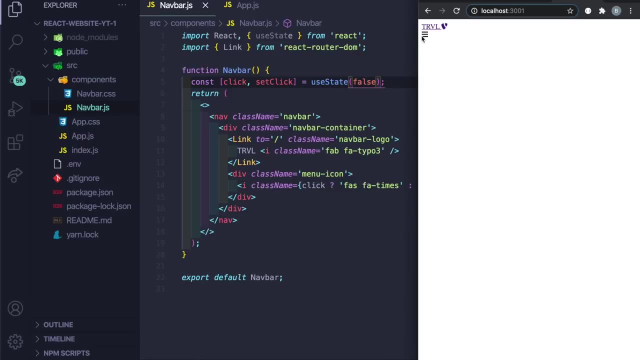 whatever it was to, whatever you want to change it to. so i'm going to say use state and then i want the initial value to be false. so if i save this right now, nothing happens because we don't have a function that actually updates this. so right. 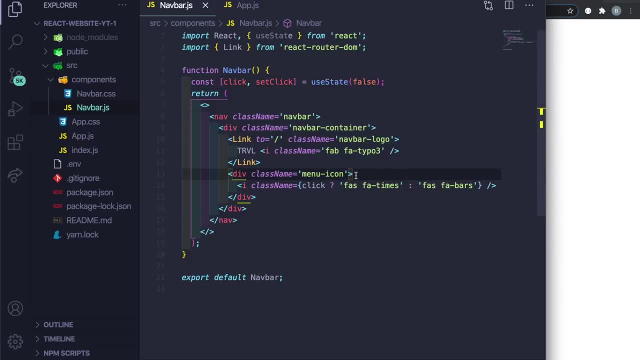 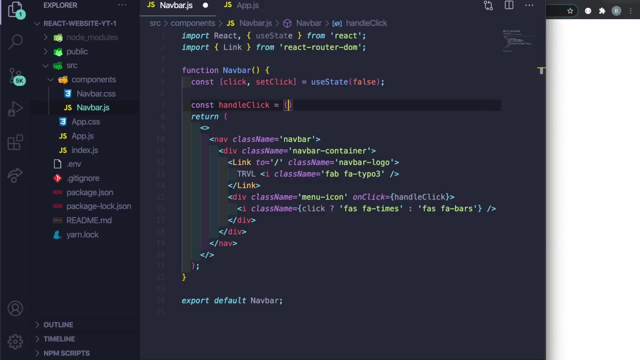 now i want to go here to menu icon and i'm going to add this on click and set that equal to curly braces, to a function that we're going to create right after this, called handle click. so now under here i'm going to say const handle click and then i'm going to set that equal to an arrow function. 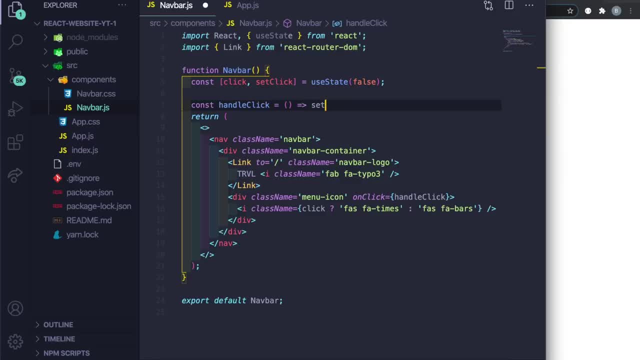 and then essentially what i'm going to do is say set click. so all all this function does is it sets the click and the value. i want it to be the opposite. i want it to set whatever click is here false. i want to just reverse it. so essentially it's false, true, false, true. so if i save this, 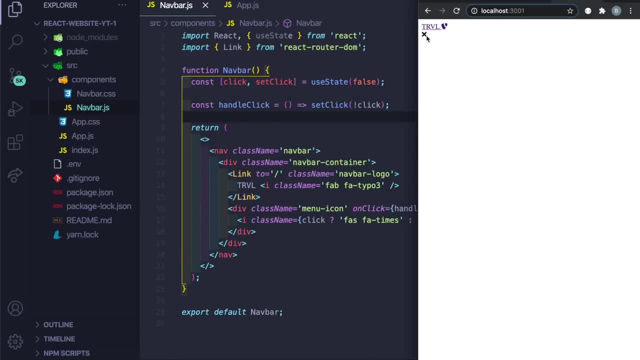 you can see here now, when i click it it switches, because now it went from. i didn't click it, so now it's hamburger. now, boom, that's not the bars. and then elle, Now it's hamburger. Now I've messed up some of the bars and those 2 and 2- zeigt in the 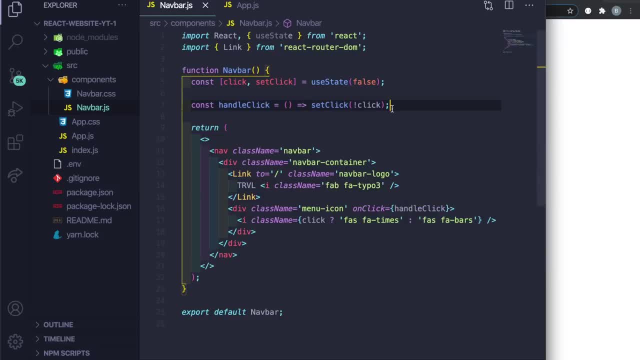 so basically reversing the state here. so pretty simple, nothing crazy here. and then let's go and continue creating this and this is again wrapped around: this handle, click div. and now let's go ahead and go underneath this and let's do ul and let's press tab. and i don't know why i did this. check cert mencion, nomin warção. 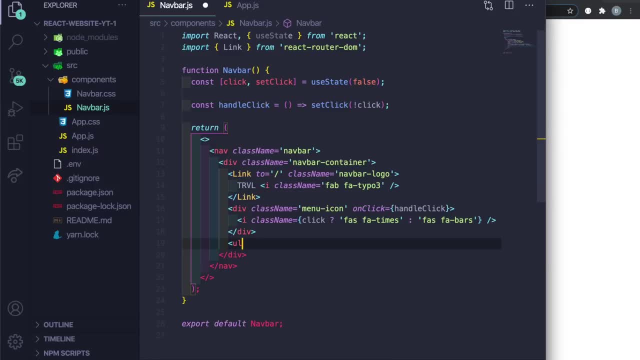 tab and i don't know why my thing is not working right now. i'm about to refresh my uh vs code but since i'm recording, might as well keep it here. but within the ul let's go inside of and say class name equal to curly braces, and then i'm going to say again: it's saying the click value, so you clicked. 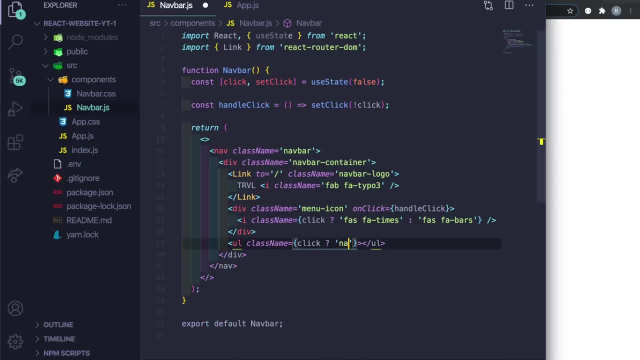 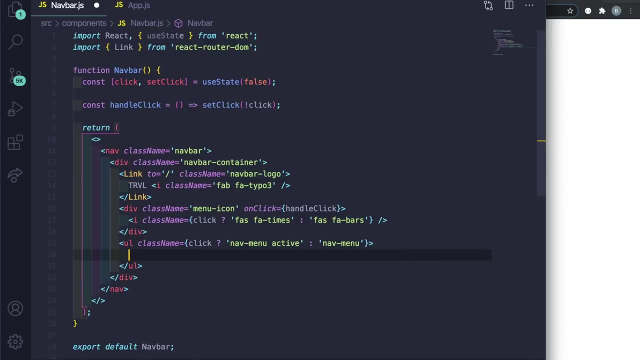 it, or, if it's true, i want it just to be nav dash menu, space active and then else nav dash menu. so let me close this out here so you can see this. what i have here and then essentially you'll see this is when, when we're on the mobile right like this, whenever you. 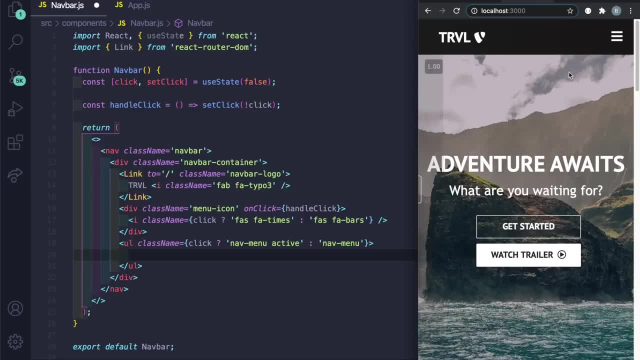 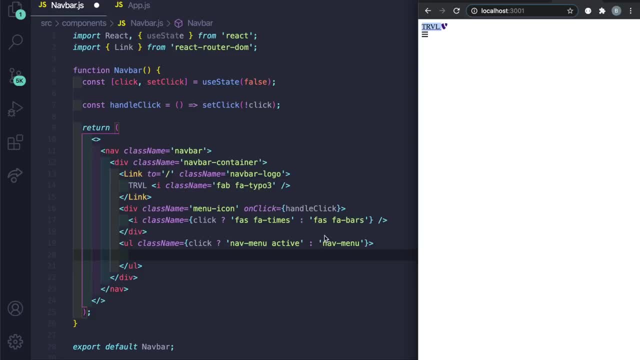 click it, i want the nav menu basically to disappear, which that's what that line is supposedly doing right now. so i'm going to go ahead and do that and i'm going to go ahead and right now, but that's basically the same thing right there. so that's what that line right here. 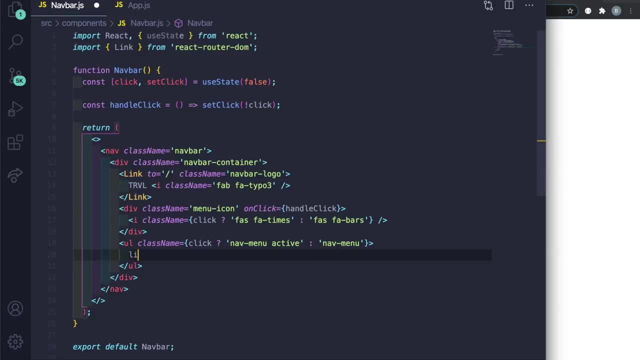 is supposed to do. and then let's go and create our li- and i don't know why my l, my tabs aren't working right now, but let's do li, class name equal to nav dash item. and then in here we're basically just going to create another link tag. so let's just say: link two equals slash. 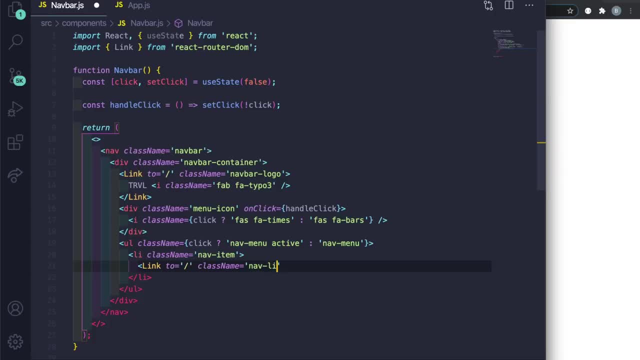 class name equals to nav dash links and then on click, i'm going to create this and it's essentially called uh, close the mobile menu. so i'm going to say curly braces, close mobile menu. and then close it out with the tag right there and then inside this you can just say home. so if i save this right, 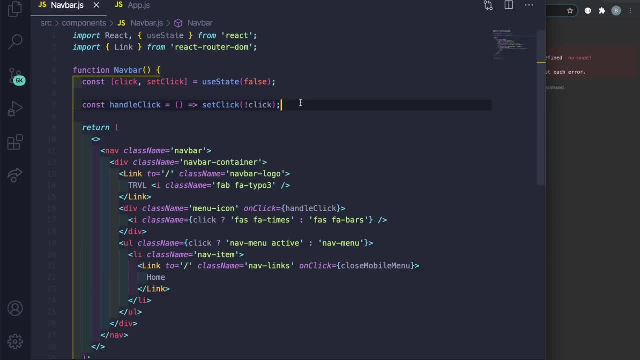 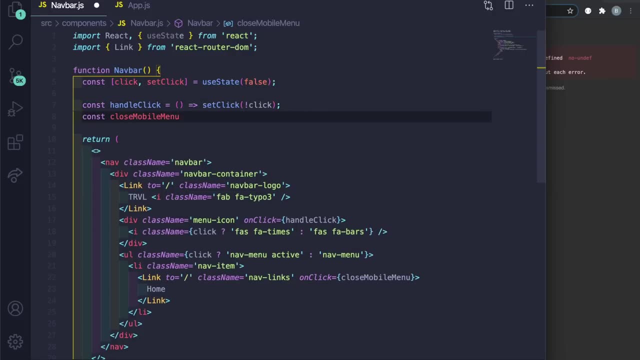 now we're probably gonna get an error because close mobile menu not defined. so now we have to go up here and create this function. so basically it's gonna just say cons- close mobile menu and i said that you go to the arrow function and basically we're gonna say set click equal to false and then 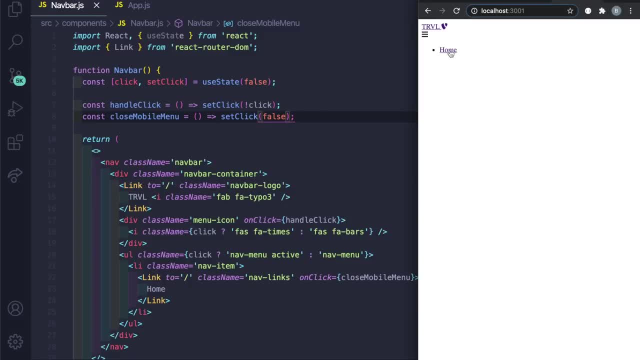 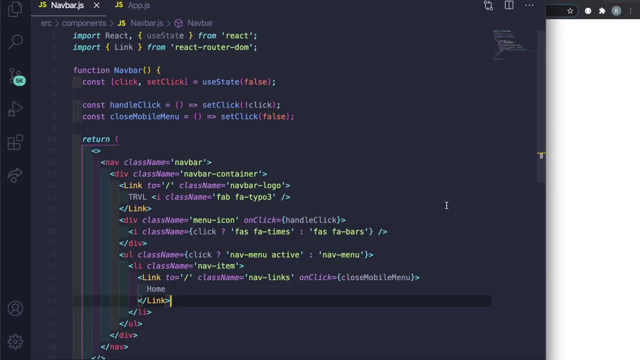 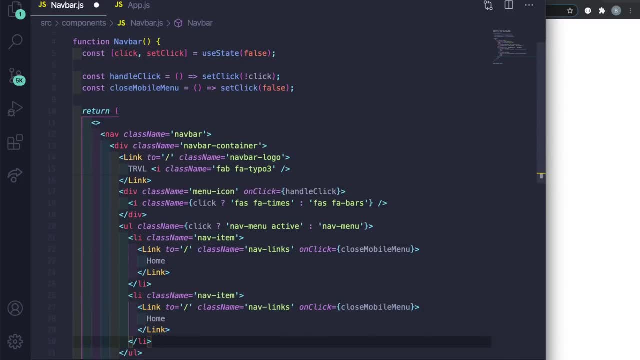 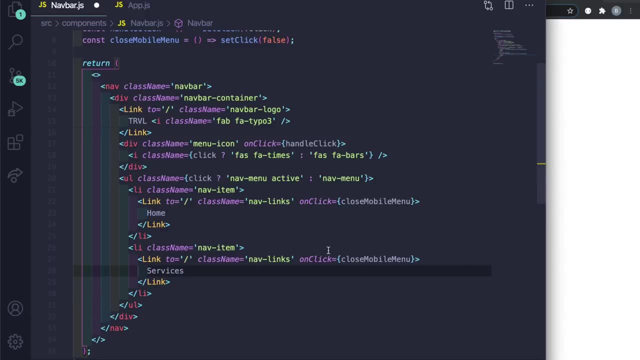 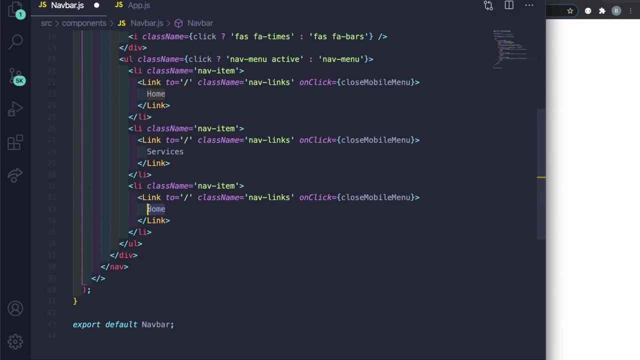 copy this, the li with the link, paste this and then we can just change the middle to services or whatever you want, and we'll keep everything here. so i'll save it here. check is there, and then go under command, paste it again and then let's just do, uh. 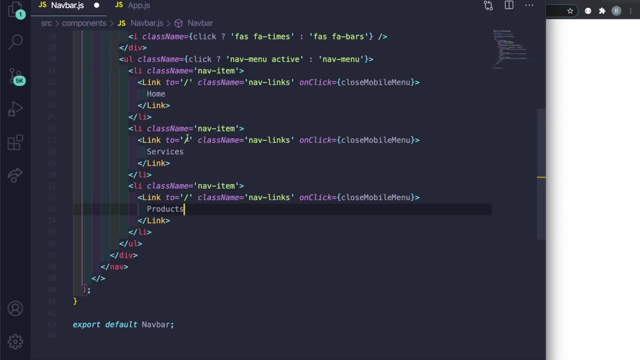 products. also the links. let's change the links to whatever you named your thing. so services here and then products there, and then, underneath that link, we're going to do another one. so this is going to be the sign up button and this one's going to have a different class name because- at least the way i did it- this disappears. 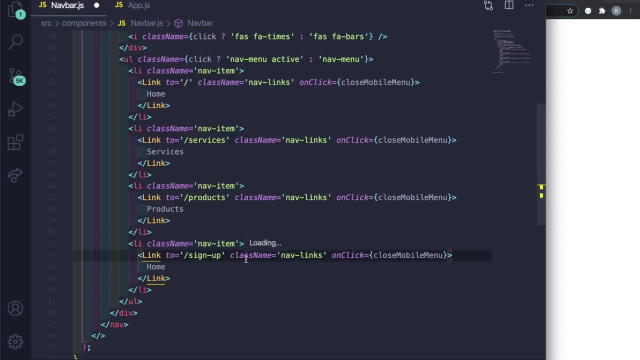 it only shows up on the mobile menu and it was just much easier for me to style in terms of the component versus having it like hard-coded, which you'll see in a second. but basically the class name is going to be dash nav links, mobile and this is the sign up right here. so 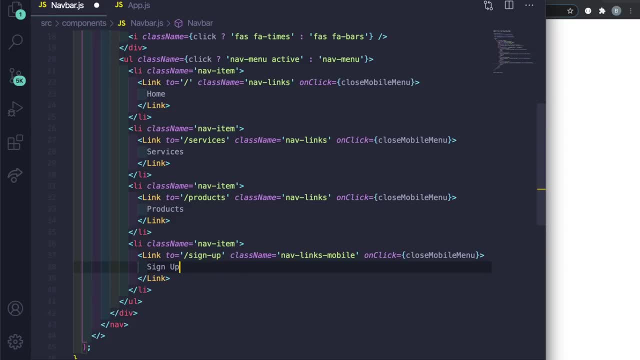 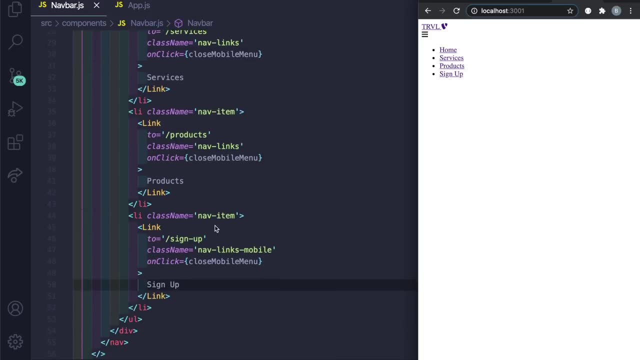 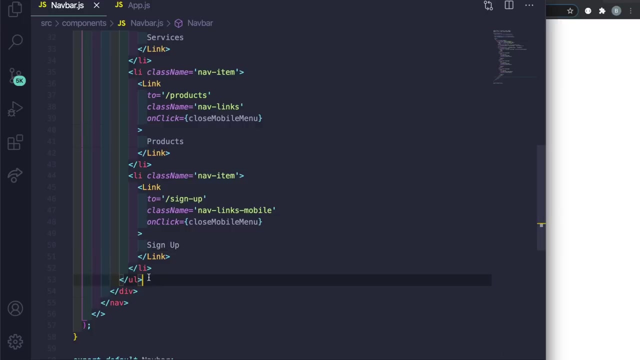 sign up and then let's go ahead and change. yeah, it looks like it's. let's save this and i pretty installed, so that's why auto saves like this. so now we got the four menus over here and then the ul outside the closing ul tag is where the budding component would go. so since we're here, 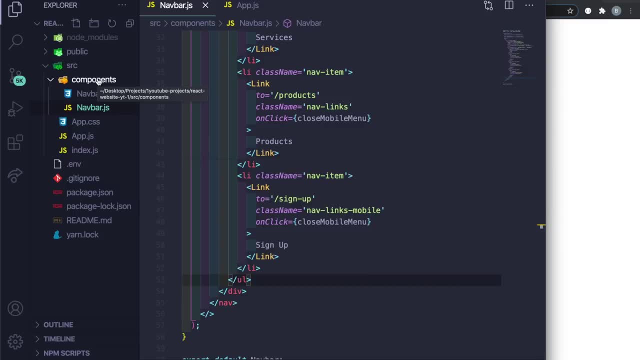 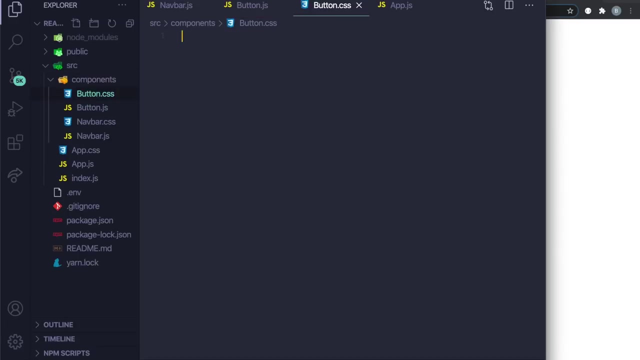 let's might as well import that, and then we're going to go ahead and change the class name and so let's go to components and right click and then go new file and just say button dot js and then also right click new file, button dot css. now in the buttonjs. 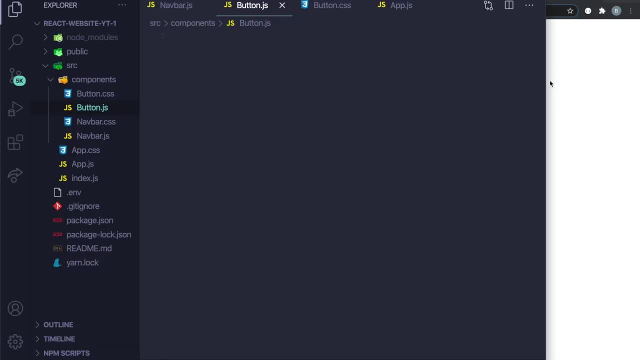 this one is going to be pretty much reusable across the website, so let's go ahead and do. let's see. i'm just going to imr and see if that works. yeah, i guess it's. i think it's because my um, my vs code. i think it's because 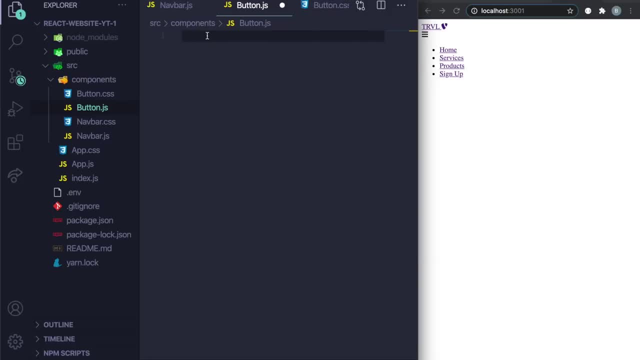 i stopped. let me try something really quick, one second, all right. so basically i just closed out vs code and restarted it and essentially now when i do the shortcut snippets, i can basically just type them out and press enter. so if you download and you're like yo, why is it not working, or? 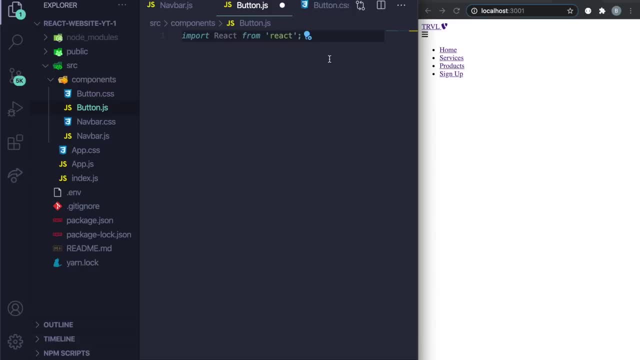 sometimes it randomly doesn't, it just stops for no reason. just restart vs code and you're pretty much back to go. you're pretty much set to go. so here we're just going to import the dot slash button, dot css, and then, lastly, we'll have to import a link. so it's imports curly brace link from react. 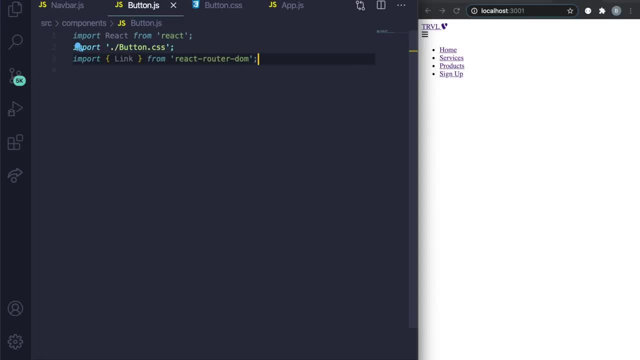 router dom, save it and then let's command b so you can see this. so right now let's create the button. so i'm going to automatically export it. so export cons button. i'm going to set this equal to parentheses and then, inside of here, the curly braces. 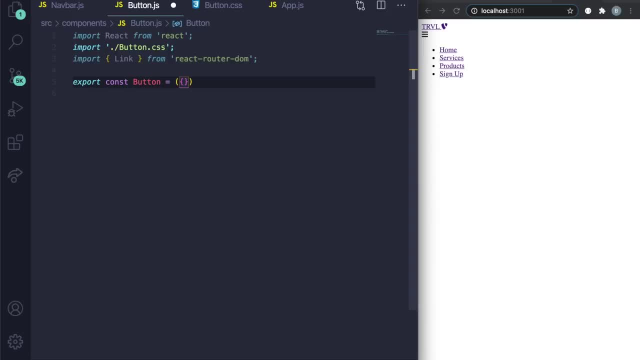 i'm basically going to pass in properties in here that you'll see the point of this in just a second. basically, let's do uh children type on click button style. so this is essentially the class and this is what i'm calling it here, and then a button. 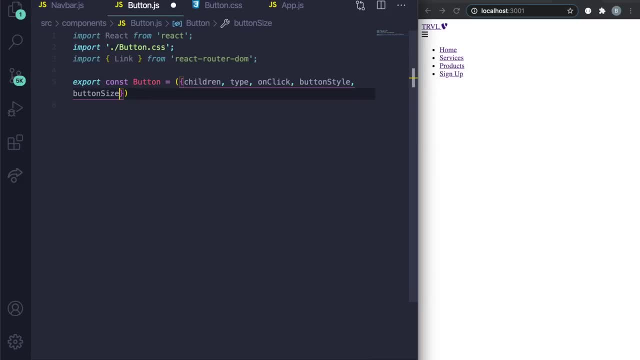 size, and then, outside of the curly brace and outside of this parentheses, we're going to say arrow function here, and then we're going to set it equal to basically some logic. so, within this logic, let me actually save this and see how it looks, right. so here, press enter. we're going to create this. 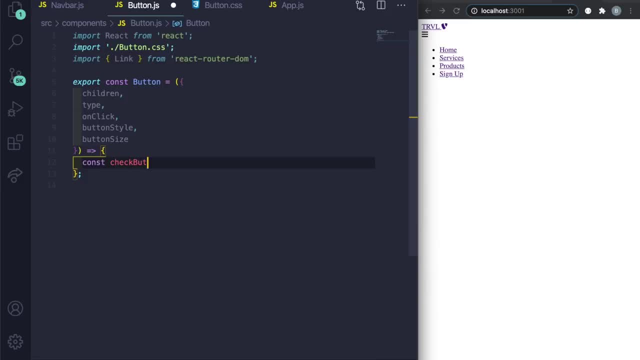 button style function. so const check button style and i want to set equal to styles. dot includes button style. now, all this, all this is going to make sense once i finish it out. you see how, where we implement this and basically here let me show you real quick, let me make this bigger. 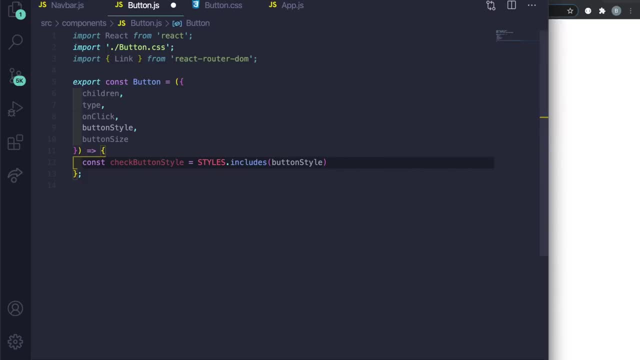 if the cutting component has a button style, then if that is true, then i want it just to be whatever the bun style that we created for it, and if it's not true, i want to set the value to to styles, the first option in our styles array. so we're going to actually create this above. 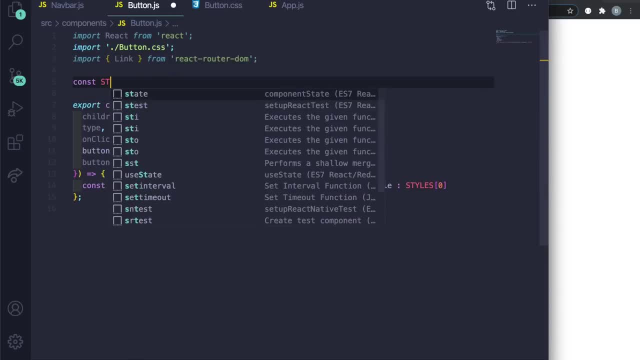 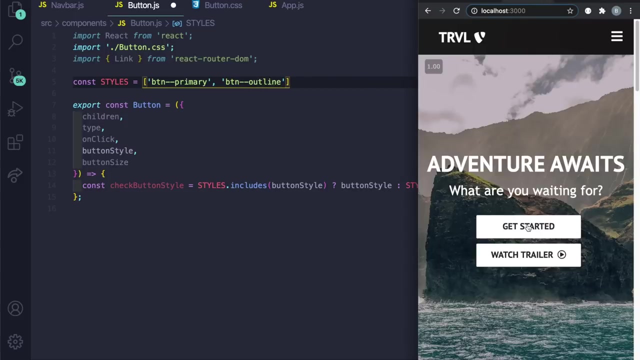 and here we're going to say const styles is equal to an array and these are essentially our css classes that i'm automatically creating right here. so i'm going to say btn- dash- dash- primary and then comma, btn- dash- dash- outline. so this was this is the outline version that gets started, and then the this one's primary, because you can see, 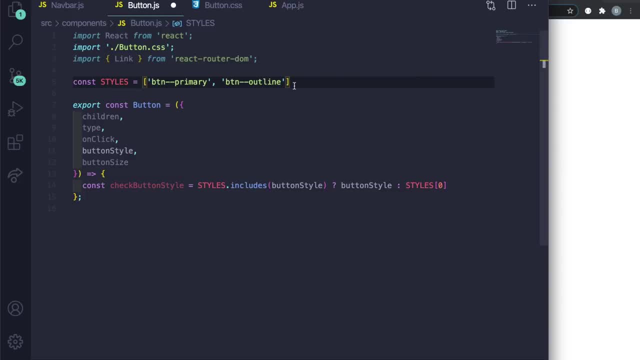 it the actual background, and these are all CSS classes that get automatically the applied depending on how you, on what project, pass in and I can say cons sizes. but now this is better, it's bigger, large, and there's gonna say button dash, dash, medium, and then we're gonna say button dash. 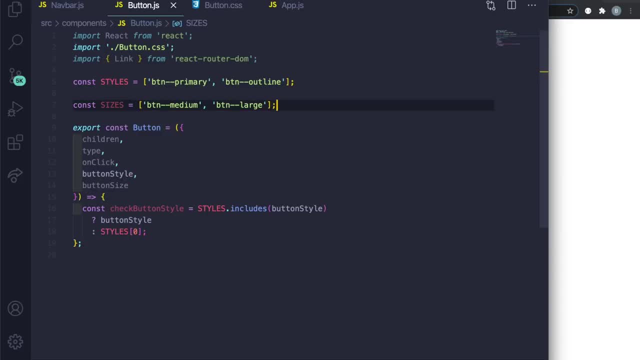 dash large and let me say that really quick now. right now here it's gonna say styles I include. so you put a bun style which I'll show you once we have the button component created, then it's gonna apply whatever. that is right. so it's either gonna be button primary or button outline. but if 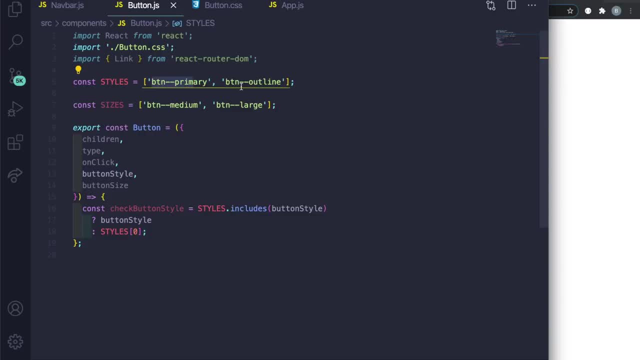 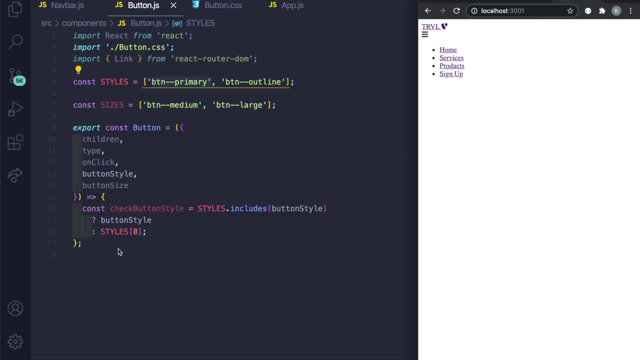 you don't have any of the classes applied to it. it's automatically, by default, gonna apply styles, the first position, which would be button primary, by default. so that's why these this is by default, but then I had to add the outline style, this one, so that it gets applied to it and you'll understand this once we get done. 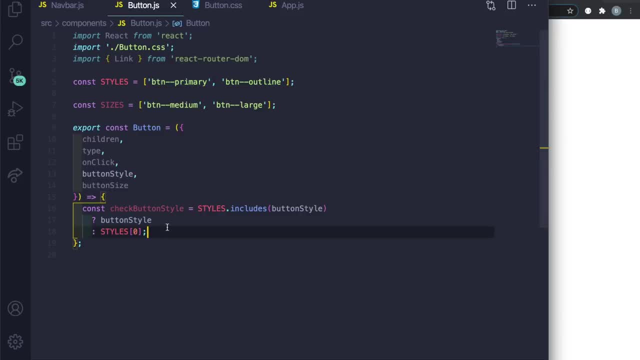 to uh coding this. so go inside at the end of the styles and press enter, because we're still in the curly braces, and then we're gonna basically just say the same exact thing for a check. uh, so let's say cons, check button size, and we're going to set it equal to sizes. dot includes. 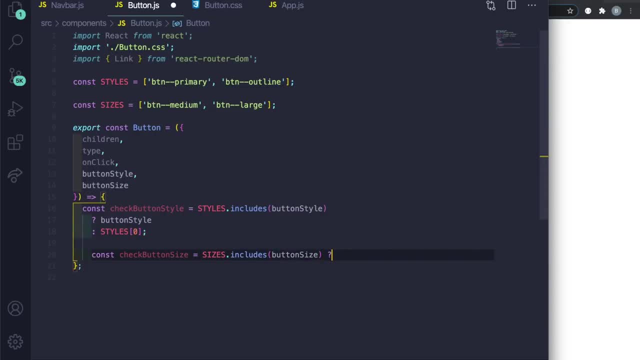 it's going to be button size. so if that has a button size, then change it to that, so it'd either be medium or large, whichever you put. and if you don't put anything, then it's going to default to the first position, which would be button medium. now, underneath this, we're basically going to return. 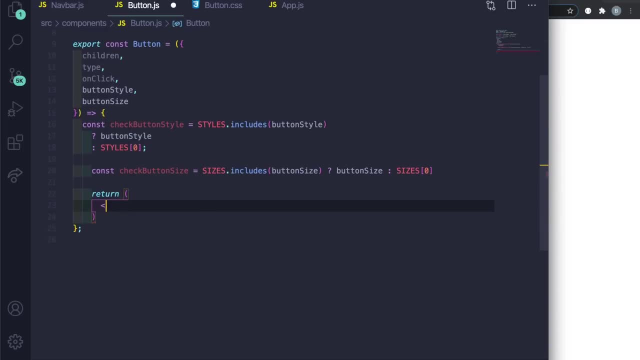 the C's. let me scroll up real quick and I want to return a link. I'm going to say two equals quotes and I want this just to go: sign up doesn't really matter where you put it. I want the class name equal to BTN dash mobile and then inside this link we're going to have the button and let's just close the. 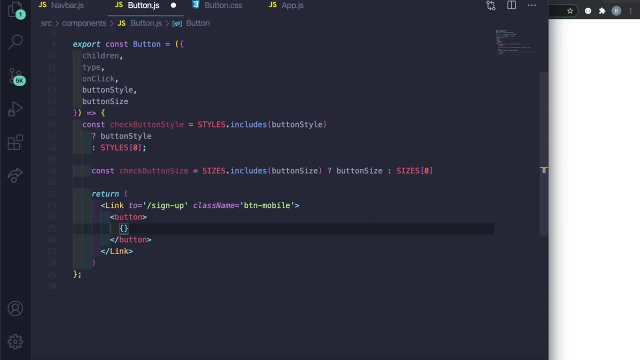 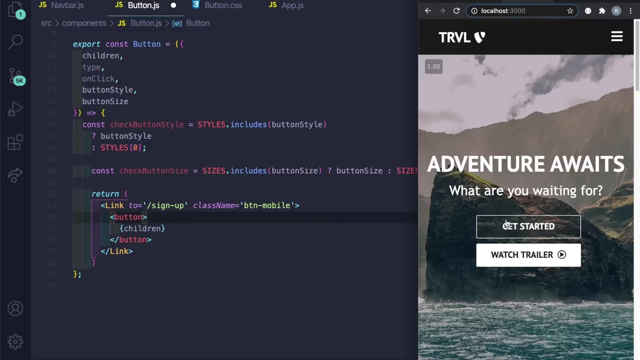 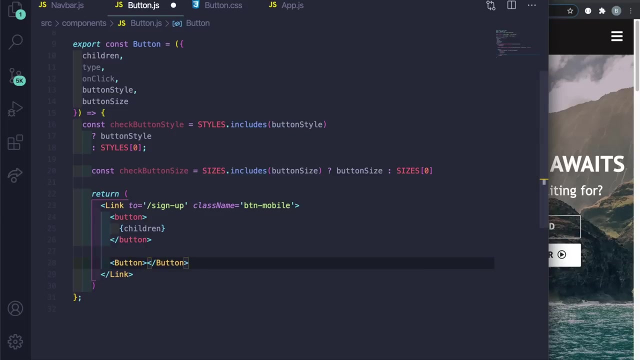 tags out really quick and inside of the button I'm going to pass in curly braces and the children. so what this does is whatever you put inside of the button, it's basically going to render that so like, for instance, get started. so if this was another component, it would be like button, and then I would 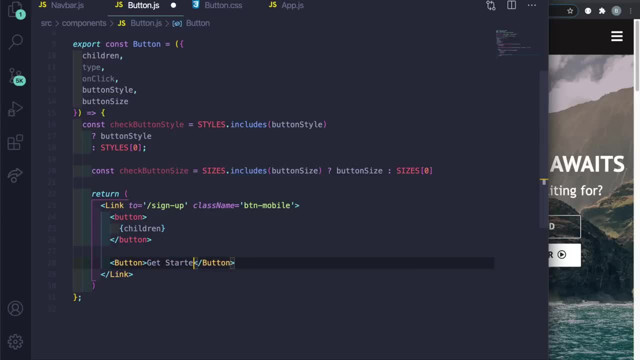 say get started, and that's, that's the children. so whatever I pass in here, it'll automatically display that as a component which you'll see later on, and that's basically whatever we put here. and then let's go and on the actual button let's add a bunch of uh things here. so let's say class name, let's say equal to curly braces and under. 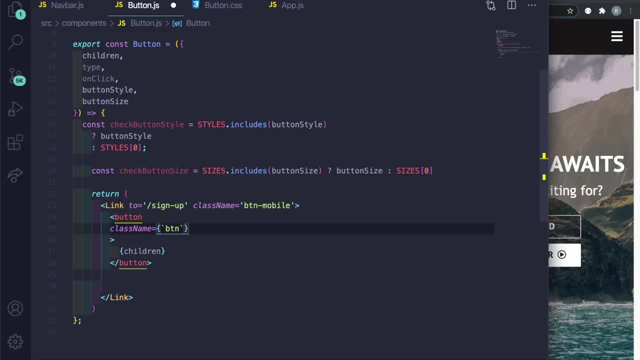 the back ticks, I'm going to say BTN is the default class space, dollar sign curly braces. and then when here we're going to say check, but in style. and then Dollar Sign curly brace is going to say check button size. so that's the class name, so that's why we can update these whatever we like, and then on. 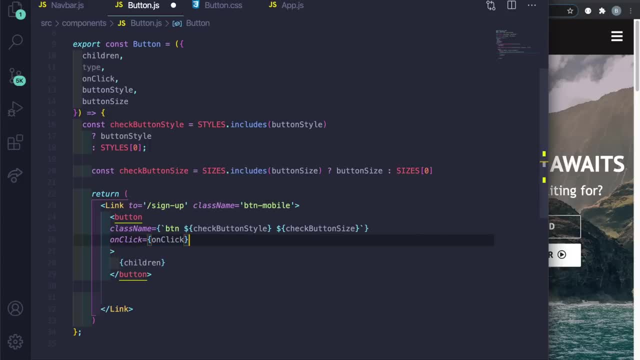 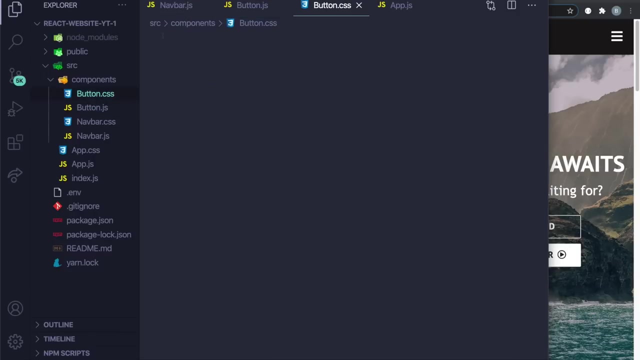 click. we're just going to set that to on click and then type. we're just going to set that to type. now this pretty much is the button component. so let me save this and then let's go into our buttoncss and let's start adding the css. so here i'm going to say colon roots, and then i want to. 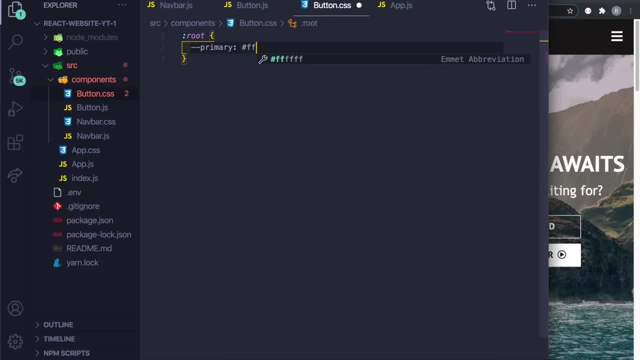 set the primary color to just white, so this way we can actually update it at the top instead of having to go through every single one individually. i'm going to say btn. i'm going to set the padding to 8 pixels by 20 pixels. border dash radius to be 2 pixels, outline going to be none border. 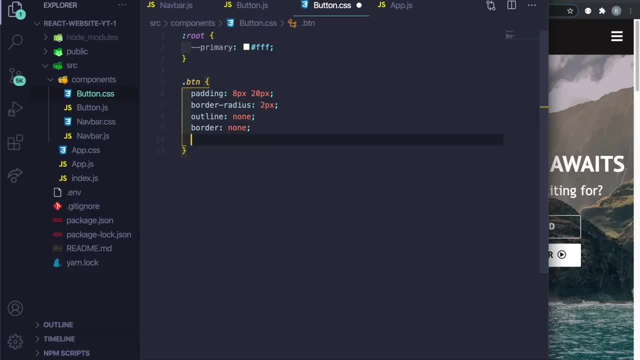 going to be none, and then cursor will be pointer, and then let's do dot, btn, dash, dash, primary. so now this is the css class that we created back in the button component. so this is what we're adding. now the styles. so here's going to say: 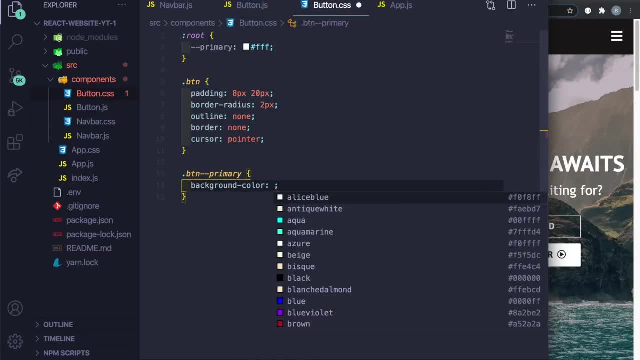 background color. let's just say var, so var, dash, dash, primary. so that's going to be white, and then color, so the text hashtag: 2f242424. and then let's do border 1 pixel solid 4, dash, dash, primary. and then under here let's do btn outline now, so btn outline. 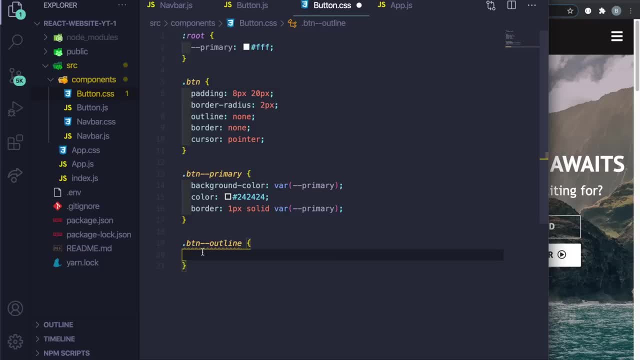 should be double dash. we're going to say same, but you know, let's do background color transparent and then the actual font color to be white padding will be 8 pixels by 20 pixels and then border. we can actually keep the border the same, so let's. 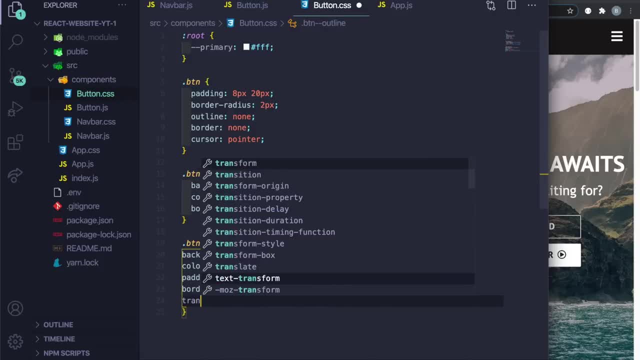 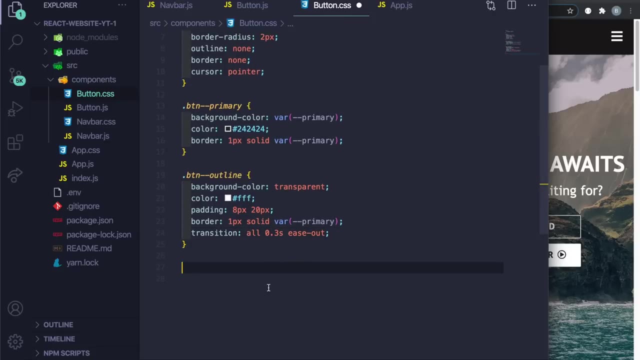 just copy this code here and i just want transition, not transfer transition, to be all 0.3 s ease dash out, so save that there and then let's just do the sizes now. so pretty much dot, btn, dash, medium, and here we're going to say padding. 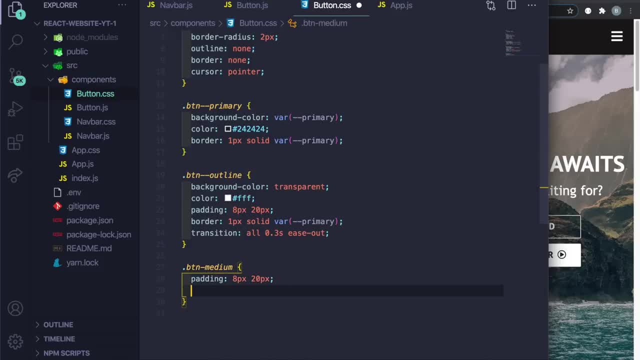 to be 8 pixels by 20 pixels, and then font size to be 20 pixels, and then we can say that btn dash, so they should be double dash. just keep forgetting btn large. and now we're going to say padding to be 12 pixels by 26 pixels. 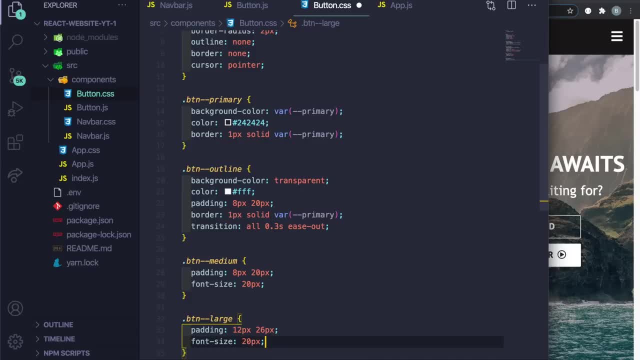 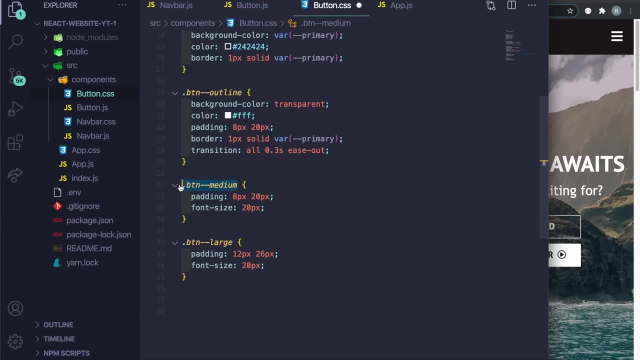 and then font size to be 20 pixels and, last but not least, let's just create the hover. so let me just copy this down here and just say colon hover and I'm gonna say comma. then I copy the BTN large colon hover and we it's a space in here and basically I want the background to be hashtag white and there's a 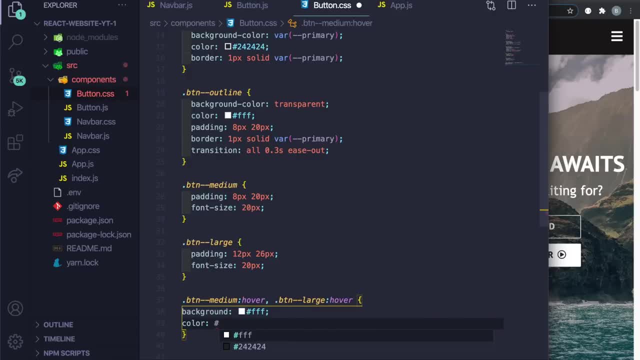 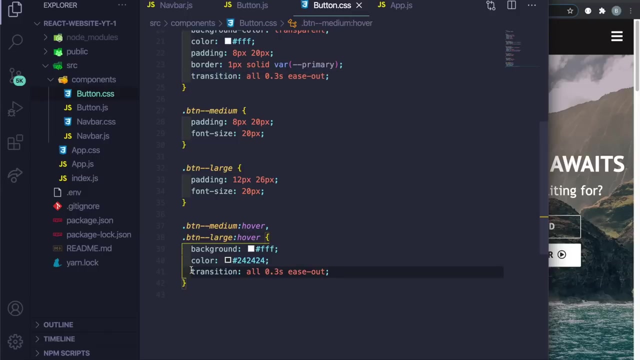 fashion, color and color. I want it to be colon, not colon. a hashtag: two, four, two, four, two, four and then transition to 50 ms. well, that's trans. yeah, transition should be this into 50 ms. actually, we can just add this here. let's just do this, just copy this, make it easier, save that. so now we're. 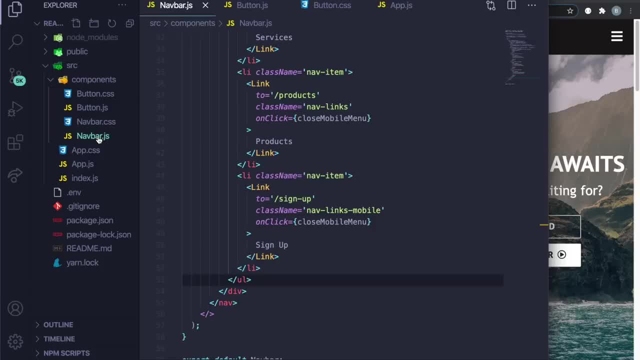 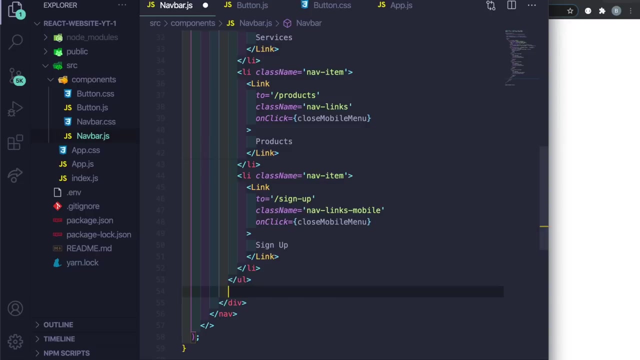 pretty much done with the button component. so now let's go to our nav bar- that J s- and let's actually implement what we just put in here. so now under the ul, let me go back to my actual app here. so I save, save this. nothing happens. but under this ul and the nav bar, 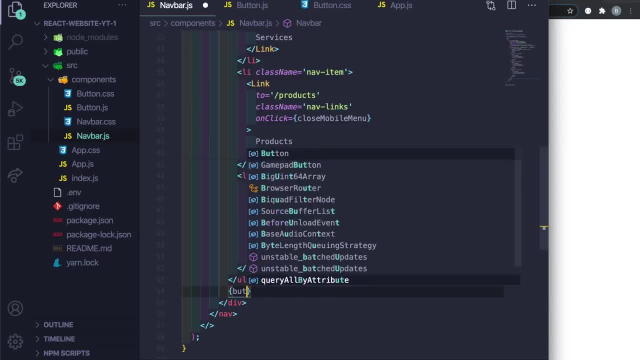 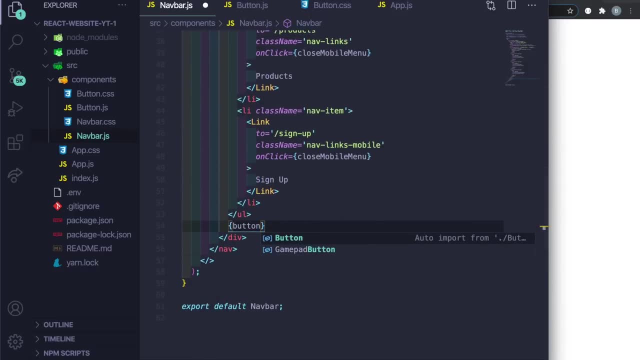 component. we're going to say curly braces and I'm going to say button, which we're going to create. I don't think we have this yet created up here, yeah, so we haven't created this yet, but we can create some state and essentially we're going to put: if button is true. 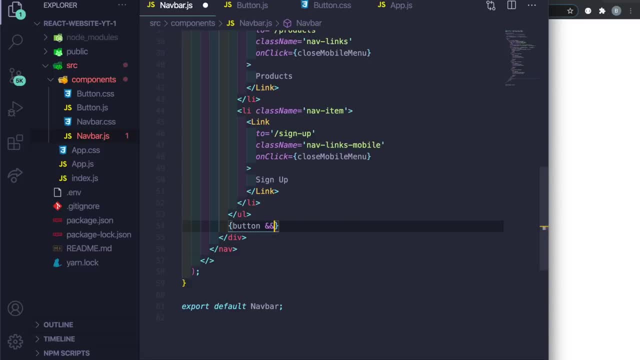 then we're automatically. this is a shortcut where you do double and it's going to just straight up return whatever is after this. so, if it's true, and return the button component, so it's a capital letter B, and let's pass in sign up. so right now, if I save this, nothing's. 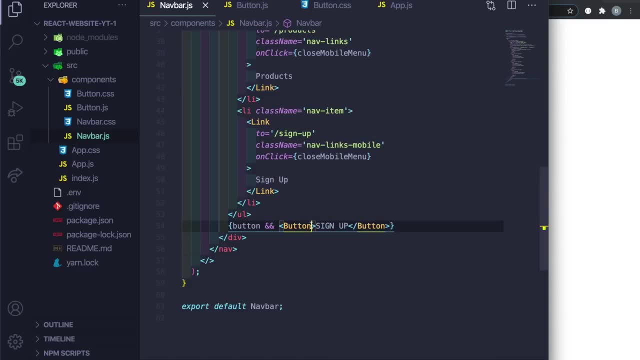 going to happen. but this is essentially the children we're passing inside of that. so that's what sign up is. and then here's where we created the button style. so I'm going to say button style and I want this equal to btn dash dash outline. so if I save that, this is automatically making the 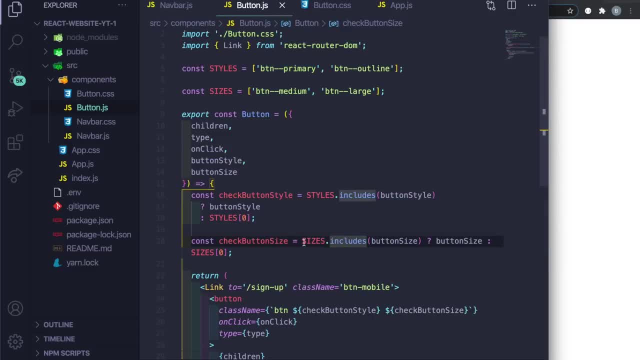 sign up an outline because by default, if it includes a bun size or unless a bun style is going to be whatever the style I put, which was here btn outline, so it's going to make it the class of this bun btn outline. now, if I didn't put that style code right here, 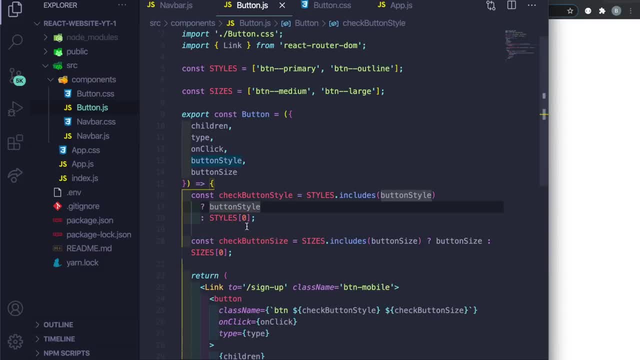 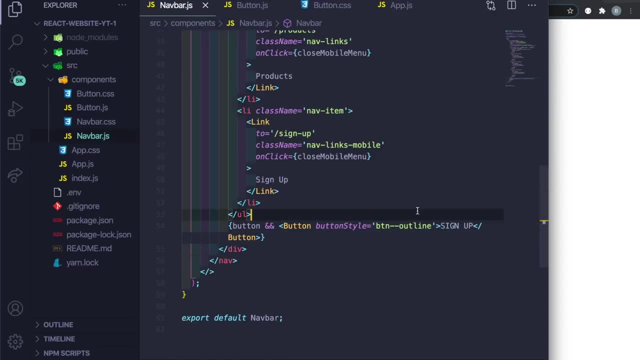 this again, this bun style btn outline. then it automatically defaults back to style of zero, which would be the btn primary. so this is where this comes in, in case you're confused about that. so let's go back to the top up here and let's just create some states, let's say cons. 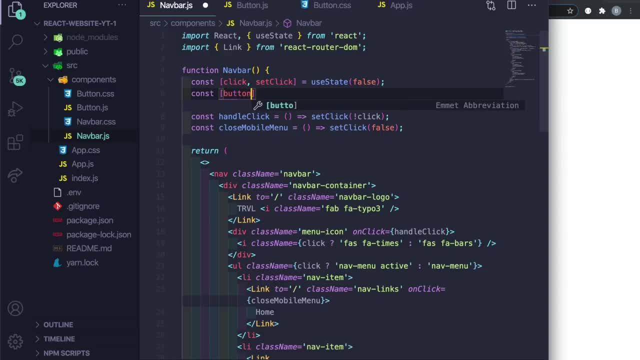 and then pretty much the passing in. I'm going to say button and then just set button. I'm going to say equal to use state and I'm going to say true, and and now? all I need to do now is go up down here to see right here, underneath this, and 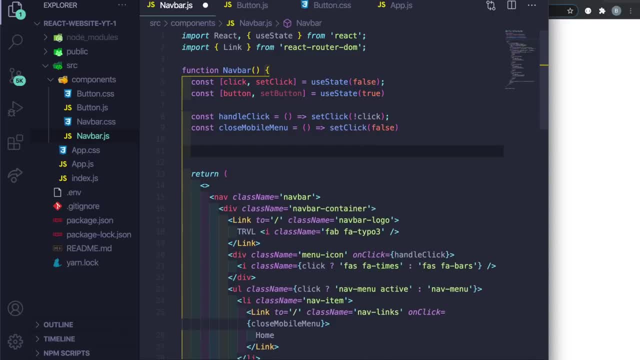 this is essentially a function that is going to display the button on mobile, or actually removes it and then displays it depending on the screen size. so I'm gonna say cons show button, so that equal to the arrow function, curly brace here. and I'm gonna say if window dot. 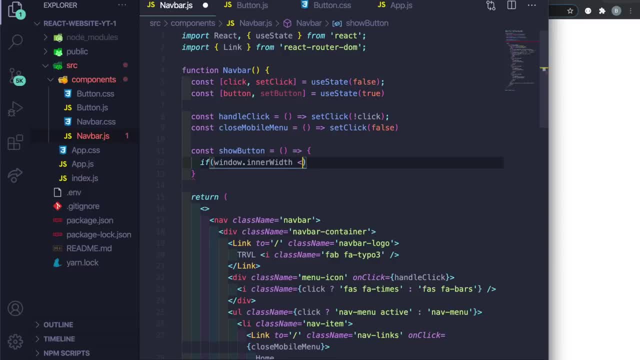 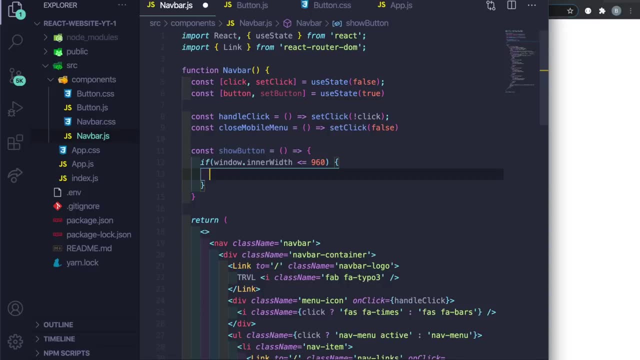 inner width is less than or equal to 960.. you have to put less than or equal, because if you just put less than at exactly 960, it's going to show up. I want these button, so I'm going to set the button to false and then, if not, if the window is much bigger than that, then just basically, or. 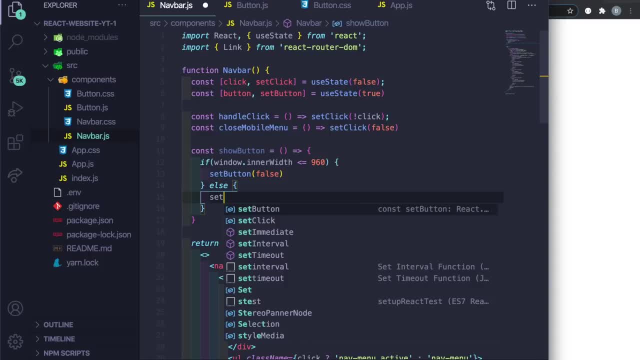 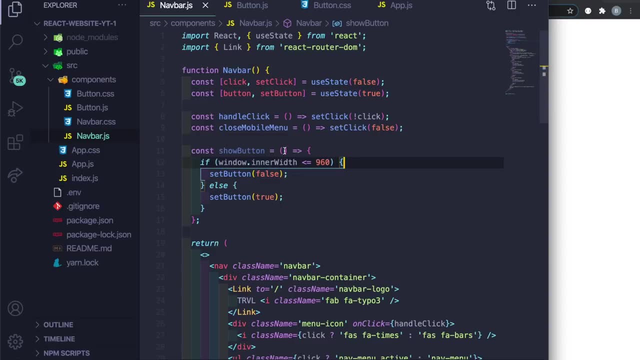 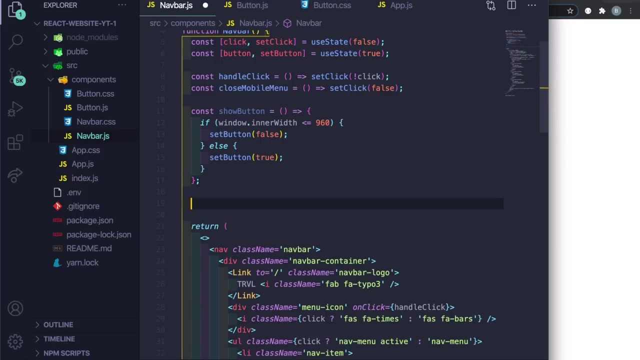 it's just as long as it's not 960- it's bigger than that- it's going to set the button to true. I'm going to say there's nothing's going to happen, because we have to actually invoke this function here, and then also so we can go underneath this and I'm going to add window. 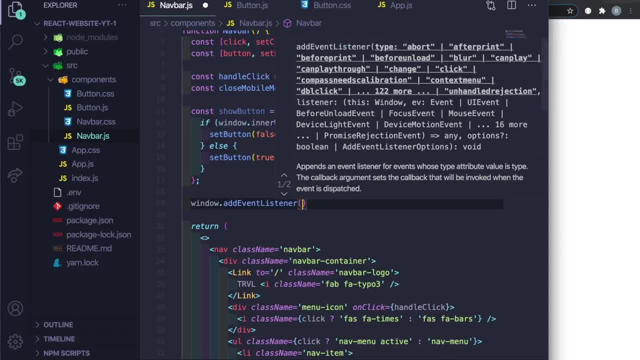 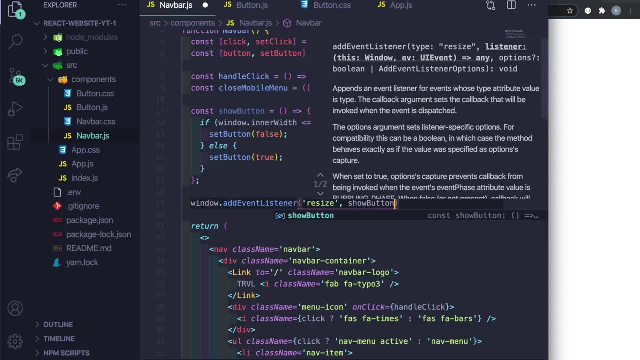 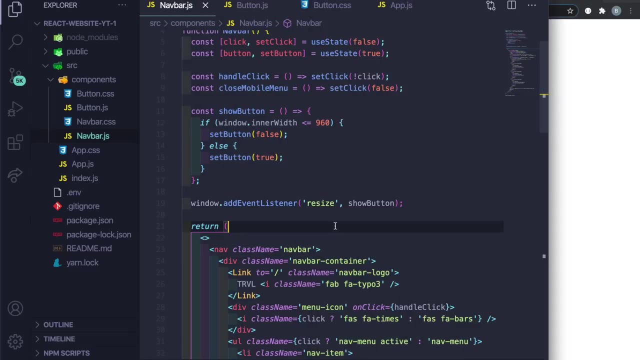 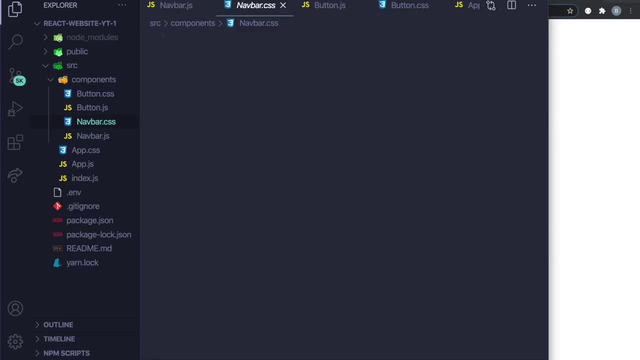 dot. add event listener and pass and resize. so whenever I resize the screen I want to get show button to basically work for me. so now I can't see anything yet because we haven't added the actual CSS to the nav bar. so let's actually add that and then pretty much let's go ahead and type this in. so 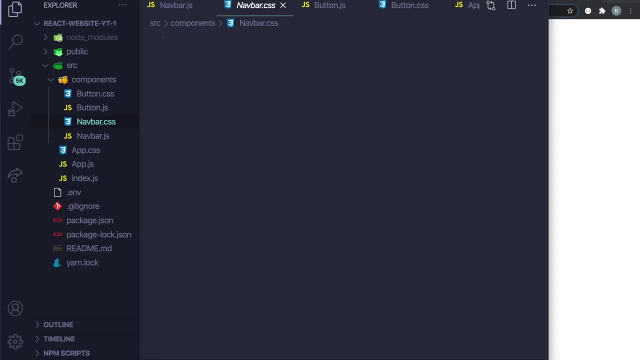 there's the easy way and there's the hard way. so the easy way is we could just straight up copy and paste this into the code, and that's probably what I'm going to do, since this is more react based. but if you wanted me to actually go line by line, I could, but I feel like if I did that for free and do anything directly, there's a lot of balancing here on thought, there's a lot of on the another side of that line of code, really in our application. so, please, please, be homes to rerator accessibility for maybe auto up if you haven't устрой the phones, for we could just kind of copy and paste this into the code and that's probably what I'm going to do, since this is more react based. but if you wanted me to actually go line by line, I could, but I 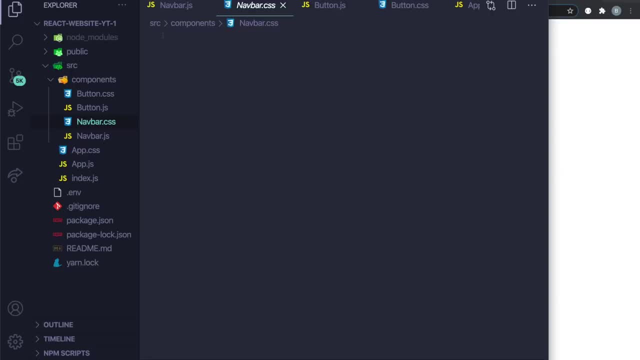 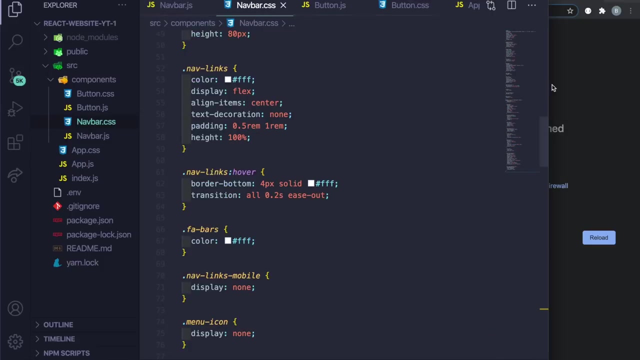 actually go line by line. i could, but i feel like if i did that for every single thing it would take like a century. so i'm just going to copy this in and paste this css right here and now. if i save this, i need to go actually go back to. and also, you're wondering: where did i get this code? it's. 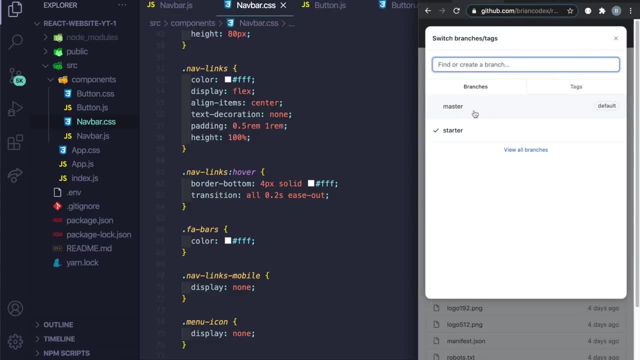 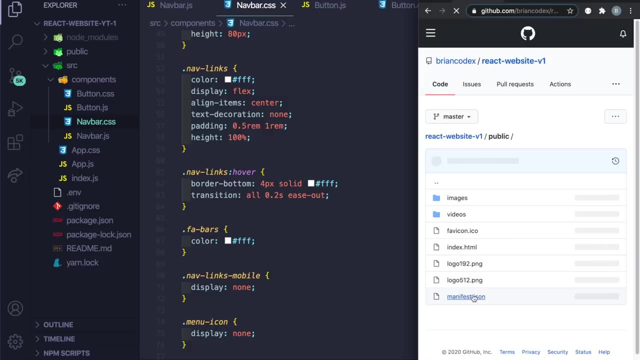 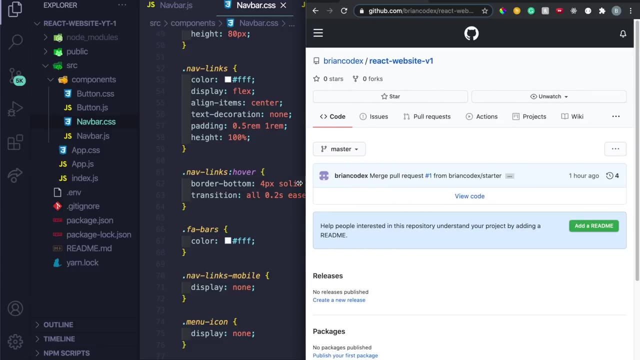 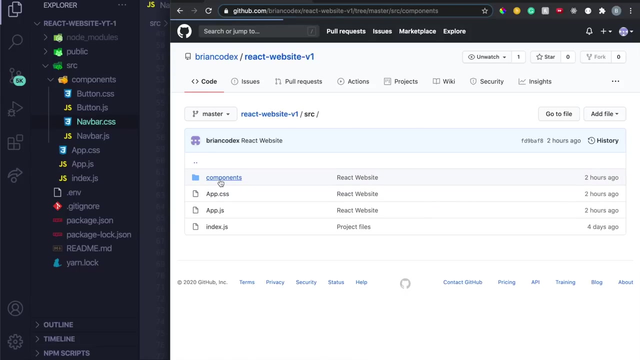 on the github. so i have the starter and then i also have the master branch so you can see all of the css. so you can go to master branch and go basically to- let me see shrink out really quick. you can go to the src, go to components and then go down. let's see to navbarcss. 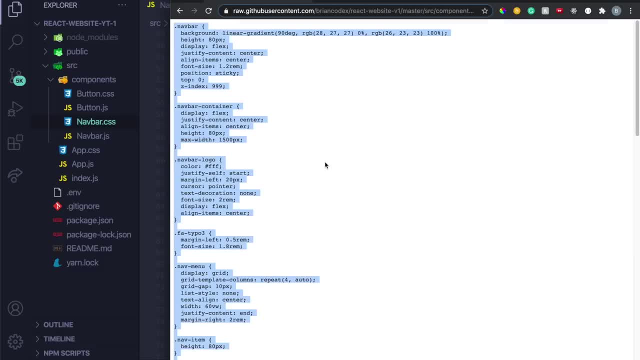 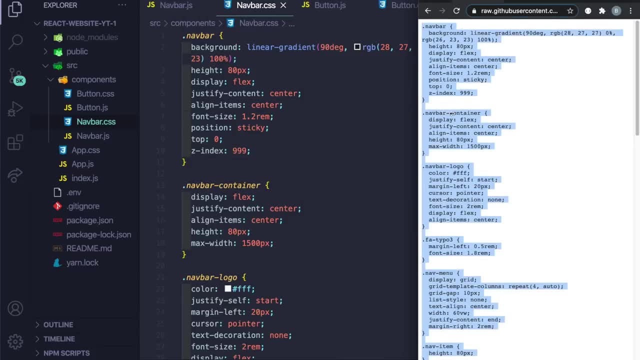 go to raw command, a command c, and then just straight up paste that in and boom, now you have all of this code here. so that csu, literally that's going to take me like probably like 20 minutes to go through, so i'd rather not and then go over. 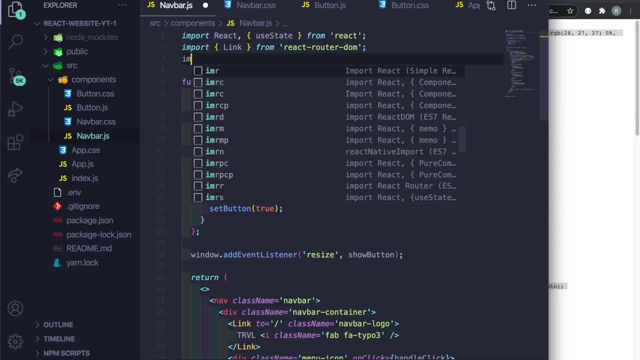 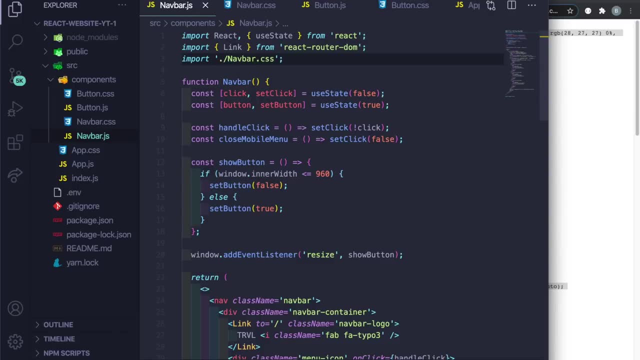 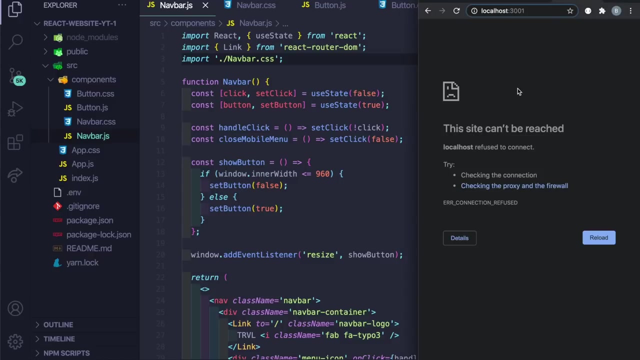 to navbar and let's import this. so let's go import dot slash nav bar, dot css, save that and let's actually. let's go to my app now. and why is it not working? it looks like, i think command j. yeah, actually, i don't even think i'm running my app, because i restarted. i forgot that. 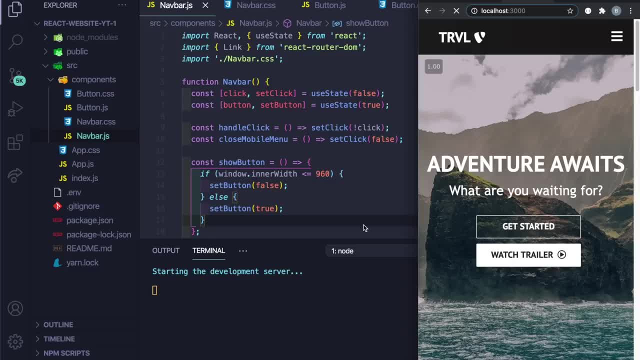 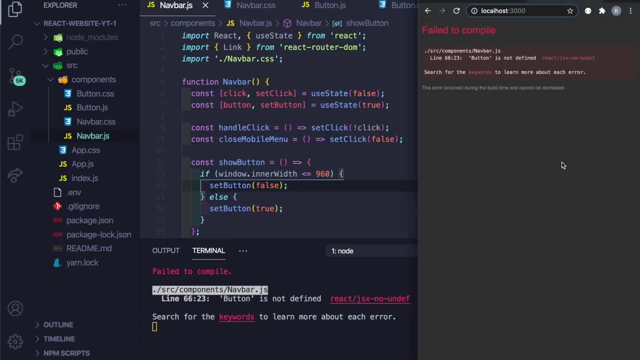 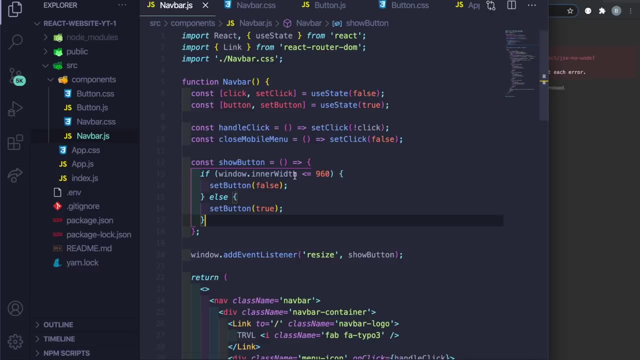 was what happened. yeah, it's going crazy. i was like: why is my my screen looking way different? all right, so right now you probably run into this to see button is not defined. so basically all we need to do is import button from the button component folder, so i can just go. 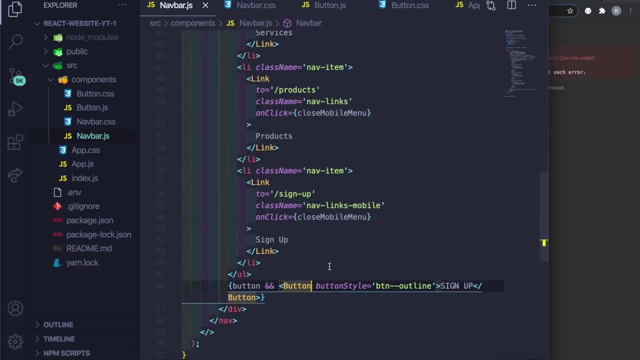 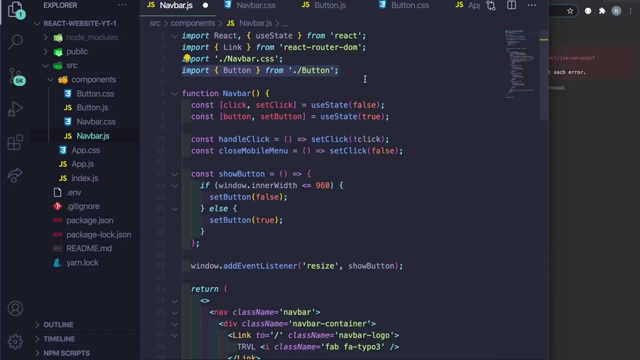 i'm gonna go here at the end and hopefully this works this time- control space and then see how it has the button. i just press enter and what happens is it auto imported for me. and also, after you type it, i also press enter too. if it doesn't work for you, just type this line: 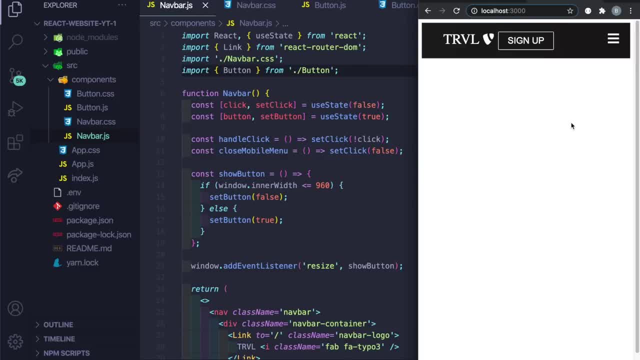 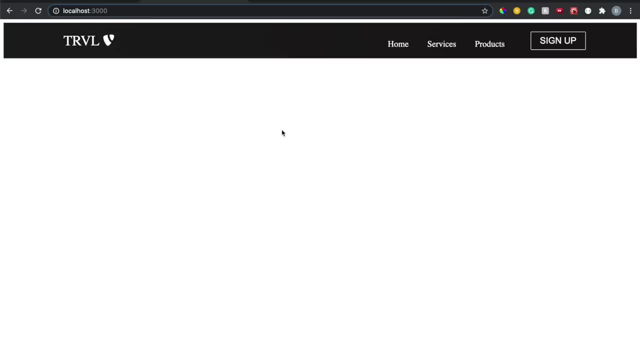 here, import button from button, we'll save this and now you can see we have a pretty looking nav bar right now. but basically here you can see that it looks like this, and then we have to add some global styles to this, but pretty much what happens is. 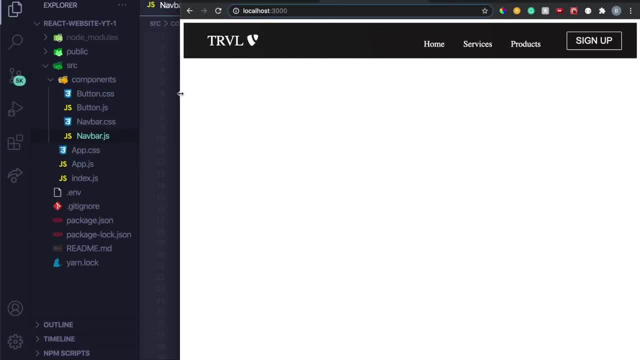 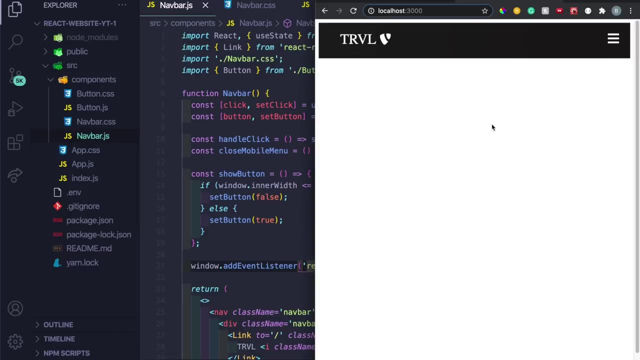 when i shrink it you can see here- the button disappears, and that's because of this code. the window width is 960 or less, so it's basically toggling and resizing the button, and then when i go back we'll toggle between here and we also have this right here. so the 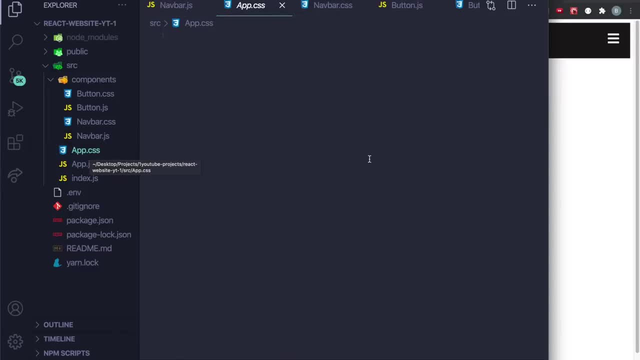 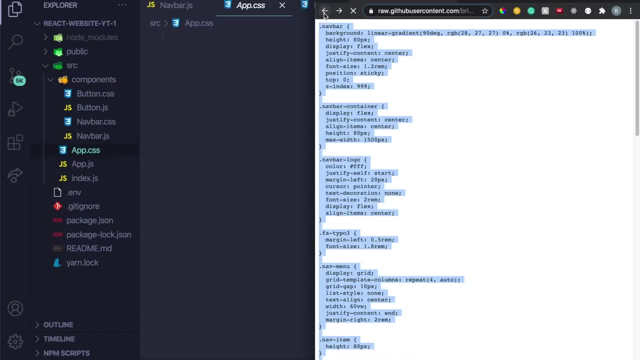 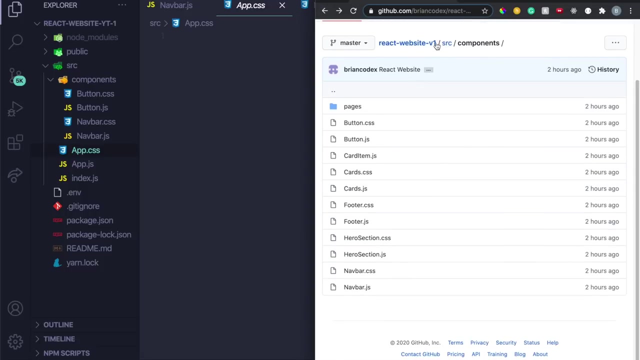 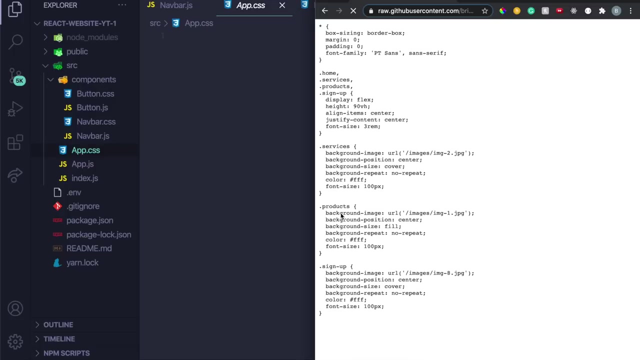 difference is the appcss actually is missing some style. so let's go here back to our github and let's add in those appcss styles, because this does not look as nice as what i showed you. so let's go back to the src, go to appcss and then go to raw and let's command a command c and then command v. 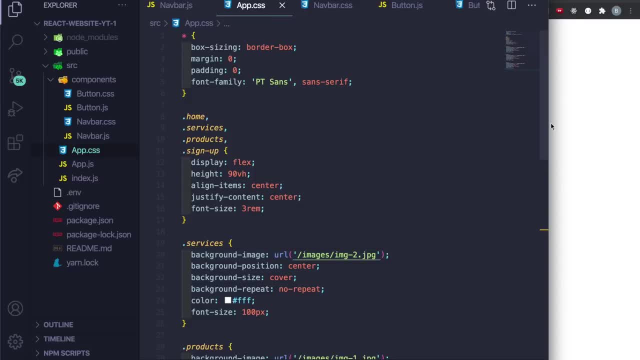 and these are the additional pages, so you won't probably notice these yet. and then also, we need to import this font so we can go to google font and actually do that, or i could just straight up take it for my file. that's probably the easiest way, so let's actually do that. since we're here, 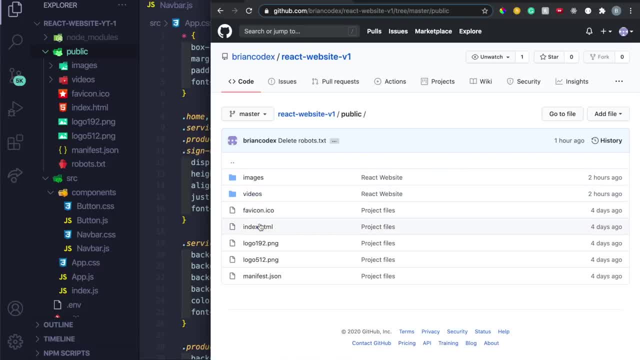 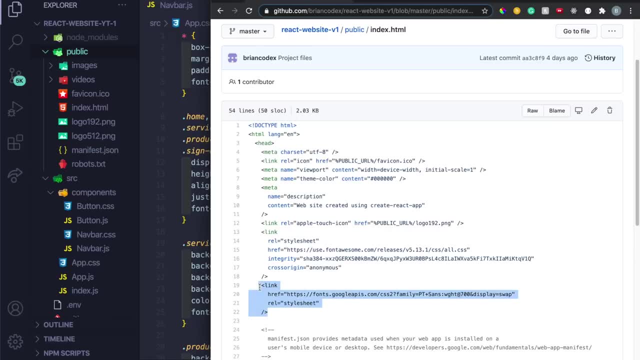 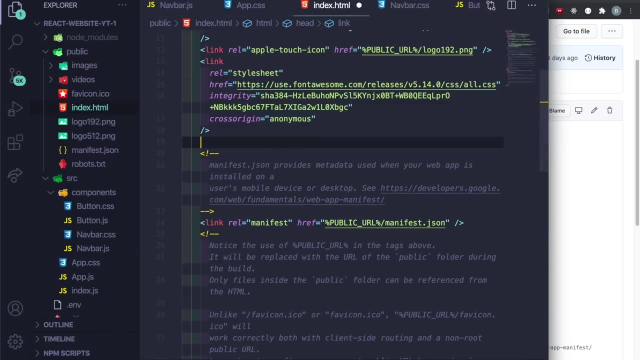 pretty much. let's go into a public folder, go into indexhtml and then let's see once it loads up. i want to take my google font right here, so this one between line 19 and 22, command c, this go to indexhtml, or you could import whatever google font you want, but this is the one i use. 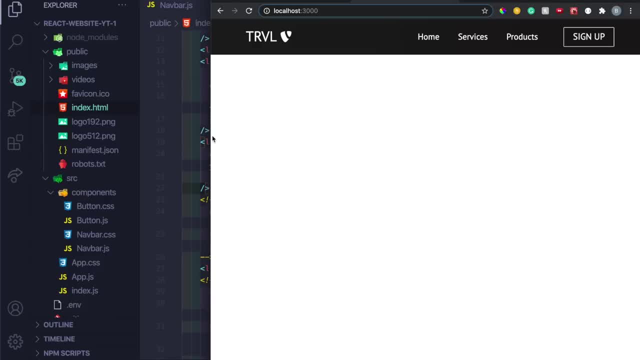 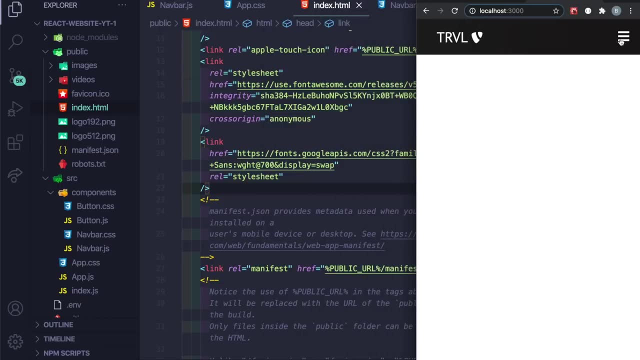 for this site and let's see how the site looks now. all right, so now it looks much, much better, much better to me, and then we can see you have, we can see have most of our stuff here. so now this it's pretty much. the nav bar is nothing crazy, and then you can see everything's working here, fine. 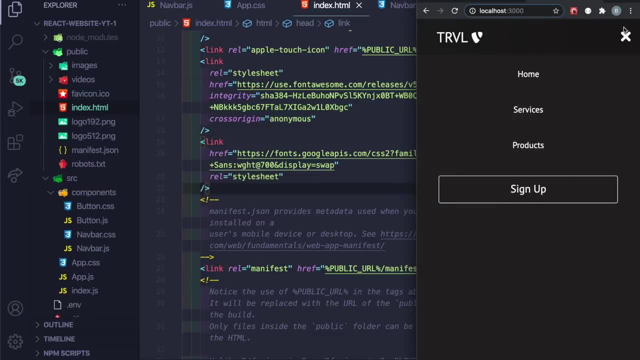 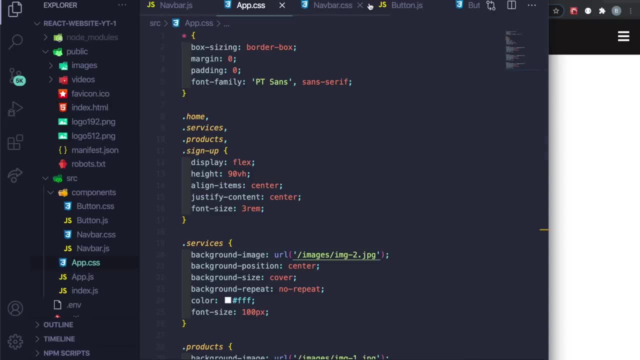 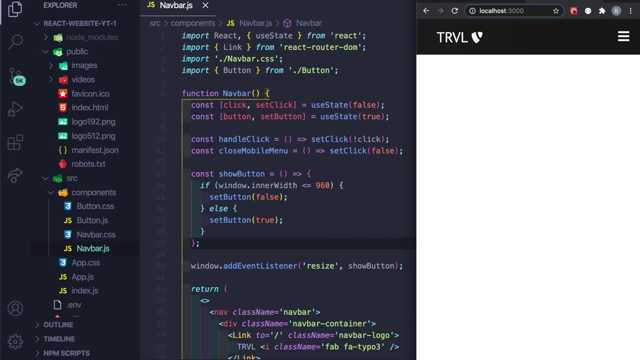 and then, when you click it, everything it basically set up. so right now, the only difference is the logo looks like it's not doing what it needs to do, so i should add some code there. but let me exit off all of this really quick. so now this: this is a little thing that um took me a. 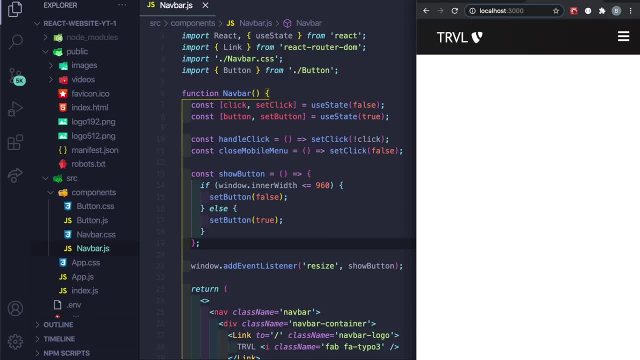 while to realize. but basically this is a little thing that um took me a while to realize. but basically you work in a web server with the app, so it's going to be very fast to do. some notice this until i um refresh the page. but right now what's happening is when i shrink, when i 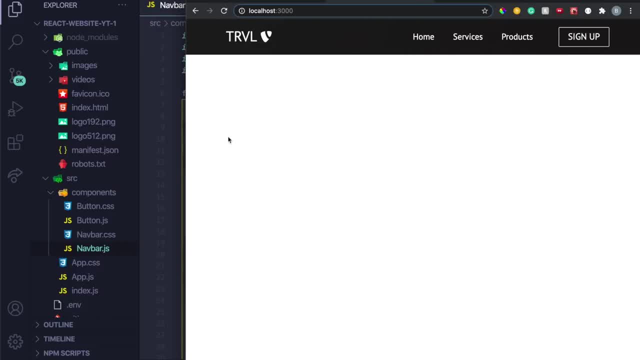 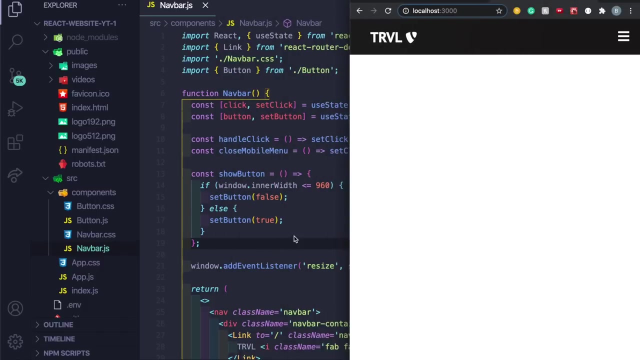 resize the screen- right the button- you see the sign up button. it it disappears. but the minute i refresh it's there again. so i gotta resize it. but every time i refresh it's there. so the problem is: how are we going to write logic to get rid of this? well, we have this amazing hook in react. so 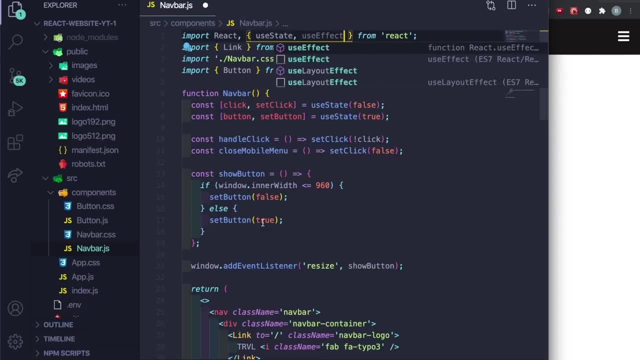 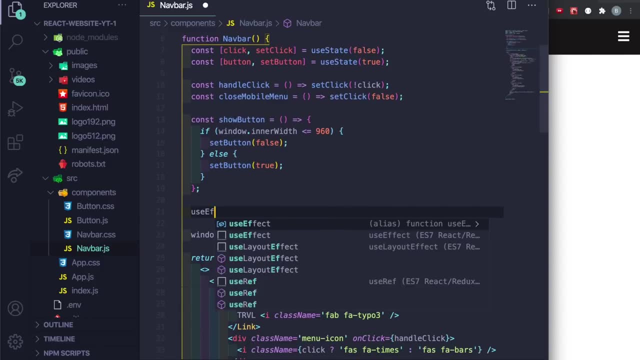 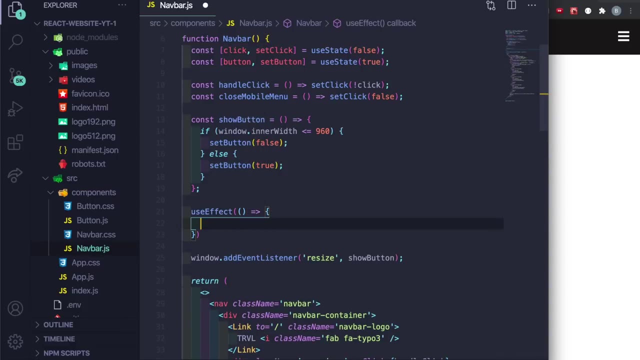 let's just say import use effect and basically it's going to allow it to just render that one time and then it's basically not going to show up anymore. so when i say use effect, i'm going to pass in empty parentheses, arrow function and then curly braces and i want to 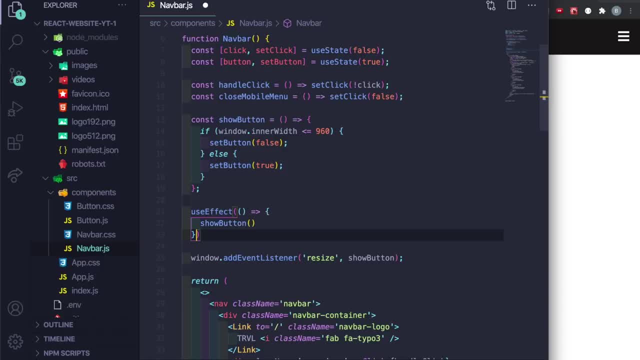 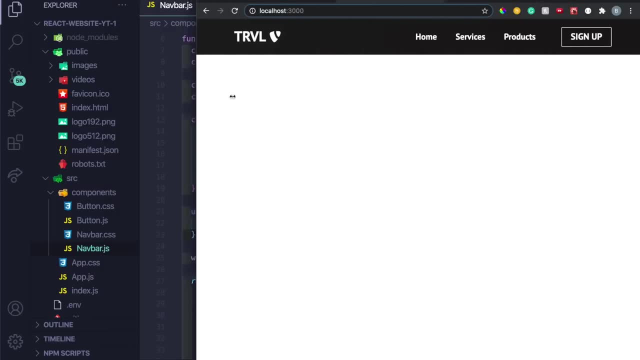 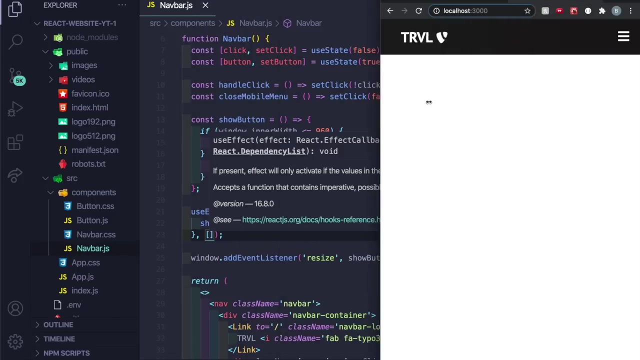 pass in the show button function here and then inside these curly braces we just pass an empty array. then when i save it now you can see it looks like this: i can refresh the page once i'm in mobile or tablet view and nothing shows up, so that basically we're utilizing use. 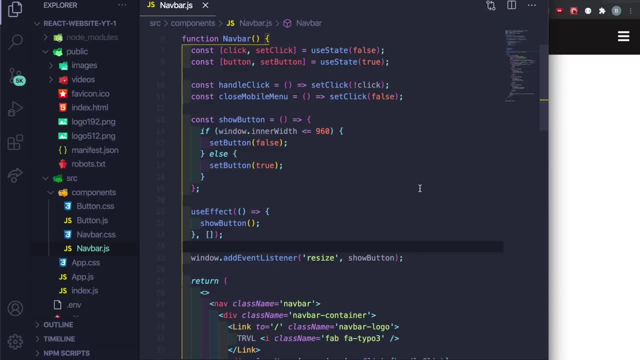 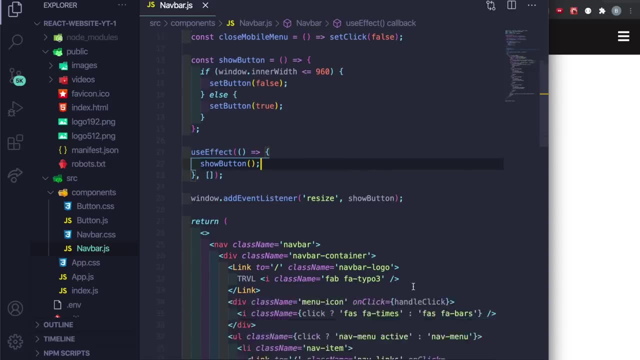 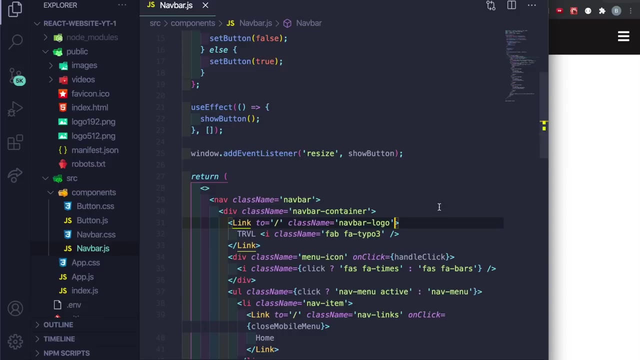 effect for that, so that it doesn't basically show up every single time i refresh and then boom, that's how we do it there. so now the only thing that looks like i need to do is add a on. yeah, close mobile menu function to my my logo icon here. so i'm gonna say: on click is equal to curly braces. 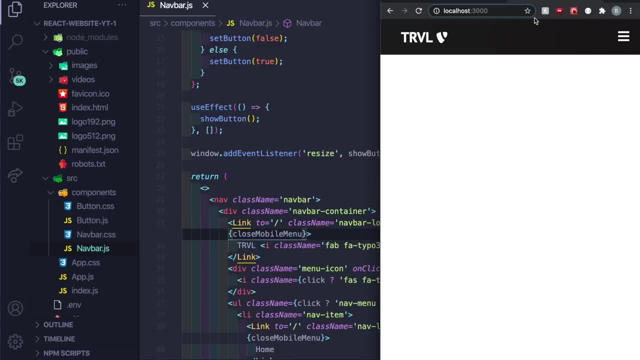 mobile menu and i'm gonna save this. so now, if i close or open this, all of these work so far, they should just make sure i check everything and then, if i click on the actual logo, aka the right there, it closes it as well, which is what this function does here. so i think we're 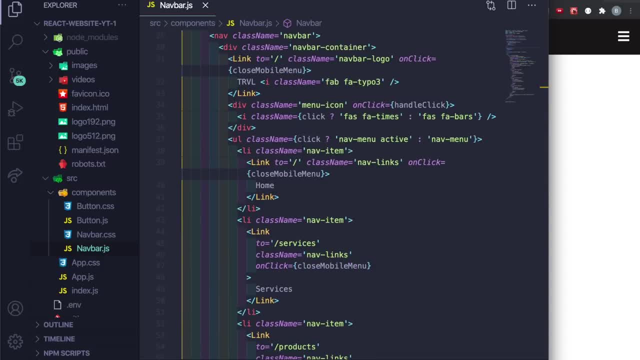 pretty much set on the actual nav bar. we should be good. so let's go ahead and start creating the- uh, actual- how to say- the hero section. i guess you want to call it. so let's, let's shrink this and then let's go to components, right click here and let's go to new file and let's type in hero. 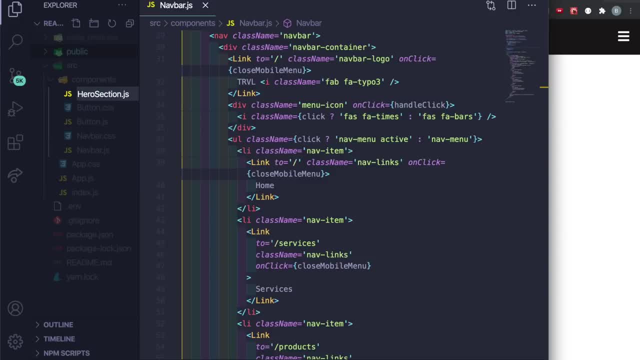 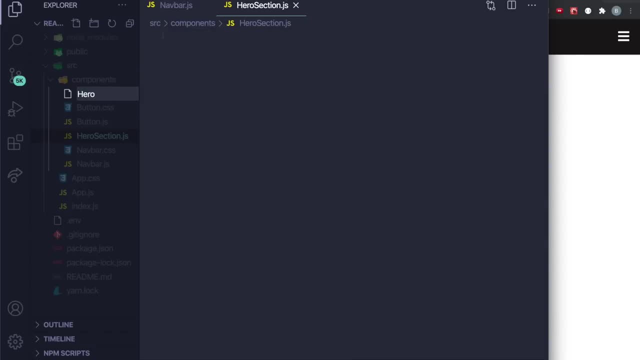 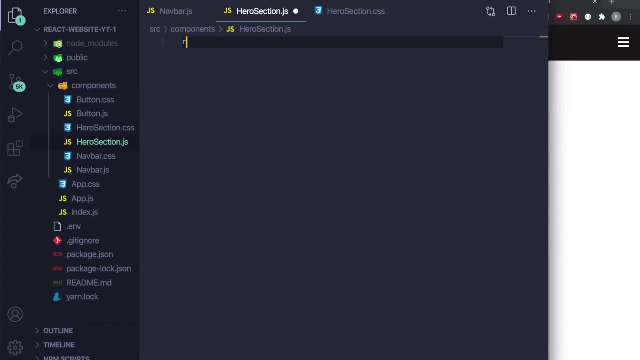 section. you can type you name whatever you want to. i just put this. and then let's create a hero section css. so new file here: hero section dot css. so now let's go to the hero sectionjs file and let's do rfce, press enter and we have our function created. and then 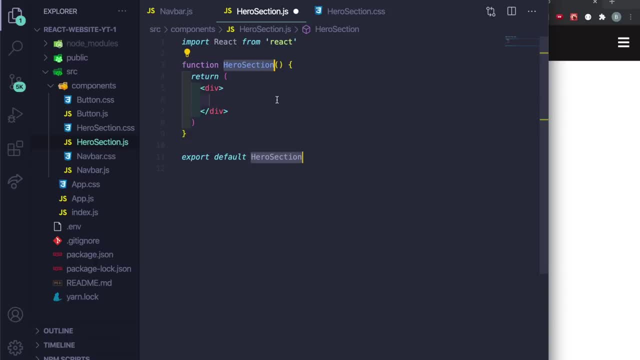 let's go ahead and start importing and adding the jsx. so here let's go inside of these divs and let me just add a class name equal to hero dash container and then inside of this, this is essentially where i put the video. so if you don't want a video, then you could ignore this line, but if you want to, 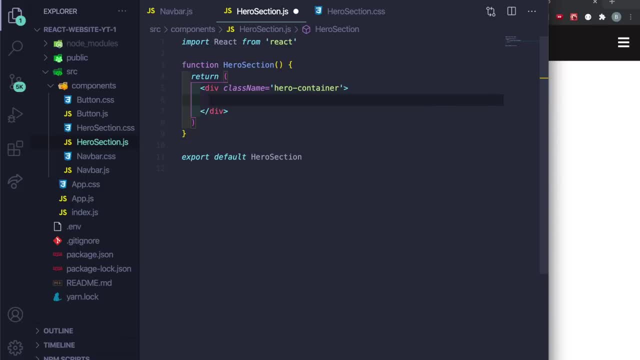 follow along and you can see how you can update it. then you can. so let's just do video src is equal to code slash, video, video dash 2, dot, mp4, and that's in the public folder, basically this video second right here, and then let's put auto. and since it's react, we have to say auto. 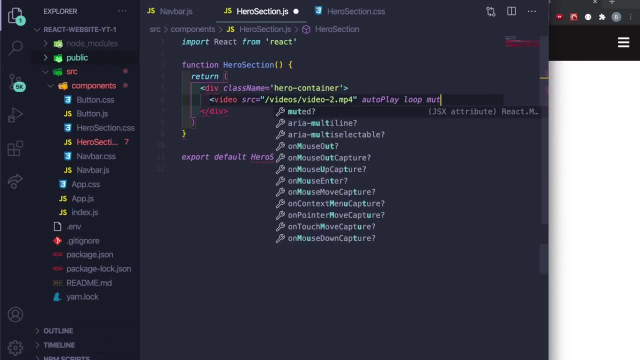 p with play. i want to loop and i want it to be muted. then under the video is where i have h1 and let's just put adventure awaits and then p tag and say: what are you waiting for? now, underneath the p tag i'm going to create a hero buttons. so basically i'm saying div. so dot hero dash btns. 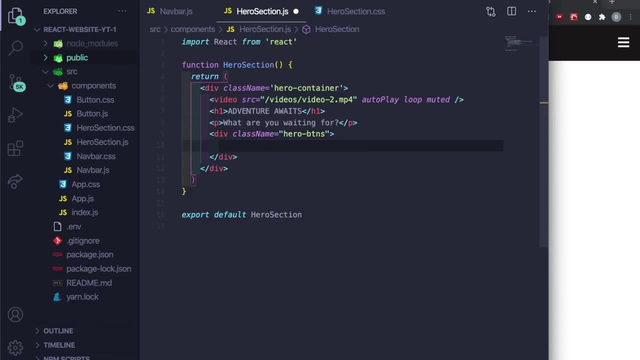 and then inside here is we're going to pass in the button component and so i'm going to say the button component, so i'm going to press tab and it automatically imported, as you see in the top, and then say class name equal to btn's. then i want to set the button style to. 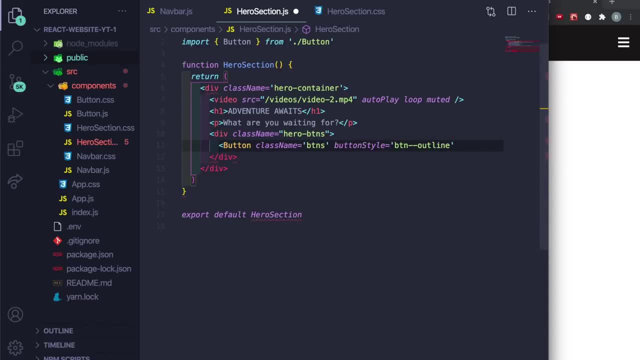 btn dash outline because i want this left one to be the outline. and then i want to say let's press enter. i'm going to say actually, yeah, but in size i want this to be btn dash dash large. and then i'm going to close it out and then i, by default, it automatically has the closing. 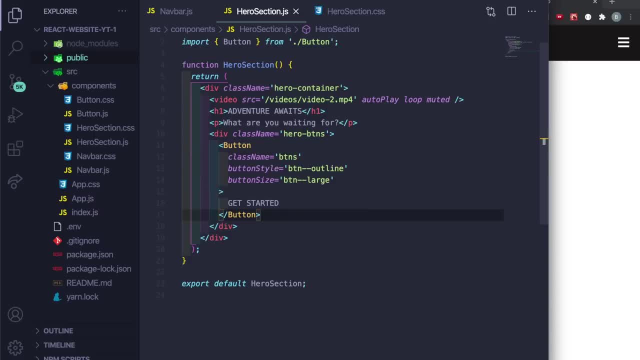 tag. i'm going to say get started, then i save it here and you probably can't see anything because it's currently there's no css. so let's go ahead and let's add the hero, second css. so let's go over here and i might actually type this one out. it's a little shorter but i feel like it's going to be. 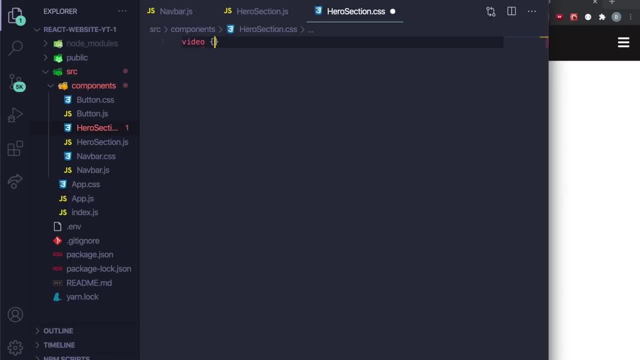 more beneficial if i show you this, because if i just copy and paste it won't make sense. the navbar videos i have- the first one i have without using hooks or router, that i do the entire css from scratch. the second drop that i just copy it. but this one i'm just going to copy it and paste it. 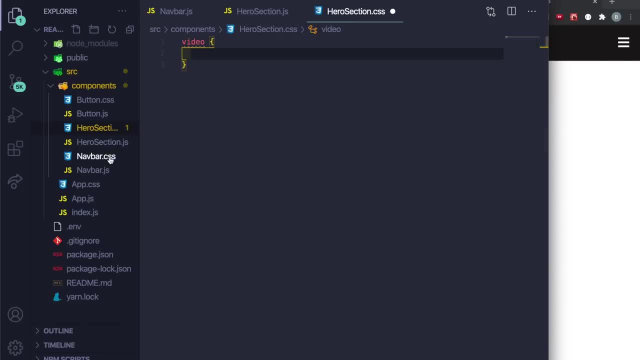 if you want to see the exact css, me explain everything and just typing it out, then that's on my other uh video, but for here let's just go and just type this out. so the object dash fit wants to be cover, and then let's say width. i want to set this to a hundred percent. 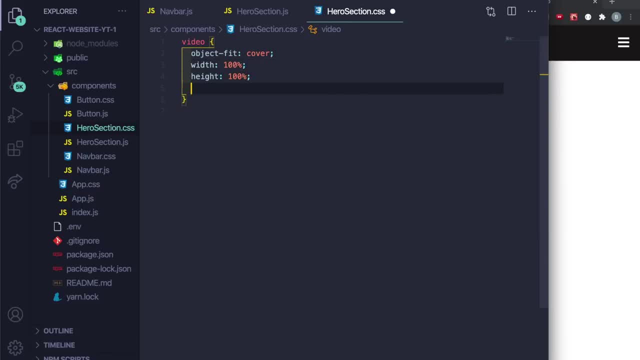 i want to set the height to a hundred percent position, i want it to be fixed so that it essentially stays in a spot, and i want to set the c index to negative one, just so that it ensures covering any of my other stuff. so let's talk to the hero dash container and then in here, so this: 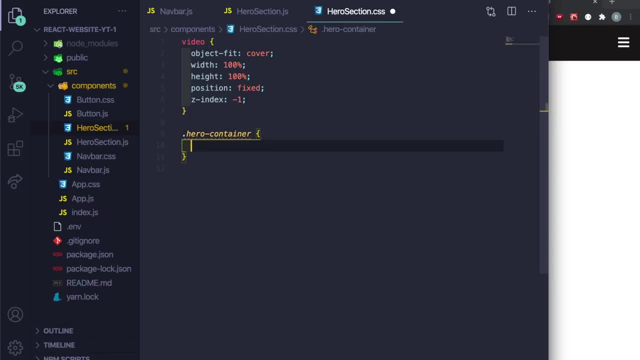 is essentially where you'd put your image if you weren't using a video. this is where, at least, i put it, and i put background url and then you would pass in the images, whatever your folder is, and then the uh picture that you're trying to import, and then i'm going to center it. so this is a. 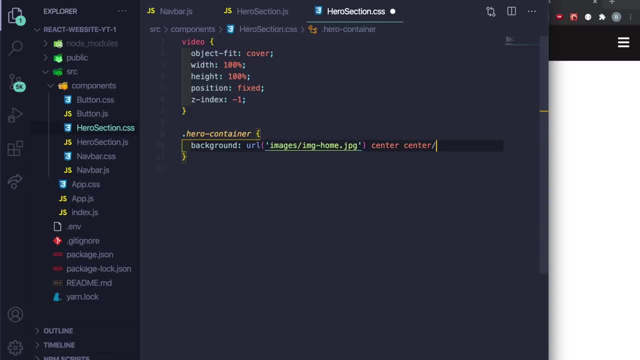 shortcut with background. it's not going to tick it off at the moment. i'm going to check that out a little bit and then i'm going to do another check and look for village to HOV comment- A good one- and essentially having everything, instead of saying like background size, background position, etc. you. 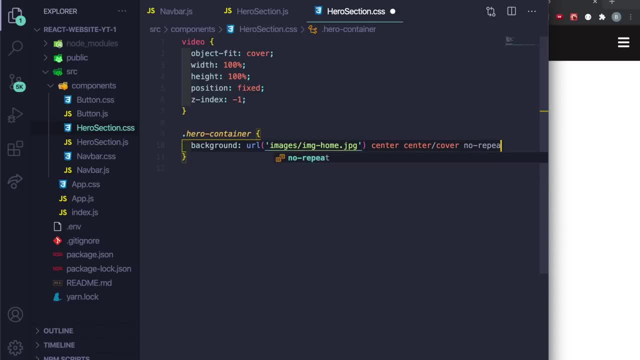 can just do it all on this one line and then repeat, and i save it. nothing's going to show up yet. so i'm going to say: height 100, viewport height, width 100 percent. let's do display flex- not i don't want to separate flex- let's do flex direction column and then align item center. i want the box. 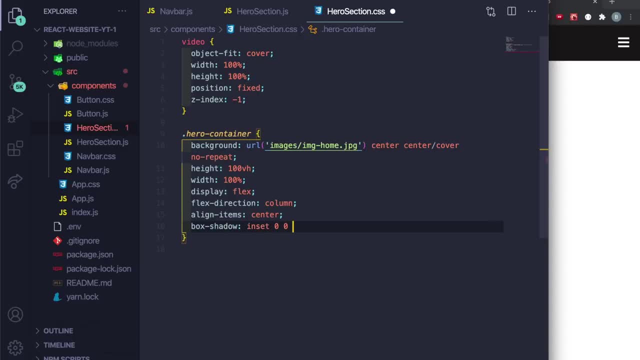 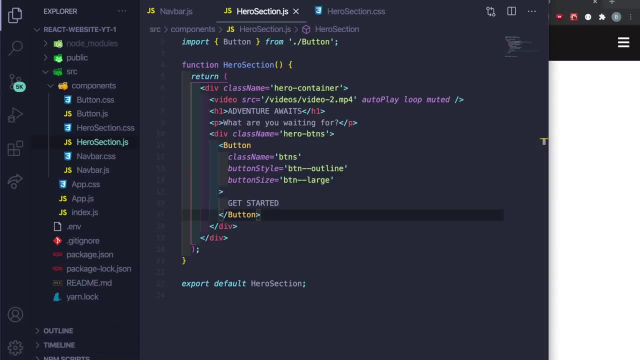 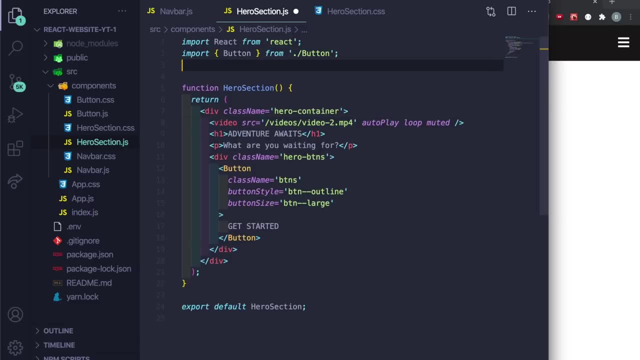 so i should go back to the here set. let's complete everything first and then we can add the actual uh css, so that everything makes sense. and also, i import this too. so let's do import close dot slash, hero section, dot css, and then looks like i need to import also appcss. 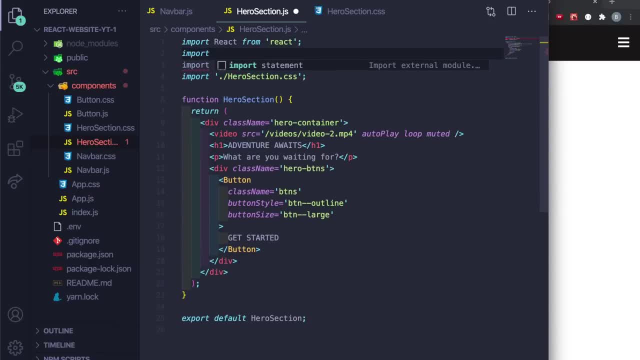 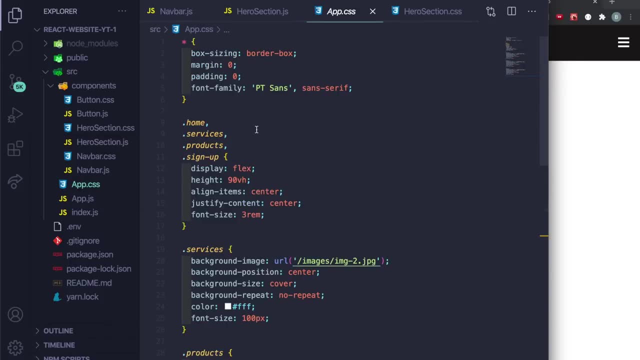 i think, yeah, let's just import this, just to make sure i have all my styles appcss set now. normally you would make uh like a global file and you have everything separate, but since the way i did it, i have these like default things. i just want to. 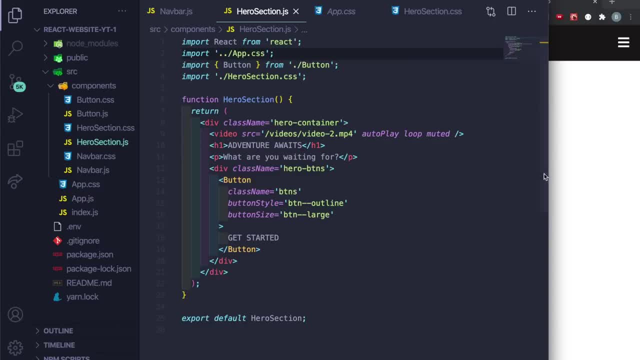 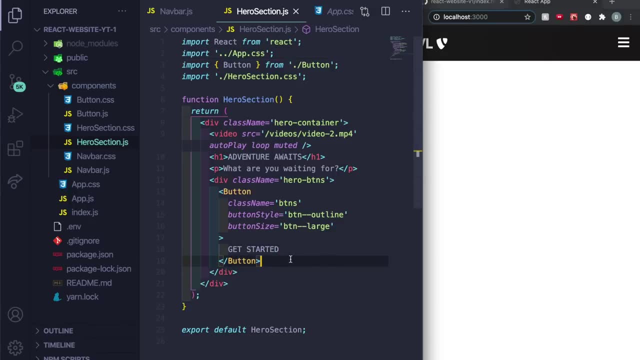 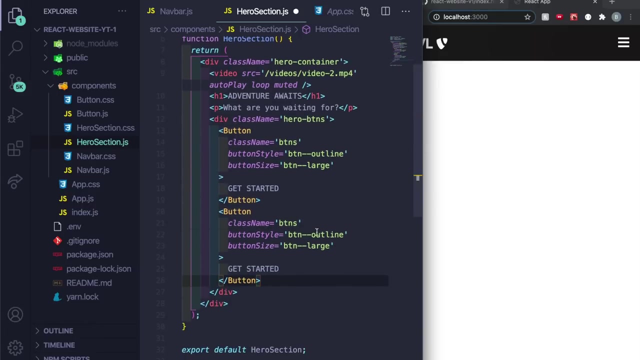 make sure everything's set in there. but, um, again, you can organize your files however you want. right now nothing is showing up yet, so let's go and finish this up. so now let me go and let's go and create. so copy this button, paste it and then let's change the button style to primary. 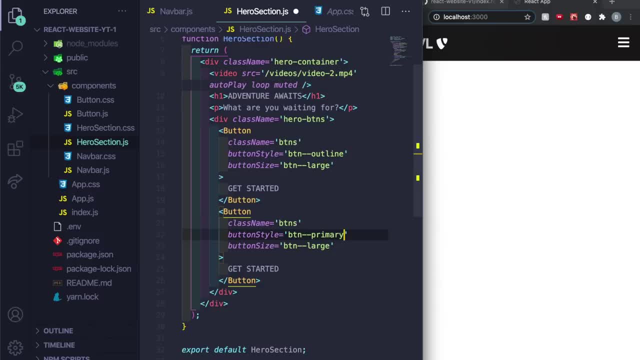 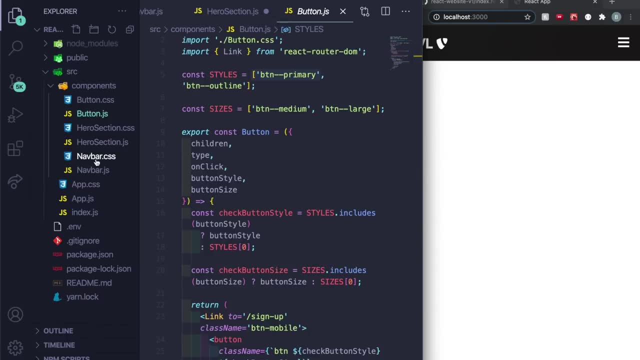 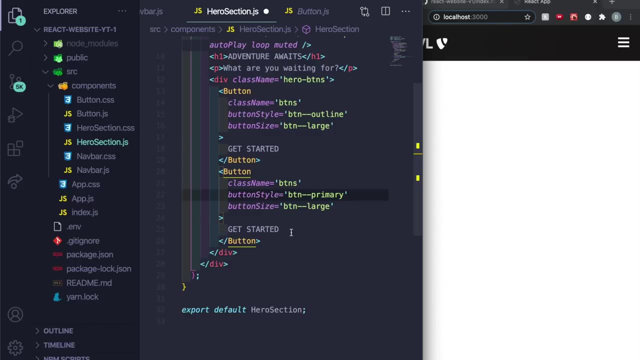 print and then button large. so keep it there. so technically we could leave off that, since it's defaulted to primary, but let's just keep it there, just in case we end up adding additional um css classes. and then let's do underneath this last button actually, yeah, within this button. 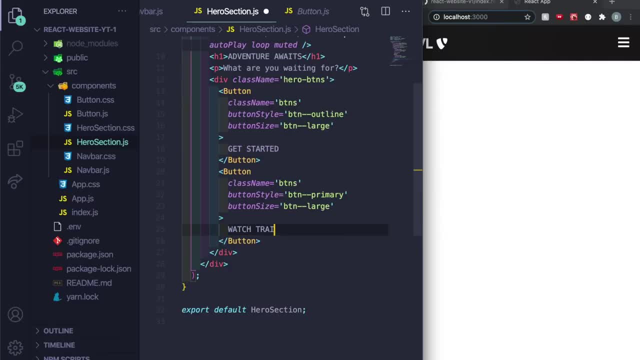 so you get started, let's say watch trailer, and then i'm just add the class, so let's see class. add the class. so let's see class name equals to far fa, dash play, dash circle. and then it's closing tag here. so save this now. right now we're not going to see anything because we haven't created. 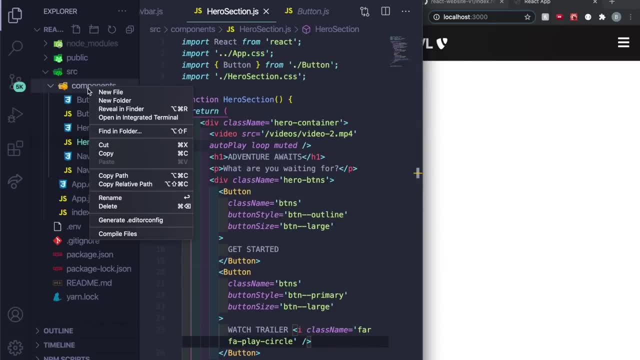 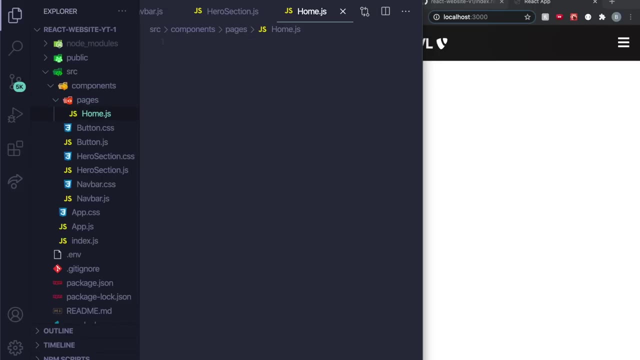 our home page. so let's go and go to components, right click this and then go to new folder and i'm just called this pages, and within the pages i'm going to go new file. i'm going to say home, dot js. now, within here, i'm going to import multiple things. i'm import: 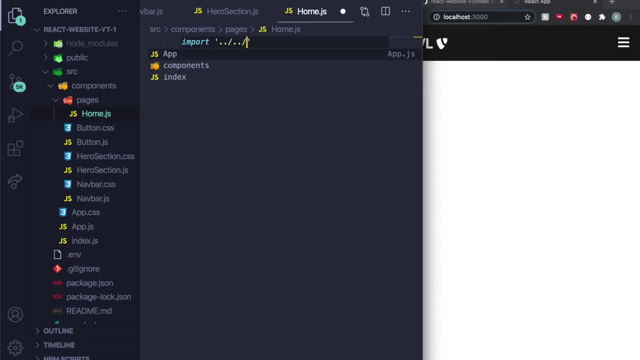 dot dot slash. dot dot slash. app dot css import. we don't have cards yet, so let's just import hero section from dot dot slash hero section and then let's go ahead and just say: function home, and then we're going to return. i should put some fragments here. i'm gonna say: let's import the hero section here and let me save this and 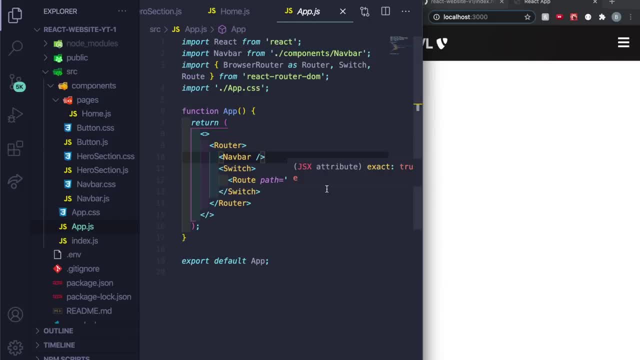 then we need to do is go to appjs and i want this to say: component equals to home. if i save this, i don't know why it's not auto completing for me, but basically we need to import the home component. so i'm just going to go here and just say: import home from coast dot slash. 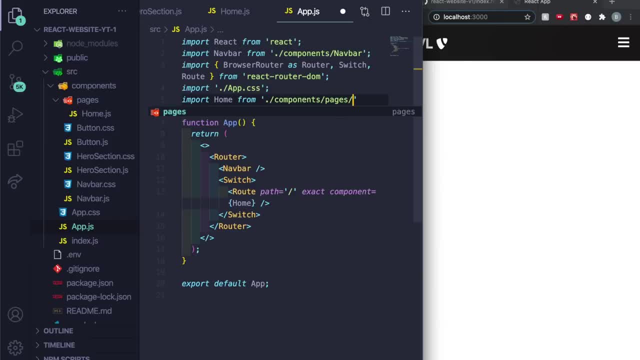 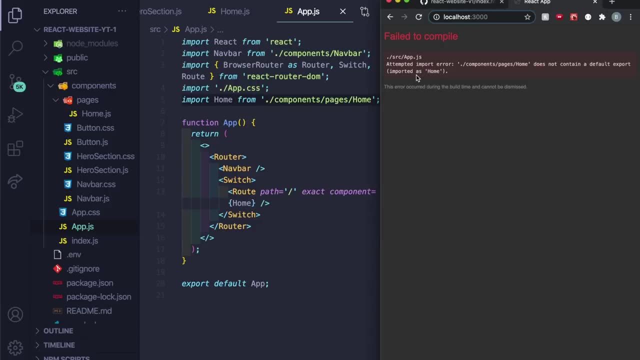 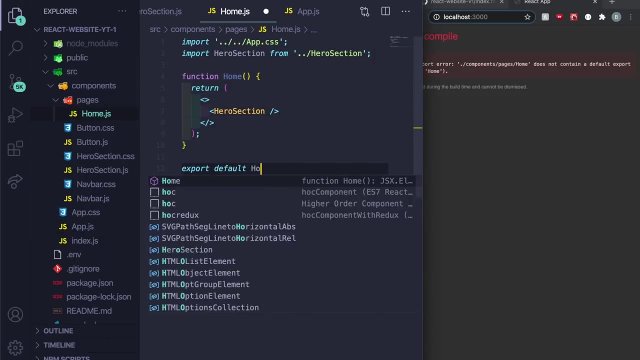 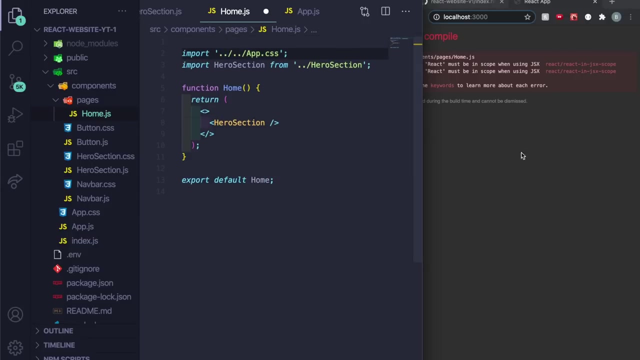 components, slash pages, slash home: save this and it looks like we need to default export on home. so oh yeah, i forgot to put that. so at the bottom: exports default home, save it. and import react from. react is very important when we need, let's just say, imr, enter space or c or c and looks like one. 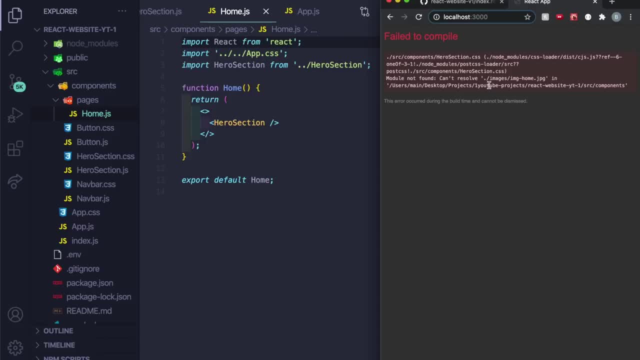 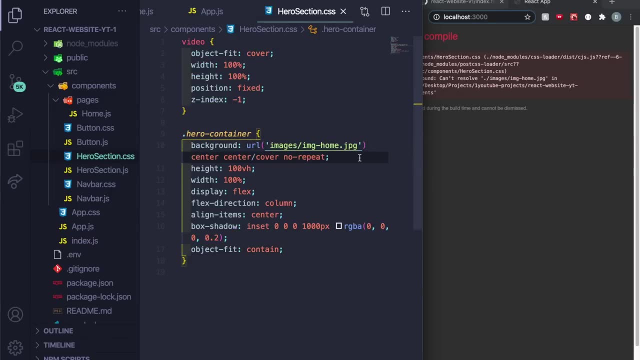 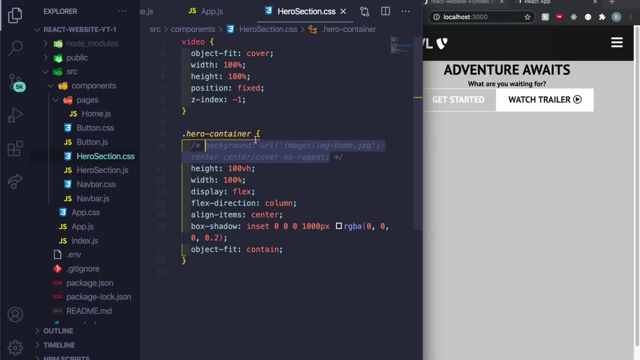 other thing. it's saying that can't find the dot slash, so let's see if that's on the uh hero section css. so since i think, since i have the video right now, it's running into an error. so let's actually comment this out for now and right now, if you save it, the video that we're currently have set in the 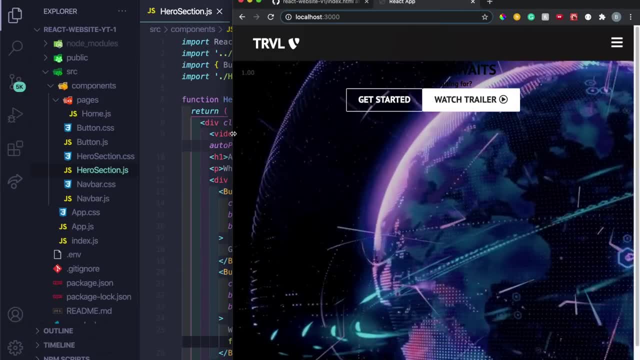 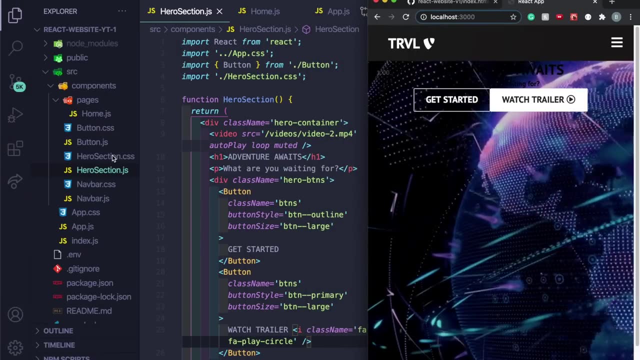 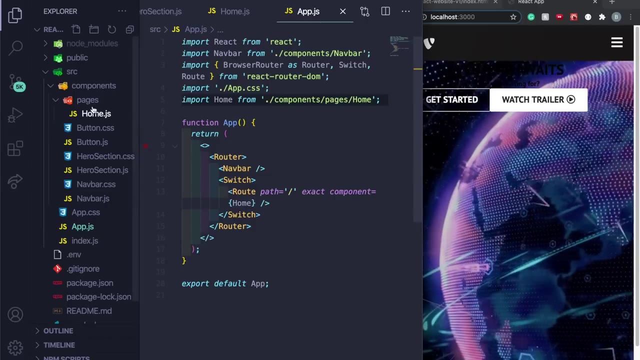 hero, section video 2 is currently playing, and this is currently what it looks like right now. so nothing crazy, but we're getting somewhere. so all we need to do now is actually just fix the css style here. also, you're wondering what we do earlier. so basically, just to recap, we created the 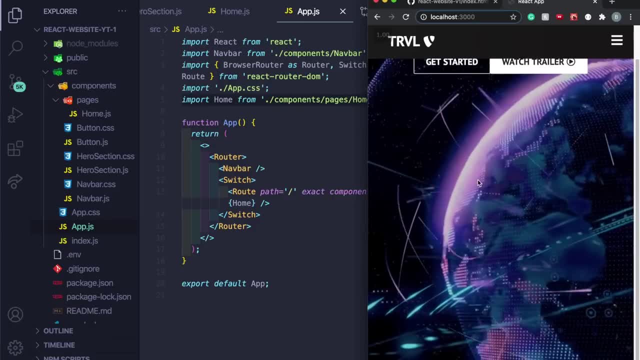 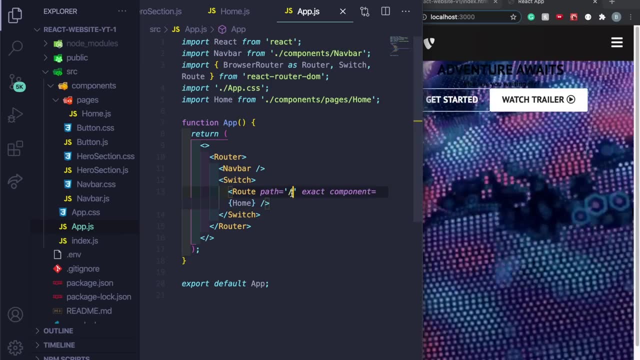 pages. so this is just a quick recap of what we're doing here. so we created the pages. so this is just a home page. so right now everything you see on this front of this site is i put that as a home and then i went to the appjs and passed in the slash pass. so basically the every time you go to 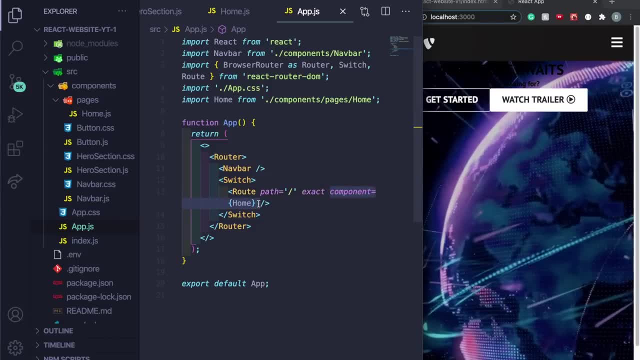 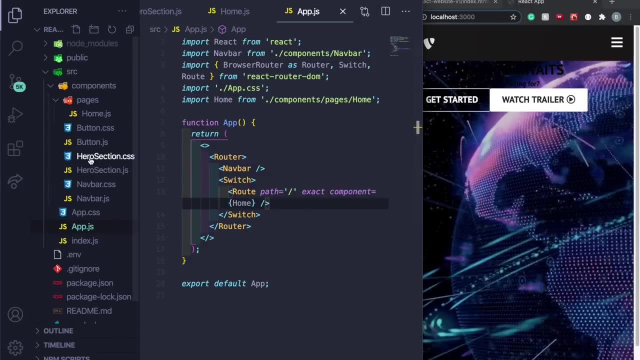 slash essentially is going to open up the home component, which basically is the front page, and that's why we have this right here, and then we'll create more routes. you'll see it makes more sense. but um, let's go back to the hero, second css, and let's finish up this so that it makes more sense. 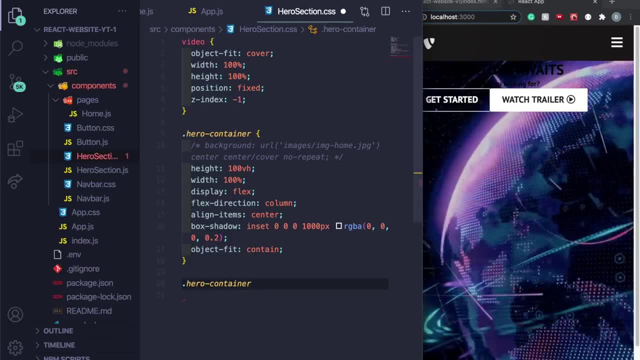 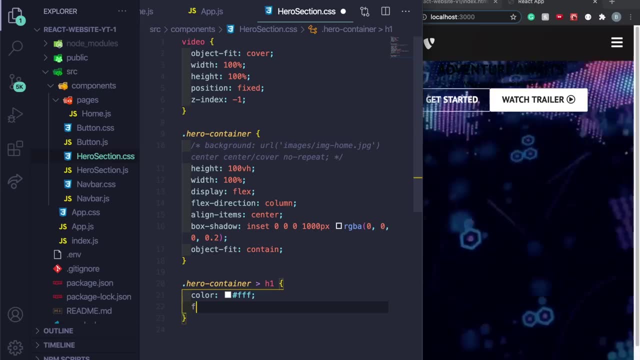 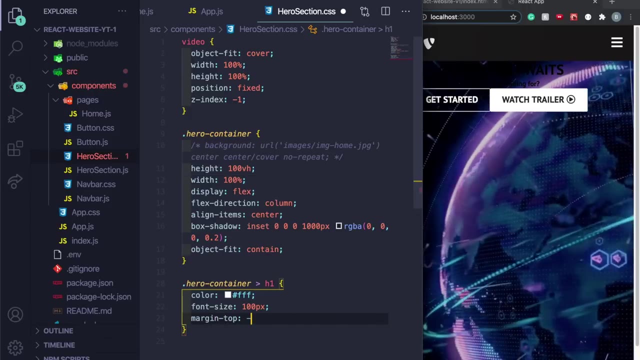 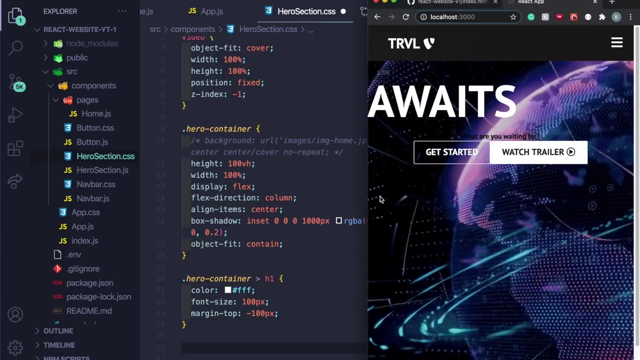 so now let's do this. so we're doing this right here. we're going to say static dot hero container and then it basically is going to target the h1 inside of it, set the color to white, font size to 100 pixels, margin dash top to be negative 100 pixels. so i saved that there. and then let's go, and right now. 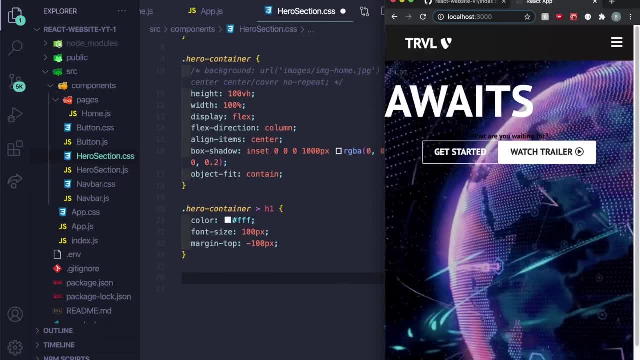 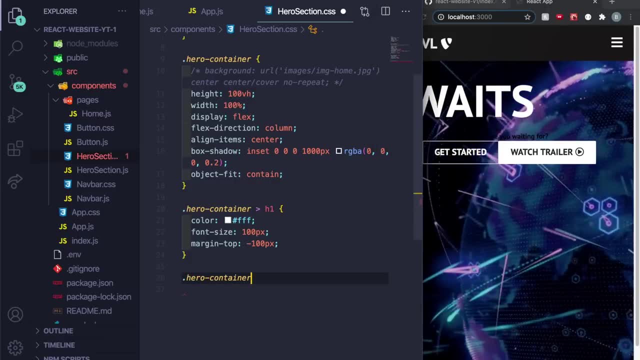 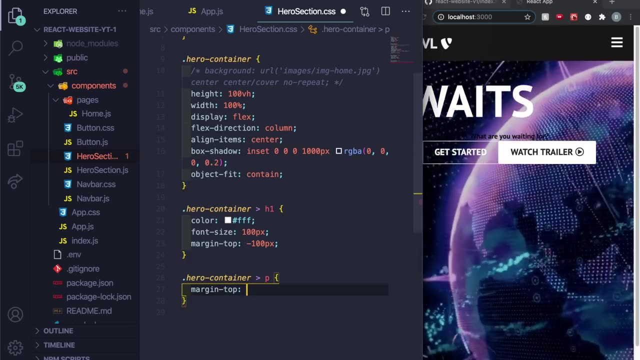 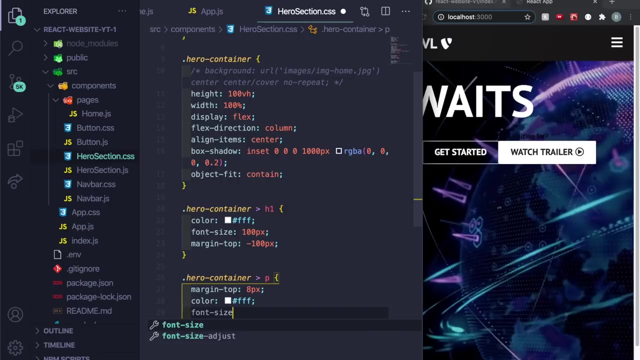 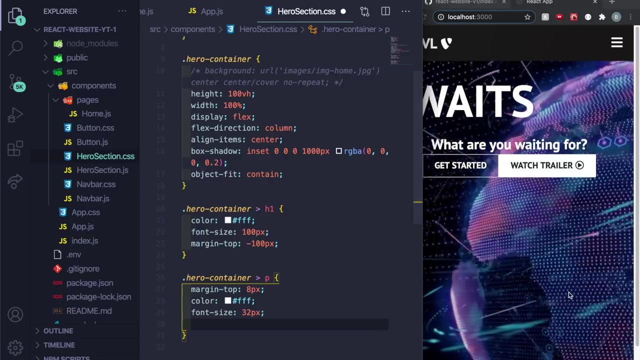 it's not um, it's currently it, as it looks really crazy. but let's go ahead and add the dot hero container. going for the P tag. now I want to say margin dash top: 8 pixels, color to be white, font size to be 32 pixels, and then let's do a font family. so this is a. 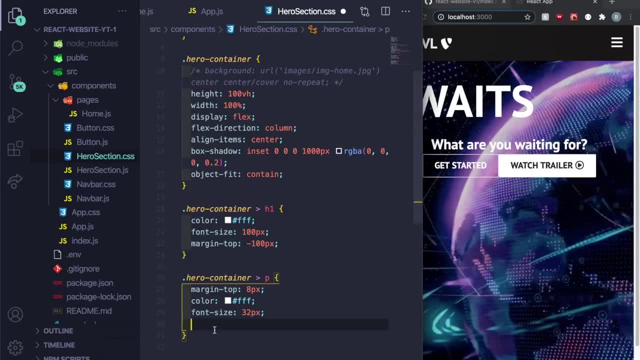 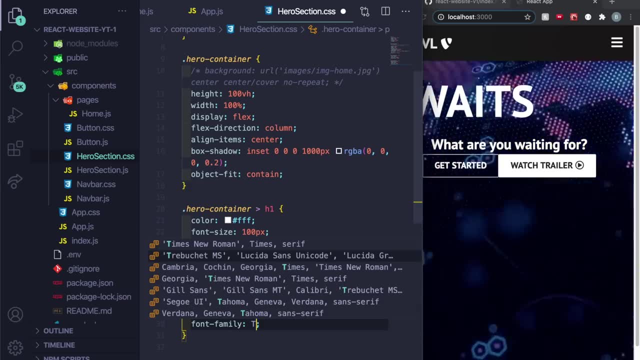 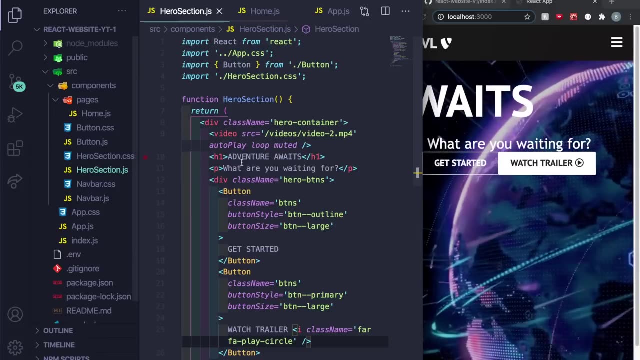 I see if I can type it out for you. font family and that's huge T. I just put it to trip Boucher. I can't pronounce that and that's the default one, so you can just do that there and let's let that misspell something. h1. all right, let's go. 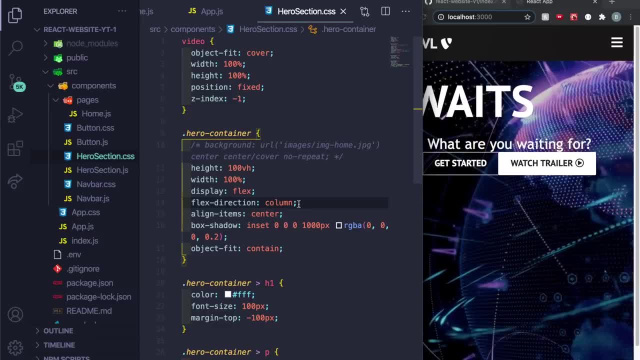 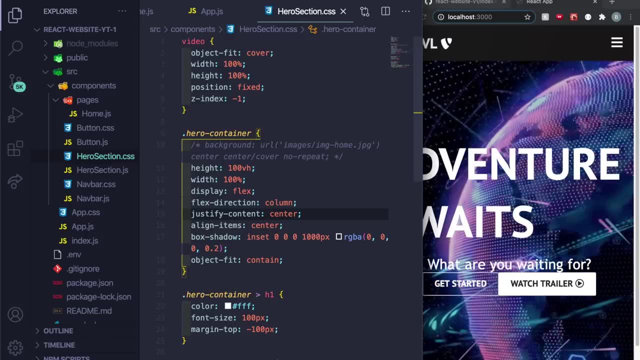 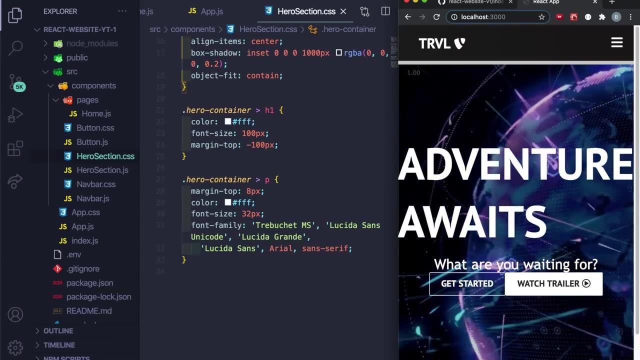 back to: yeah, let's go here. oh yeah, one thing is, let's add inside of the hero container, let's do just like content Center, and it looks like: yeah, it looks much, much, much better now, alright. so now, if I scroll it out, it's like this: so now I just need to finish up some more. it's. 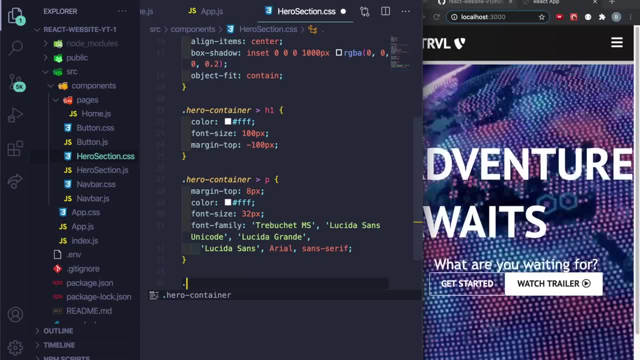 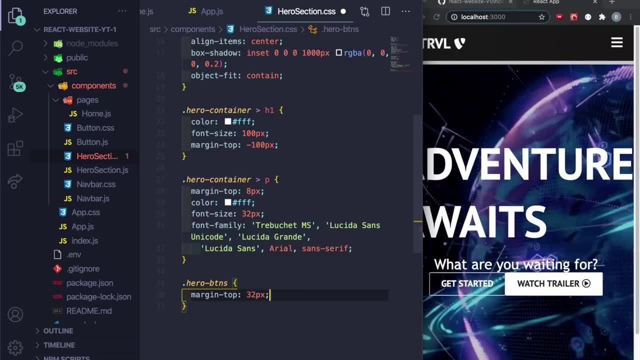 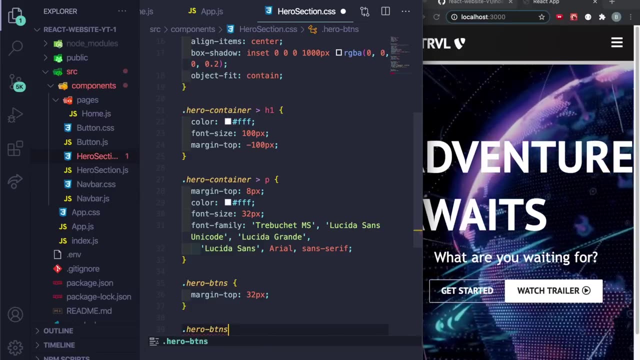 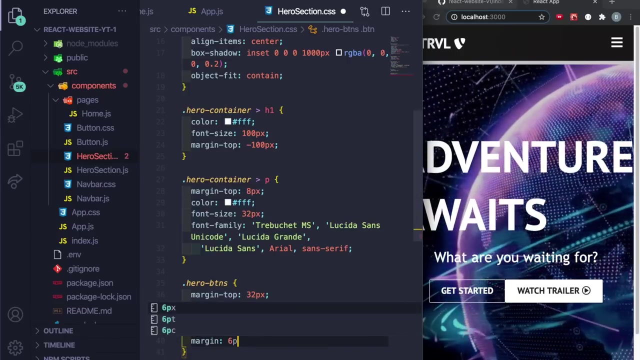 all more almost on this part. let's do dot hero, dash, BTN, and there's gonna say margin, dash, top to be 32 pixels. save it. so out of this one I can do dot hero dash and then dot BTN and I just say margin six pixels, slow spacing in between them. 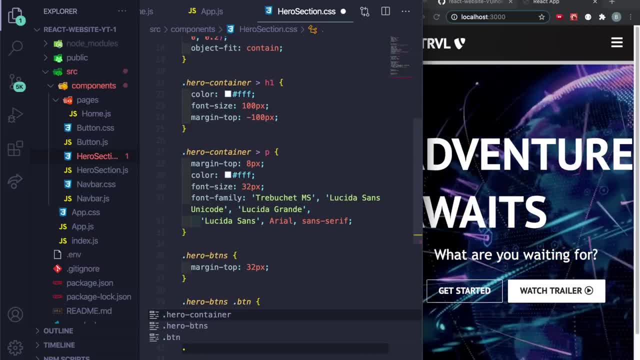 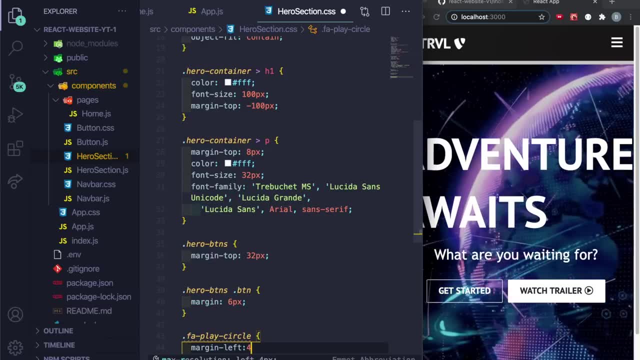 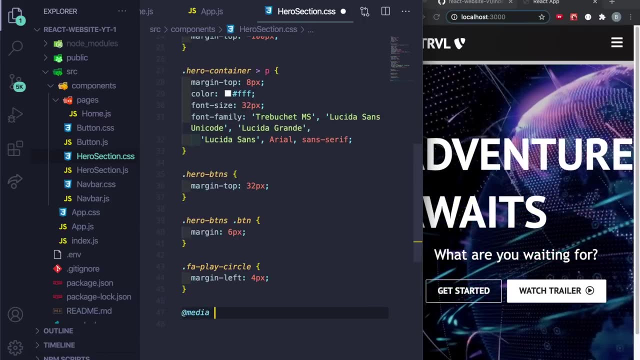 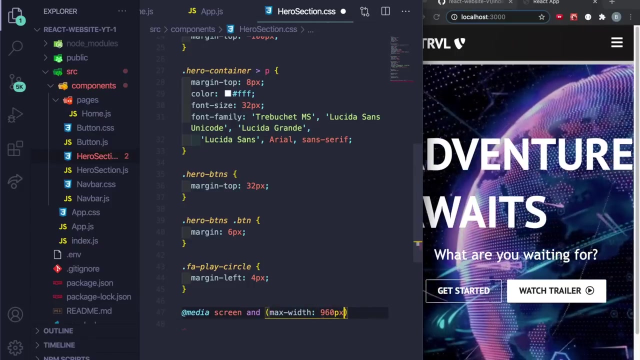 right there. and then let's just target the little icons of FA, dash play, dash circle, and let's just set that equal to margin dash left of four pixels. so now I'm gonna say at media screen and max width of 960 pixels, and then I'm just gonna target the h1s. let me just go. 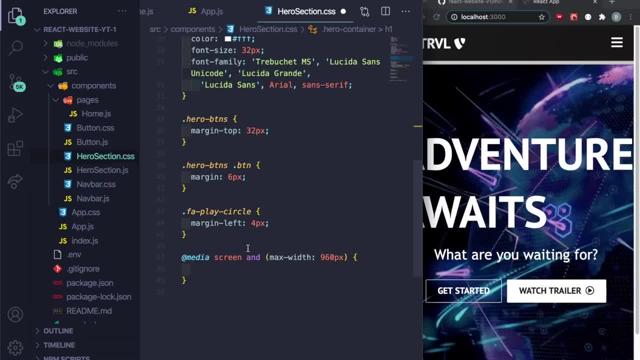 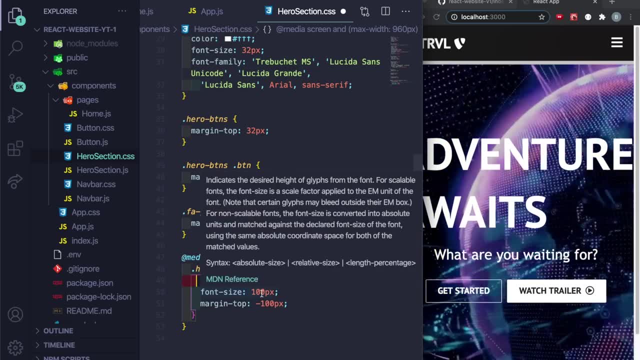 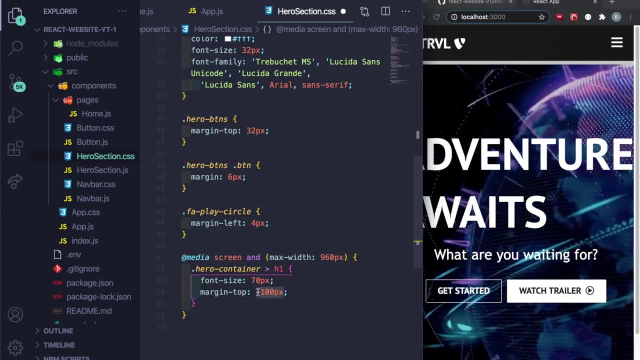 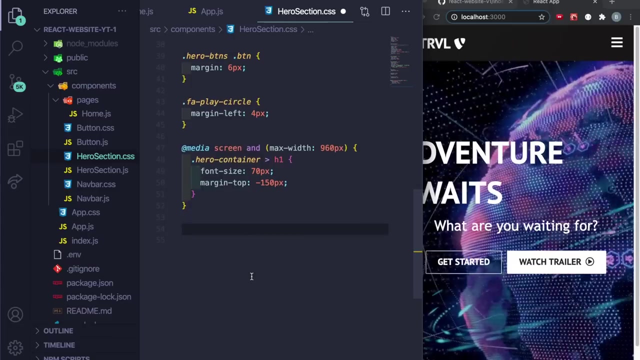 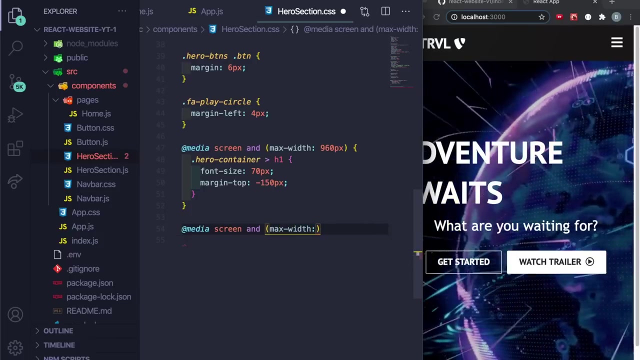 over here. copy this to save time. and then I just want to change the. take it. rid of this color. okay, because it already passes in by default. and then we'll say font size to be 70 pixels and then margin to be 150, and then underneath this let's do at media screen and max width to be 768. 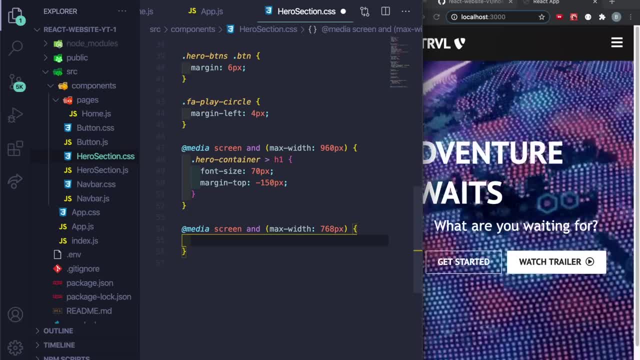 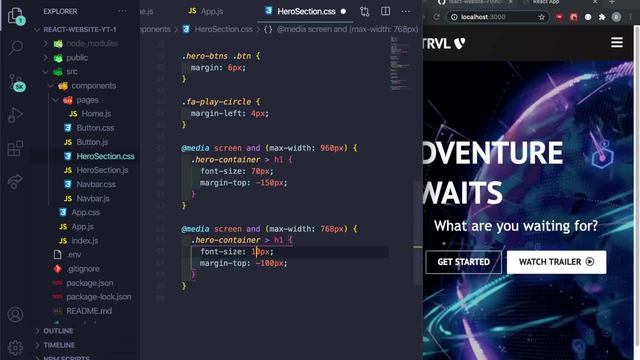 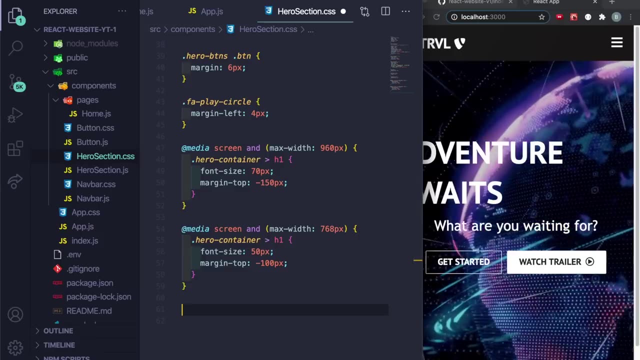 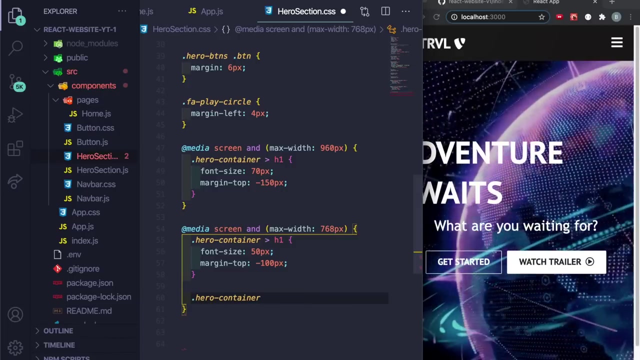 pixels. and then let's just say, copy it again, and I want to change the font size to 50 pixels, and then Martin, top 100. that looks good to me, and then I'm gonna select the printображ graph scrolling to the blue circle. back pee now. 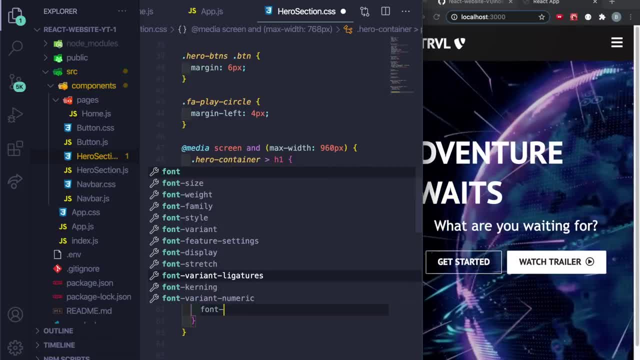 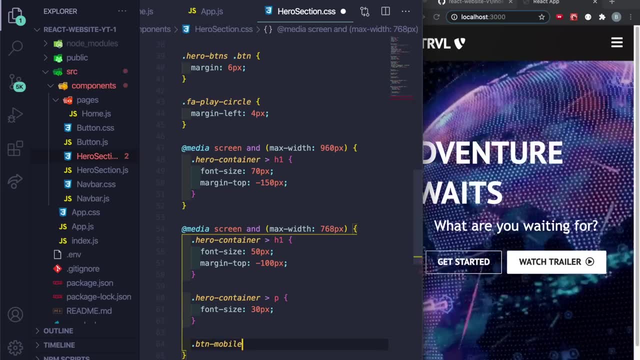 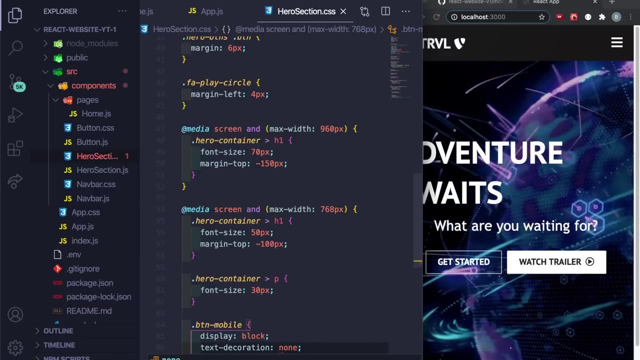 everything. yeah, so everything would be in this midi create. so underneath that, but still in the brackets, we'll do about hero container, the P tag. underneath that will say font size: 30 pixels, and then let's do the BTN dash mobile display block and then the text decoration: none. 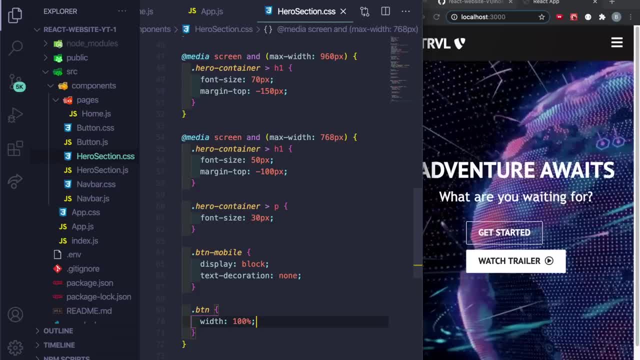 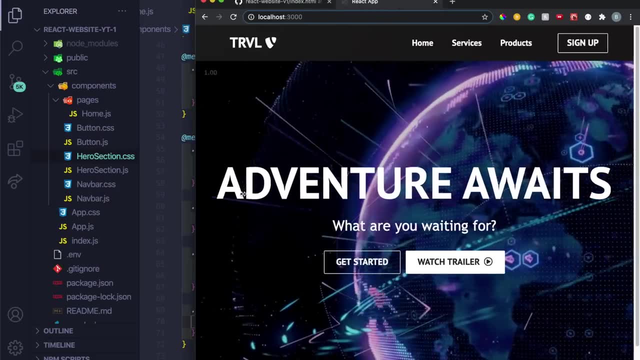 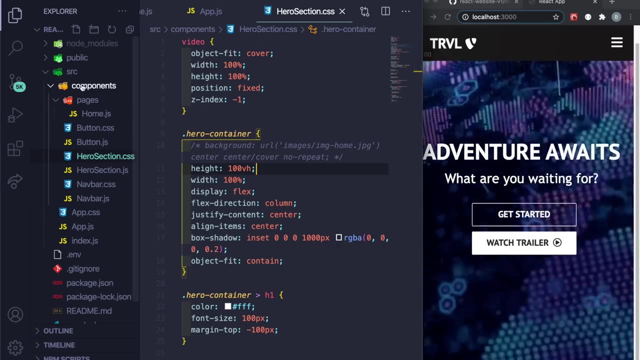 width to be a hundred percent. so now you can see, here we go. so pretty much we're set there and this is what it currently looks like. so now let's create the next section, which was the card components. so I'm gonna go here to components and 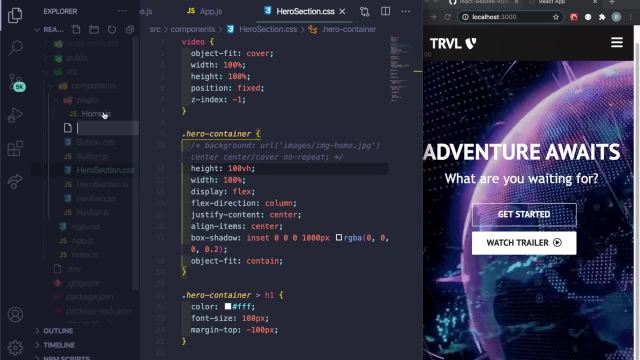 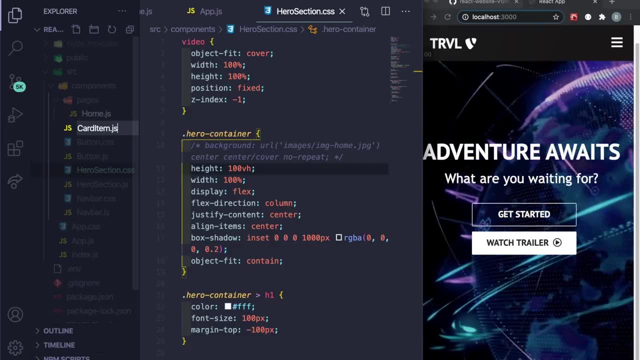 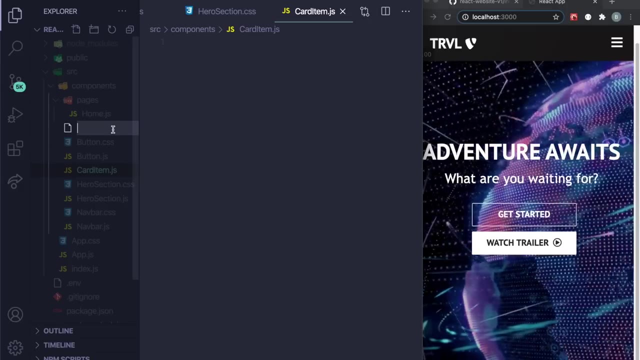 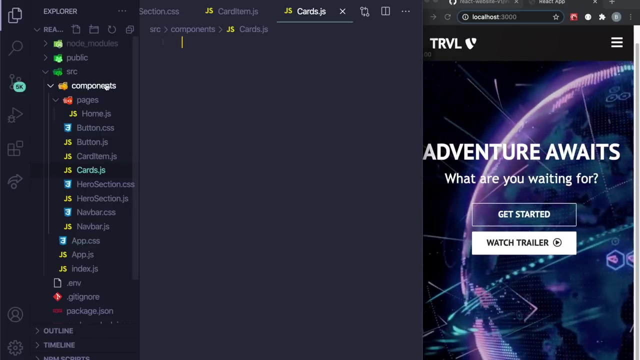 basically I'm gonna right click and chain click on new file and I'm a type in card item, so these are the individual cards that I created here, and then I'm gonna create a cards component so that's gonna hold all the cards. so basically say cards, dot, J, s, and again you name this however you like, and then 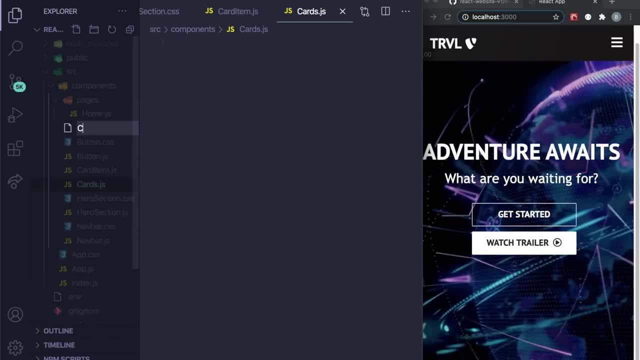 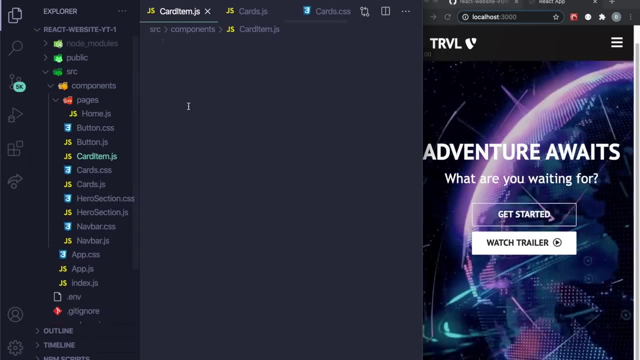 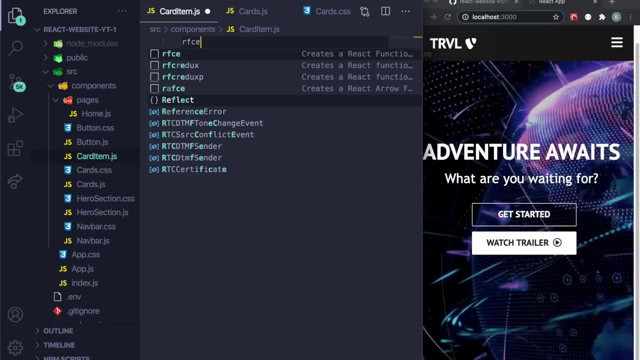 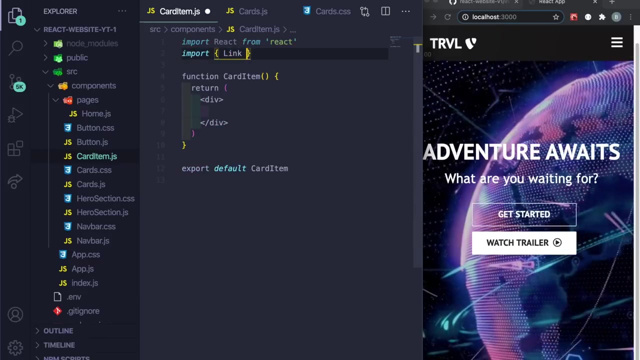 let's create the car does ESS or cards dot CSS, and I'm gonna keep all the CSS within this one, but they're also gonna cover basically the car item too. so for the court item, let's go ahead and do or F, C, E, and then, above this, let's imports link from react router Dom. so now I'm 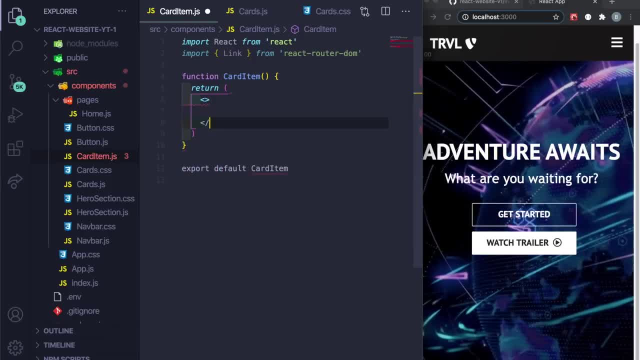 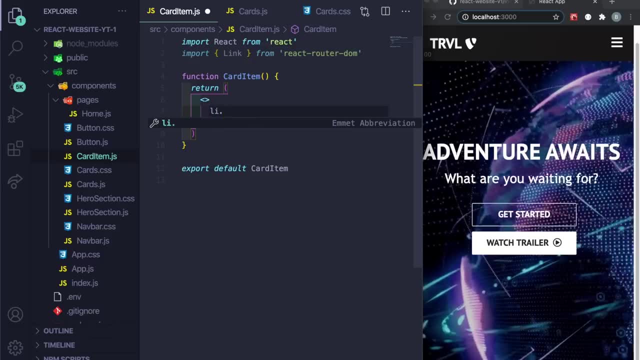 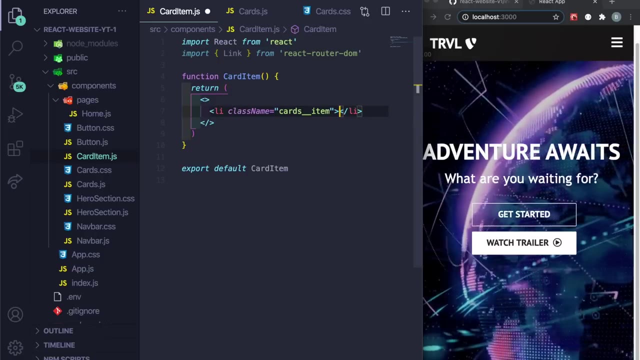 gonna go ahead and just take these, turn them into fragments and then I'm gonna say Li and my put: I'm gonna utilize a different styling for class names, just for this, just just to make a little different. but, um, usually double underscores of BEM styling and they will say class name cards. 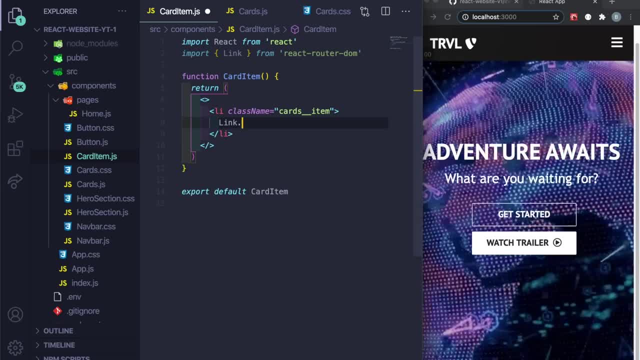 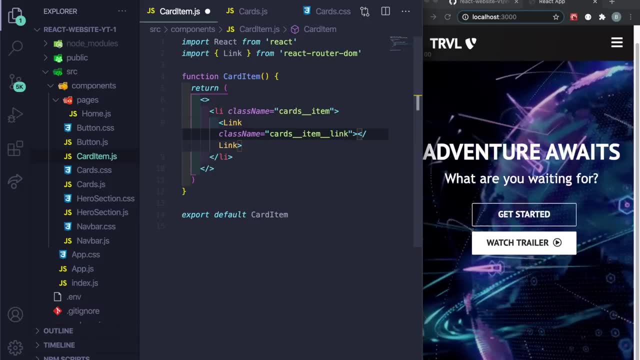 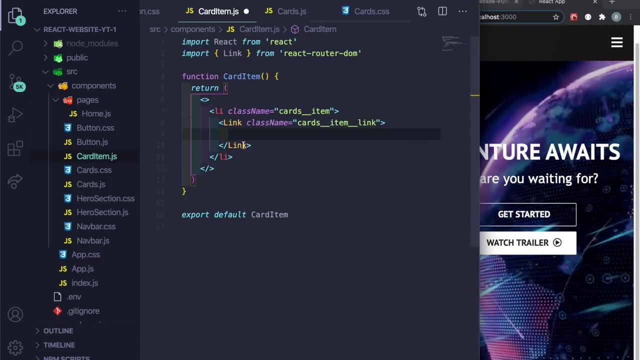 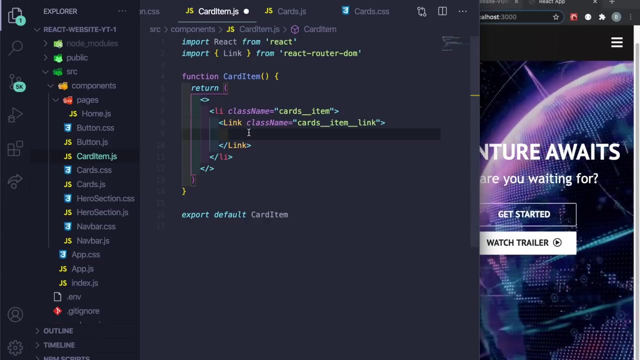 underscore item. it's a link that card underscore underscore items, underscore underscore link tab in there and then within the actual week tag. so let's go ahead and drag this out. I'm gonna pass in. this is basically the image and the description. so when its rabbit with 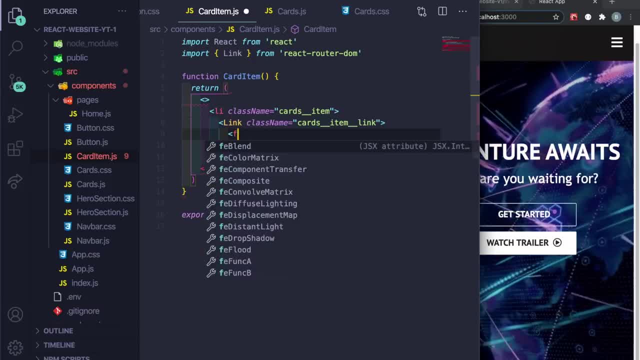 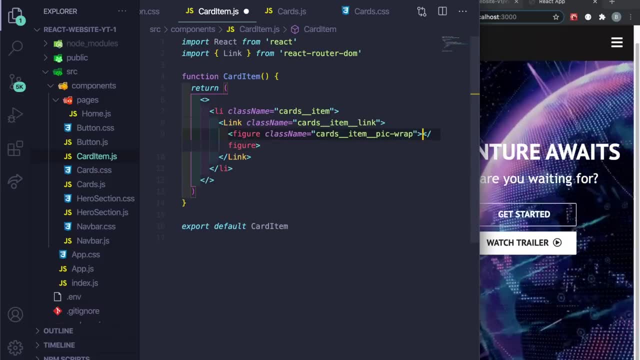 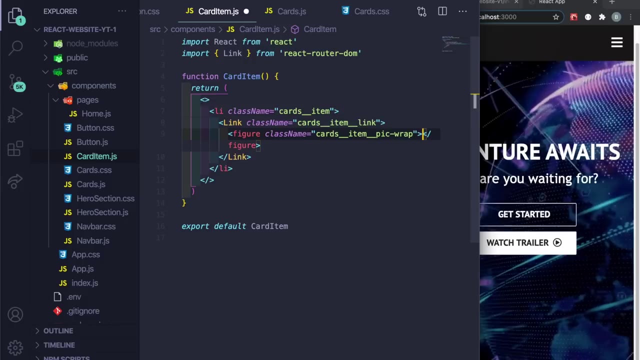 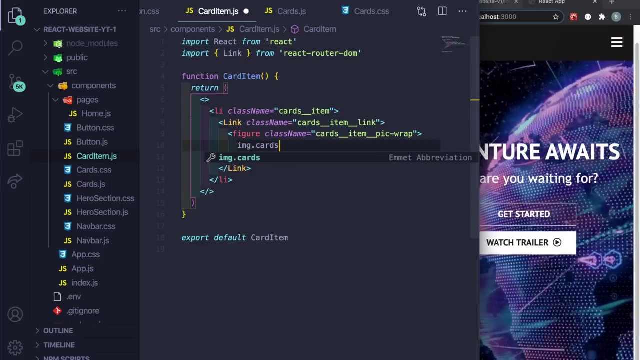 figure. actually let me do figure dot: cards: item pick wrap, so press tab. so we have the class name card on and pick a wrap, and then this is going to have a data category which we'll add all that stuff later. but, um, here we have image and it's going to have the class of cards underscore. 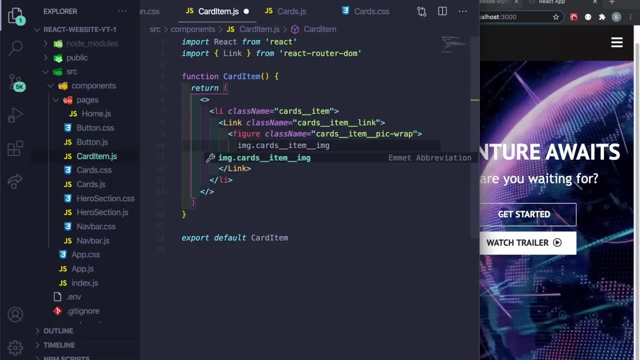 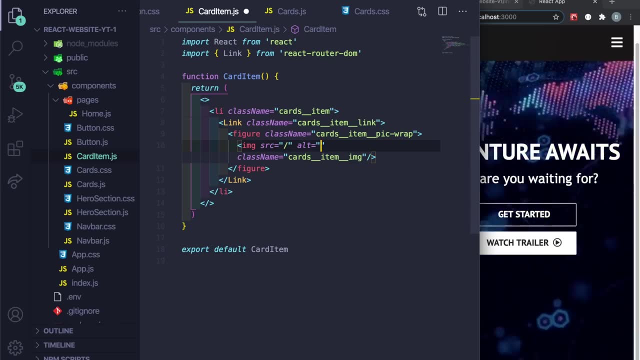 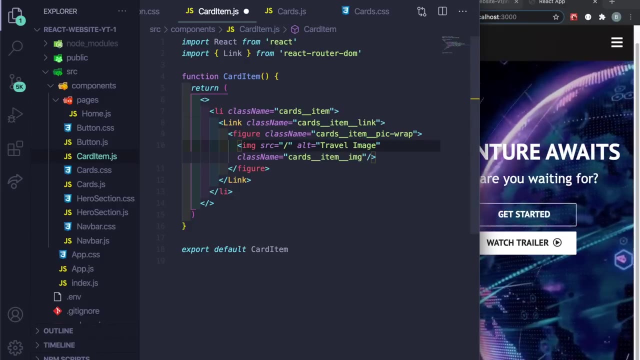 underscore item. underscore- underscore image: press tab. here the src. we will actually update that in a second, but here i'm just going to say travel image. now we could also pass in the alts and props, but for this, for this tour, i'll just show you this way, just because it's much easier and 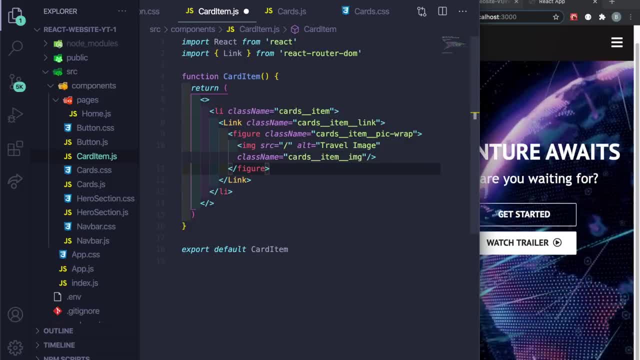 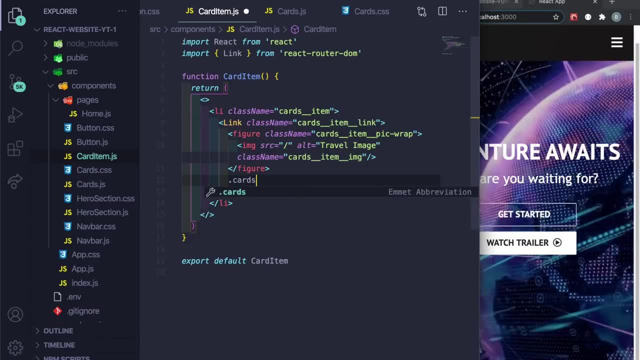 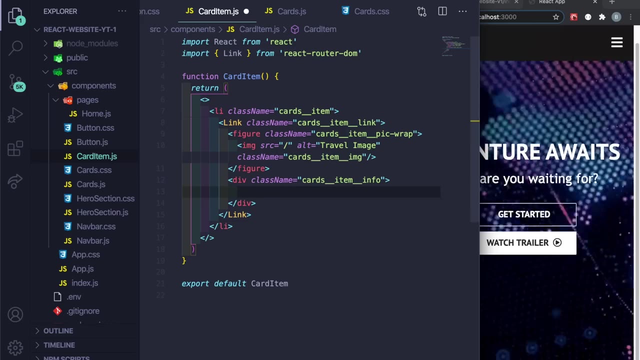 it gets the point across too. but let's go and, outside the figure, press enter now. and then we're going to say credit div for cards info. let's say dot cards- underscore, underscore, item underscore, underscore- info press tab. and then we're going to do it again for the h5 this time. so h5- dot cards- underscore, underscore. 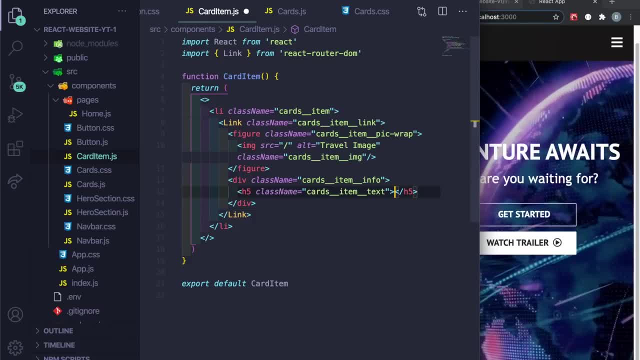 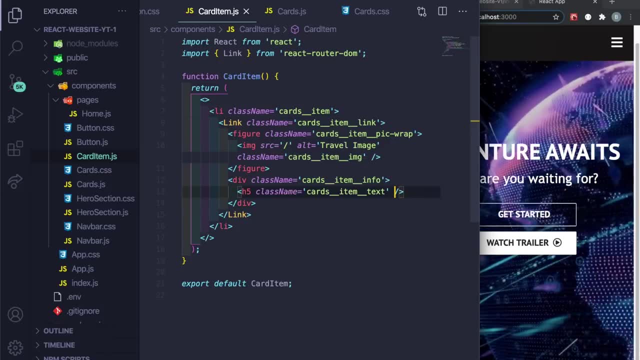 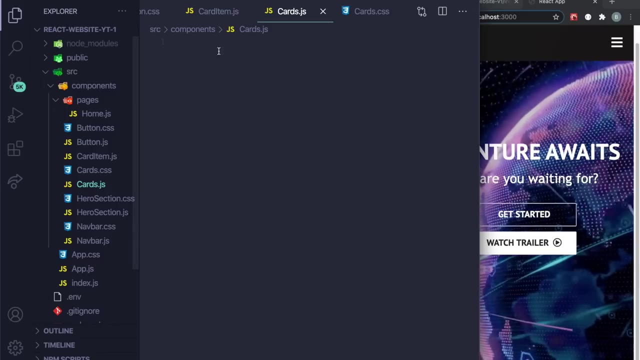 item: underscore. underscore text: now, right now, if i save this, nothing's going to really happen because there's no card data that we're passing in. so now i need to go to cards now and make sure i default: yeah, have everything exported and go to cards, and i'll make sure you so this. 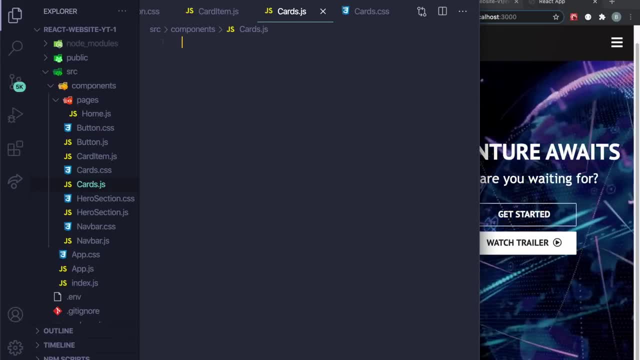 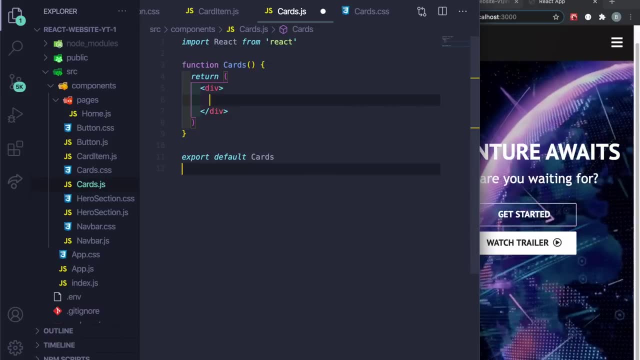 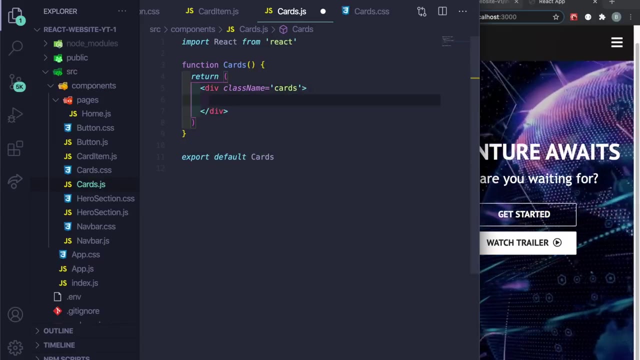 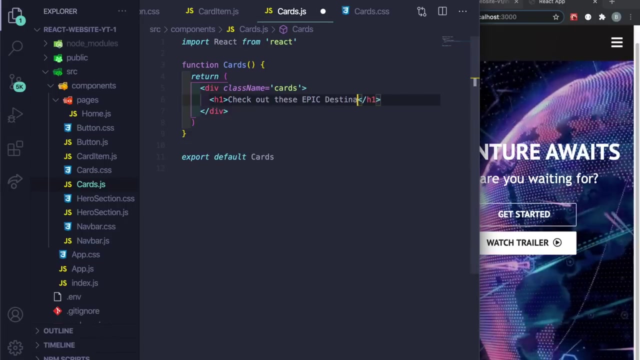 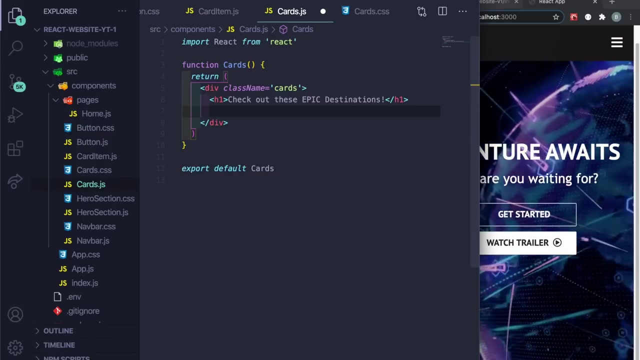 makes more sense. so basically, let's do the rfce and then, pretty much, here we're going to have the div with the class name equal to cards and that h1. i'm going to just say: check out these epic destinations. now we're going to have the cards container now. so this is essentially. 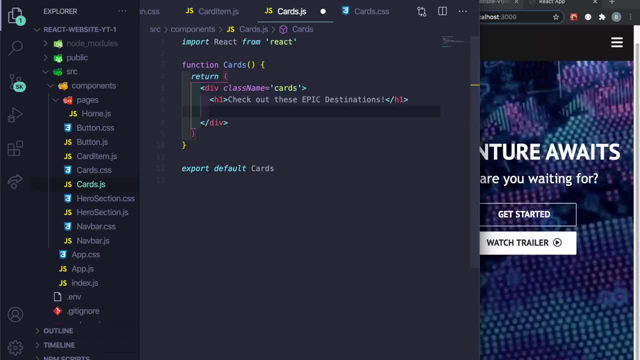 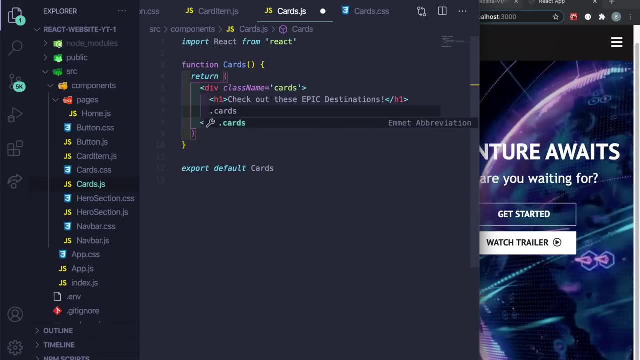 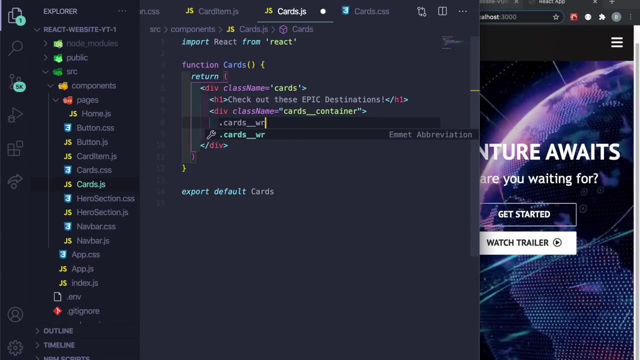 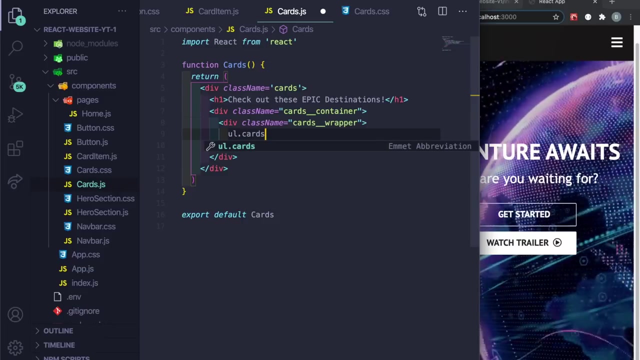 wrapping all of the allies with the ul and also cards wrapper container, which we'll see. just saying so we're going to say dot cards, underscore, underscore container, press enter. then we'll say: dot cards, underscore, underscore wrapper, press tab there. and then we'll have two excavations. okay, the item segment that i think we just made, that's the one that. 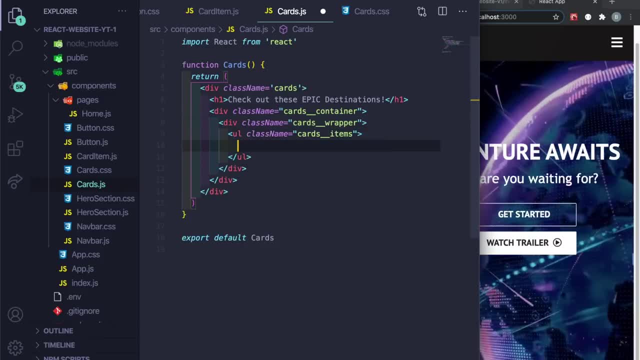 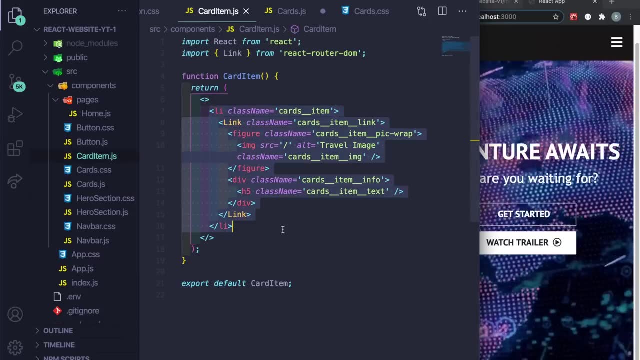 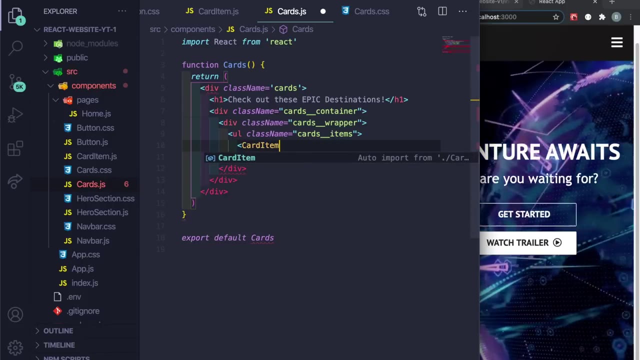 i wanted to add: now Это W-L-I-T And we read this one thing. we're going, You're in to your website, we read this, and then we're going to have the ul dots, And then we're going to have the ul dots cards underscore items. so now, inside of this is where we will pass in the actual 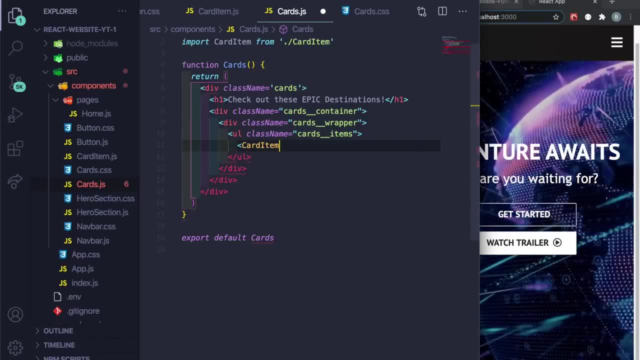 Li a kayak, the card component we just created right here, So that's the way i did it. i'm sure there's different ways to do it by basically you wanna say card item, so that's the name that component just created, or I press enter so it imports this now here. 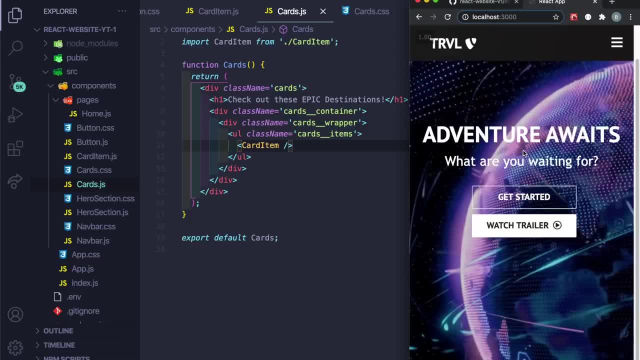 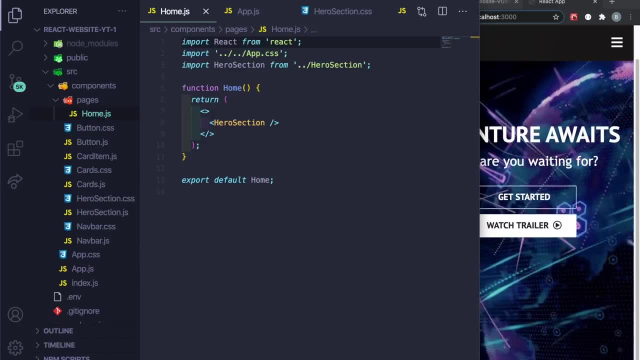 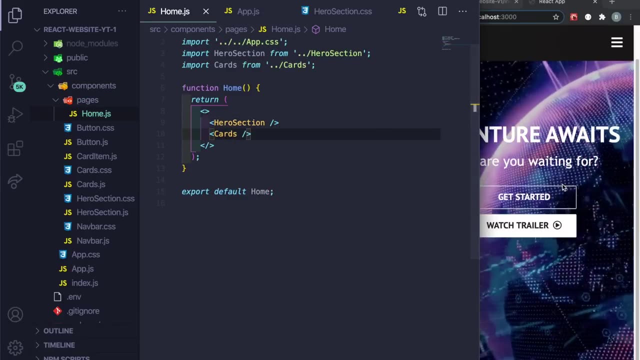 nothing's going to show up, but you can see. also we do need to uh, add this cardsjs to home, so you can see it. so i'm going to go here and basically add under the hero section cards and i'll save this. and now i save it right now. you can see, we have these. check out these epic destinations, so let 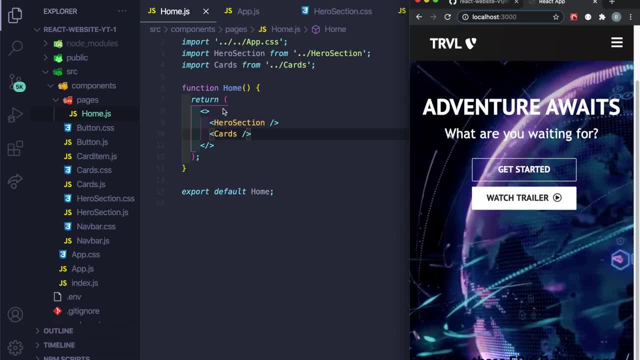 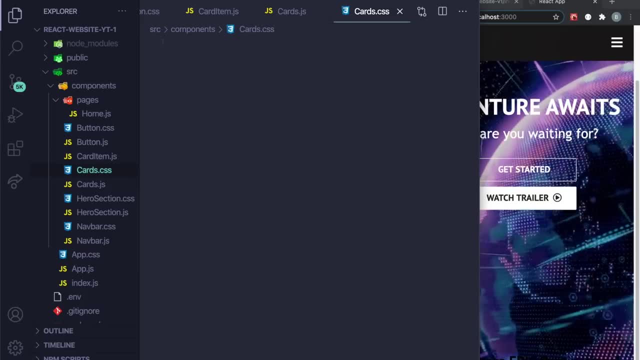 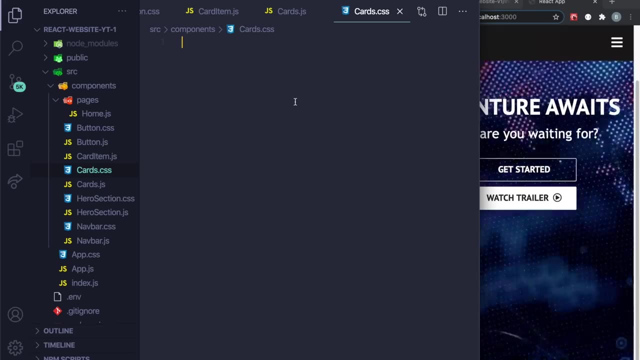 me actually: um, let's add the css, because right now you can't see anything, so let's go ahead and add the css really quick. now there's actually a ton of um, yeah, i don't want to actually go in and have to type in every single thing, so i'm just going to go and copy the css from the github. 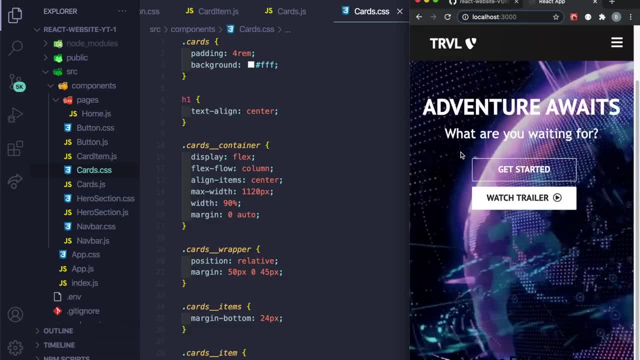 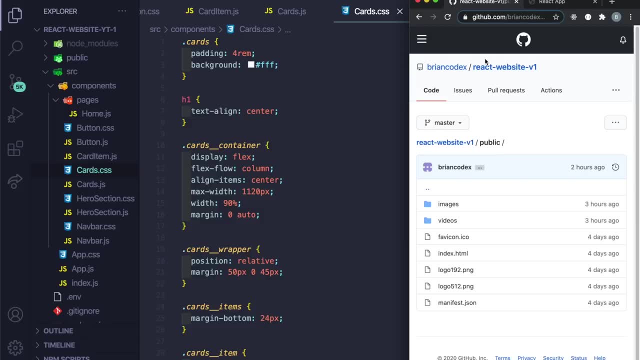 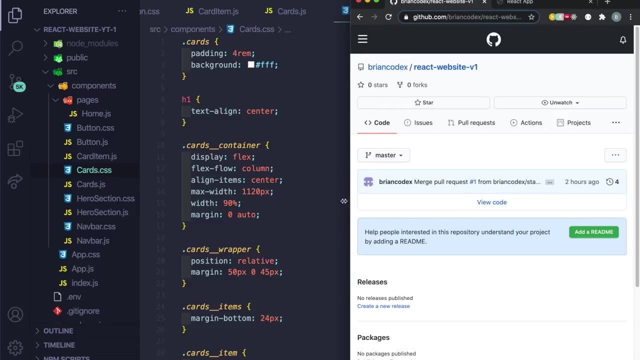 and then just save it and then basically you can see here let's actually add this to. so go ahead, go back to the um, the github, let's see right here, react, we're on the master branch again and then pretty much let me pull this out. src components. 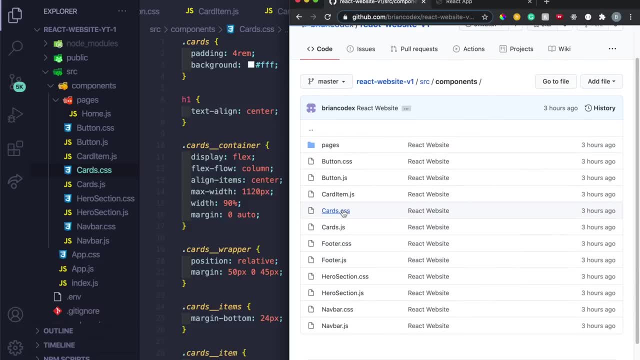 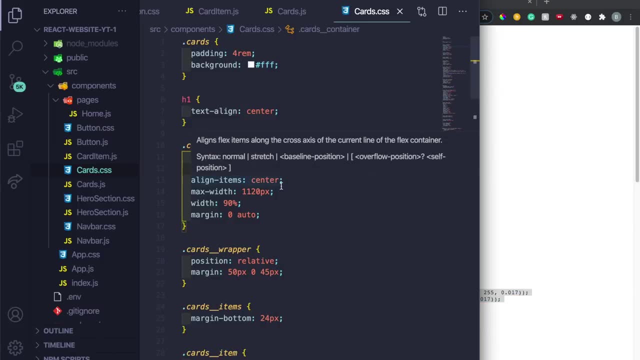 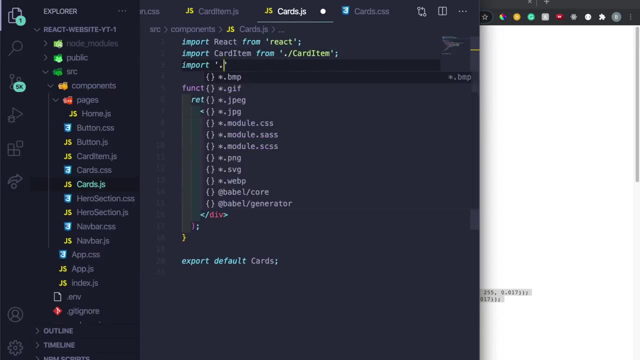 and then go to the cardscss, click on raw command, a command c, and then paste it into car the css, and then now let's go. i think i need to import this here, so let's do import dot slash cards, dot css. let's save this. let's see our app looks now all right, so it looks much. 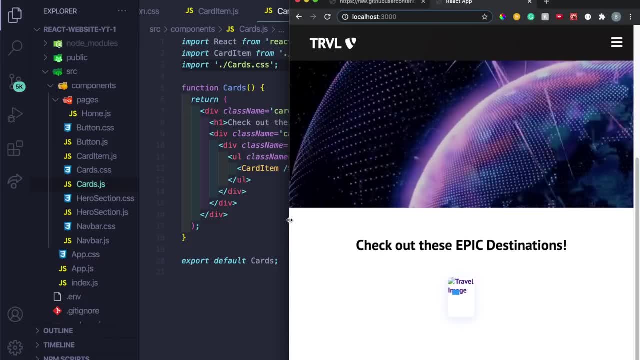 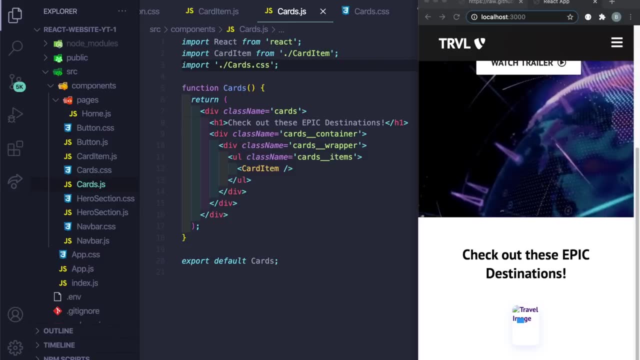 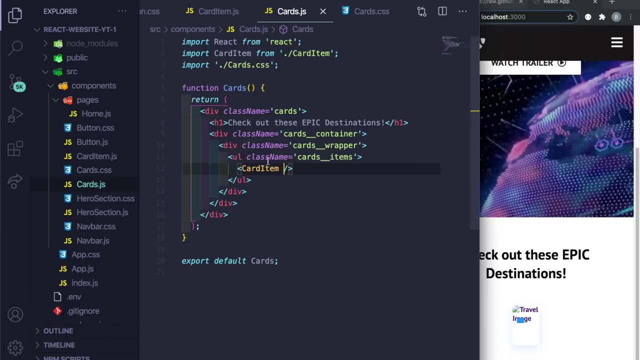 better. so now it looks like we need to add in some properties so that our actual card shows up. so what we're going to do is actually pass in some props, and they're going to do this first by setting the values on the cards component, and then we're going to pass props from the actual we're. 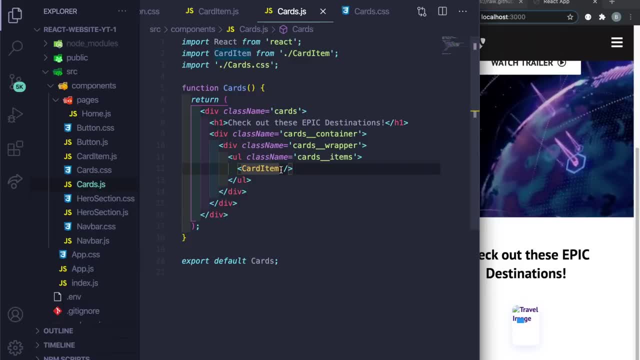 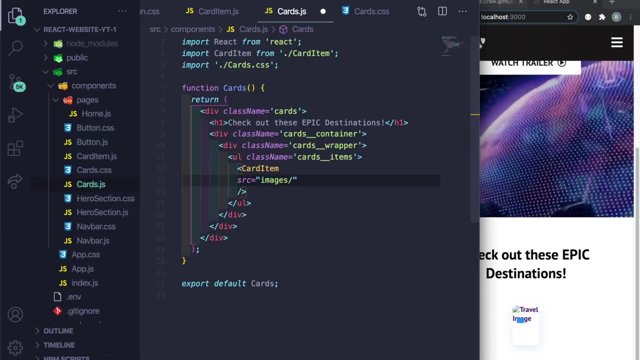 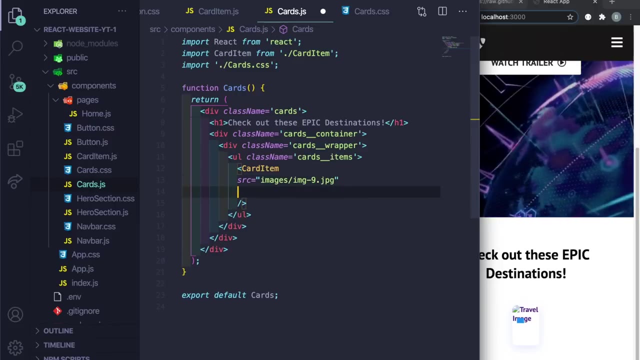 going to pass it in on the cards item. so basically here what i'm going to do is we're going to set the current image link and we're just going to say images slash, let's just put img-9.jpg and then let's do text equals to explore the hidden water fall deep inside the amazon. 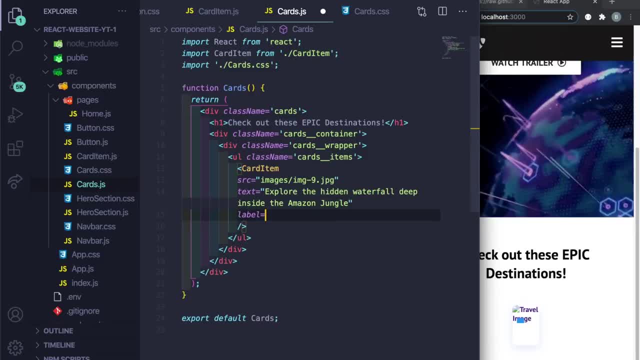 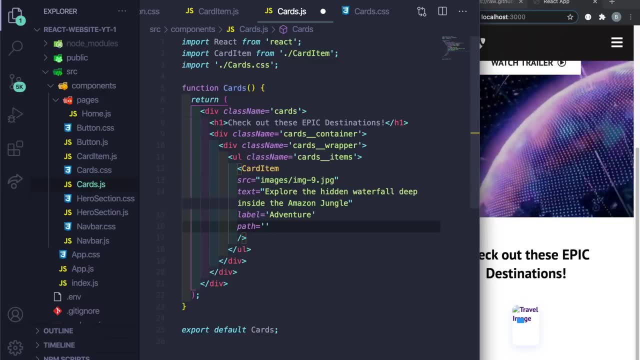 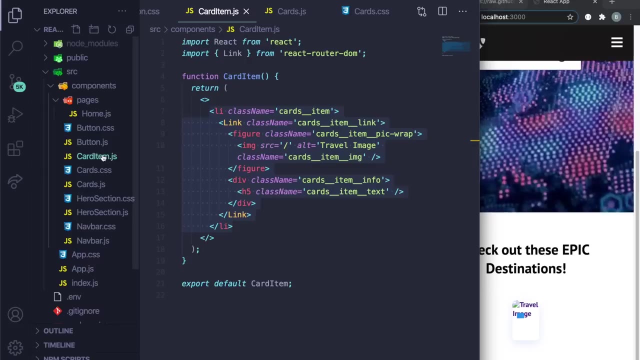 jungle and then label is going to equal to adventure, and then let's do the path so the link it leads to. let's just put slash services. now, if i save this, nothing's going to happen, because we have to go to card item and we actually have to pass in those properties. so what we're going to do is go to the 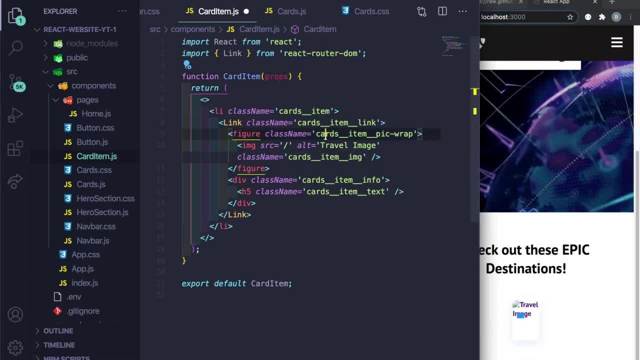 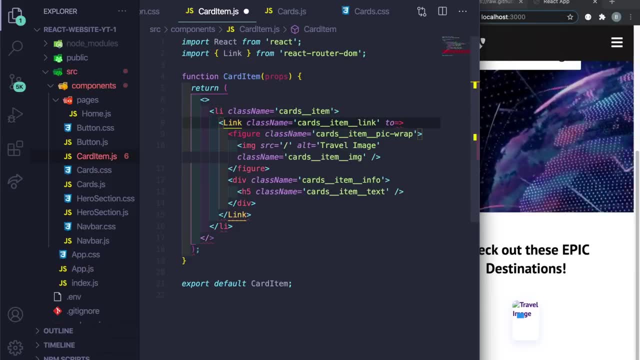 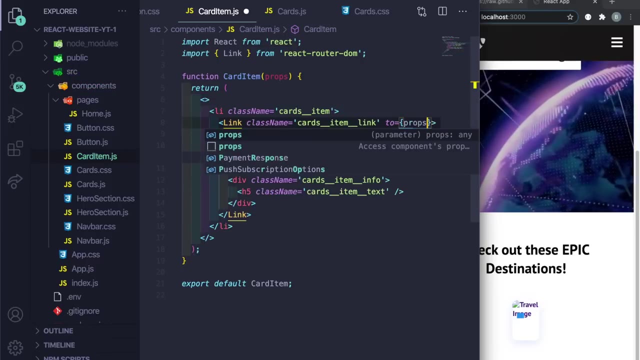 cart item parentheses, and just type in props. and then here we're going to go for the link. i want to say set the two, which is how you do it in react router. i said the quotes. i want to say that quote. i'm going to say equal to curly braces, and then we're going to pass in props. 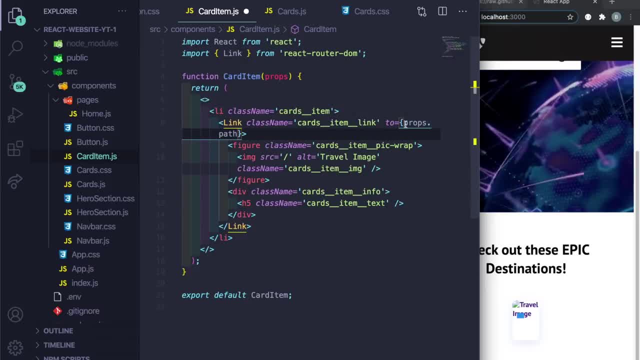 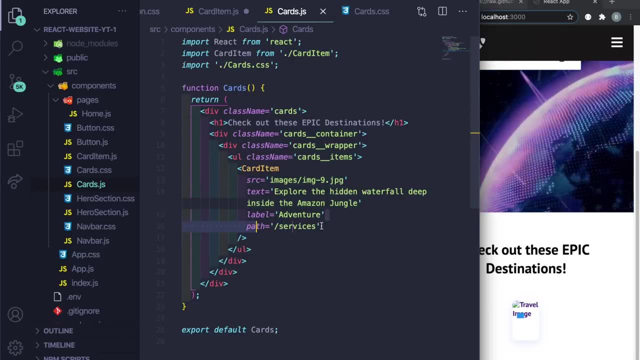 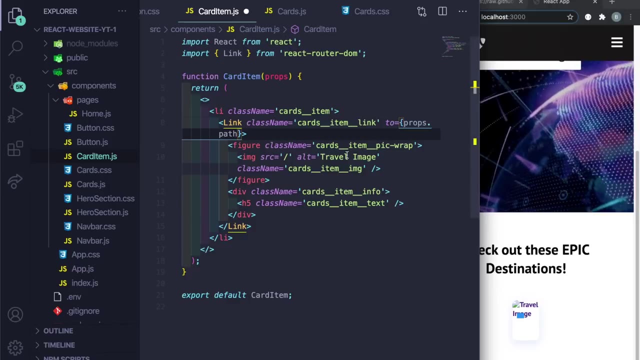 dot path. so this is essentially taking whatever we added on the cards property, aka the, the path right here, and it's going to pass it down to this component which is going to display on the screen. so then we're going to do for the figure. so let's let me command b so you can see more for the figure. 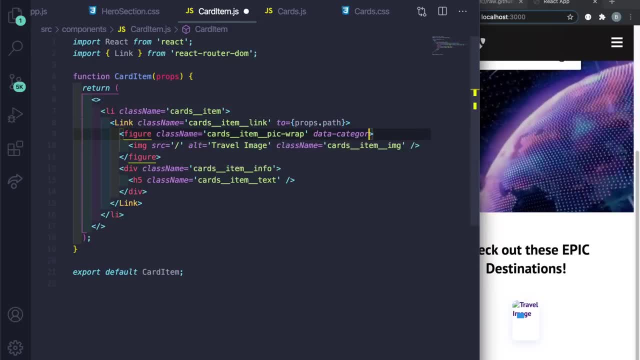 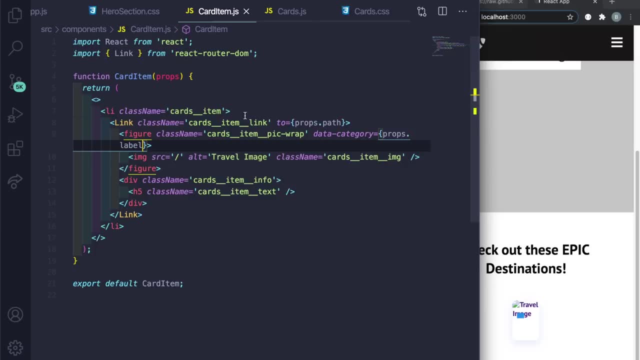 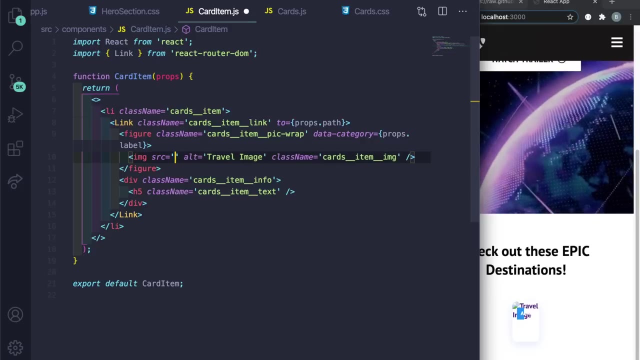 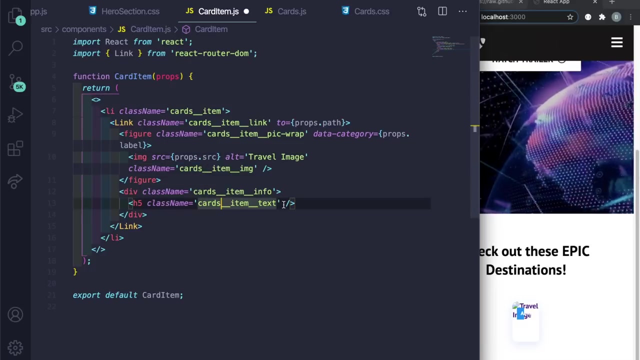 i'm going to say data category equals to props dot label. so right now, this is the- uh, let's actually just type everything out, then i'll explain it after. so image src- curly braces- props dot src. and then for the text it's just going to be: it shouldn't be a sub closing tag. so let's close this out. 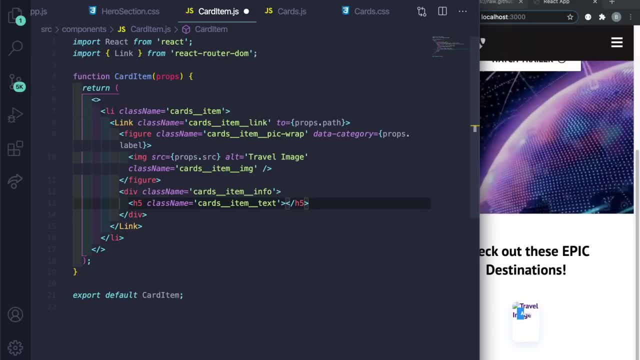 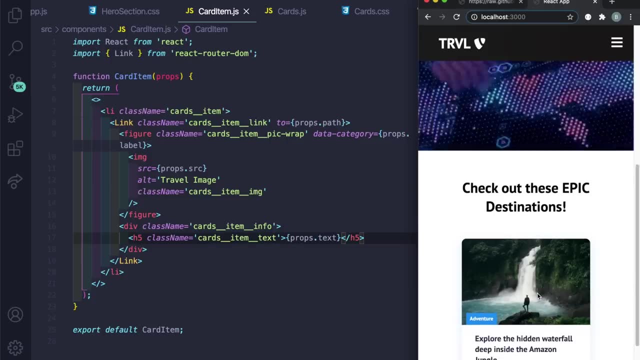 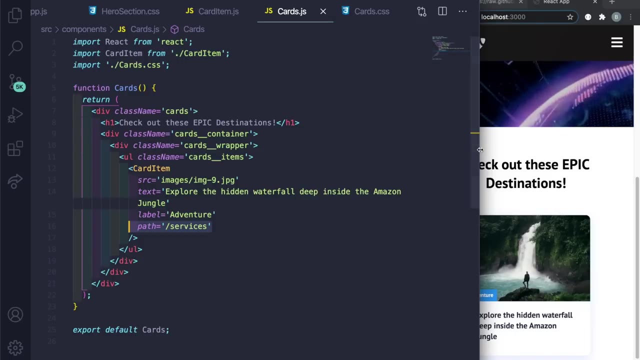 it should be like this, and then i pass in props dot text and then curly brace. so if i save this now you can see i have a nice little clean card and basically if you go to carjs, all the properties that we passed in are showing up on here. so this is the label, which is: 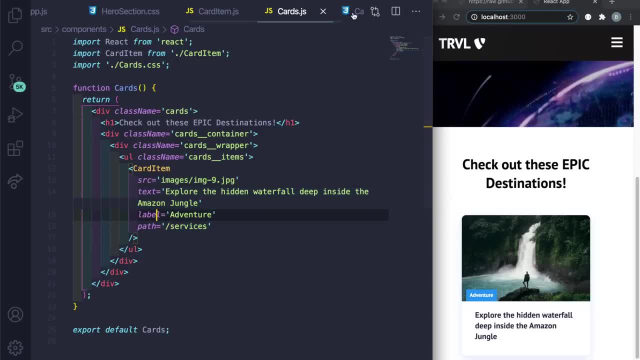 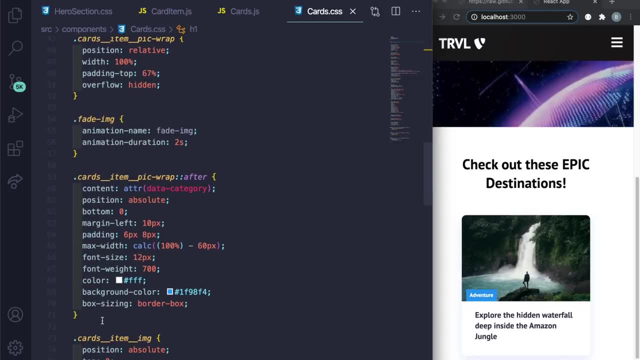 adventure right here and then in the css. if i scroll down, most of the stuff is typical. you know flexbox, but this is where this uh little adventure- blue css here and basically the content. it's set equal to data category which, when i go to card, what happened on my card when i go to card, item. 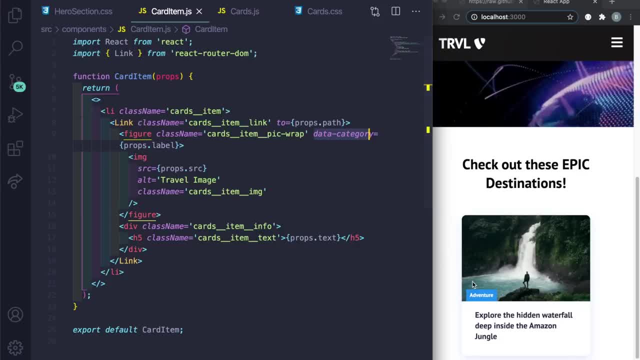 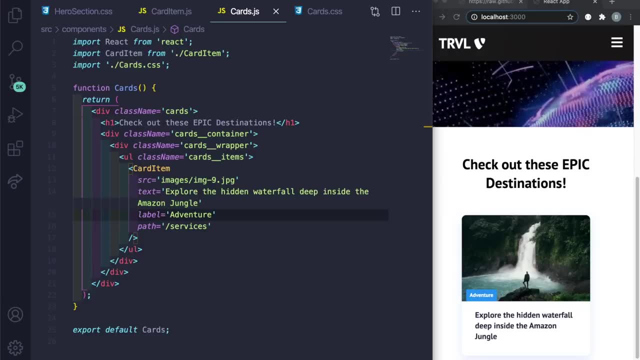 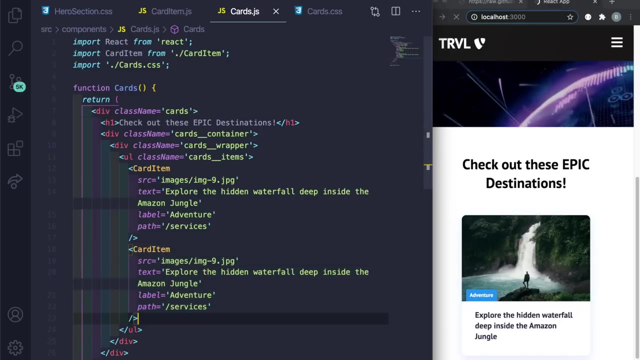 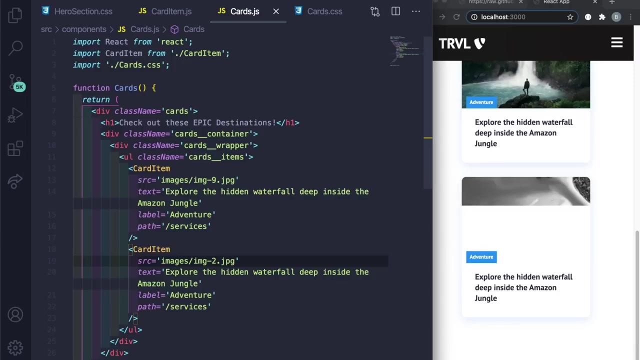 we set it equal to data category. so that's basically how we did it over there, and now what we can do is pretty much just copy and paste this entire card item component and then just update the properties. so now, if i save this here, we have the second one, and then i want to change this image to number two. now you can see, we can easily. 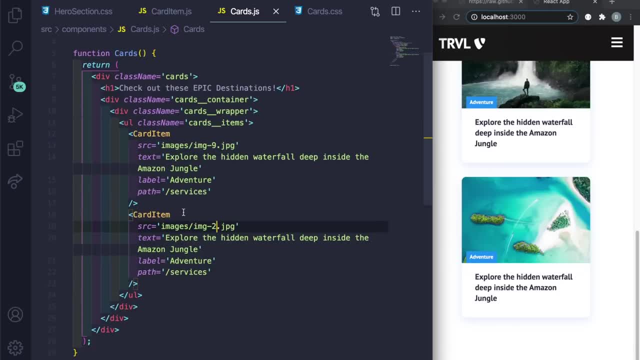 do it right here in the cars component and we don't have to sit there and copy and paste it like a million times, doing everything else here, and then we can basically just go ahead and show up in theót�� setos for a text. let's change the everything else. so for the text we can just say: 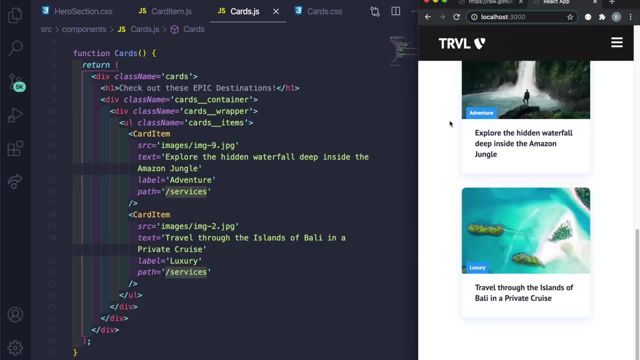 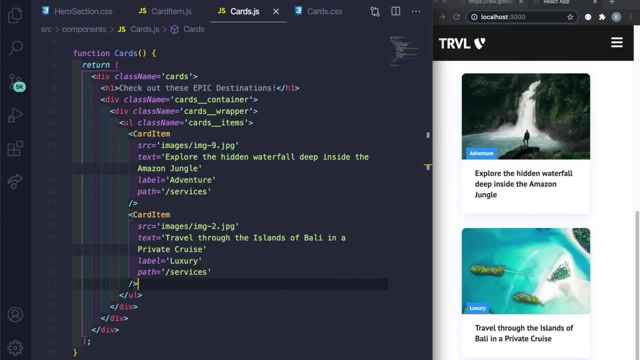 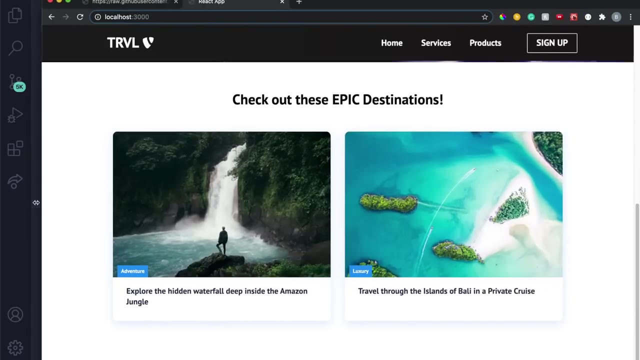 travel through the islands of bali. updates. we got all the CSS added, so now, basically, you can just sit here and I'm just gonna straight up copy and paste the actually no, I'm not gonna copy it, I'm gonna show you what I did. so when you saw in the video the intro, there was: 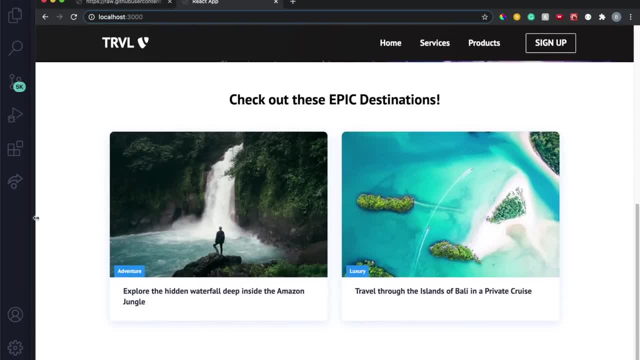 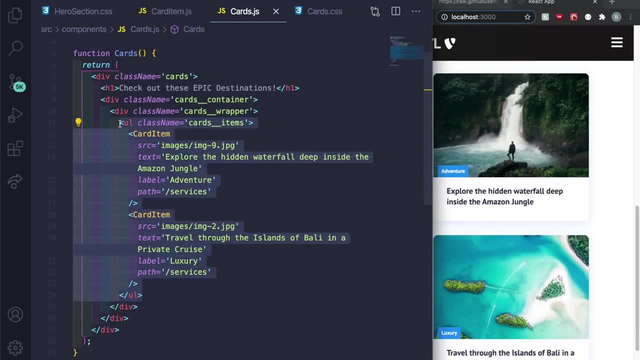 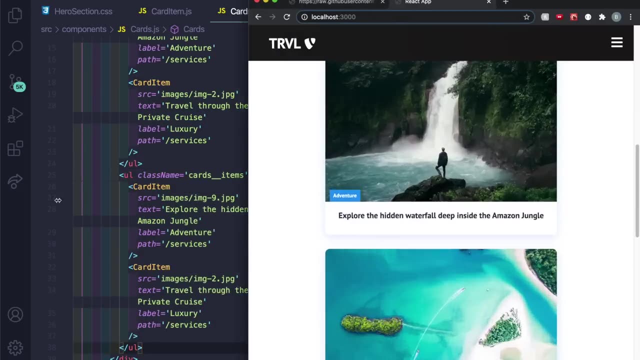 two like this, and then I had three on the bottom, so you can't just copy another three underneath, you have to wrap it around. this ul tag, this ul tags what makes it to where it separates. so if I go like this and just copy two in and then show it in desktop, it's basically something like this. so now, 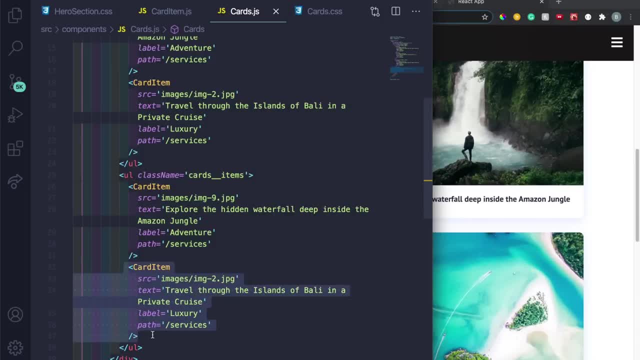 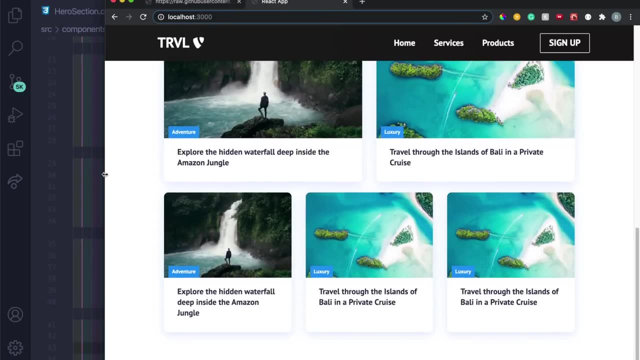 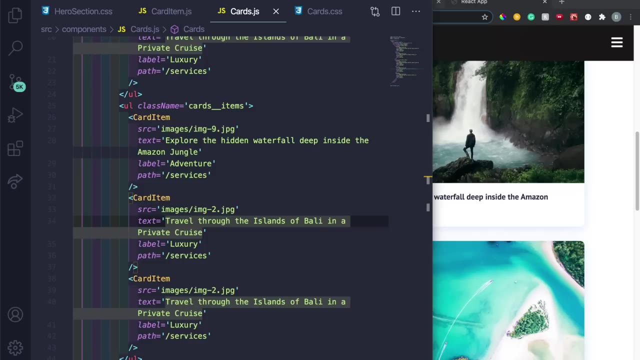 let me just add a third one here, this, and save it. and then now, when we scroll it out, it's basically like this: so now I'm just gonna go into my original code and just copy in what I had for this third section, just to save time, but you 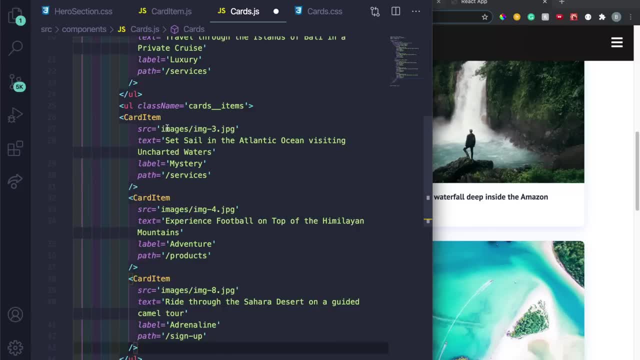 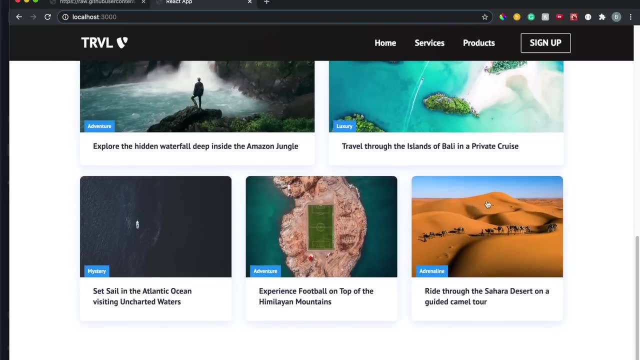 feel free to customize these whatever you like. whatever they say, it's basically the same. as I think I just updated all the images in the text, so I'm just gonna copy this and paste it in here and then I'm gonna go back to the text. so now it's pretty much. uh, you can see here, so it looks. 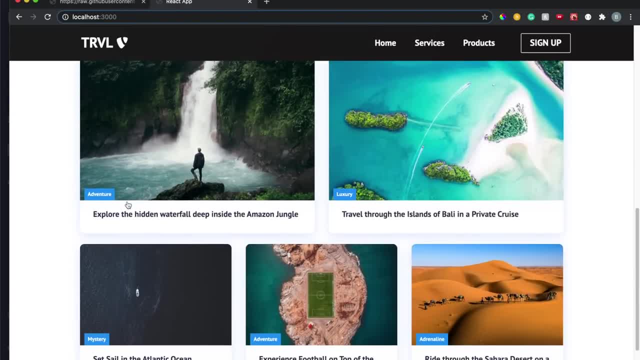 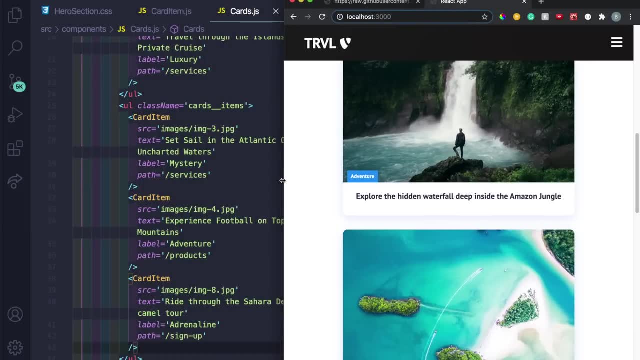 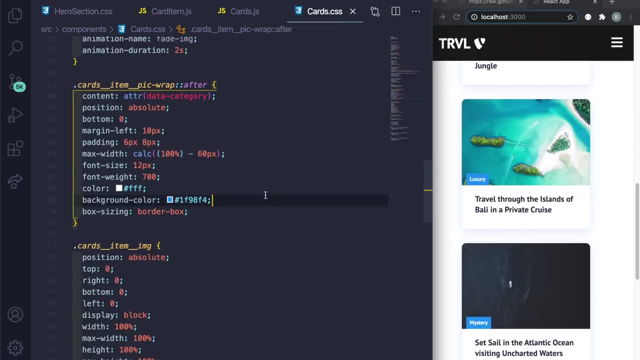 like this. it's basically the car component, so wasn't too crazy so if I were to actually go here and shrink it now, you can see that they change and they basically are more responsive. and that's pretty much from CSS, which you can go through line by line and check it out and play around with the code in. 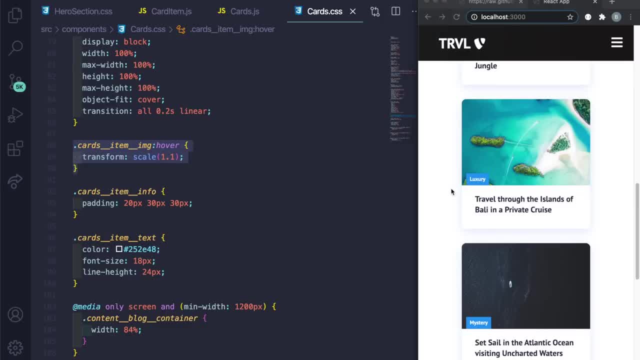 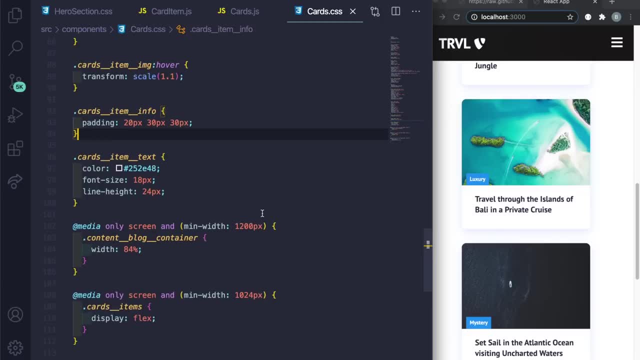 case you're confused. and then this is the little, this is the code to make it hover. so if you're wondering how I did that, this is basically just scaling and making it bigger and zooming in, and then this is just a media query. so these basically are reversed. so it's going from: 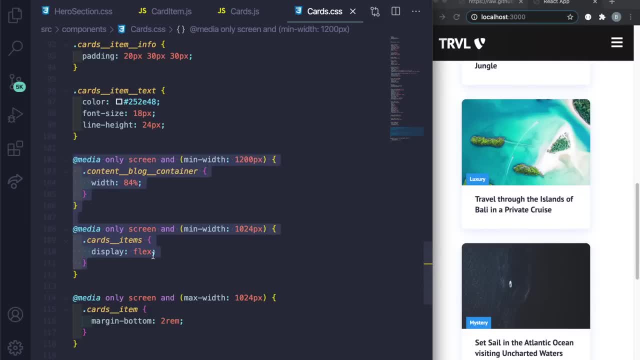 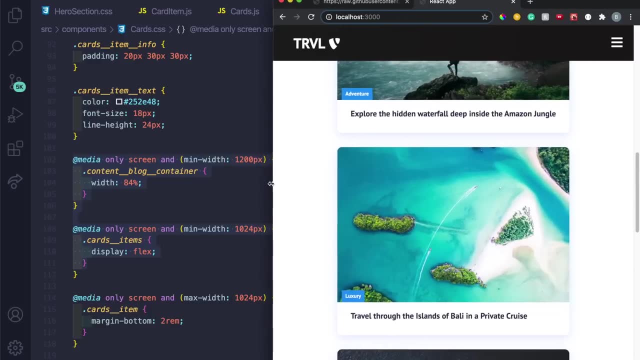 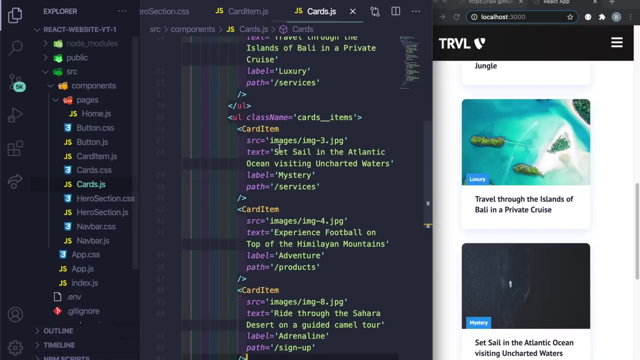 uh, like min width for these, so it's only displaying it if the screen is this size. so once I get to here it's going to increase the splits, like that. so go, feel free to play around with this card CSS to see what it's like. but we're pretty much good, I think, on the cards. 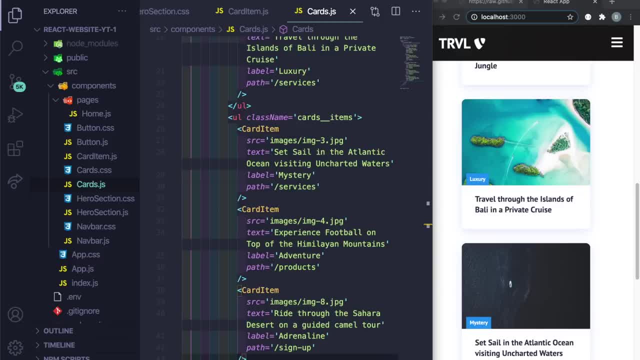 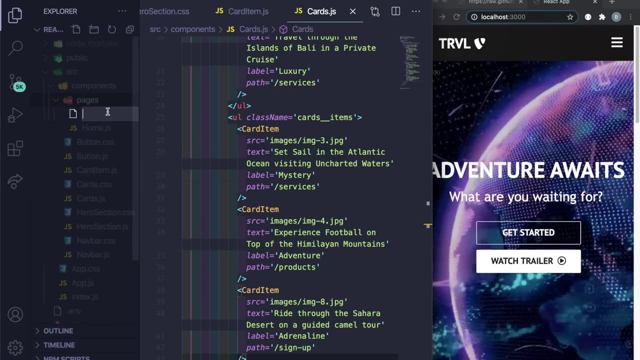 section. so now let's go ahead and let's finish up and create some pages now, just because I want to, um, when I click stuff, like if I click here, nothing happens. so let's go ahead and um go to our pages now right click, hit new file and then just do productsjs. 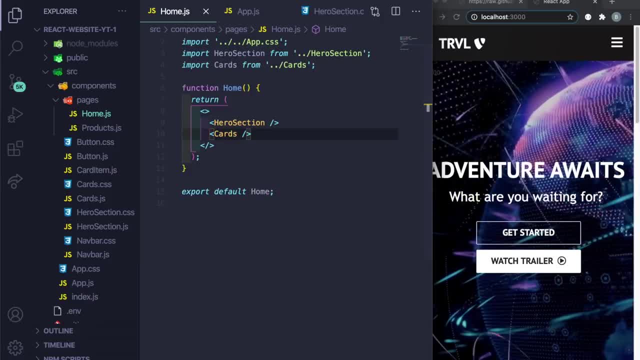 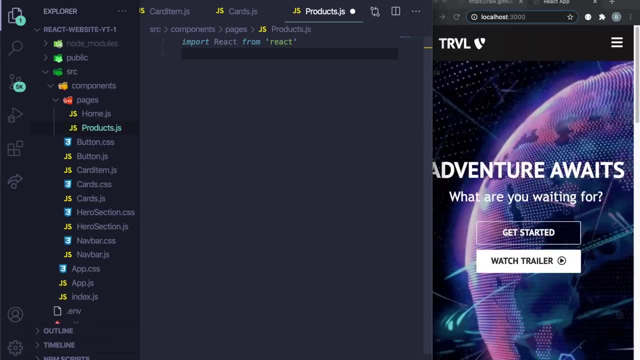 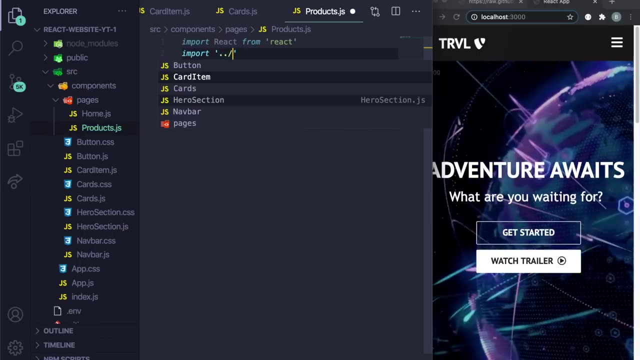 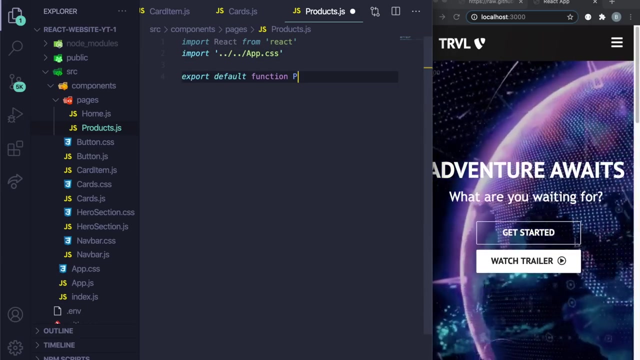 and then let's just do- we pretty much. let's see I can copy in. let's just go here, let me do this once, then we can do this over and over. so let's just do import react from react import dot dot or quotes: dot dot, slash, dot dot, slash, app dot, CSS, export default function products. 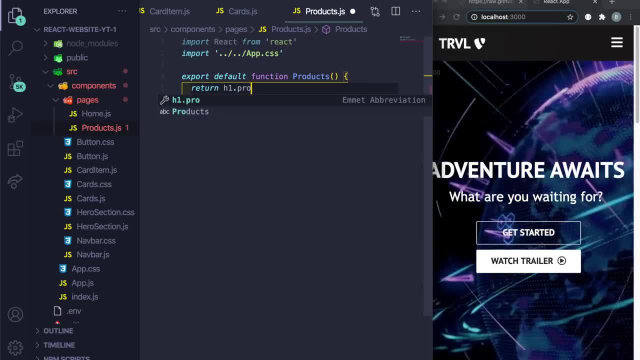 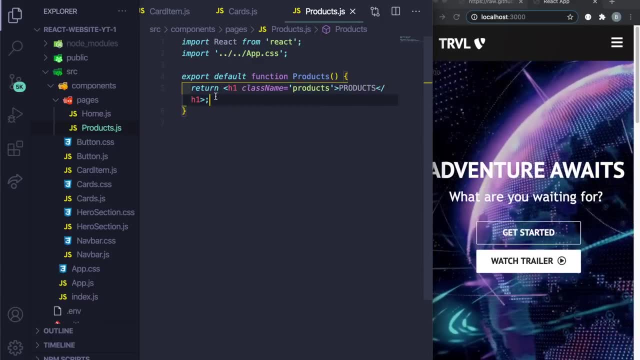 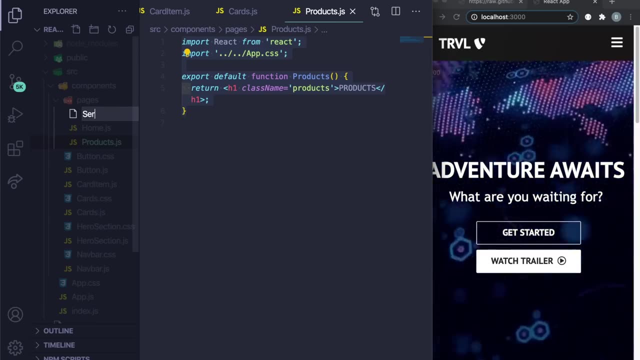 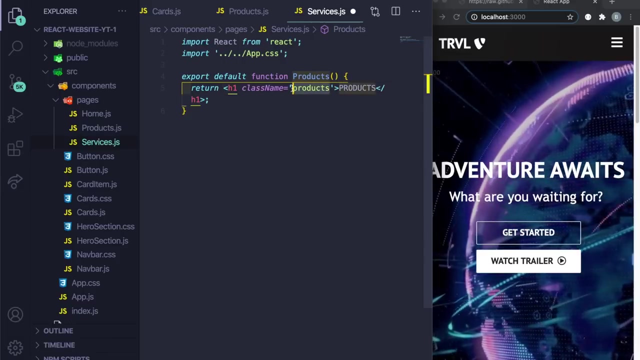 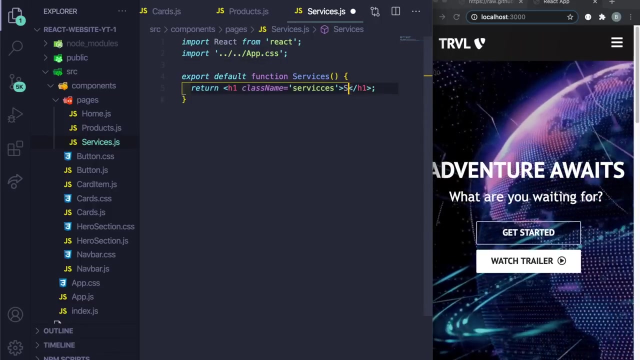 and then return H1 dot products with products inside. so save this. so now, if I were to actually go, let me just copy all this now and then pretty much make a new file and just do servicesjs. copy everything in here, just change the thing to say services, and then here will be services, then products will be service. well, 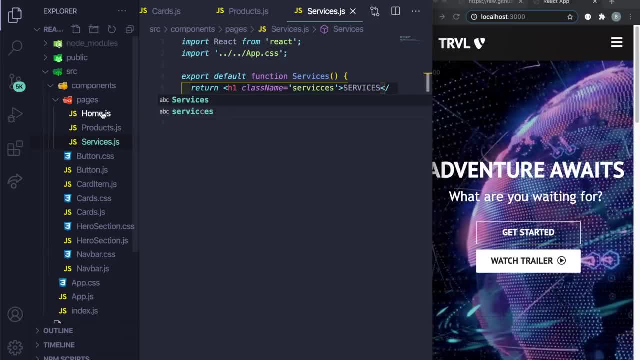 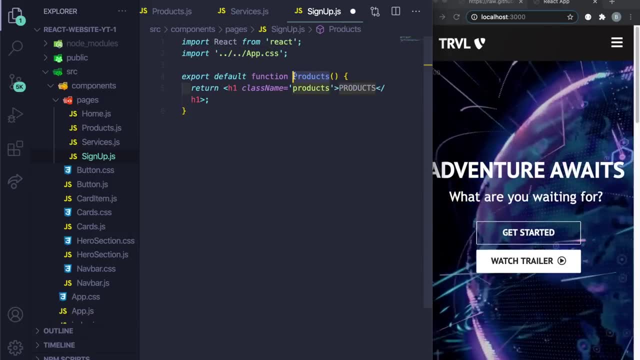 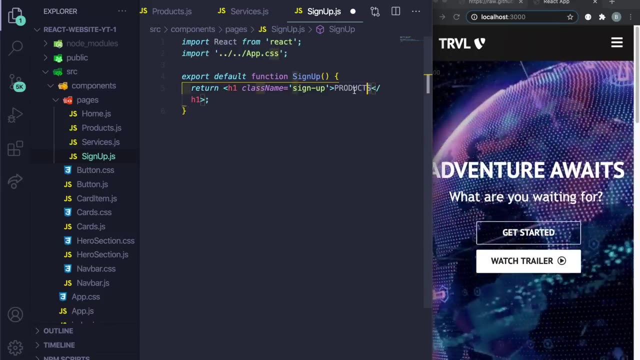 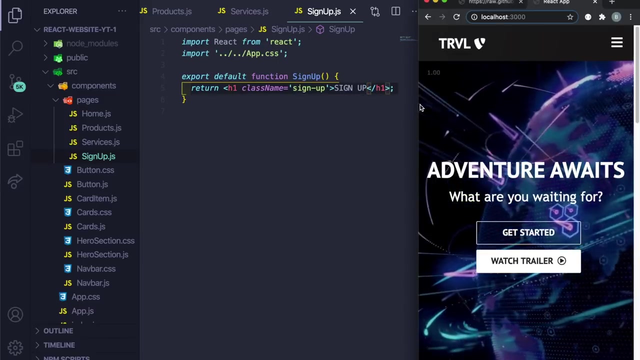 actually just do save that there, and then let's do one more page and let's just say sign upjs, and then you can just say sign up, sign dash up, and then it should be sign up. save that now, and if we go, actually let's go to our appjs now. 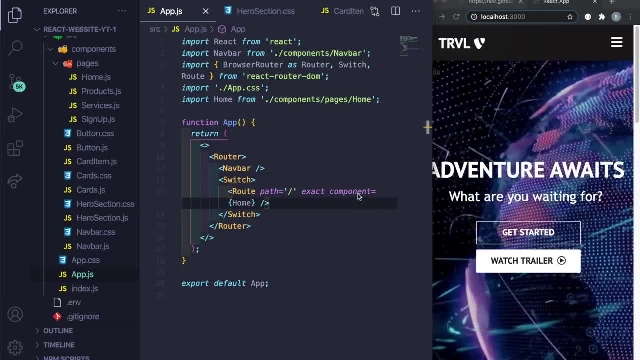 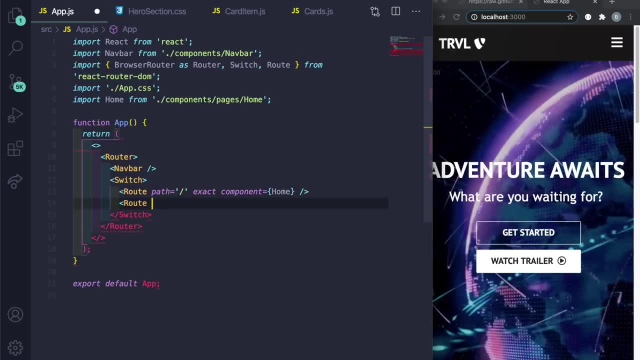 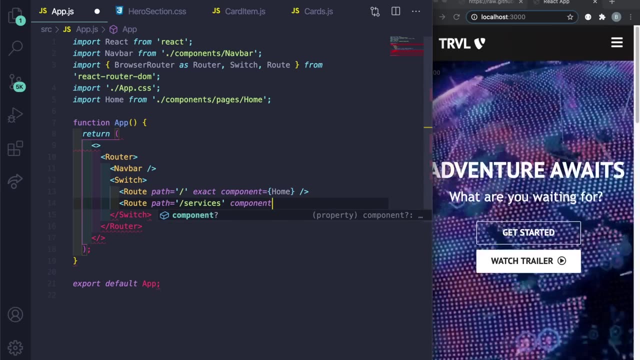 and what we're going to need to do is import the remaining paths so that whenever you click on these, they'll basically work. so, pretty much, let me talk about the first one for a route, and once that, the pet equal to slash Services, and then I want the component to pop up will be the Services. 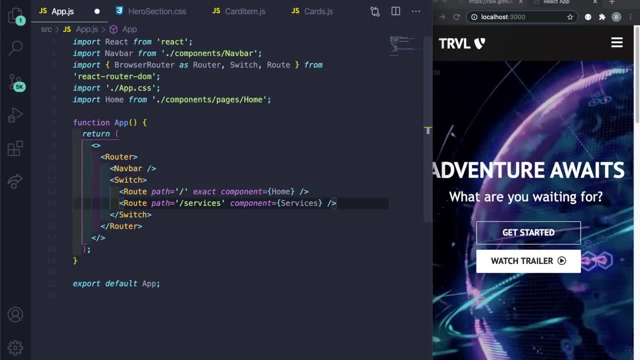 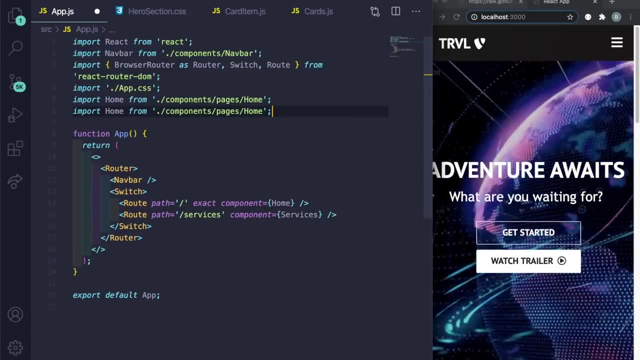 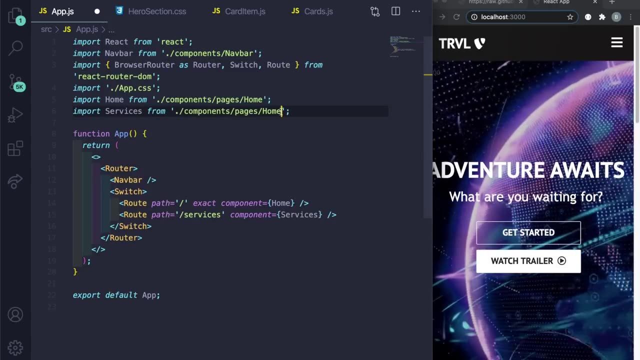 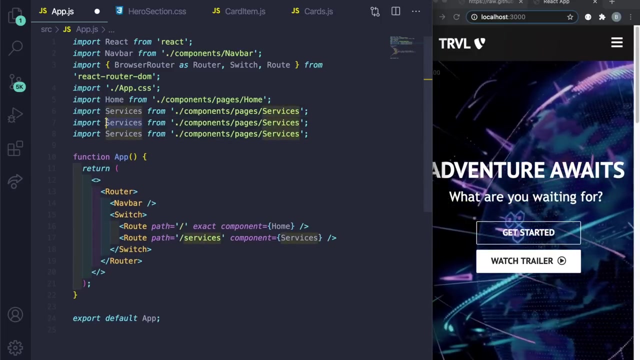 component, whichever you just created in the pages, and then we just have to import this pretty much. so let me just so, where it did doesn't put alt shift down arrow and it copies that line. and then let's just say services, four elements from home, services, and let me do it two more times because we're going to do the products. so 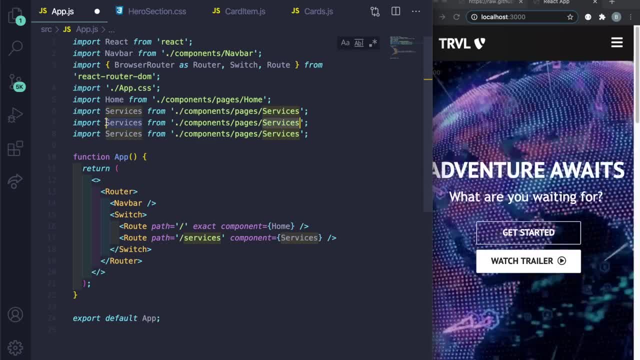 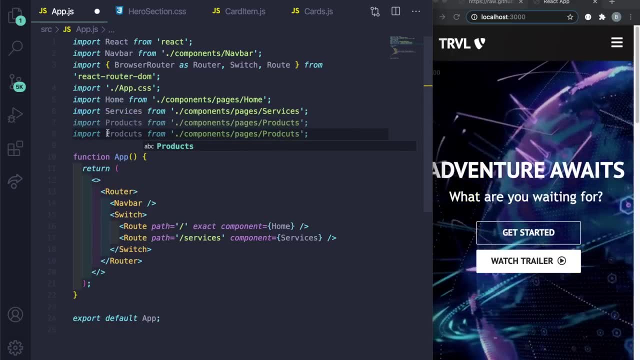 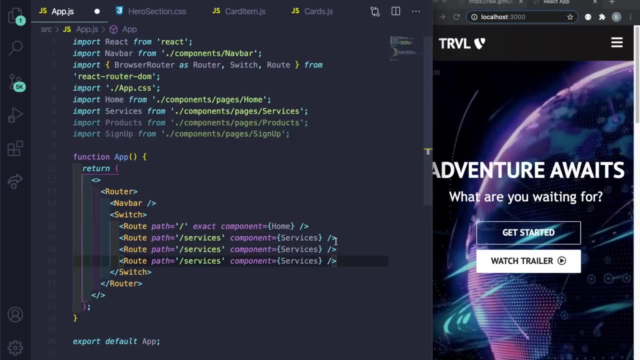 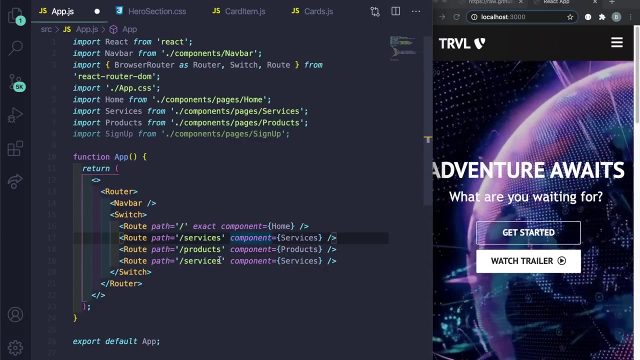 you can highlight the word and do command d, so highlights all of it. let's just do products and then do the same thing here, say products or not, product sign up, and then we can basically just copy these links again and then let me just change this to products, products, and then here: 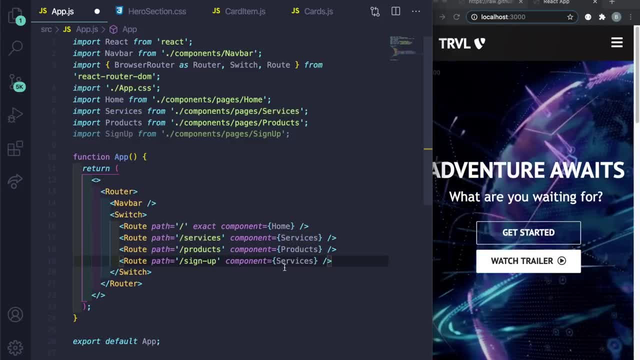 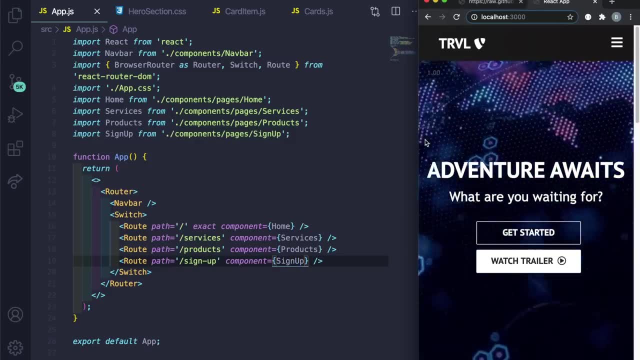 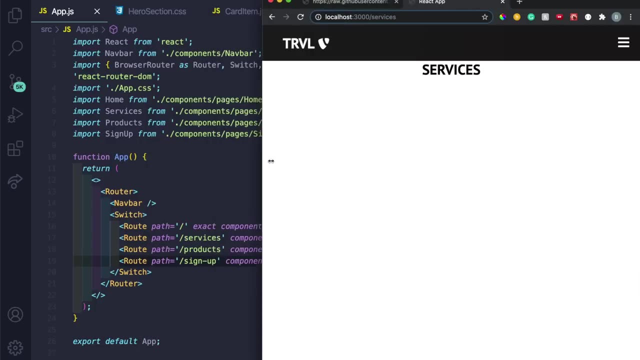 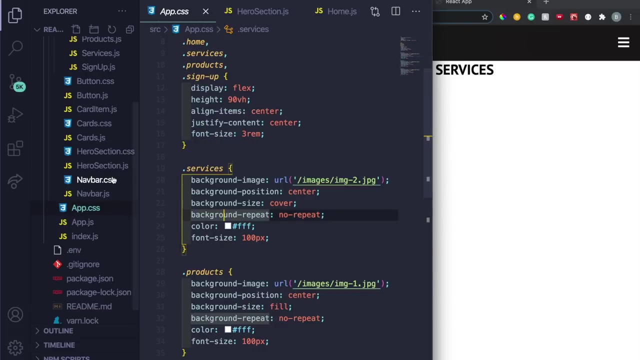 we can put a sign dash up and then we have sign up, which was the page one that we created. so now, if everything is working out, services should show up and it looks like: um, let me see, i'm missing it on my appcss. all right, so let me go and check the. uh see, services should be service. 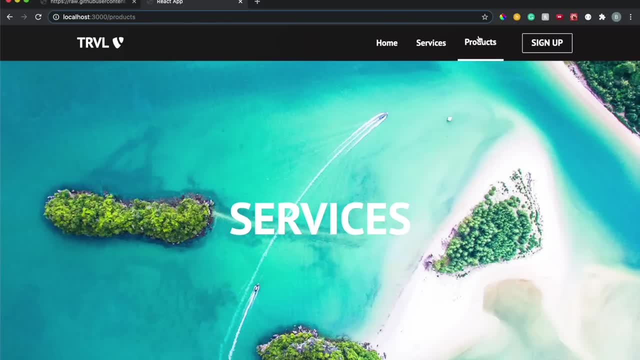 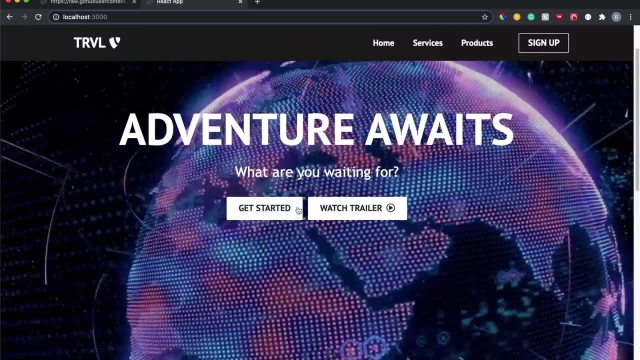 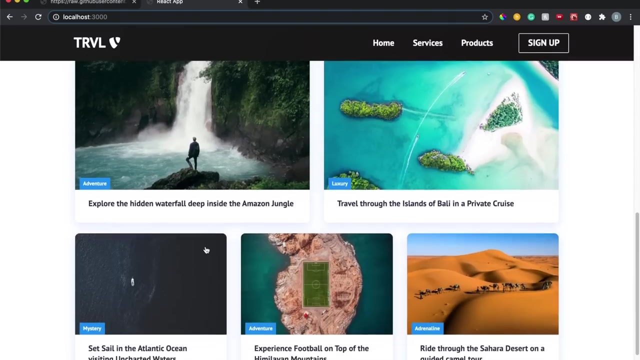 all right, so perfect. so now that looks like it's good. so then i click on products- looks like it's good here, and then sign up home, also here, and then i can check these buttons here. so these basically the, this one goes to sign up, same here, and then also let's check out these cards. so i think this: 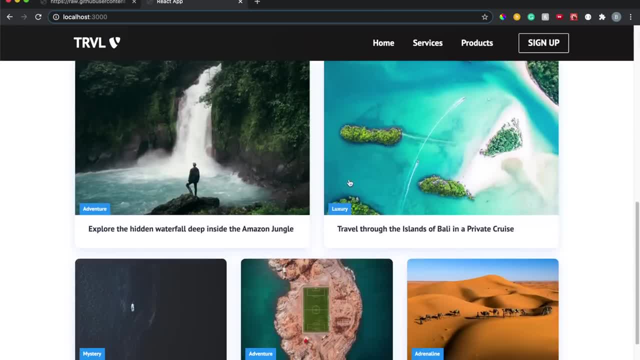 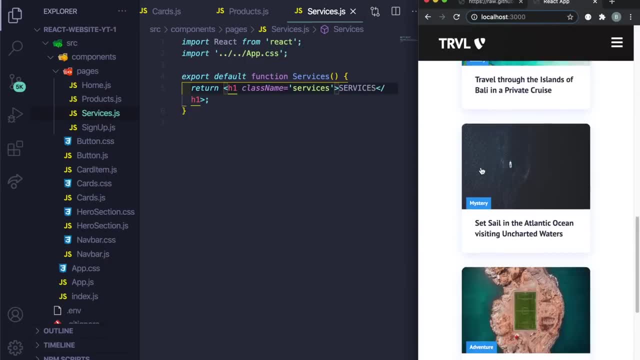 one. yeah, they're pretty much all services, i believe. yeah, so pretty much good. looks like everything's working and, in terms of everything in terms of mobile, looks like we're looking good right now. so now we just need to do is create the footer and then we'll pretty much finish off this website. 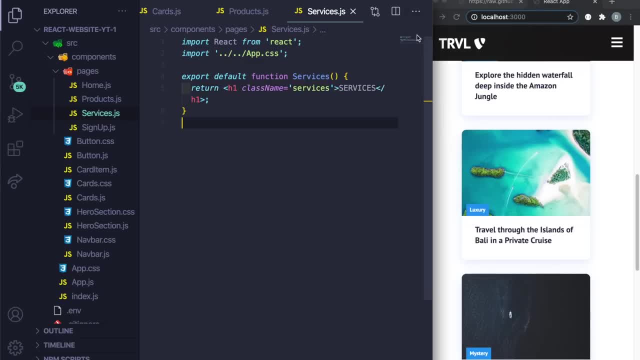 design. so let's go back actually to our code editor and let's start coding. so now let's go over to the components, right click and let's do new file and let's just type in footer dot js. and then let's create another file and let's just call it footercss. now the foot, i'm put. all of the 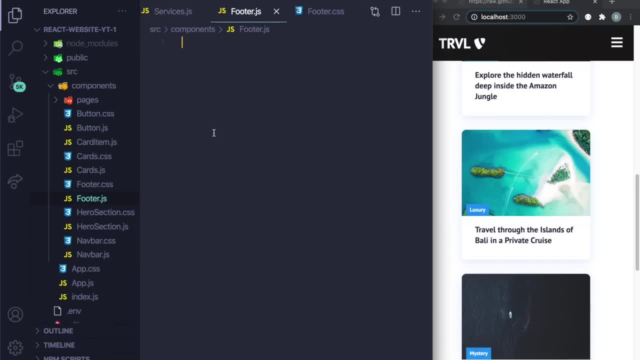 jsx inside of it, because i'm not really planning on reusing it like a car component. but again, you can separate this, make it however you like, but let's go ahead and let's just do rfce and then let's go and inside this top div i'm gonna say class name equal to footer dash. 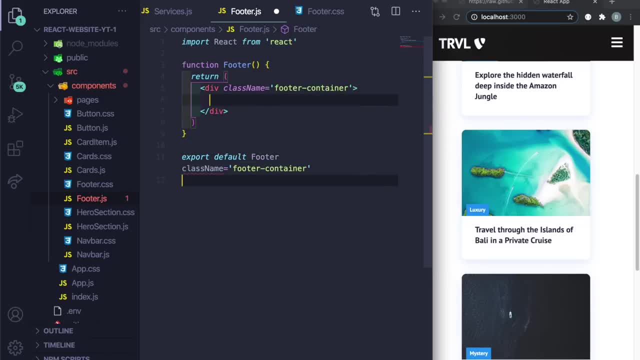 container. now in here i'm gonna create a section and this is going to be where the little uh like email sign up was. so i'm gonna say section dot, and sometimes it does this. so let me get rid of this for a second and let's just do section dot. footer, dash subscription press tab and let's press enter. 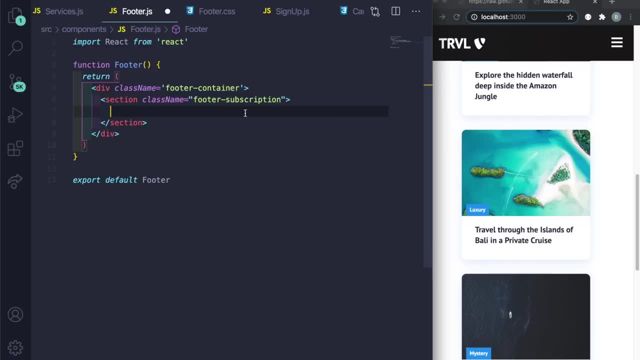 let me command b so you can see this. and now let's create the p tags. i'm gonna say p dot footer, dash subscription, dash heading, press tab. then inside here i'm going to say: join the adventure newsletter to receive our best vacation deals. and then, underneath this, i'm going to do: 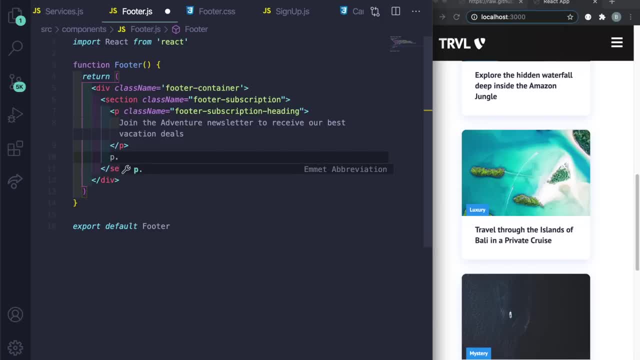 another p tags. i'm saying dot or no p dot footer, dash, subscription section, dash text. and then here i'm going to say you can unsub, unsub, scribe at any time. and then outside of this we're going to say input areas or dots, input, dash areas, press tab. 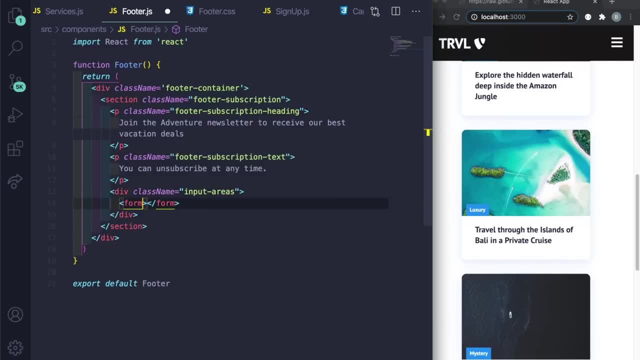 and create this form. let's get rid of this action. i don't need right now essentially what this form wrapping in the input tag. so basically whenever you press enter, it just automatically will submit. so let's say: input dot, footer dash. input type will be email, name will be email and then place: 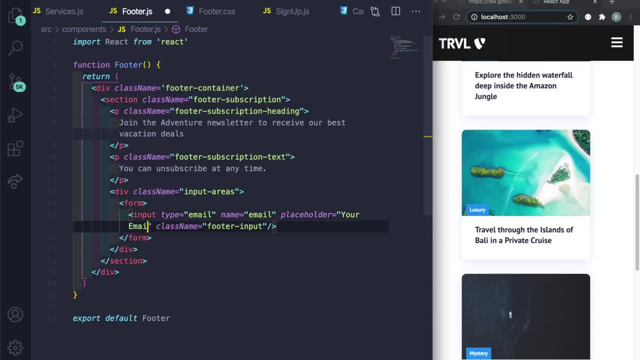 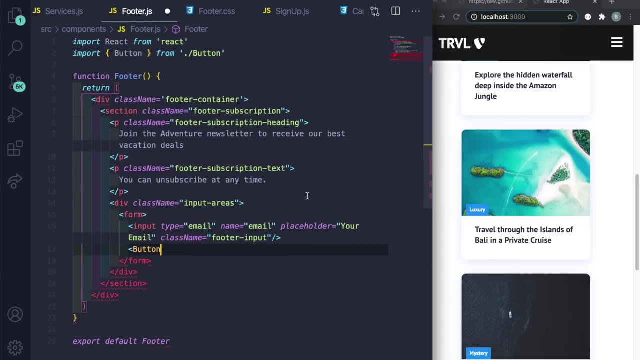 holder will be your email and then, underneath this input tag- it's still inside of the uh form- we're going to pass in the button component and it looks like it imports automatically. i'm going to set the button style equal to btn dash, dash outline, and then we're just going to say subscribe. so i'm going to save this now. 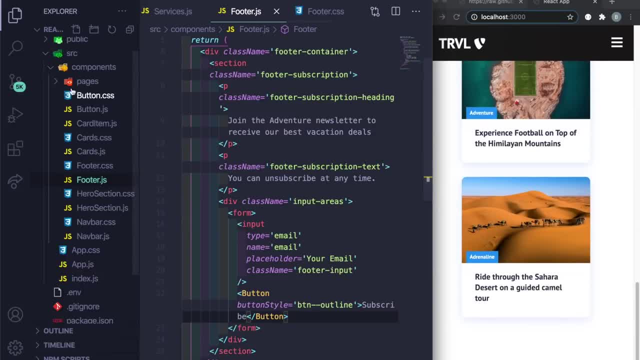 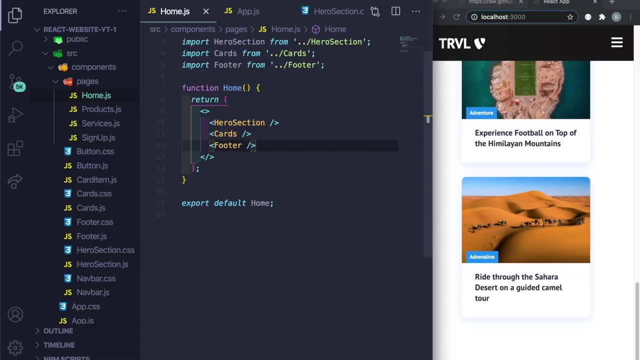 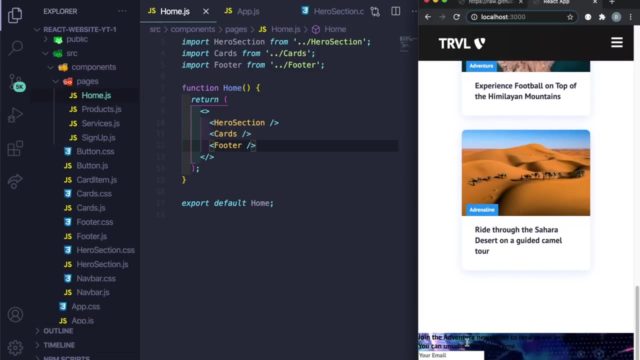 and basically nothing shows up. so let's go over to the pages home and let's import this footer, save this here and now. we got this little footer action now you can see right now we got this crazy like video show in the background. but we're gonna cover that with the um. 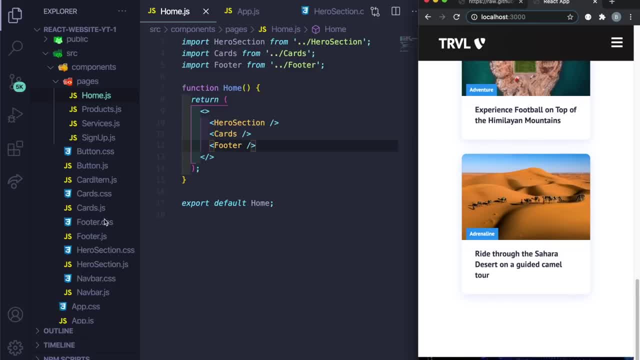 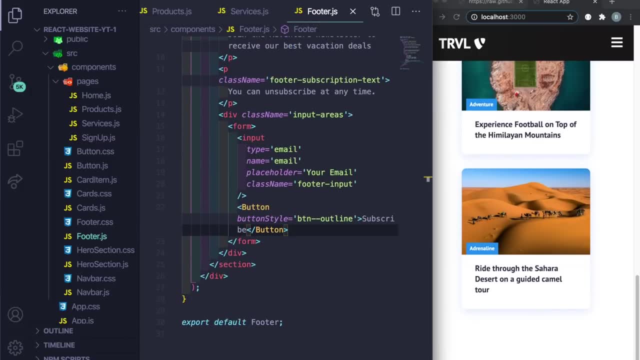 the css eventually. so let's actually go over to here and i'm actually going to uh, type out, actually let me see if i can add something for now, just to get this covered up. so let's do go to footercs dot footer dash container. and i'm actually going to go through this one because 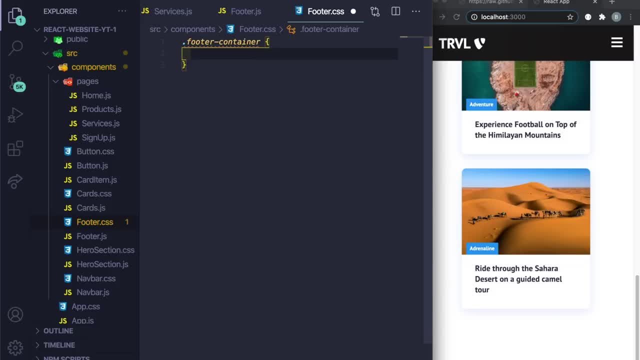 in terms of responsiveness, it might not make sense if you just copy and paste it, so i want to explain stuff i did, so let's just do background color: hashtag: two, four, two, four, two, four. padding will be four: ram zero, two ram zero. display flex, flex. direction to be column. 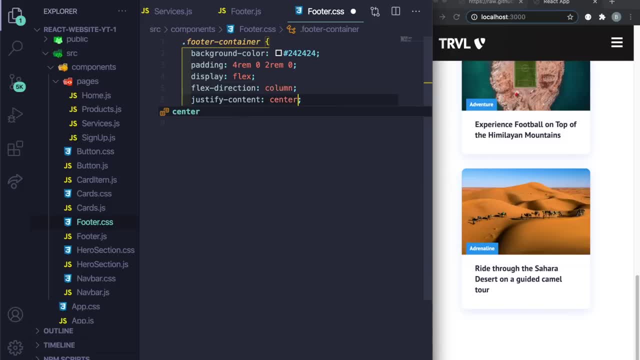 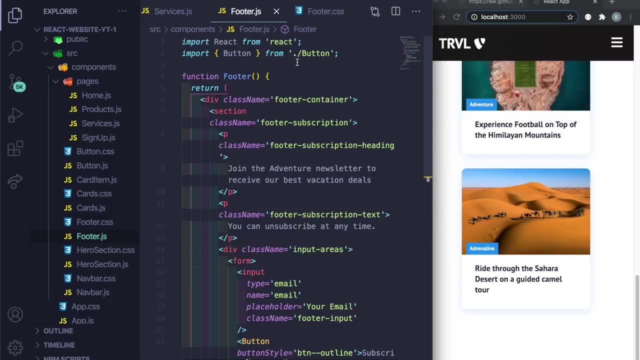 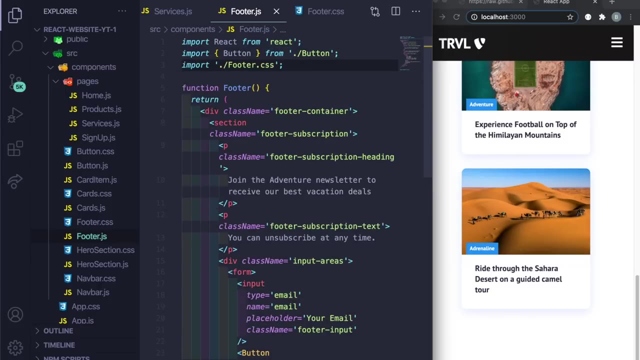 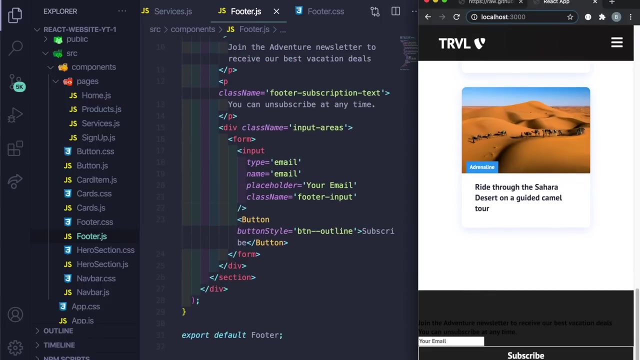 just like content center, and then let's do a line item center and then we just got to import that in a top. so let's do import, dot, slash, footer, dot, css, and right now you can see we got our little thing right here. so now let's go back to adding some more of our footer jsx. so this should complete the section tab. 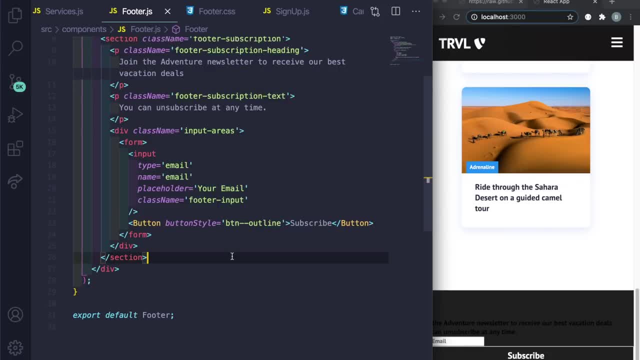 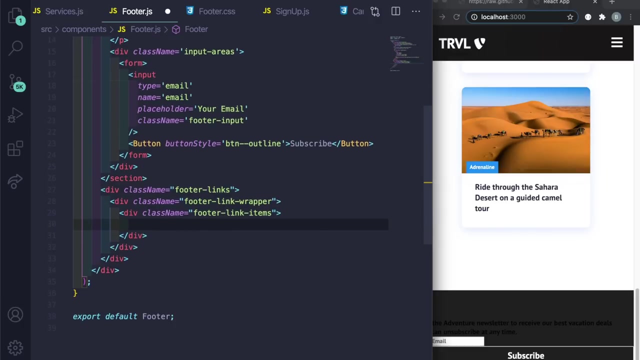 here. so underneath this section i'm going to say i'm going to put dot footer, dash links, and then i'm going to say dot footer, dash link, dash wrapper, and then i'm going to say dot footer, dash link, dash item. so the actual items now. so these are the links. so in here i'm going to put an h2. let's say about us. 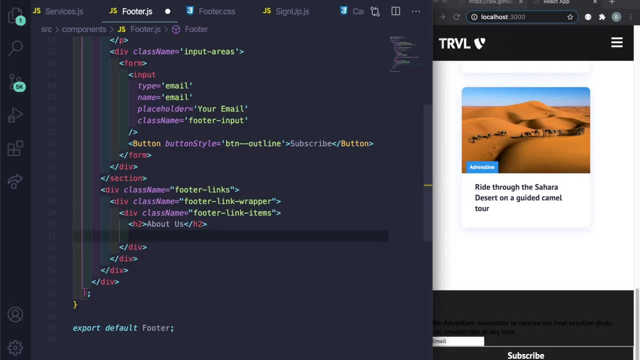 now, under this h2 we're going to add a bunch of links. let's just say link tab, how it works, and let's just put two equals to slash sign up. this is just. it's not necessary, but it's just to show you like if you click, it works. 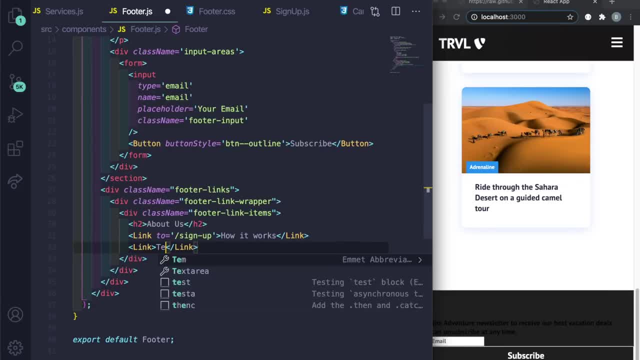 and then we can just say link again and just put you know testimonials and then set the path equal to dot slash and then you basically just rinse and repeat and copy this. so i'm just going to go and copy this from my code. so we have the three here. 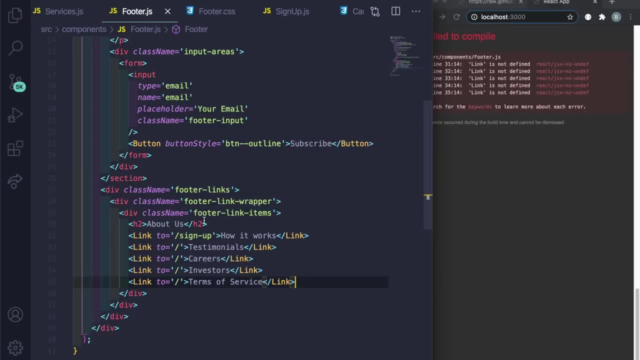 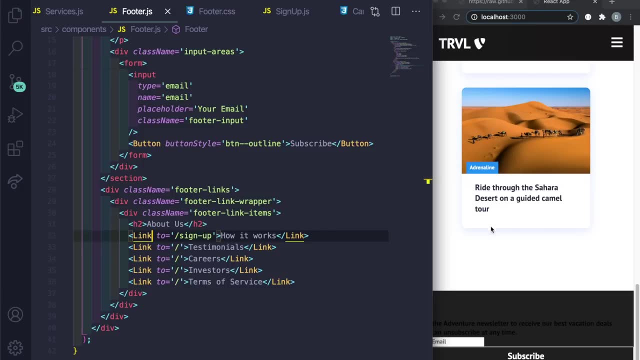 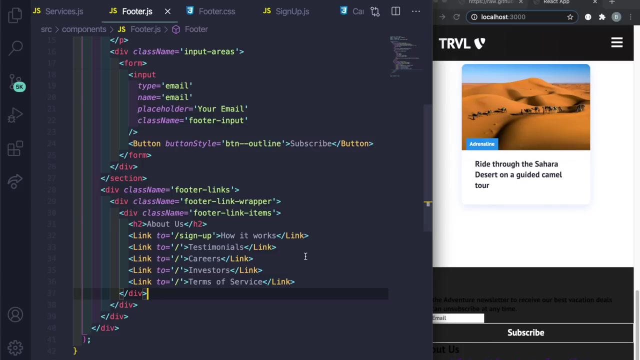 so let's save that. and right now it's gonna say links not defined. so i can click on the end of link control space press, enter, save that. and now we got these like links down here. so now you pretty much can just copy and paste this over and over again. so what you could do is copy this entire footer items. 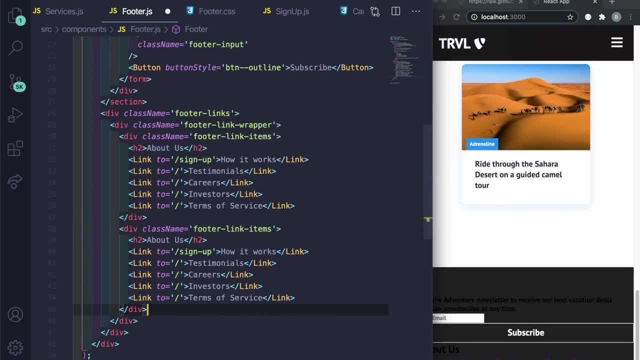 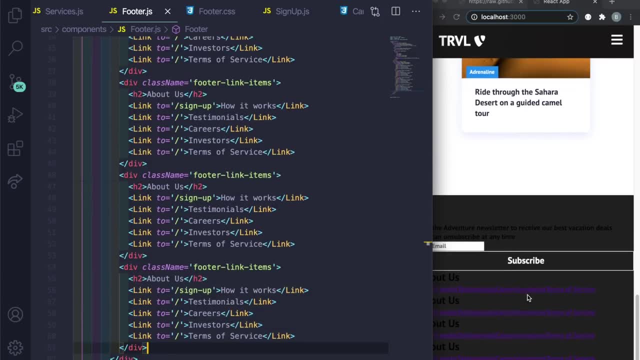 did with the links: paste it and then paste it again and then basically paste it again. so now you have the entire footer links set up here so you can do that, and then you can edit them individually to whatever you want and then whatever you want to hear. so let's put like: 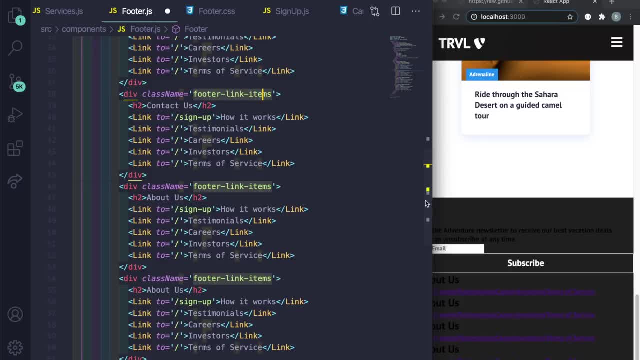 contact us now. to save me some time, i'm just going to straight up copy my original footer, just because it's. it's going to take way too long for me to sit here and type all of this stuff out when it already makes pretty much the most sense, so let me get my. uh, now one thing? no, let me actually. 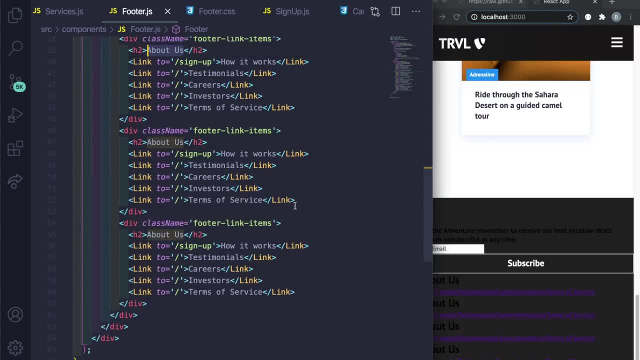 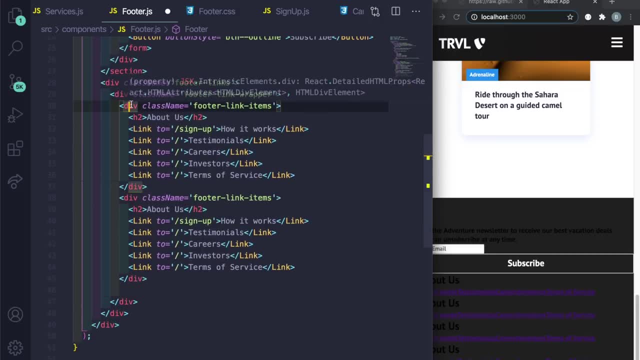 command z this because there's there's a specific code that i have that i forgot. i put so basically here. if i go here, this is the footer link item and then we have this footer wrapper, so i can't copy like i did. i have to wrap the footer wrapper my best, so it has to be this whole thing. 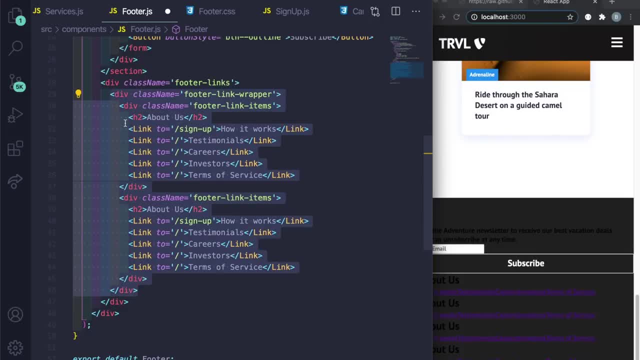 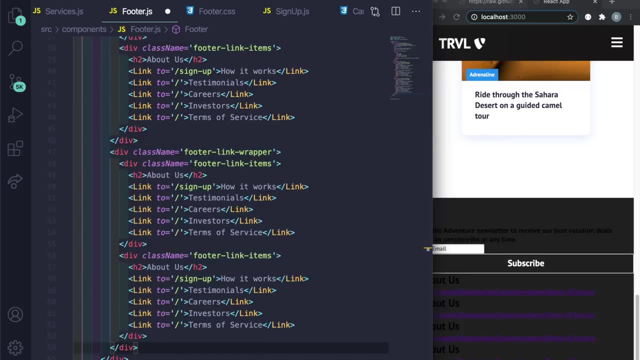 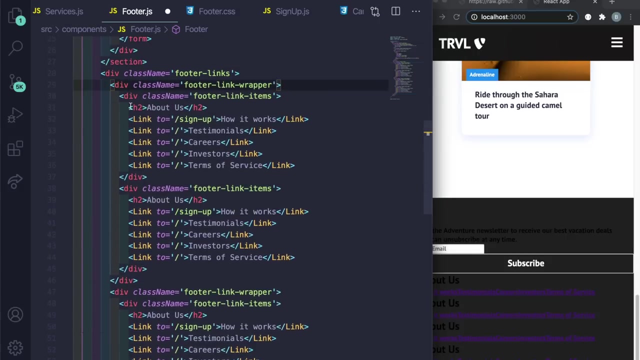 with the wrapper here that you need to copy and then paste that underneath, because if you don't do this when you do mobile response, it was going to be a pain and it's going to be really annoying because it's not doing what you wanted to do. so now i'm going to go back to now in my code and basically copy the same code i have. 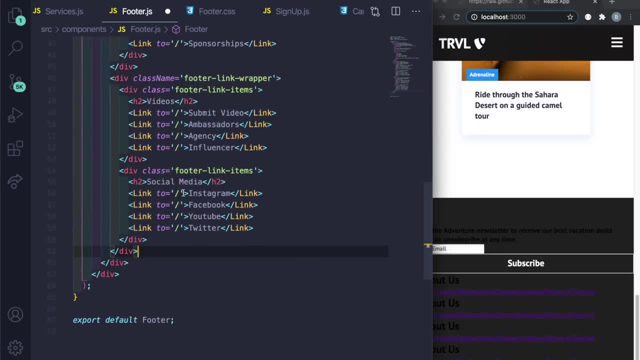 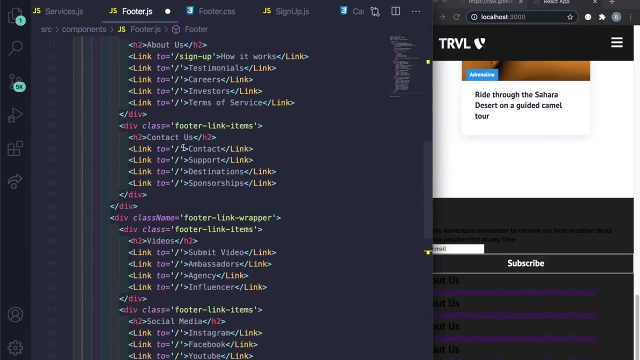 you can get in the github you want. copy that. and let's make sure i have all my divs properly dividing, because if i have a mistype it'll be really annoying. so let me save this and it looks like everything's looking good. all right, perfect, so go ahead and just feel. 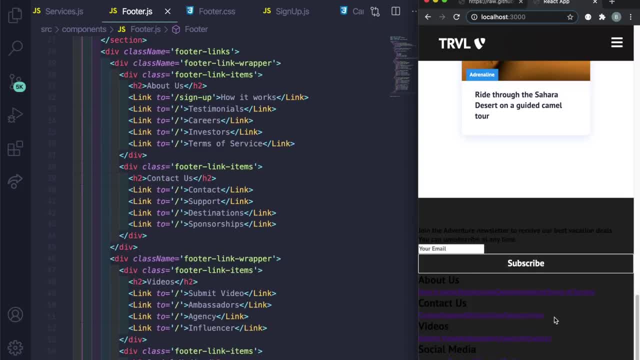 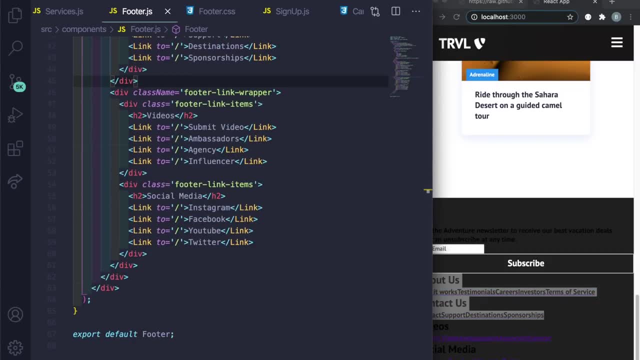 free to edit this. just make sure you have the first two within the wrapper, because if you don't, then the columns will look weird. on more responsiveness. so now we're done with this section. so now, under this third div, i'm gonna press enter and then here i'm just basically going to create. 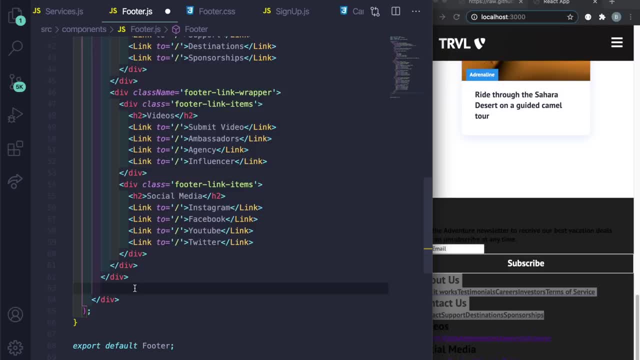 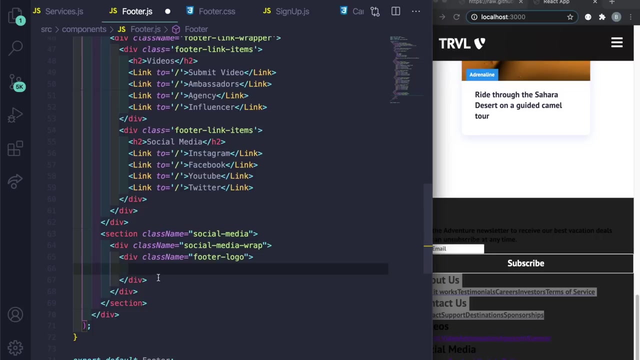 the last thing, which is the social media icons. let's just say section dot- social dash media and then let's do dot social media wrap and then dots footer dash logo. so now footer logo. i want to pass in the link, so let's do link dot social dash logo. 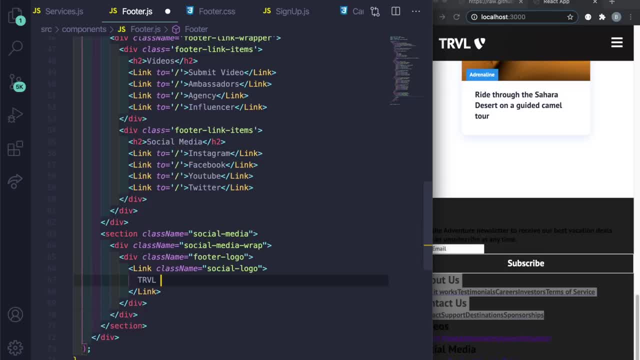 within here i want to put t r v l and i'm going to pass in actually the i dot f a b dash, oh no, f a b dot f a dash type oh three. and then in the link to i want to set that equal to just put: uh, just a slash, let me. 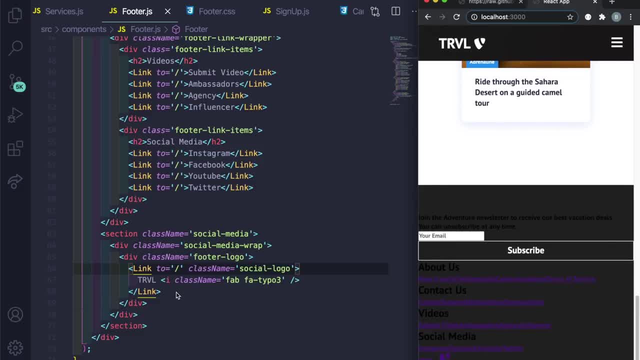 save there for now. you can see we got a little travel logo link here and then underneath this div we're going to say small dot website rights and this is basically just going to say trvl and i have the copyright logo. you don't have to put it, but you can just say like: 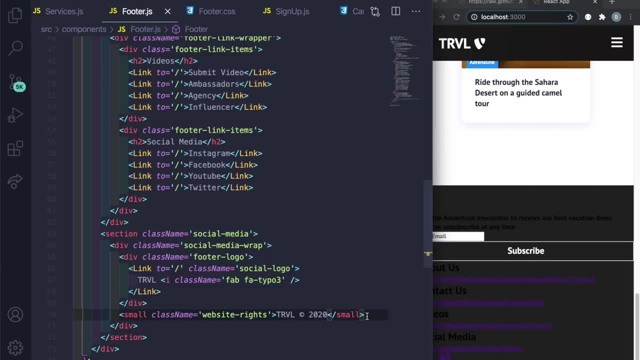 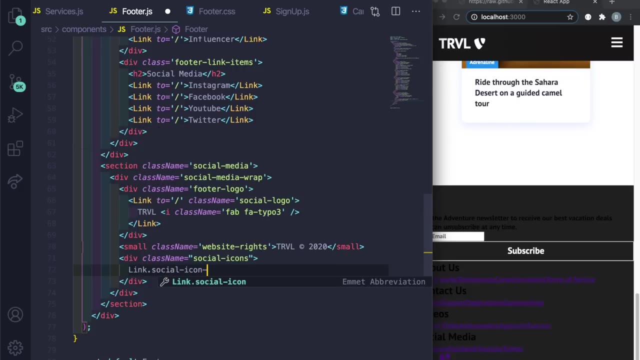 whatever year, and then under here we're going to do dot social dash icons. i'm going to add a link again with a class of social dash icon dash link. now you can customize it by adding facebook to it too, but it's not necessary for this take, but i'll just keep it like this for now to show you options. 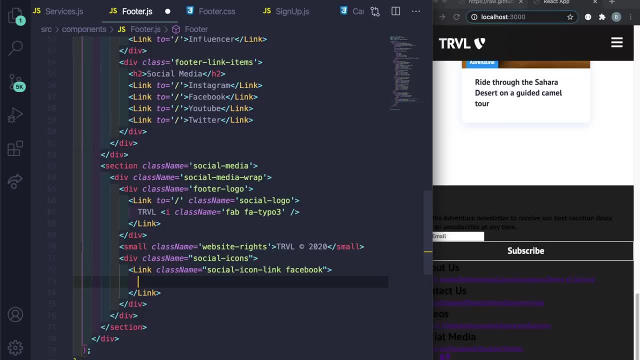 and then basically, if i press enter, i want to pass in i dot f a, b dot f a, dash facebook, dash f, tab it and then pretty much go inside of the link and add additional properties. so class name i want to set: 2 equals 2 slash. 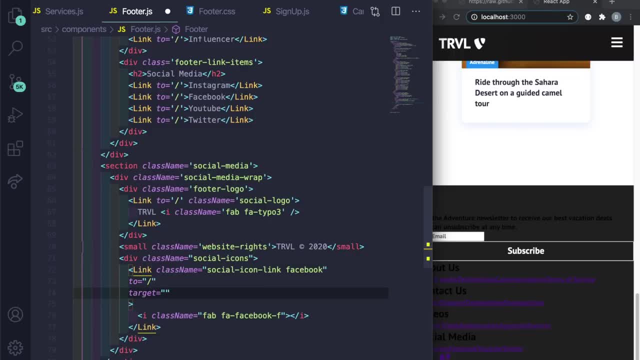 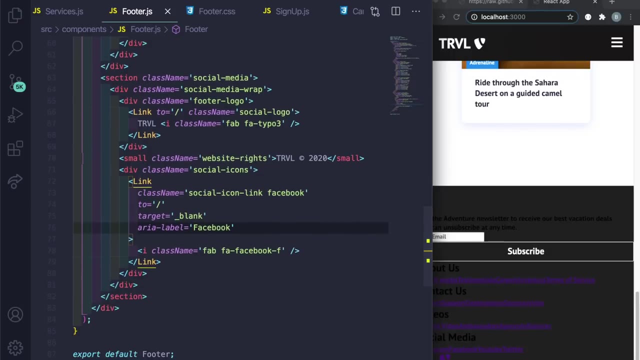 i'm going to set target equals 2 underscore, blank, so this allows it to basically open up into another window and then aria label. this is just an accessibility thing, so put facebook here, save that and pretty much now you just copy and paste this link and then you would just update this. 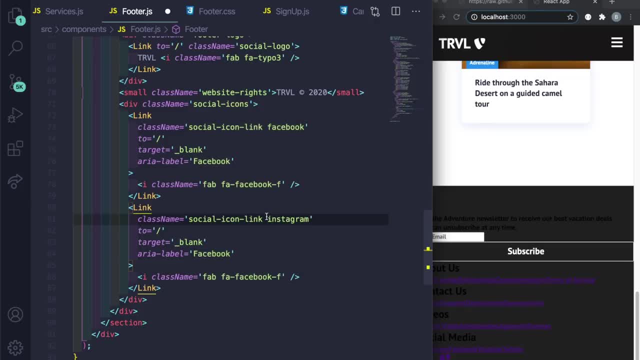 with whatever you want. so let's just say instagram. change this to instagram here. this will be: let's see fa dash instagram. save that here and then we can check our icons below make sure you can see them. they're like super tiny, but yeah, they're working right there. Now, to save some time, i'm going to go and copy. 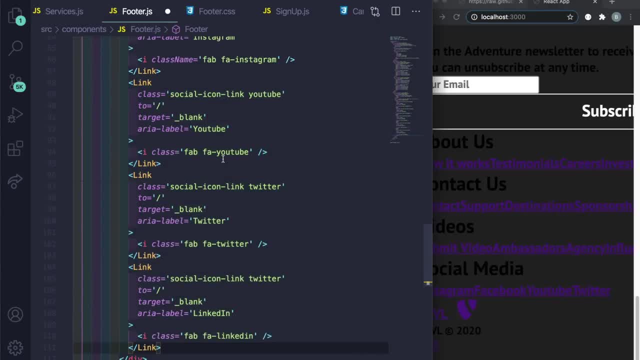 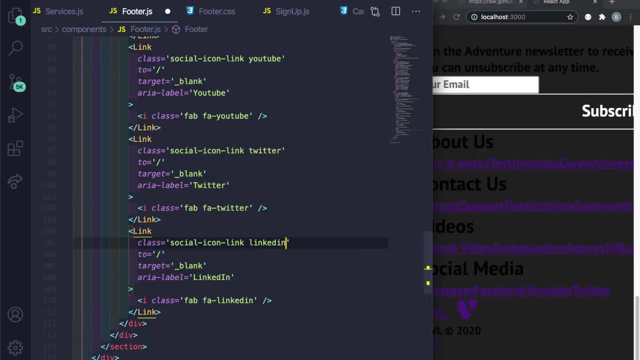 and paste the rest in. so just three more. So you can either copy and paste this, or you can also- and looks like i didn't change this one so it could be linked in- i'll save that and then basically we have it here and now we're pretty much set with the actual uh. 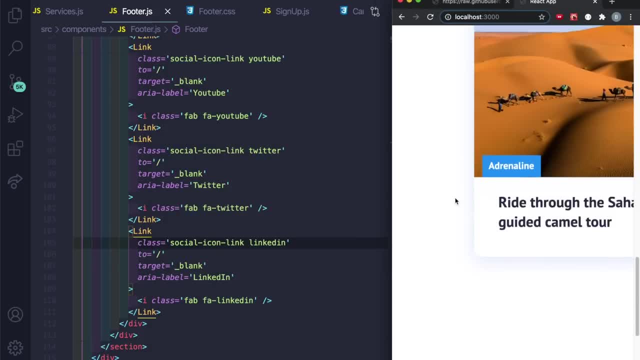 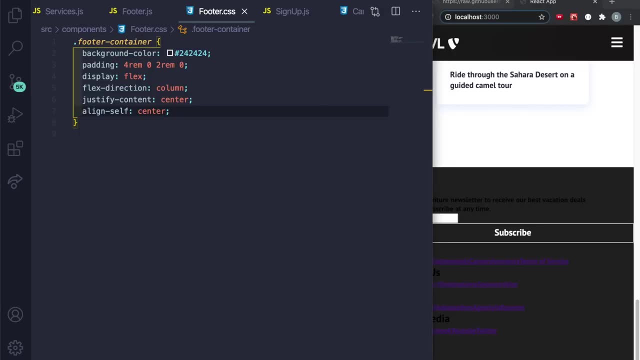 jsx or html, i guess you want to call it. since we're doing react, it's technically jsx. now let's um zoom back out. now let's go to the footer css and let's complete this now. reason i wanted to go through this with you is because you wouldn't. just it would be easier if i show you like what. 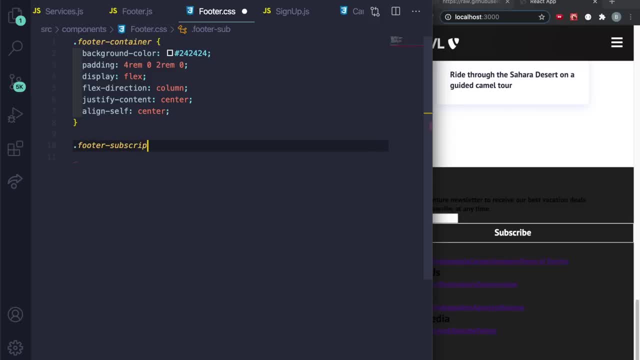 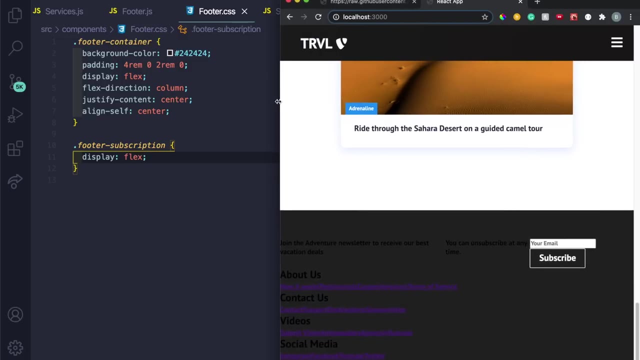 we're doing so. let's see footer subscription and let's do display flex so you can see now the actual um, see if i can make this smaller so that you can see more of it, because right now it's kind of hard to see- and see how it's like. yeah, like this. 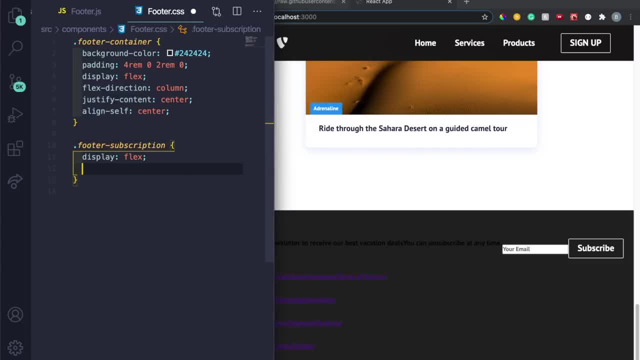 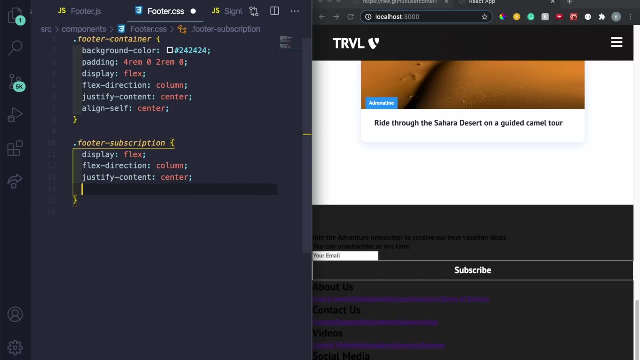 all right, i think that's good, we know. and let's do flex direction now to be column, so now you can see they turned up here. actually this might be a little too much, let me. let me shrink it down more. let me say: justify content to be center, let's do align items center, text align center. 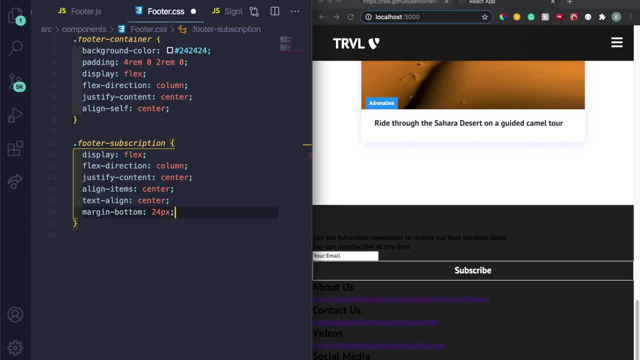 margin bottom will be 24 pixels and then padding 24 pixels, and then let's do: the color will be just white. so now you can see it looks like this. and then let's do footer subscription. let's target the p tag. this is an alternative way to do it, or you can add your own class to it. 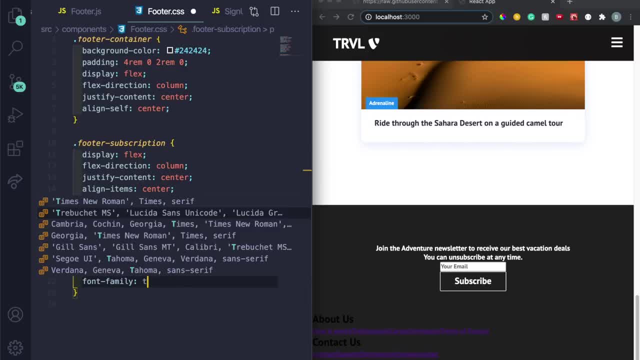 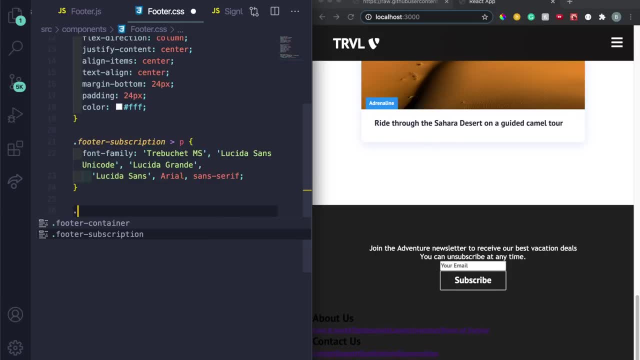 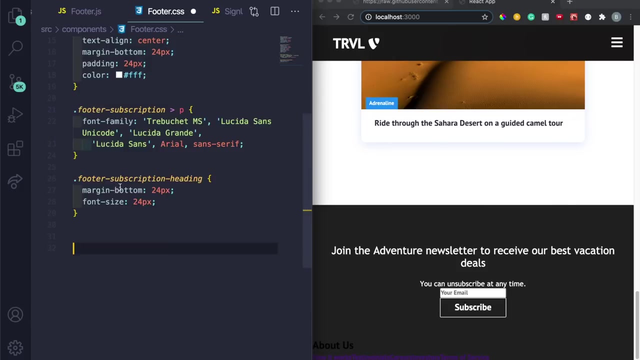 and let's do font family t, which is this one here, so that basically changes that font there. and then let's do footer dash subscription, dash heading. let's do margin dash bottom to be 24 pixels, font size to be 24 pixels, and then let's do um dot footer dash subscription. 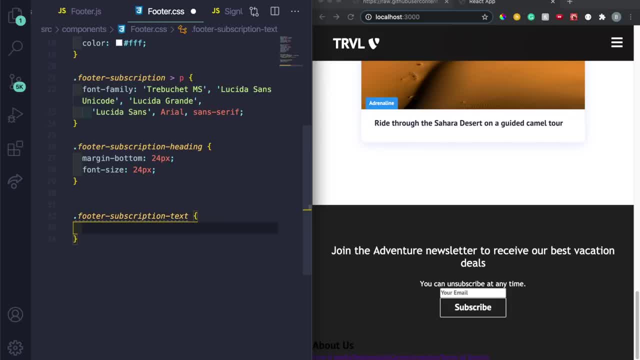 dash text. and then let's do keep the margin bottom the same 24 pixels, but i want the font size to be a little smaller, so 20 pixels. and then the footer input is next. so let's do dot footer dash input. let's say padding to be. 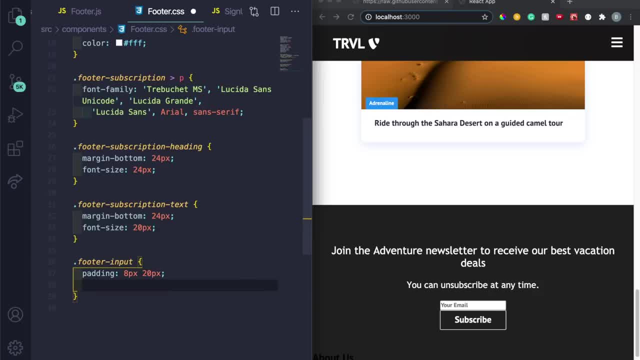 eight pixels by 20 pixels. border dash radius to be 2 pixels. margin dash right to be 10 pixels. outlines going to be none. border is going to be none. font size: 18 pixels. and then let's do margin dash bottom to be 16.. pixels here. 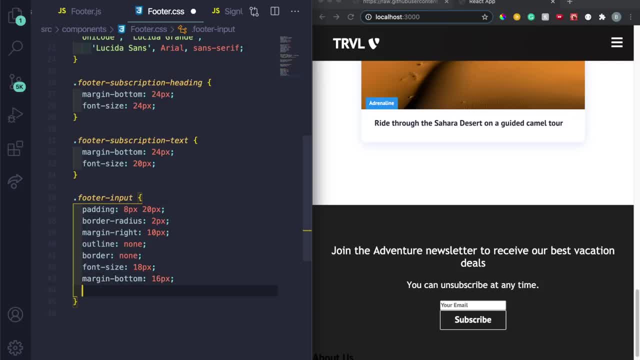 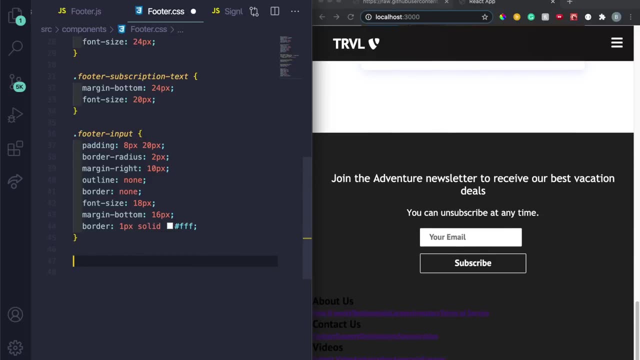 and lastly, let's see border call and see one pixel solid hashtag FF. and now you can see we got a little input action going on here. now let's target the footer links, so for dash links with I want that to be a hundred percent. then let's do max width, so I wanted to not surpass a thousand pixels. display flex. 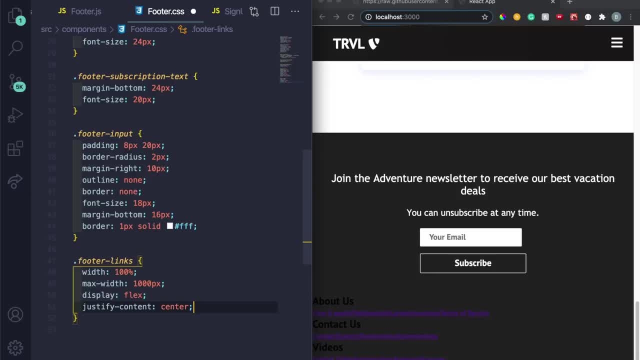 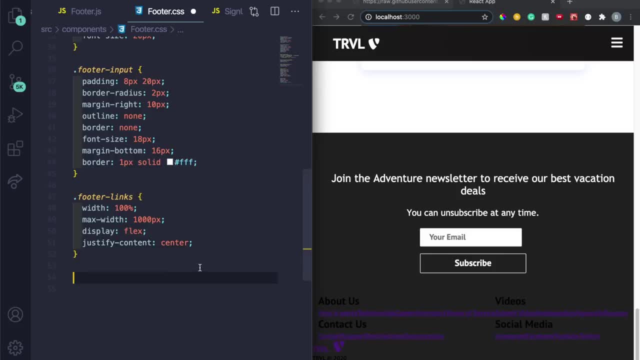 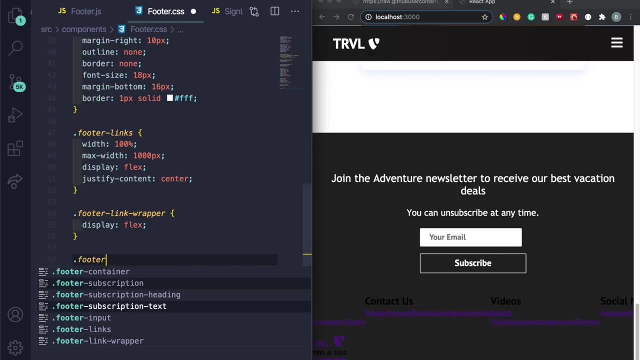 and then just like content Center. so now we got that going on here and see, these are the wrappers. it's basically keeping it in two different um columns and let's do footer dash link dash wrapper. let's just display flex here and then let's do dot: footer dash link dash items. display flex, flex direction. 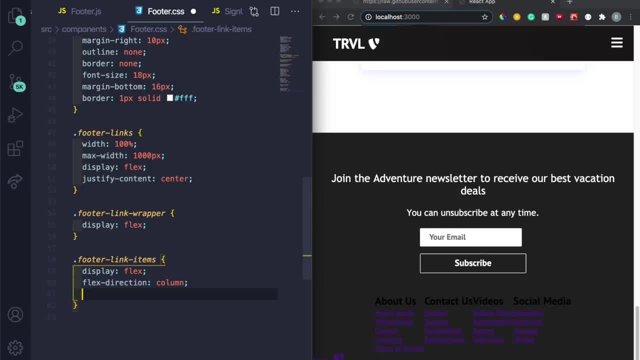 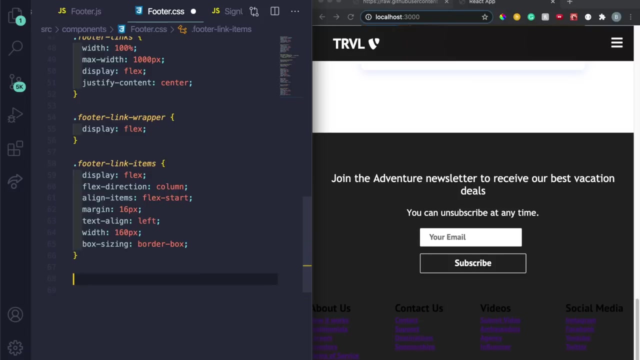 column. and then let's do align items, flex start. let's do margin 16 pixels and text align to be left, width to be 160 pixels, which would be right here, and then box sizing, border box. so now we're starting to get a little looking like a 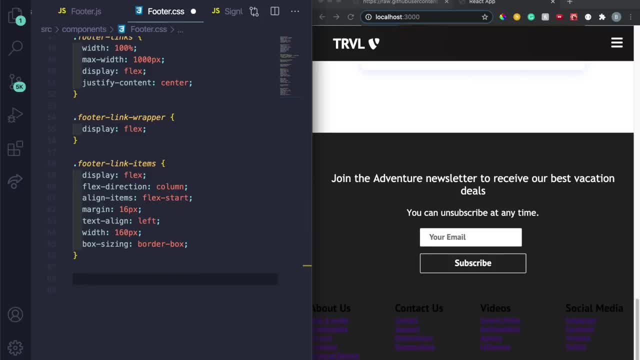 footer. now and now let's target: dot footer dash link, dash items: h2. let's do margin box. these are the titles right here. so let's put 16 pixels, see a little gap. and now let's do dot footer, dash link, dash items less than h2- let's do. 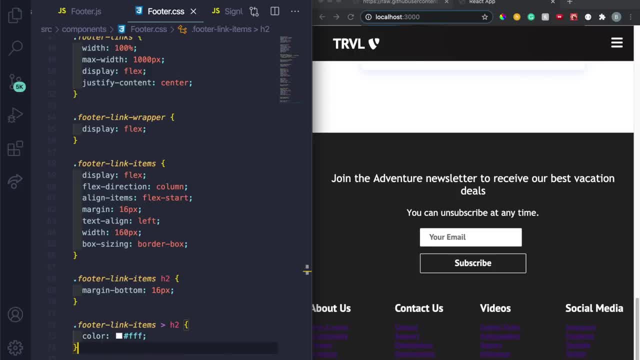 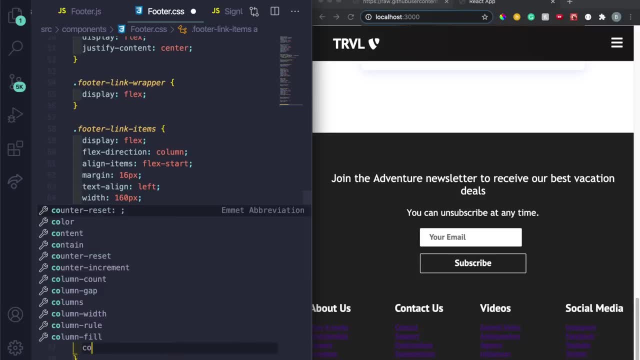 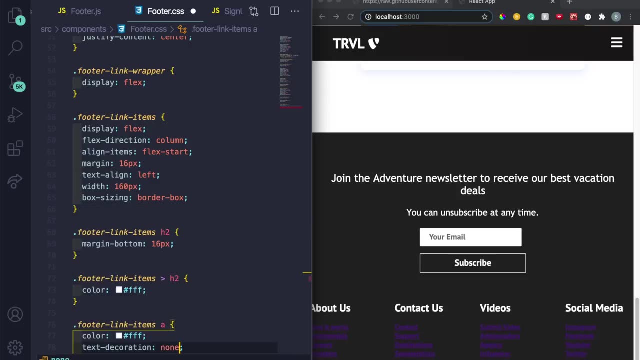 color to be colon: FFF. and then let's do dot, footer, dash, link, dash items. a color to be FF text decoration. if I did this in the lassoiders, in these files let's just say color to be edges. so let's just copy this. actually. 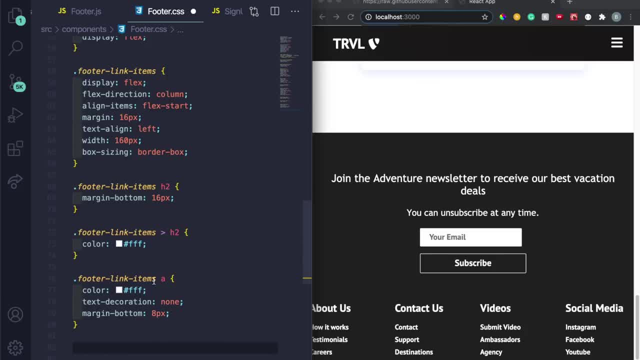 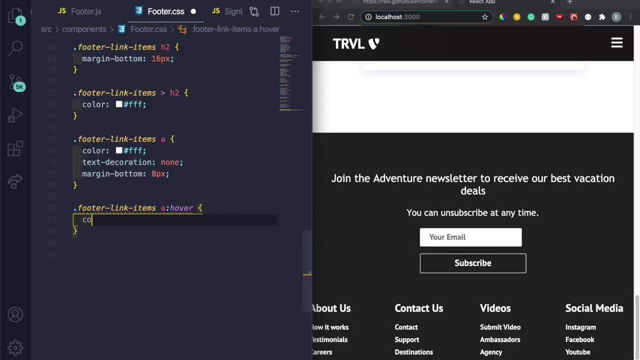 똡. let's just copy this and I'm just going to do everything like I'm going to go and jadi, where do you want��? Then 999? and then let's do transitions, not transform transition to be 0.3 s ease out. 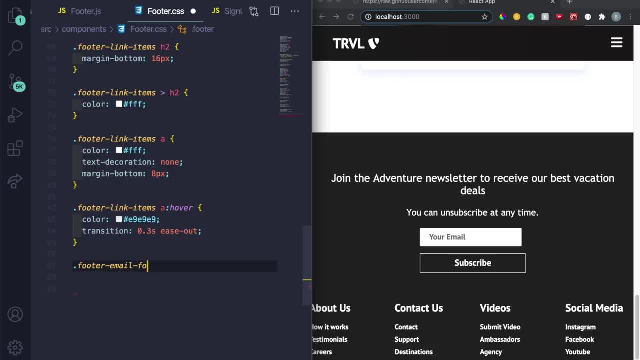 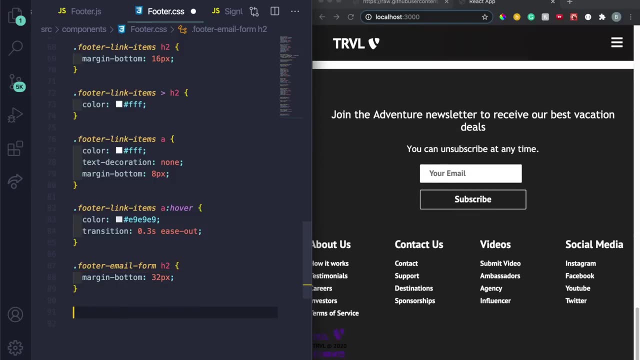 and let's do: dot, footer dash, email, dash form h2, let's do margin dash, bottom to be let's do 32 pixels and then let's do uh, dot footer dash, inputs, colon, colon, placeholder. so now we're targeting the um, the email thing. i should put these up there, but basically doing it here and 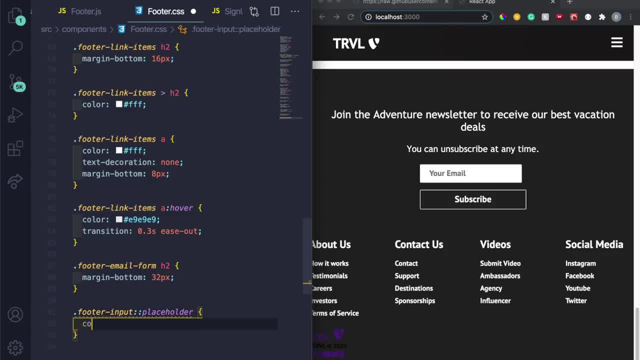 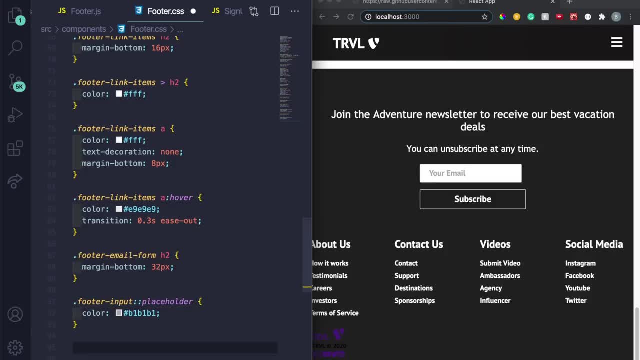 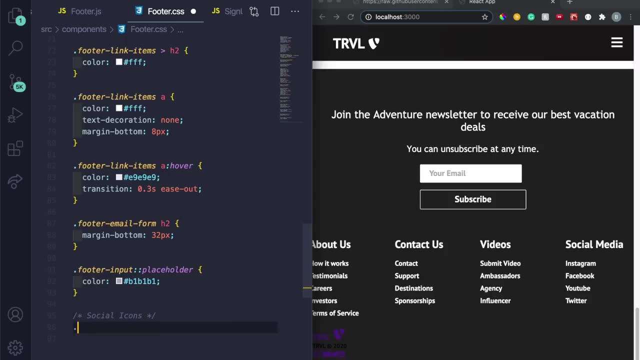 let's just change the your email, the little input color. let's just make it like a lighter gray. so hashtag: b1, b1, b1, as you can see it turned lighter gray and then here essentially the social icon. so let me just put social icon so you understand. here let's do dot: social dash icon, dash link. 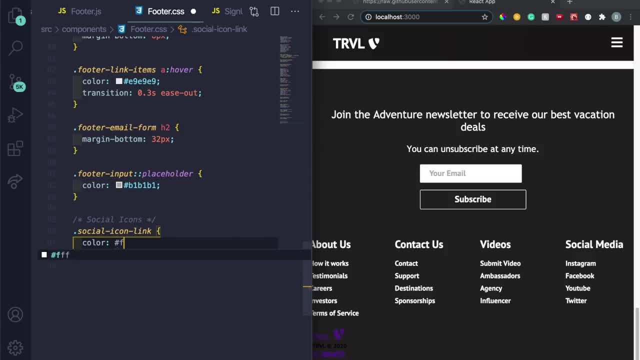 and let's just put the color to be f and then font size to be 24 pixels. dot social media: let's make it the max with a thousand pixels and then with to be a hundred percent, and then let's do dot social, dash, media, dash wrap. let's do display flex, justify content. 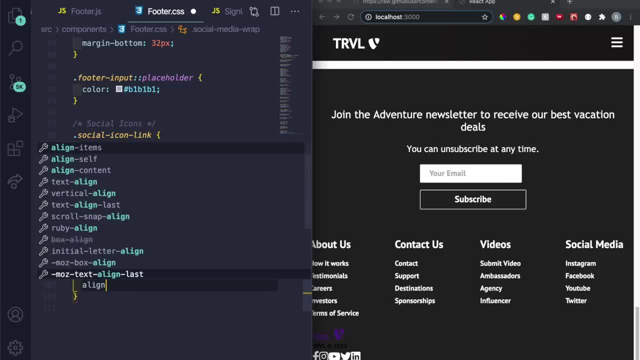 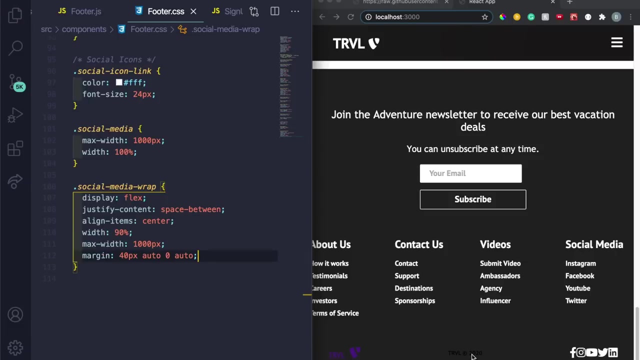 space between line item center width is 90 max with a thousand pixels, and then margin: 40 pixels, auto, zero, auto. so now you can see you got a nice little clean set up here. and then let's do dot social dash icons referring to the buttons display flex, let's do justify content space between a line item center and then i put a width. 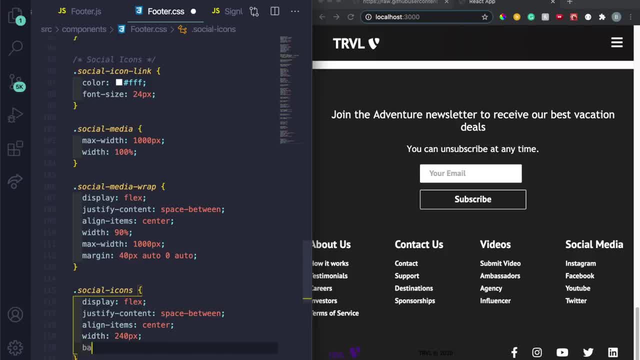 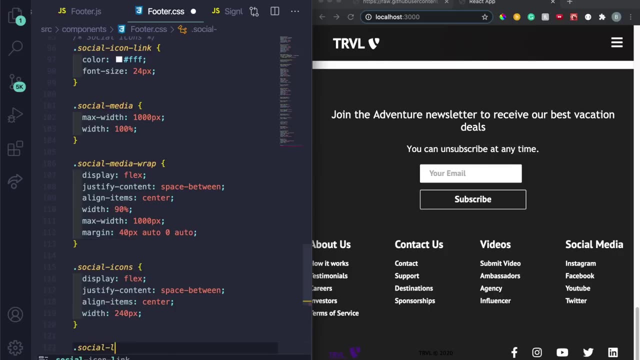 of 240 pixels so that they space out like that. and in case you're like, what is going on? basically, if i put a background of red, that's what we just did right there. so i set the width to 40 so that it to justify content and let's do, uh, see that social dash logo and yo, if you're still watching this, 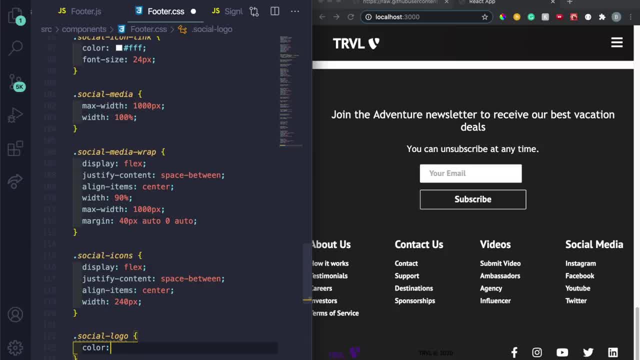 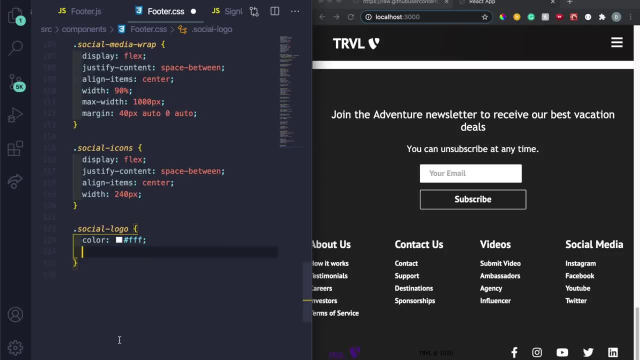 video right now. hit that like button just so i know who's staying strong. you know this video is quite long, so let's go color here. fff, let's do justify self. i'll put self here. let's just say: start: margin dash left to be 20 pixels. cursor pointer text decoration to be none. 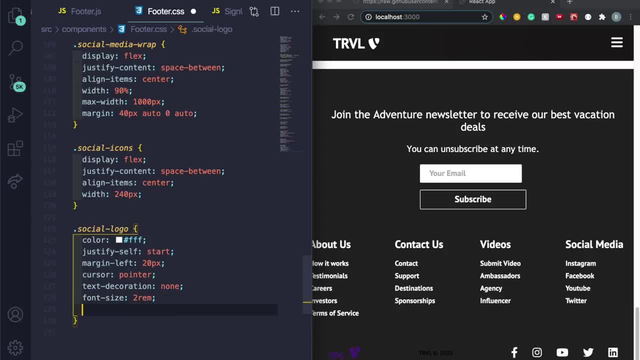 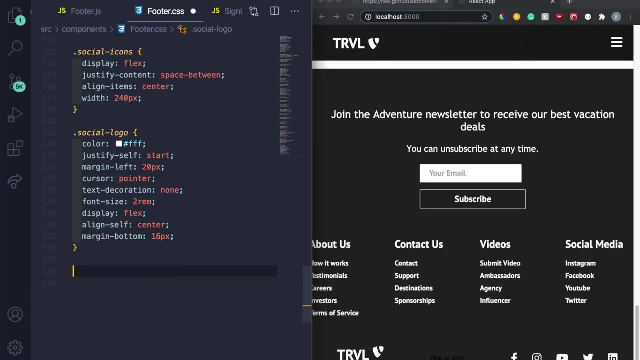 let's do font size to be 2rem, display flex, align items to be the center and then margin bottom to be 16.. pixels- okay, get in there, we're getting there. and let's do the last one before we do the mobile response parts. website rights: color to be whites, margin dash bottom to be 16 pixels. 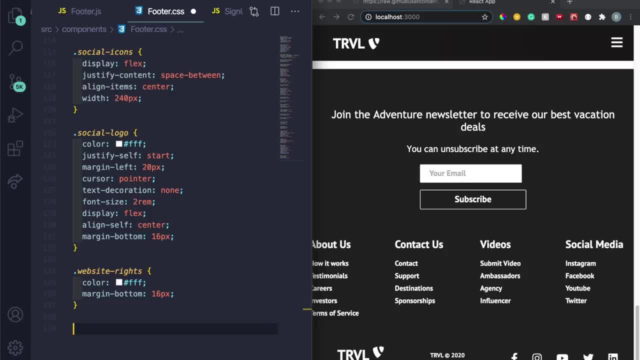 and now let's start editing the mobile part, which is really really basic, but i did it here, so let's do add media screen and and most of the code is already like set, so the media queries. i have my breaks at 820 pixels but, depending on your screen, i'm going to say dot footer dash links to be padding top of 2. 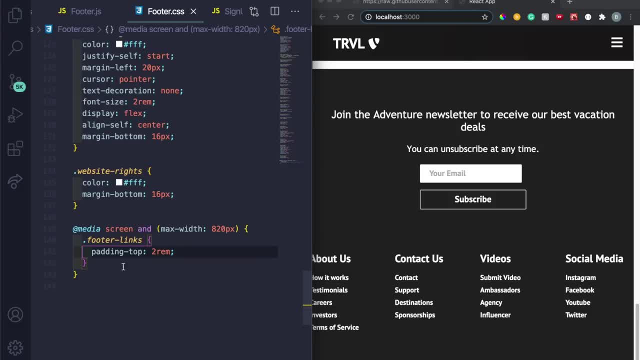 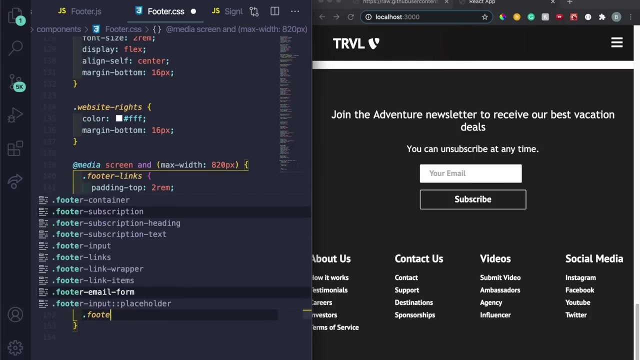 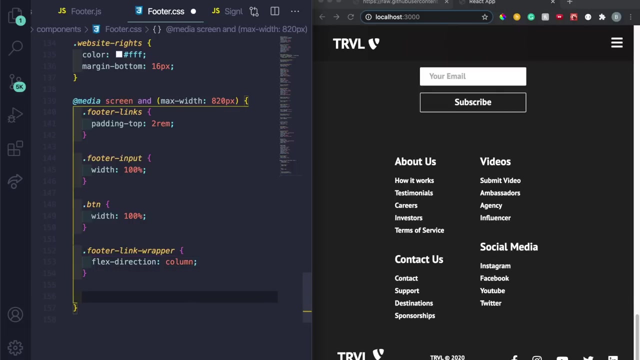 rem and then dots footer dash inputs to be width of 100, to be width of 100 percent. that BTN is going to be with of a hundred percent. dot footer dash link dash wrapper will be flex direction column, so this is essentially what makes it mobile, pretty much so this is where you see that. and then dot social dash. 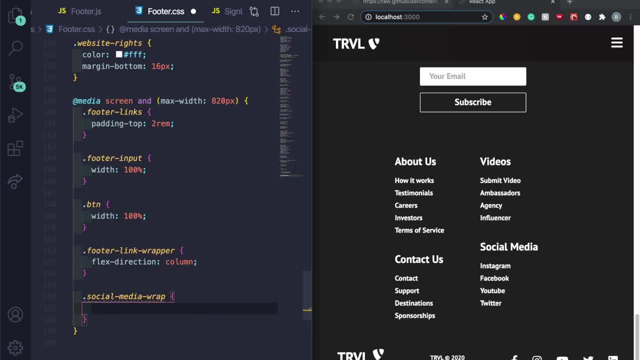 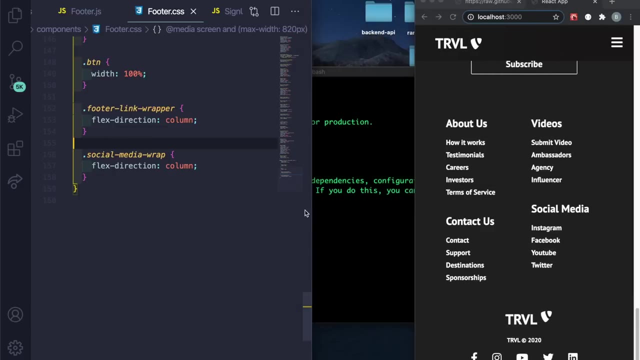 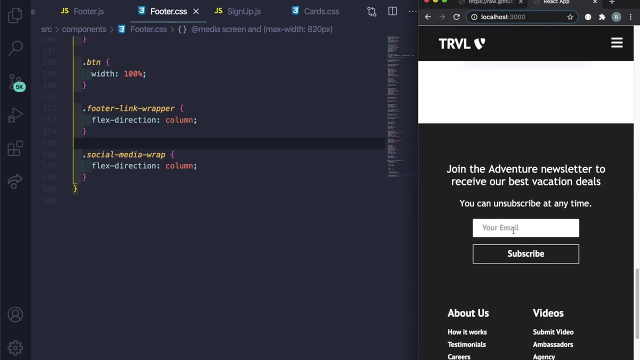 media dash wrap. same thing, flex direction column. so we have that nice little mobile responsiveness and then when we shrink everything down, it pretty much- let me shrink this- looks like this and we're pretty much set to go in terms of mobile responsiveness and everything. so now let's just check out the sites and also: 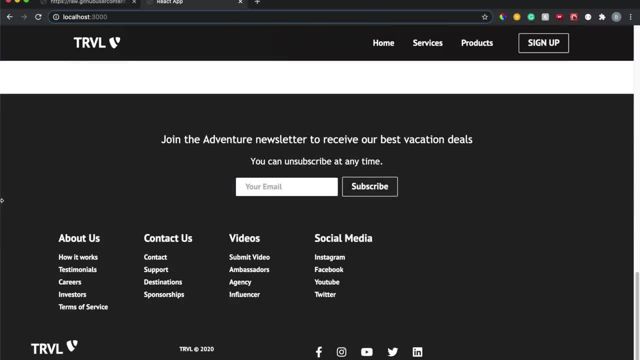 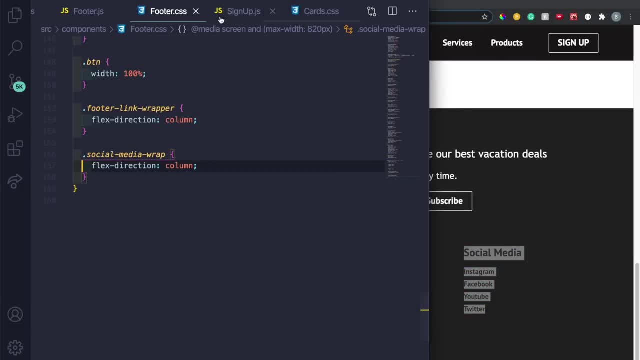 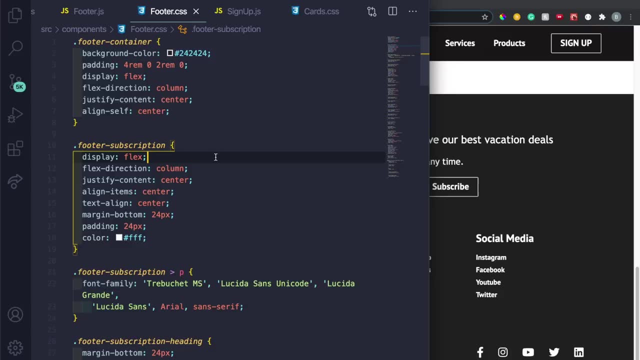 let me show you something. looks like. it looks like: uh, I guess this would be outside of a div, so let me make sure, let me check, make sure my codes right, as I realized it was on the top. um, for the container should be a line items, not self making me go crazy for. 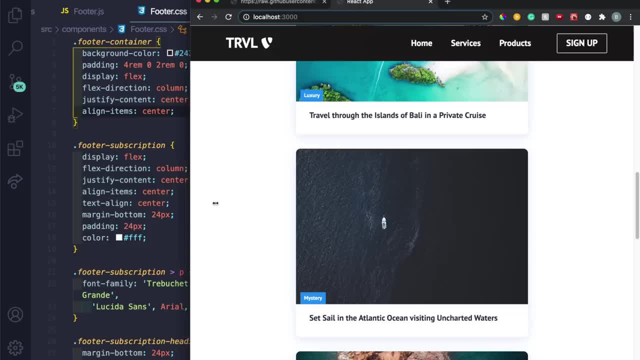 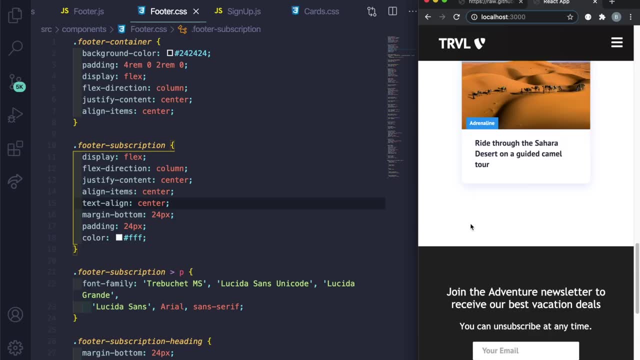 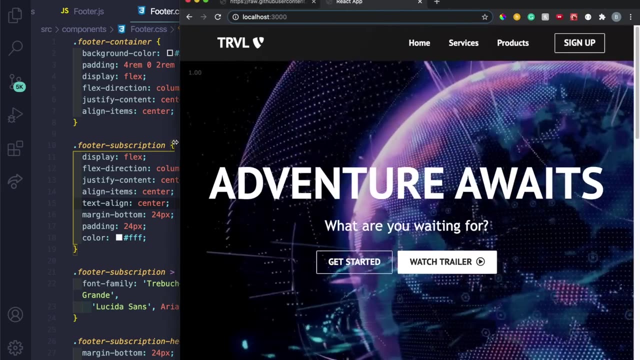 that. but basically we have it where it's like this and everything shrinks. make sure, shrink it down and look at nice and clean, all right. so now let's go ahead and go check the menu. so let's go back and let me show you how I added the. 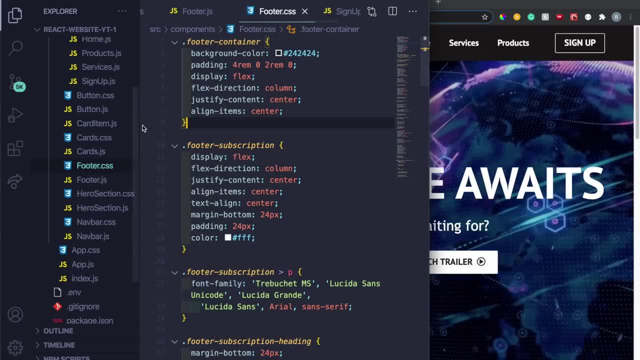 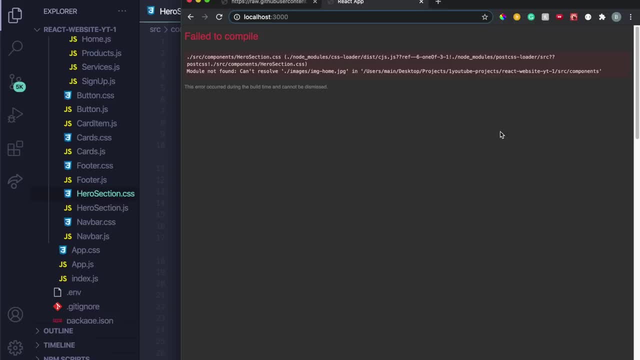 image, in case you're like: I don't want a video, so let's go back really quick and let's check out the home section CSS. let me go here, let me uncomment this out and then right now it's going to say something like this: so let's see. so the reason it's saying this. 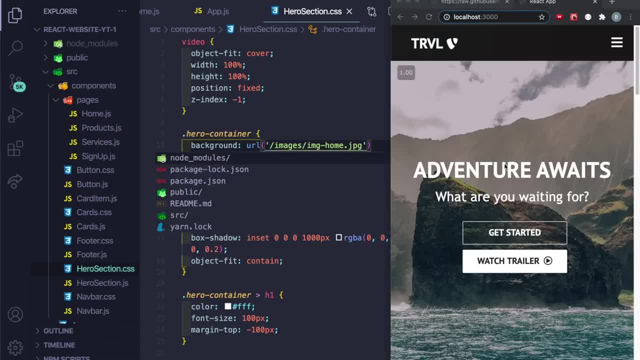 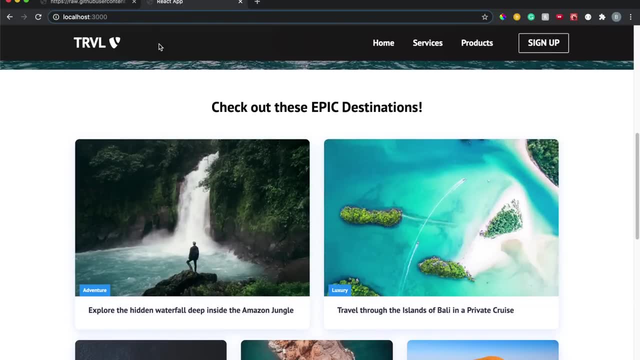 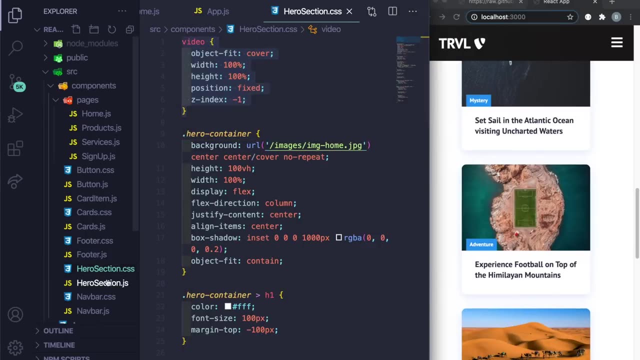 is because I just need to add a slash in front of it and boom, now we basically have a picture image and also you can see that the um, the net bar still there, and then all you would do is just basically delete this video code here and then go here: you can just delete this code. 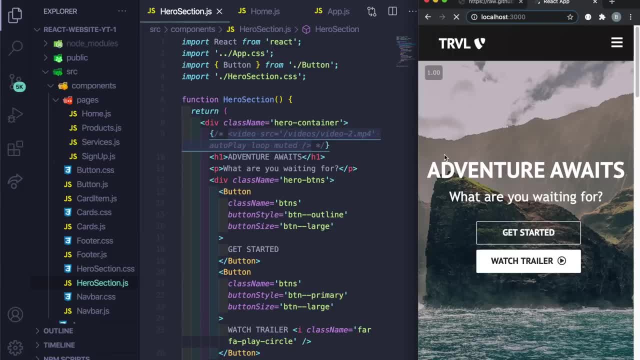 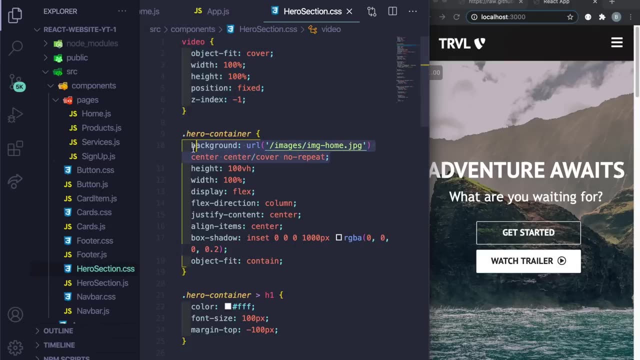 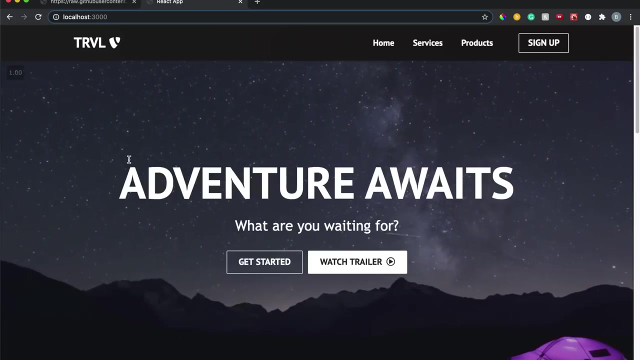 here, or you can just comment it out and basically you can see at the video now and the background is not there anymore, nice and clean, and then if you ever want to switch out the video again, just video one here, go to section, do this, comment this out and boom. so this pretty much completes the video for today. so if you, 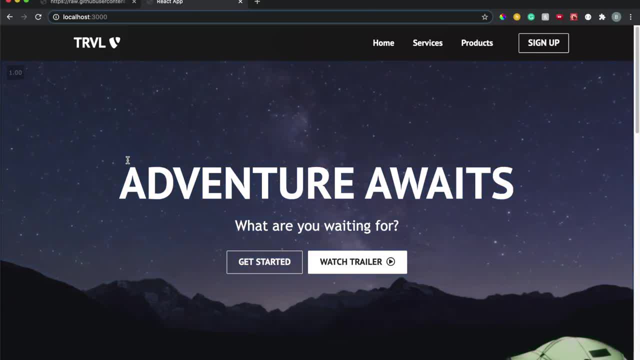 did enjoy this. definitely it will help a lot if you go down below and give this video a thumbs up. share this video with your friends or anyone that you think will find value in this comment down below what you think. also, feel free to refactor the code, make it better, because at the end of the day, I'm just 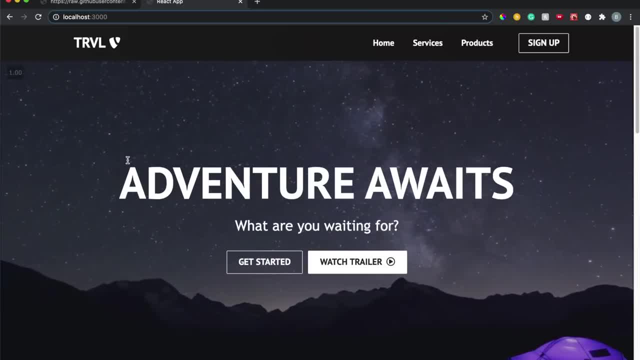 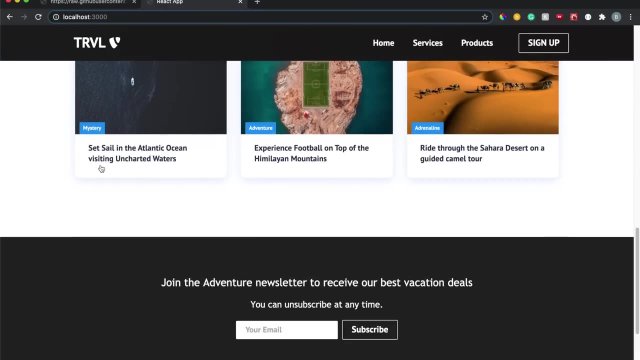 docking myself, learning code and showing you guys what I'm building and you haven't already. you'll go down below, hit that subscribe button, comment down any other video ideas I should work on and, aside from that, I will see you in the next video. peace.